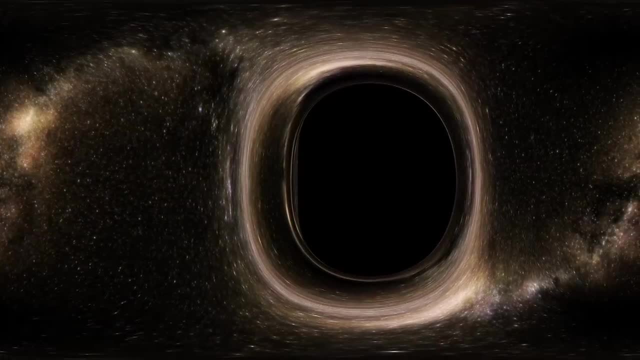 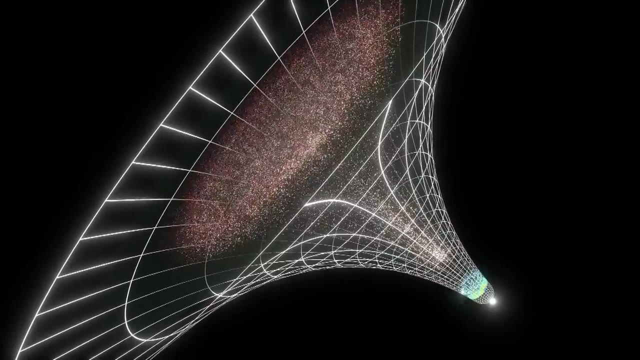 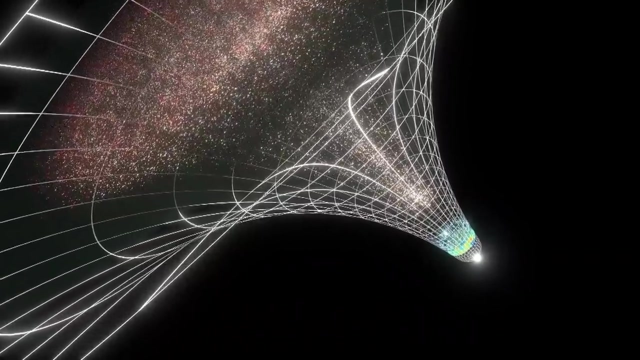 Inside a black hole lies a mystery. What happens at its center? The same mystery applies to the Big Bang. Einstein's theory of gravity seems to give way, predicting the existence of a singularity, a point of infinite density, curvature and pressure, When the entire observable 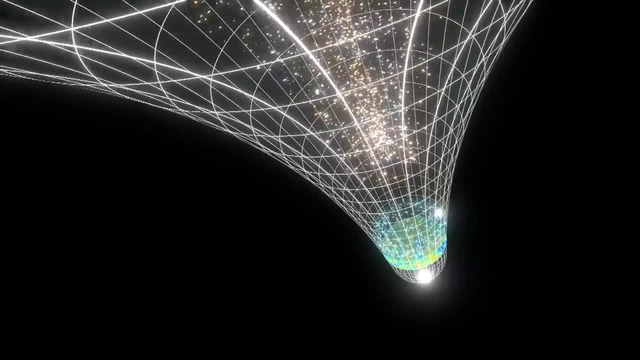 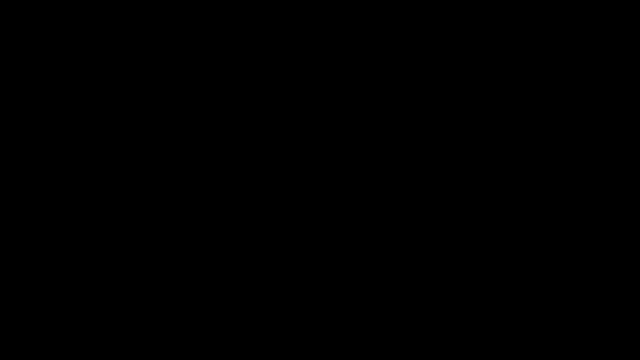 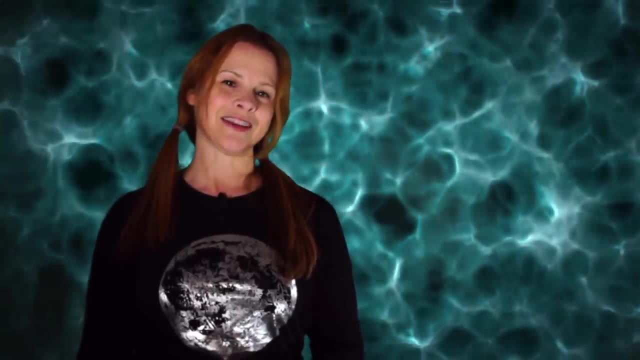 universe is squeezed into a space far smaller than an atom. new physics is needed, taking account of both gravity and the strange microscopic world of the quantum. We need a quantum theory of gravity. One of the leading candidates is loop quantum gravity. In this film, we'll 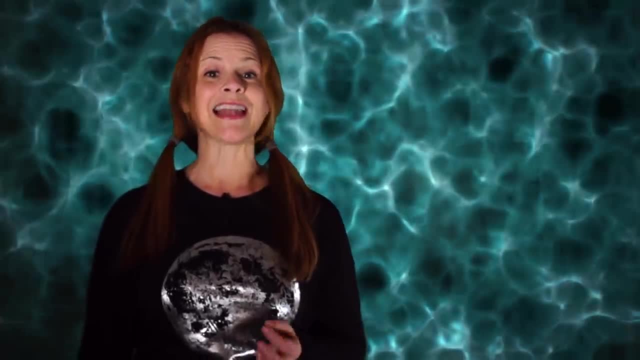 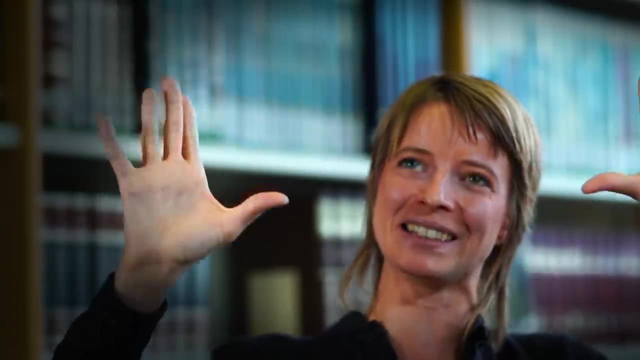 tell the story of this theory, how it was developed and how it might finally be tested. We'll meet some of the key players in the field, from the younger generation of scientists to the founders of the field, including Abhay Ashtekar, who, even as a teenager, 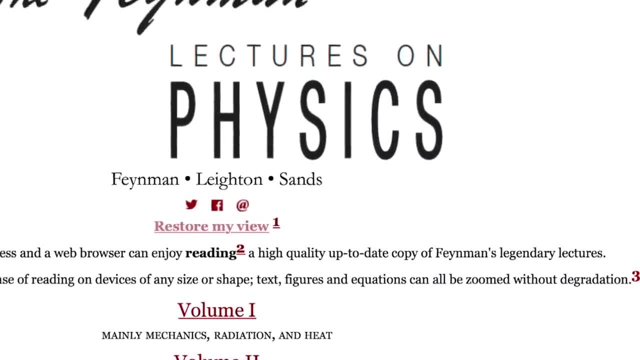 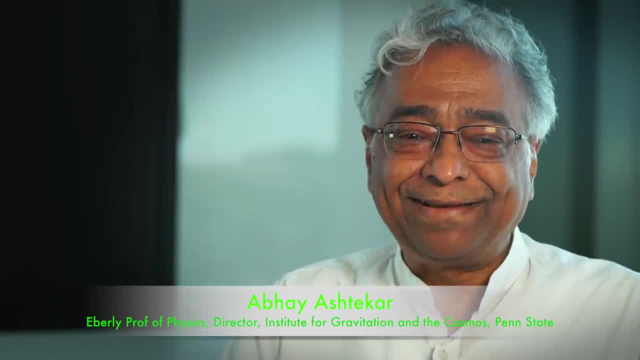 found a mistake in a textbook written by Nobel Prize winner Richard Feynman. Well, being a little bit brash at that time, I decided to write to Feynman, And I didn't really expect that he would reply, but I was a bit surprised that he did. And he said something. 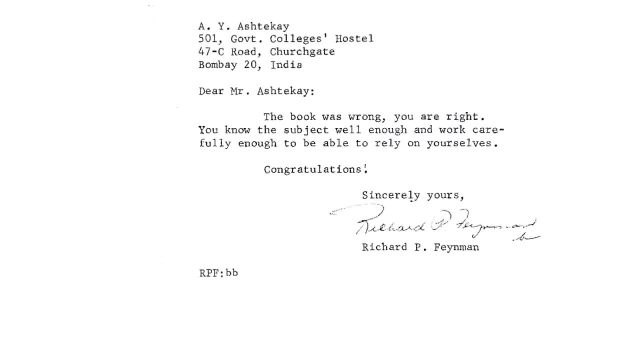 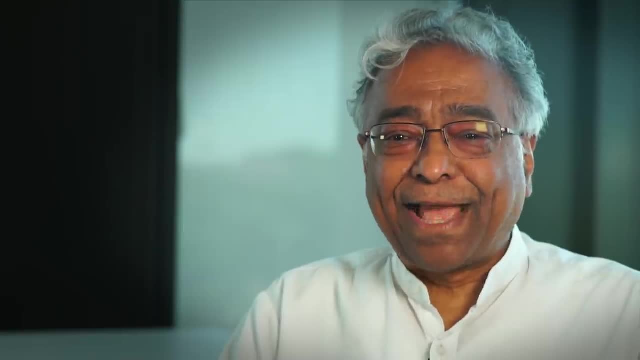 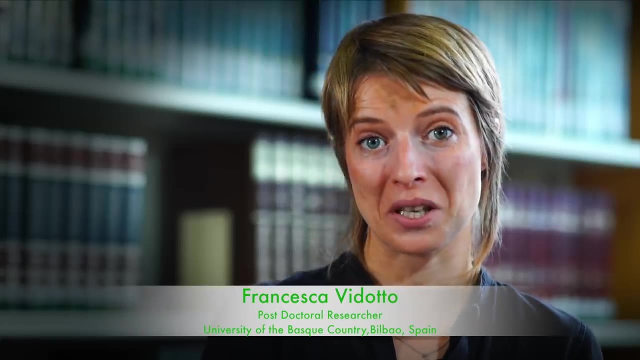 like you know, congratulations. the book was wrong, you're right. But then he also ended basically by saying you can rely on yourself. I think this was kind of a subtle note saying I shouldn't keep A passion for astronomy was there since I was a child, The first book I remember I picked- 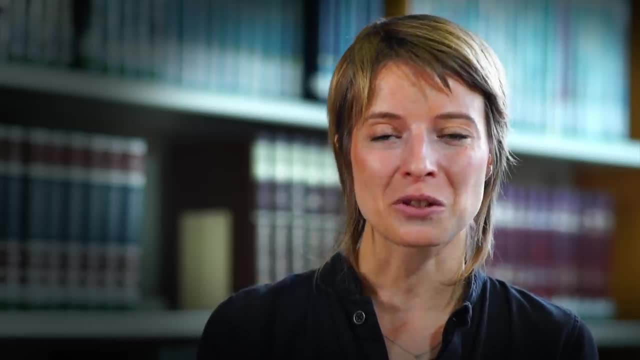 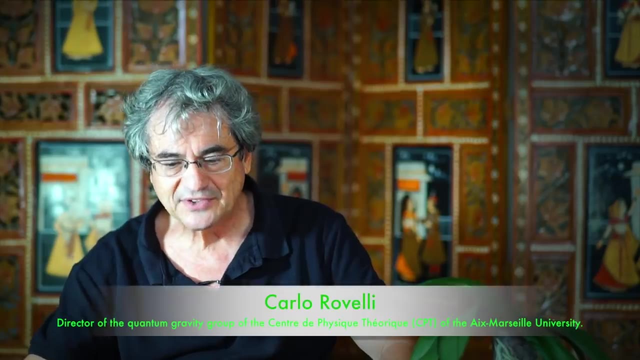 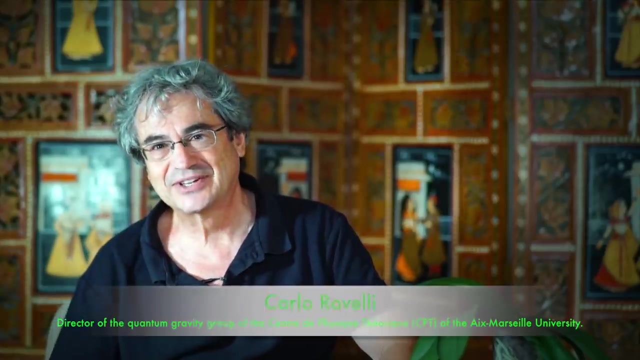 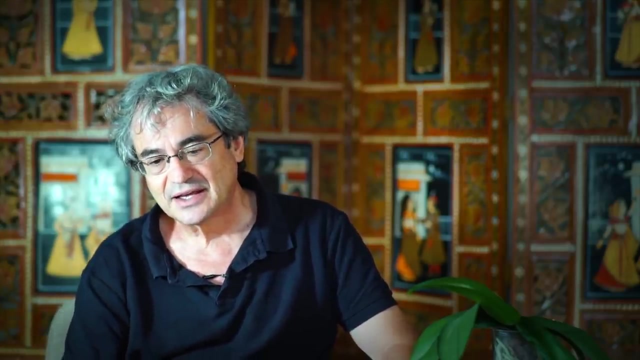 up myself from the bookstore was about astronomy And the other one was about cats. So I was a cat and star person. I count myself fortunate for having read and spent time in going intellectually in various directions. Then I got completely enamored. It was a very simple question in physics. I sort of got in love with physics. I remember 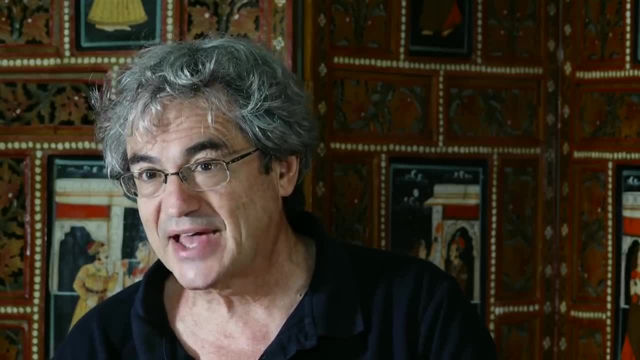 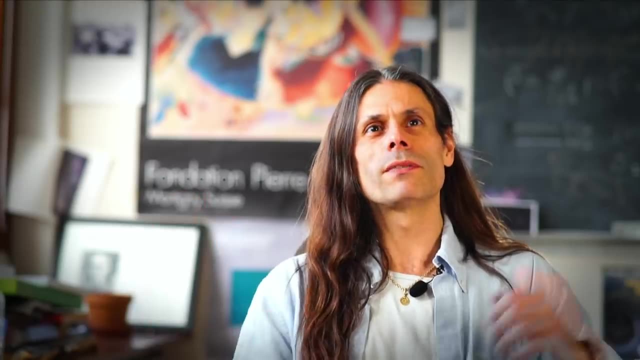 distinctively. at some point I said: this is so beautiful, Maybe I want to do that in life. When I was very young, I wanted to be a researcher in biology because I was really interested in animals, plants and all the living world, And then I switched to physics. I don't really 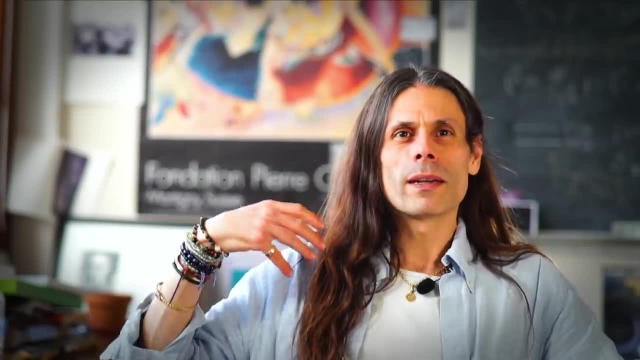 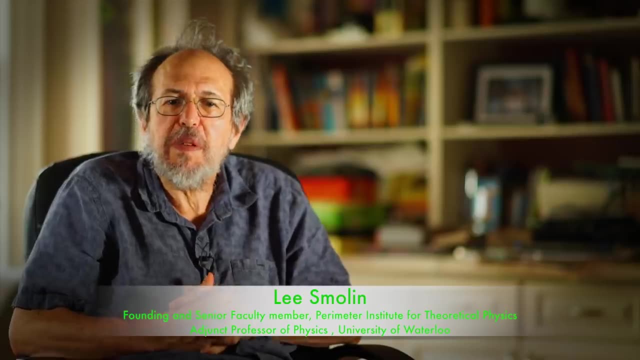 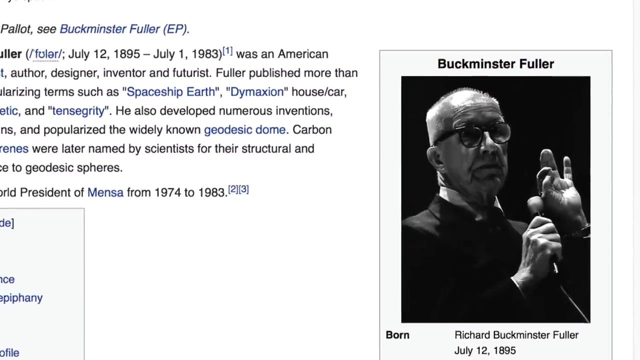 know why, probably because it was even stranger to me. It was a desire to go and to see what cannot be immediately seen through architecture. I got interested in architecture because of Buckminster Fuller, who was the great visionary and ecologist and engineer and architect, So I thought that I would. 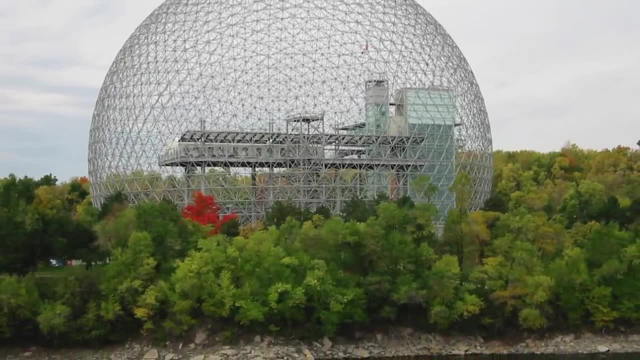 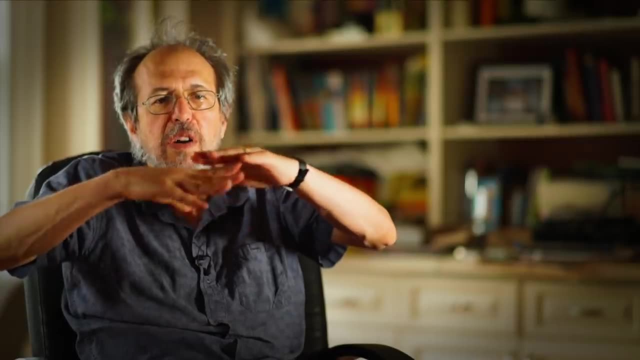 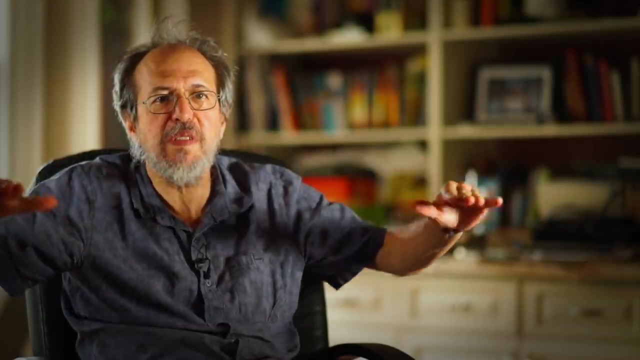 design greenhouses and swimming pool covers and second homes and things like that out of geodesic domes. but I had this idea and I'd written a code, a program which could stretch a geodesic dome and basically make a triangulation out of any curved surface. Little did I know that that would be what. 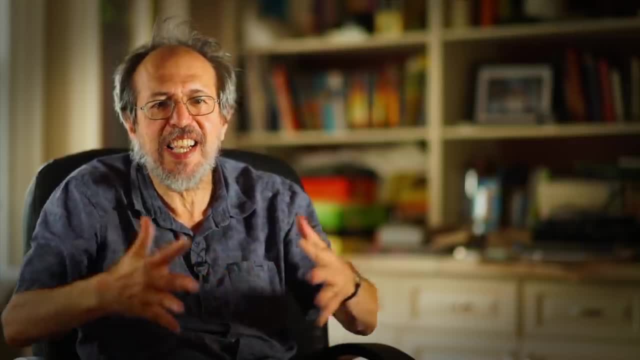 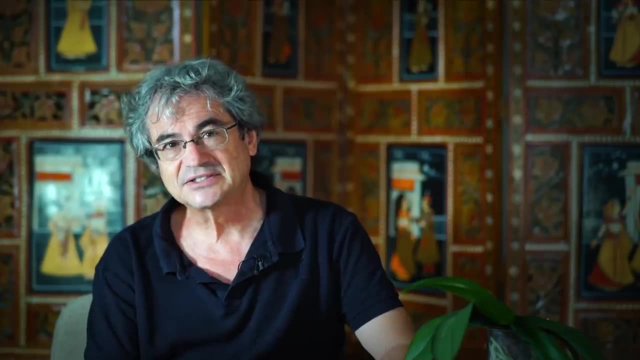 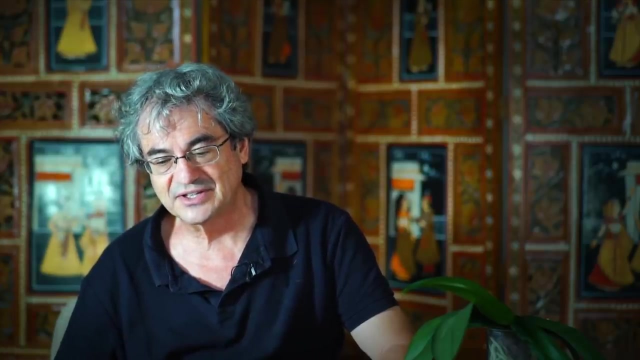 I would be actually doing in science years later. The realization that there was a problem with quantum gravity is by Einstein Immediately after having done his theory generativity. he wrote the main equations of generativity in 1915, and one year later, in 1916,, he writes this: 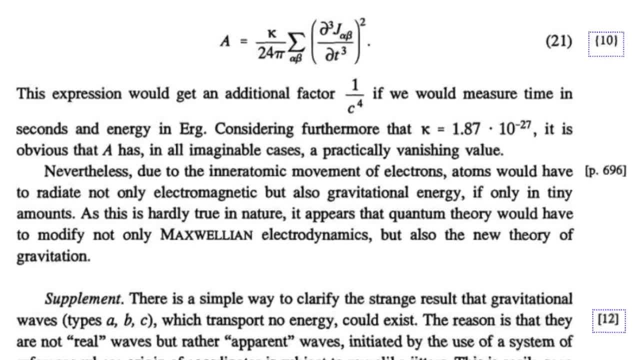 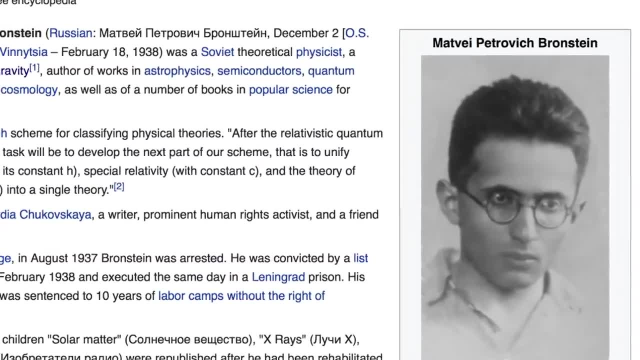 paper saying: well, actually, by the way, this cannot be the end of the story, because there is quantum theory. Matvei Bronstein, a young physicist, a friend of Landau, who, in my opinion, is the first one who 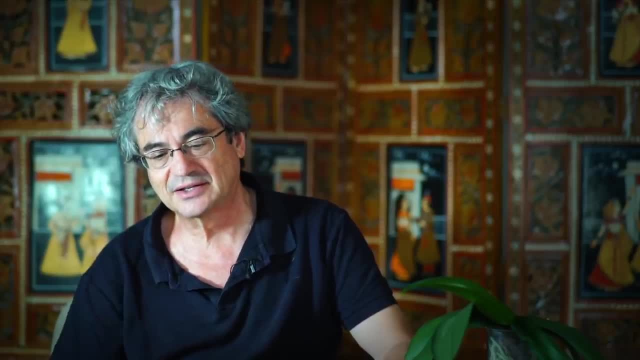 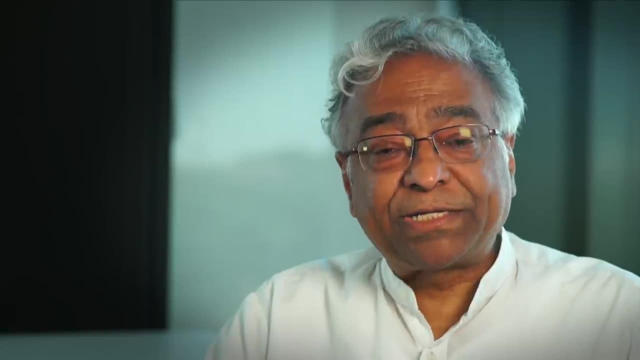 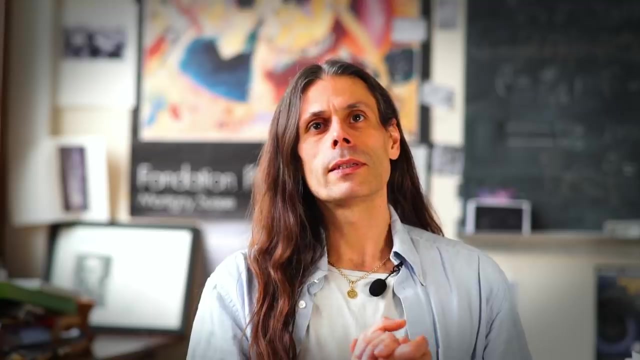 had full clarity about the deepness, the depth of this problem. So in the beginning people like, particularly people like Feynman and Bryce David, he tried to incorporate, tried to generalize the methods that had been used in quantum electrodynamics to gravity. It's quite usual in physics that we 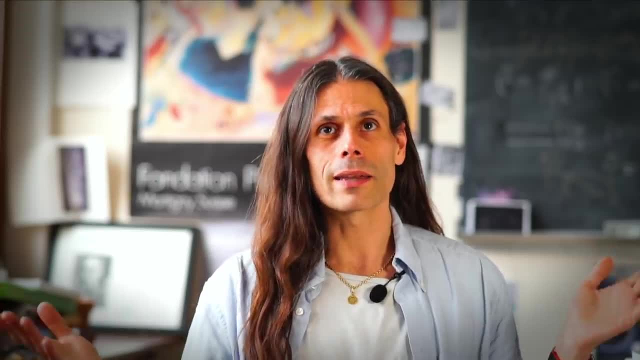 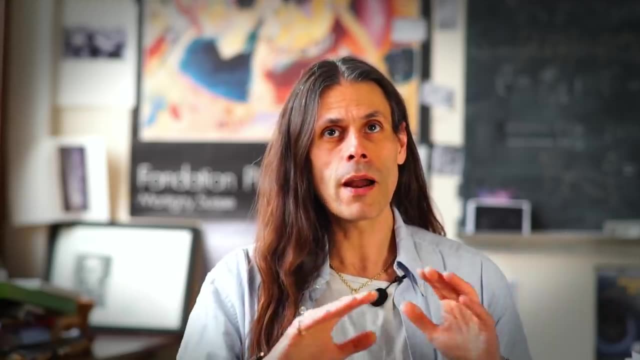 end up with infinite quantities. The problem is that nature doesn't like infinity. So renormalization is a technique that was invented to get rid of those infinities and it works very well and it leads to measurable results. But for gravity it turned out that 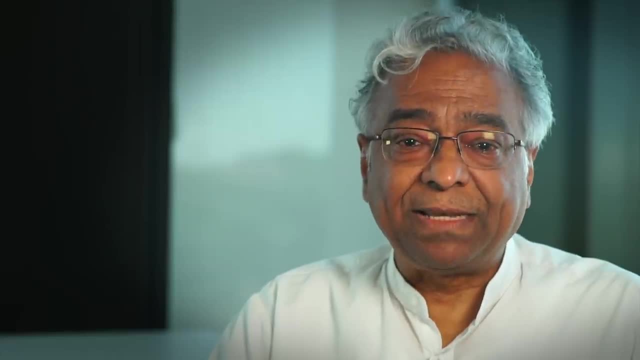 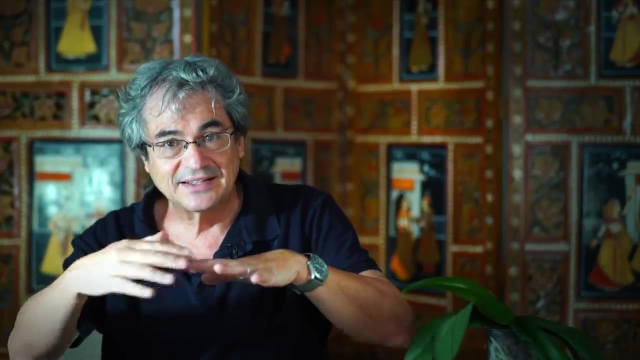 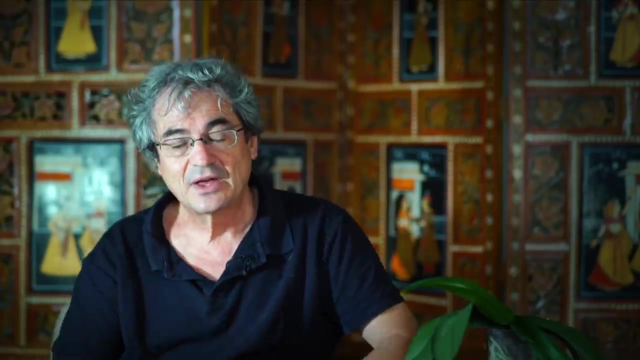 the theory is not renormalizable and therefore these ideas ultimately had a real roadblock. Usual physics is done with space and time and the physics happens in space and in time. So to say, the space is there, it's given, While in quantum gravity space itself 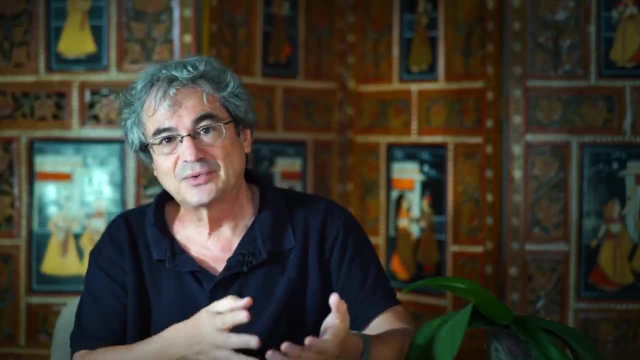 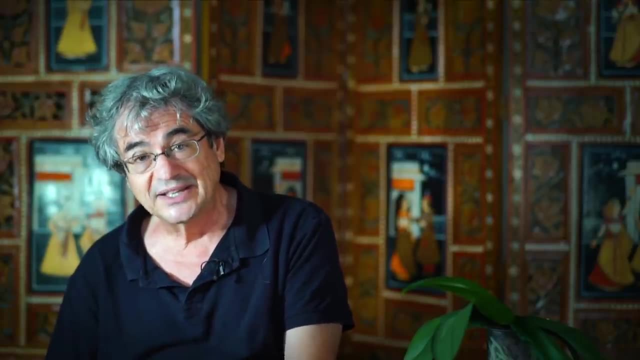 that becomes a quantum object. So the usual technique of quantum field theory don't work And I guess the breakthrough in the 60s was by John Wheeler and Bryce DeWitt who wrote with this very famous equation, which is the Wheeler-DeWitt equation. 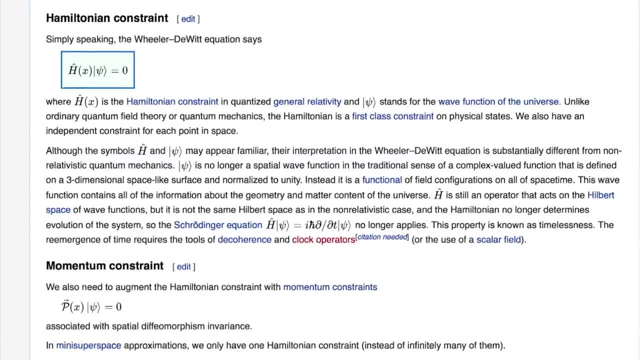 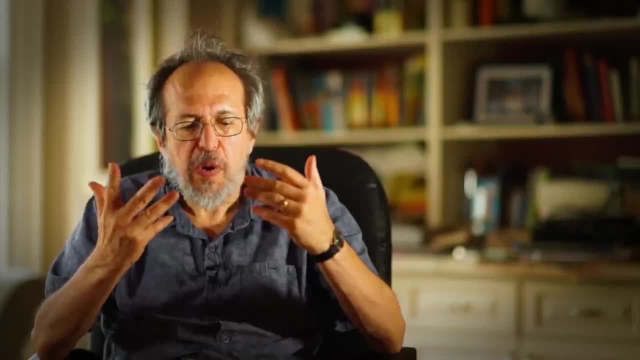 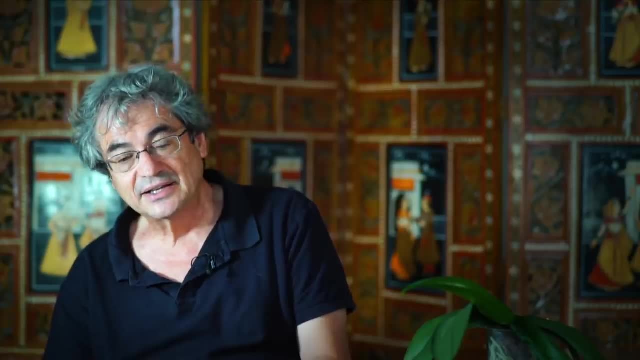 The Wheeler-DeWitt equation was an equation invented by DeWitt, by Bryce DeWitt, which is like the dynamical equation of quantum gravity. It's analogous to the Schrodinger equation of quantum mechanics. Wheeler-DeWitt equation is not well defined mathematically, but full of ideas And 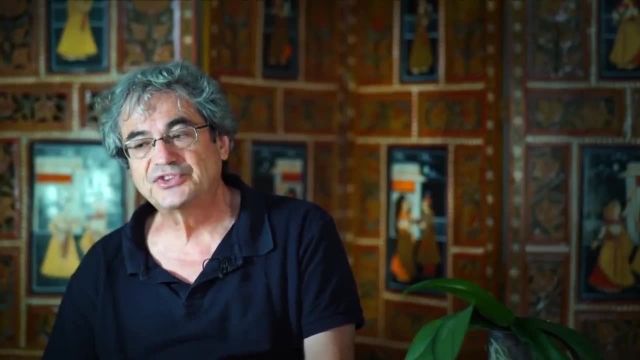 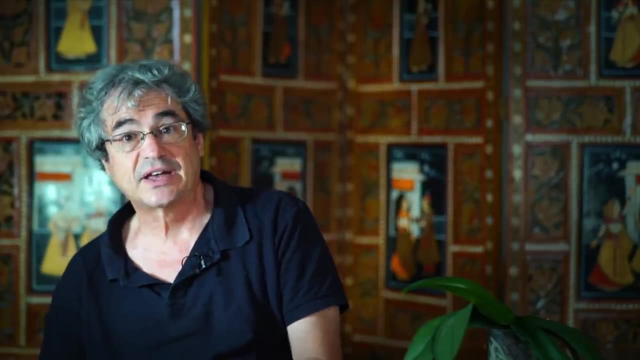 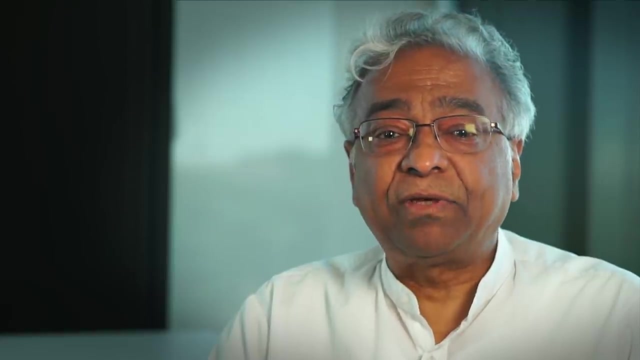 people at the time, especially John Wheeler, produced a lot of the intuition that later on became the driving force for quantum gravity. John Wheeler in particular was much more interested in also issues having to do with singularities of general gravity. He often emphasized an analogy with hydrogen atom. 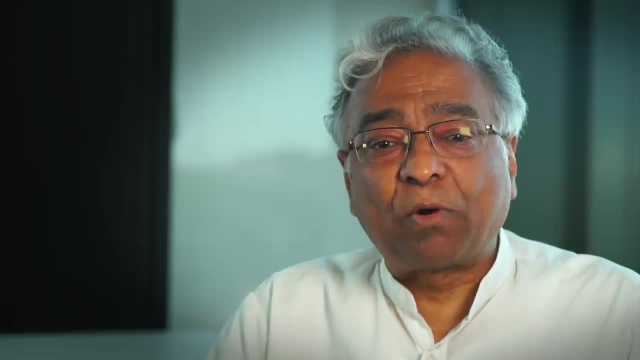 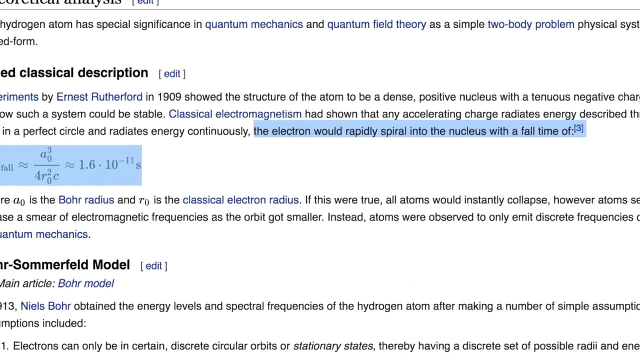 See for the hydrogen atom. if you ask for what is the lowest energy available to it, then the classical theory that lowest energy is minus infinity. But that is an artifact of ignoring quantum physics. So Wheeler was convinced that singularities of general relativity 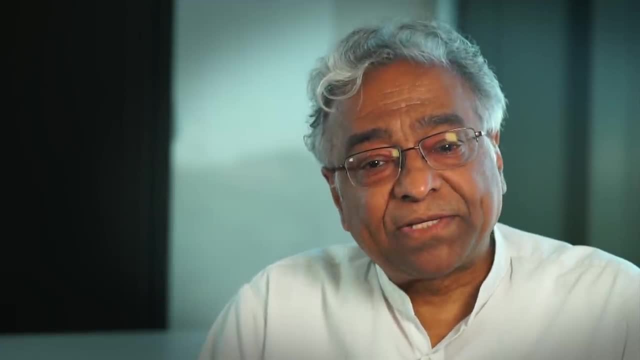 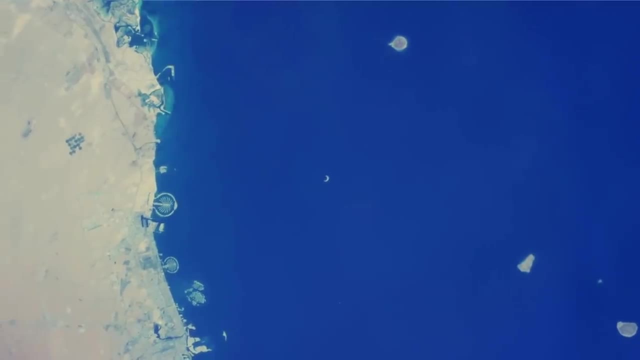 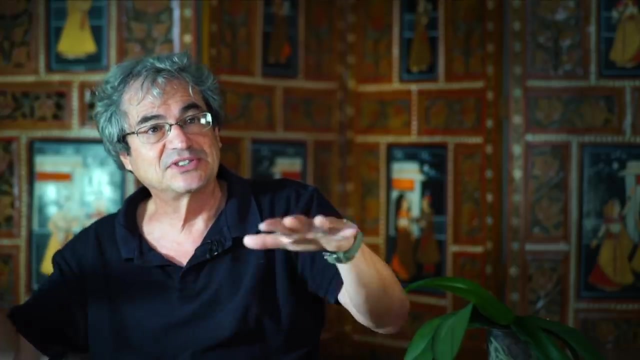 are really artifacts of ignoring quantum effects Here. this picture: if you, if you, if you look at it, if you fly over an ocean at very high altitude, you see the ocean as a flat surface. That's how we see the geometry at our scale. 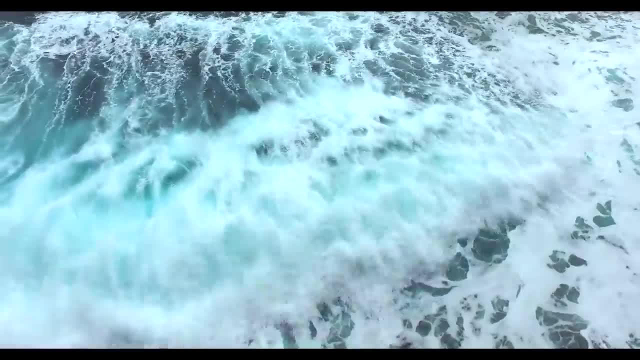 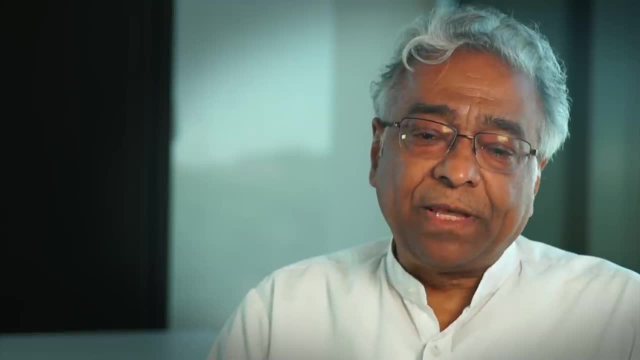 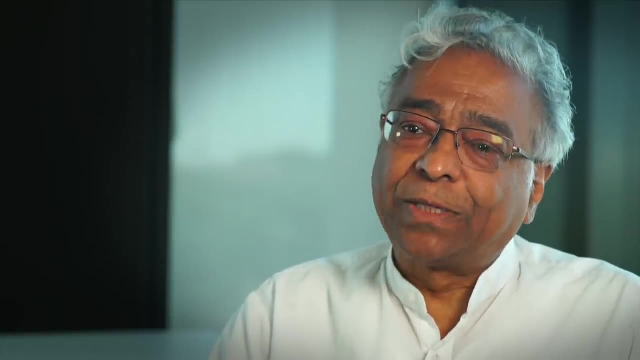 But if you come down, you see the waves and then you see the form over the waves And that's how the short-scale structural space-time should look like. I started thinking about working on gravity as a graduate student And in fact the very first paper I wrote was the review paper. 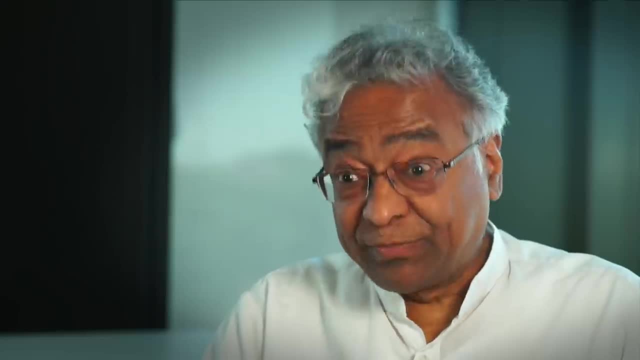 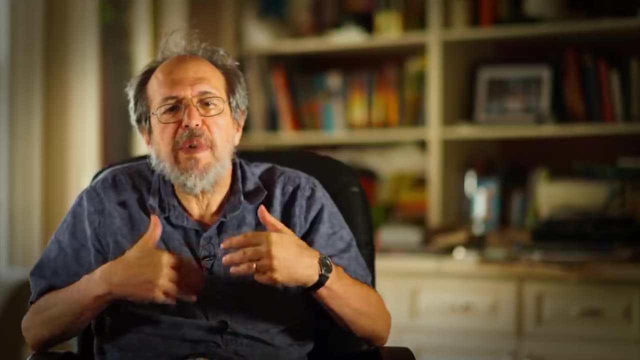 Because I wanted to learn all about it, And so it was a review paper I wrote with my advisor, Bob Girosh. I chose to go to Harvard, where there was no interest in quantum gravity but there was a great mastery of the Standard Model. 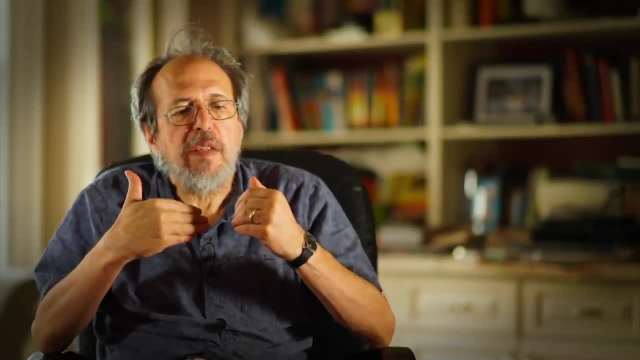 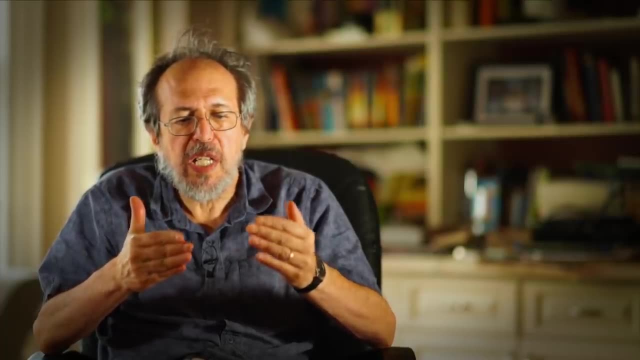 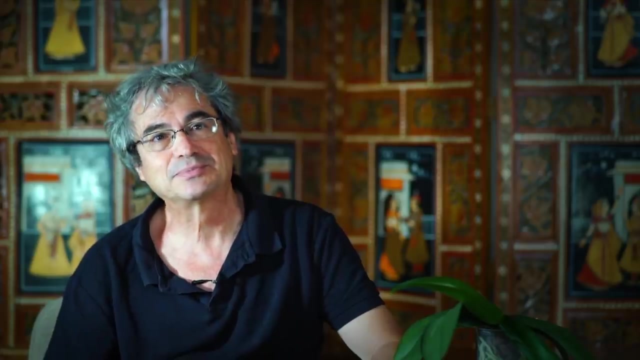 And I had this idea that maybe the mathematical and physical techniques that could guide understanding QCD and the Standard Model would be useful for quantum gravity. I decided that this was a worthwhile problem to get into. You know, when you're 20, you're all the courage of. 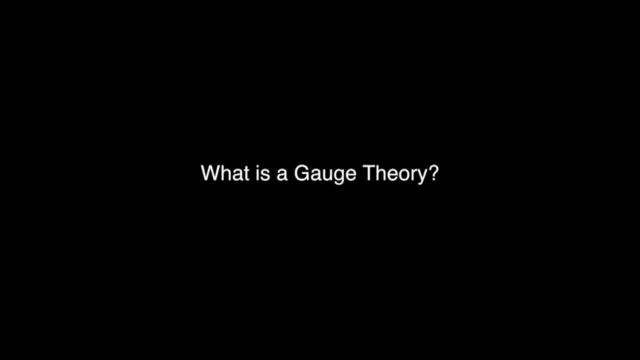 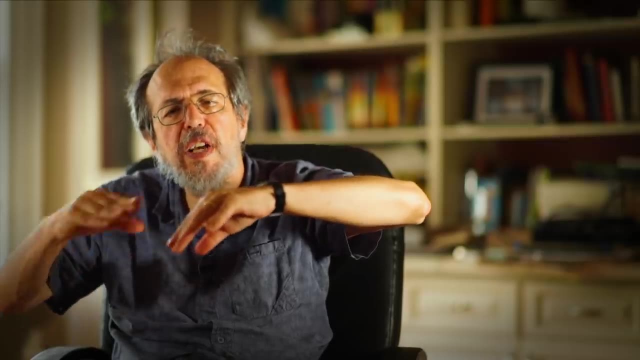 the world. So I said, okay, that's what I want to do. To gauge means to measure, And the gauge theory is a theory where the degrees of freedom, the things that vary, are fields that tell you how to bring systems to. 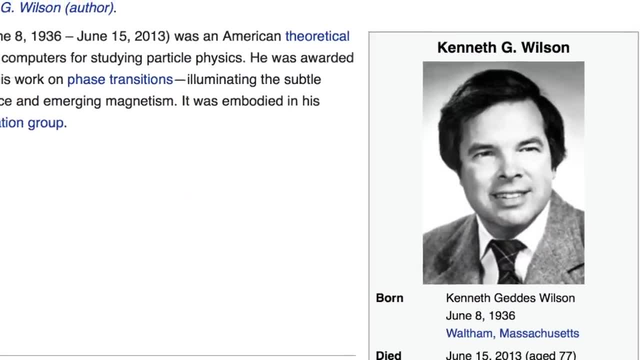 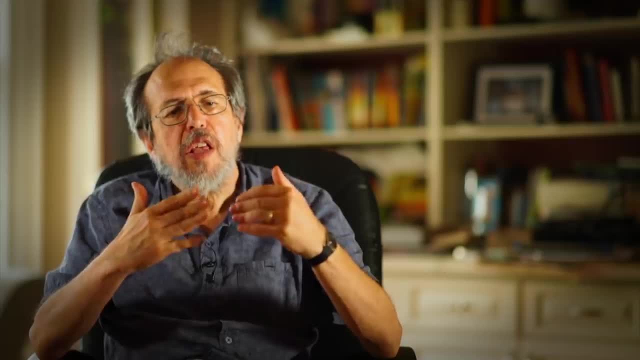 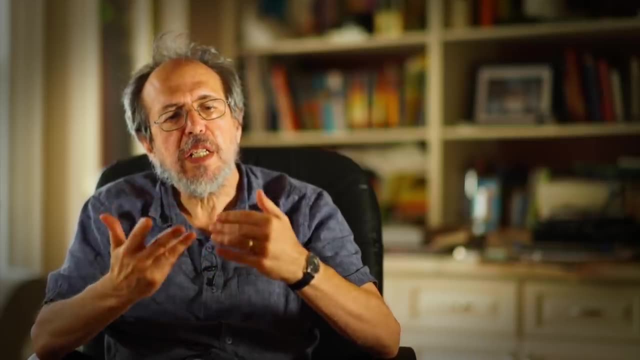 the observer in order to measure them. I heard a talk by Ken Wilson, and this was. he introduced a revolutionary technique to understand the quantization, or how these gauge fields describe quantum mechanically, And the important thing that he discovered is that they make lines or tubes of flux which can be 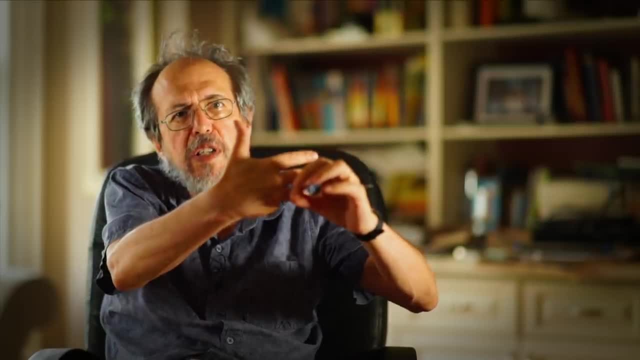 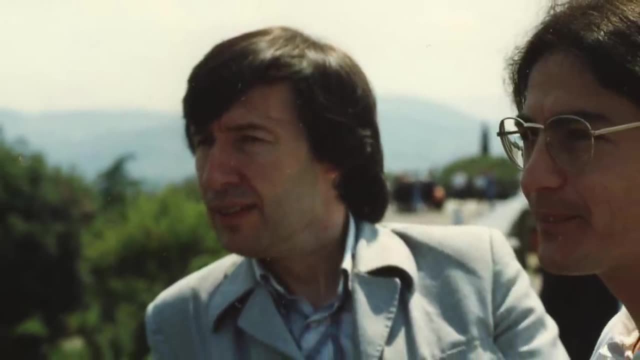 quantized into carrying discrete amounts of flux of the charge. The first person I went to see is going to be the first person I went to see is going to be the first person I went to see, Chris Isham, the person whose review papers had pushed me into into the field. 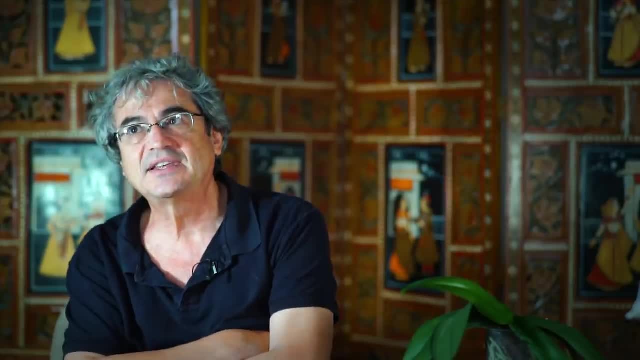 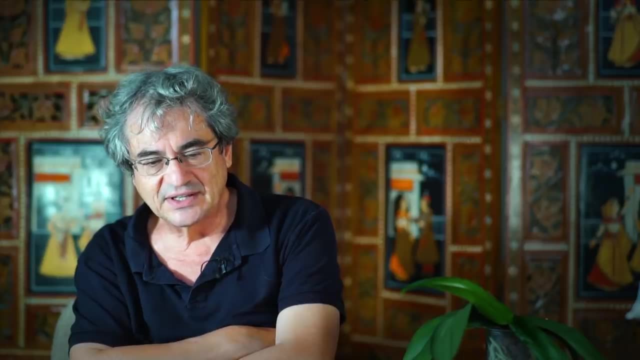 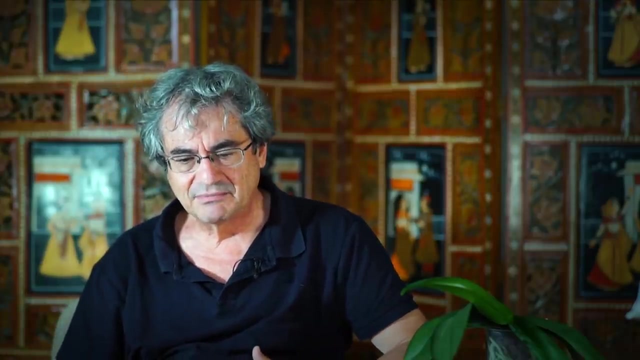 So I went to London. I remember distinctively Chris telling me that a few days before I left he told me that there was in America this young Indian, Abhay Ashtekar, who apparently had made the change of variables in general. 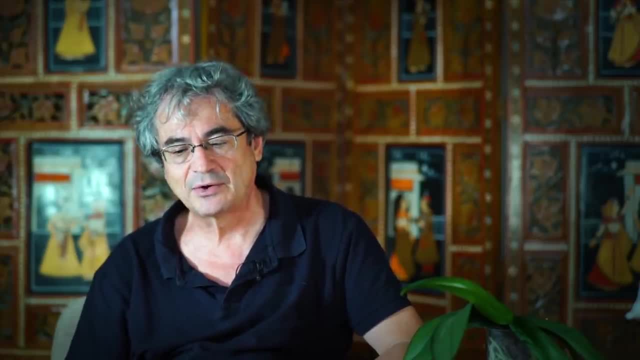 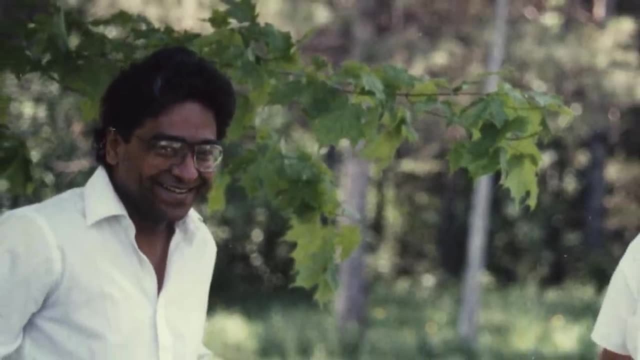 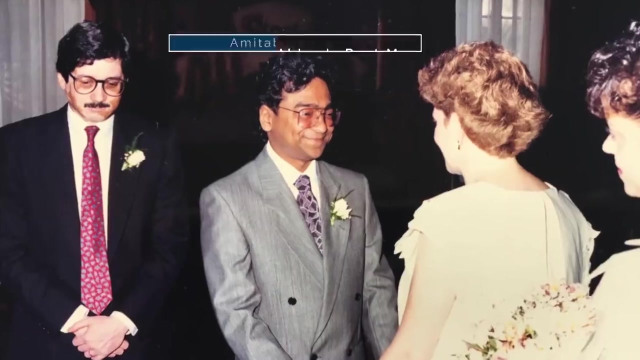 relativity, who might simplify the problem somehow. So I got interested, I wrote to Ashtekar and I went to see him in Syracuse and the work of Abhay was based on a previous work by Amitabh Asen, who had rewritten general 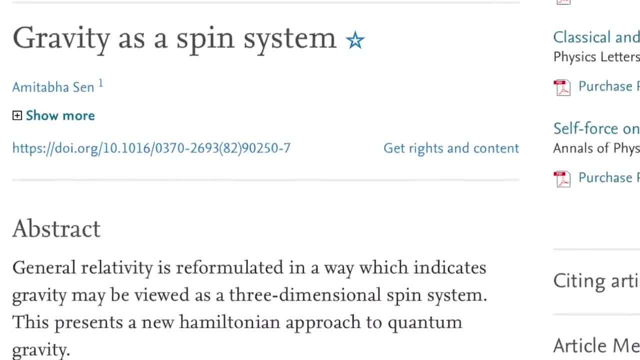 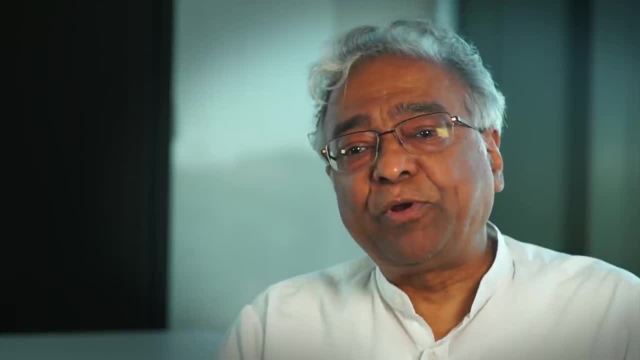 relativity, classical general relativity. so Einstein theory in terms of some variable, a connection instead of a metric. What are metrics? Well, they define distances between two points, or they define angles between two vectors. They define light cones at every point, so they give a meaning of causality. 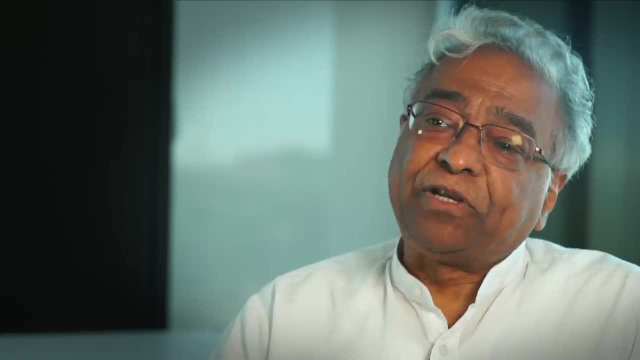 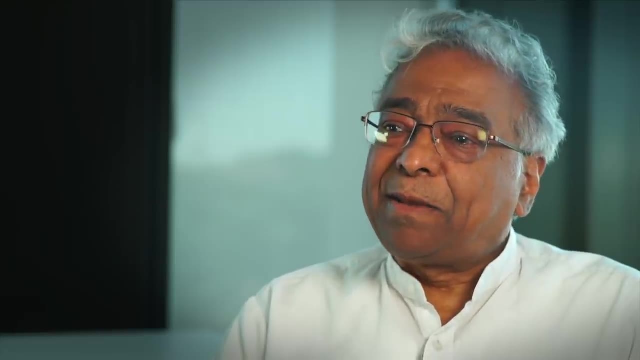 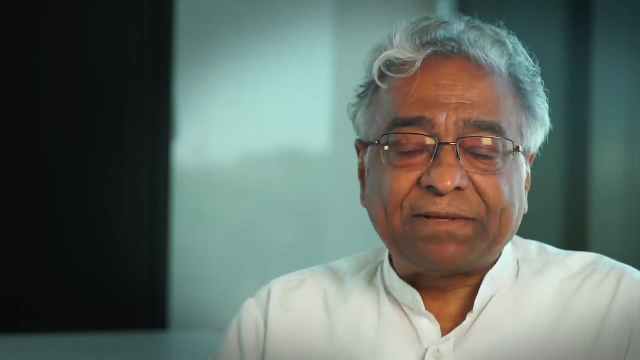 and therefore they metric, appear in every differential equation we write down in general relativity. So these were always regarded as a fundamental object. But it turns out that all other theories of all other basic forces of nature- the electromagnetic force, the weak force and the strong force- They are really based on connections rather than metrics. You know, in physics we are interested in the way things change and it is encoded in the concept of a derivative. But it's complicated to define a derivative in a curved space. So basically the connection is here to define properly a derivative. that is a way of comparing. 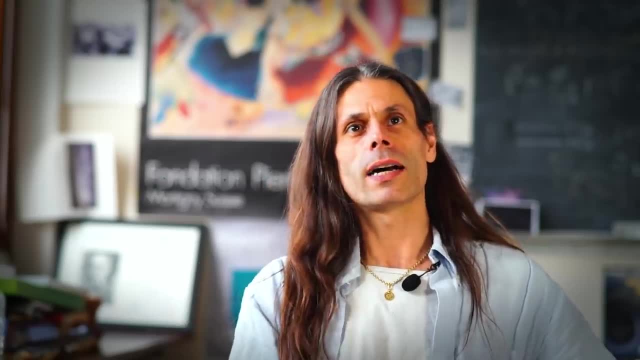 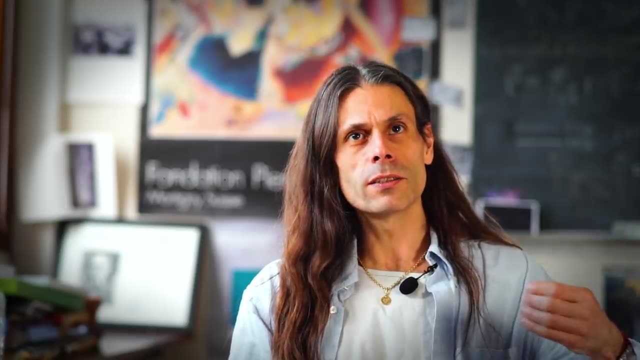 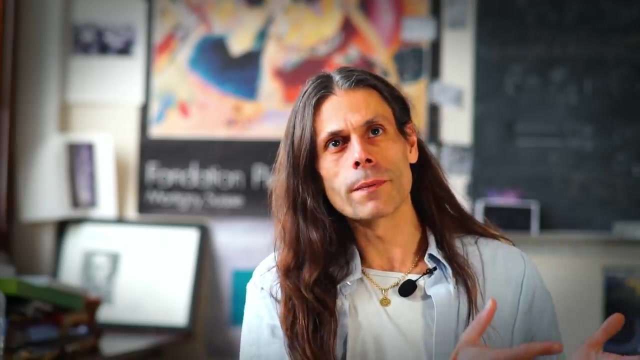 things in a curved space. The key point as far as technical details are concerned, is the fact that when we return in terms of connections, and specifically in terms of Ashtekar connections, general relativity looks like a gauge theory. Gauge theories are theories of particle physics. 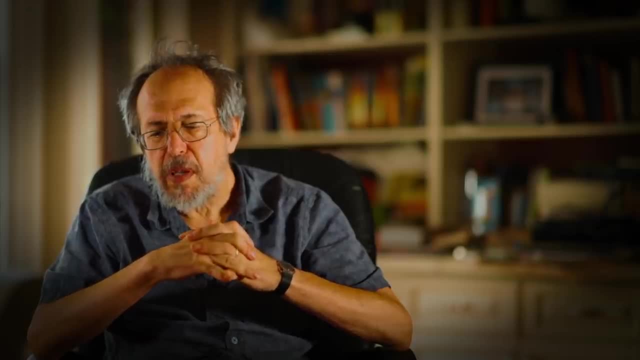 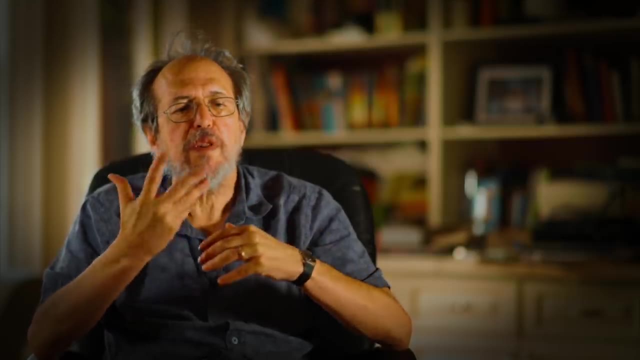 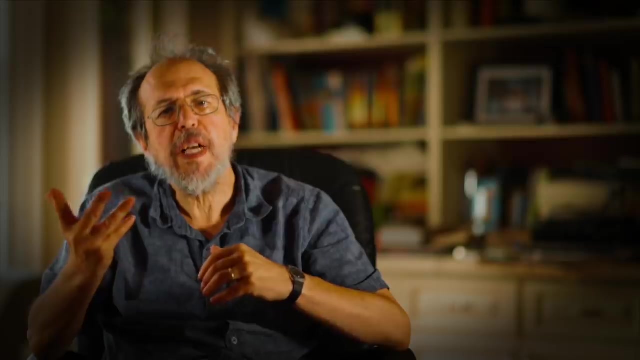 and we know how to quantize them. Abhay Ashtekar showed up and he had called me and said that he had managed to make a complete formulation of general relativity, extending Amitabh Sen's work, Because Amitabh Sen's work was wonderful but it was incomplete. The equations of general: 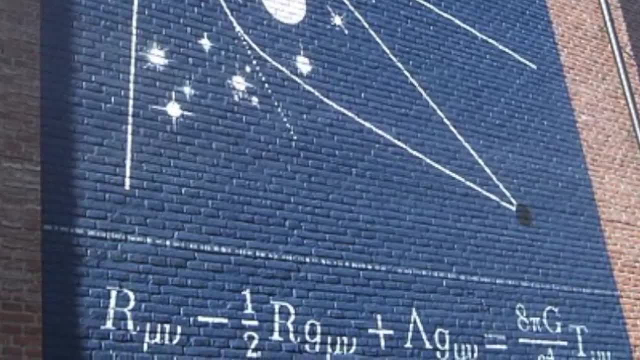 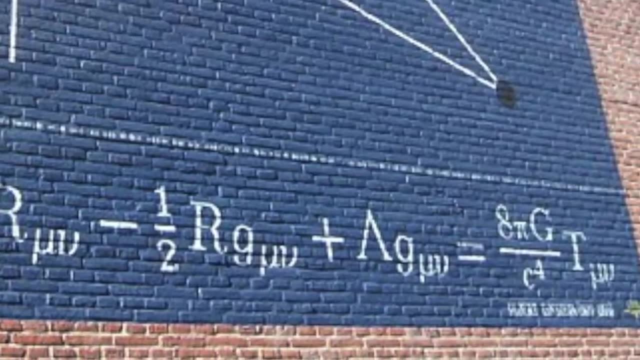 relativity are of infinite order. Any power of the fields is involved and it makes them very hard to study, even classically, but it makes them basically impossible to quantize. When Abhay was done, his form of general relativity had only quadratic equations, so it was a. 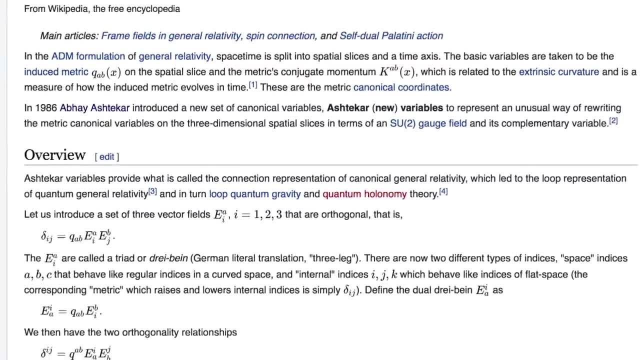 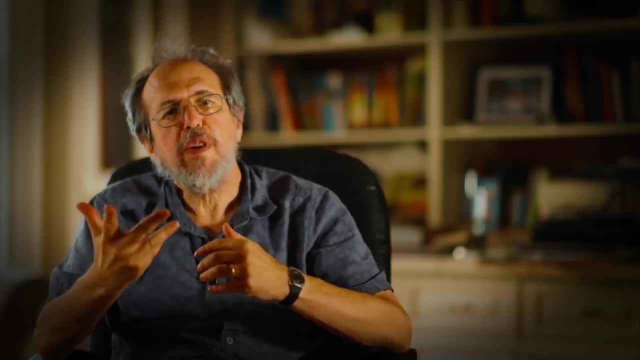 vast simplification And it was clear to me that that was the way to go. The way to go was to take the two Subtitles by the Amaraorg community toolkit of trying to reformulate a quantum theory in terms of loops of flux and apply 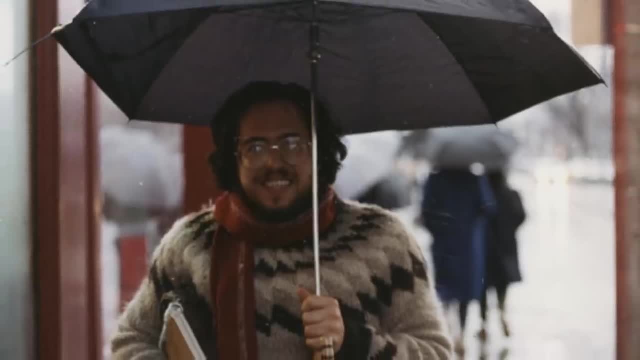 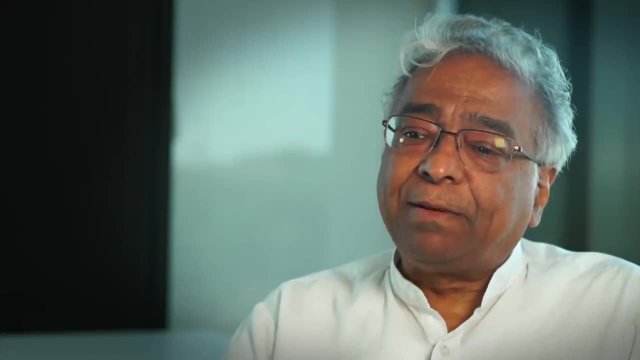 it to Abhay's formulation of general relativity. Lee had, you know, very solid background, coming from quantum field theory. He was a student of Sidney Colman, So. but Lee liked to make big jumps. Carlo was very interested in these. 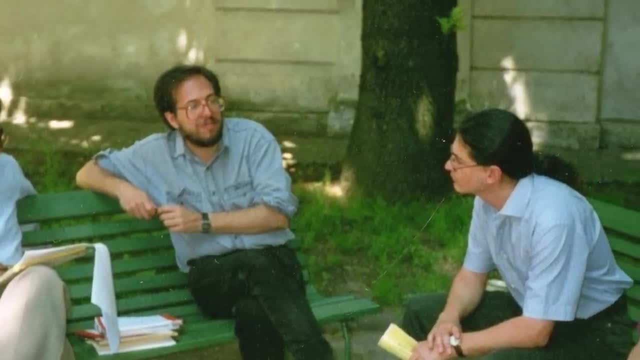 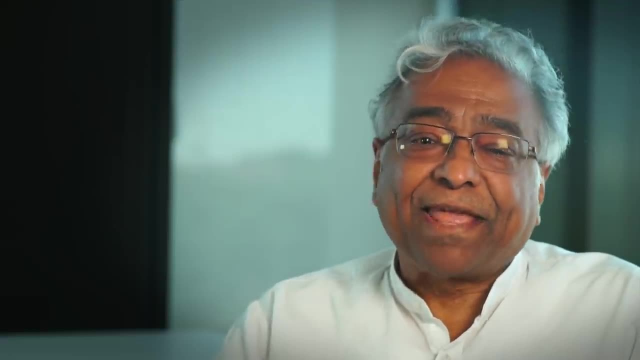 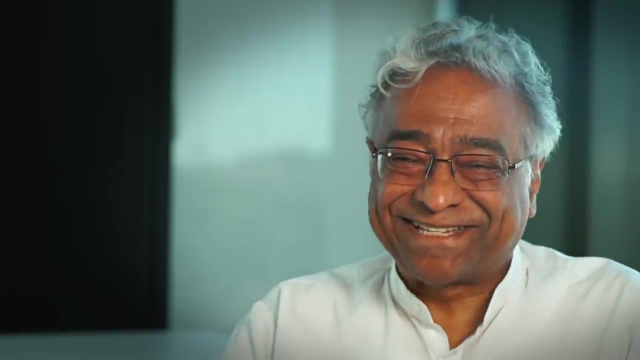 foundational questions. They had very different personalities. in some ways It was a very, extremely pleasant sort of clicking together. that occurred at the workshop And then it continued. It has continued all these years. Carlo and Abhay became very good friends And in fact for some time the three of us. 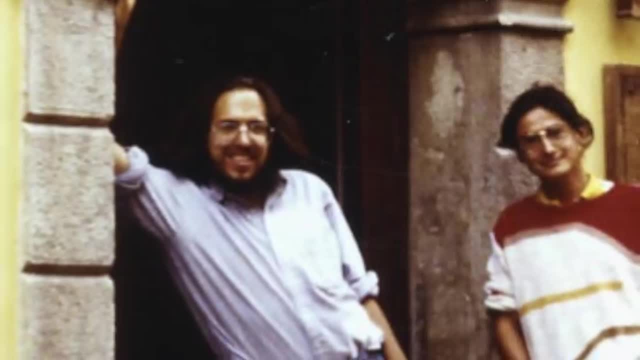 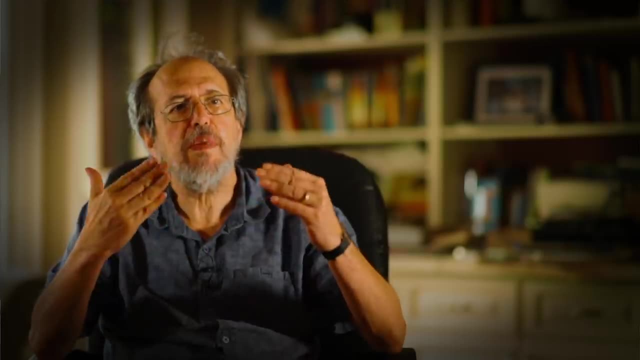 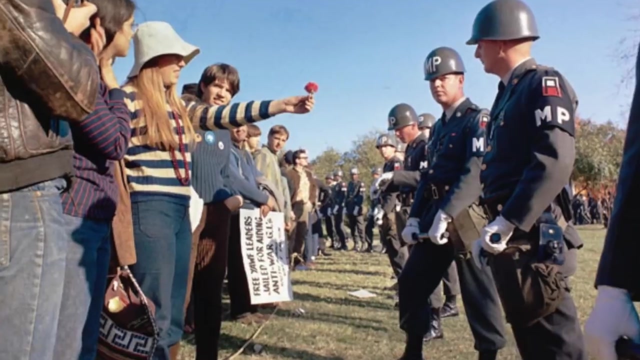 were quite close. I guess it's kind of emotional. Carlo and I have some similarities. We both came out of the left wing of politics. We were the generation below, the generation that made the great resistance to the Vietnam War and begun the feminist movement and ecological 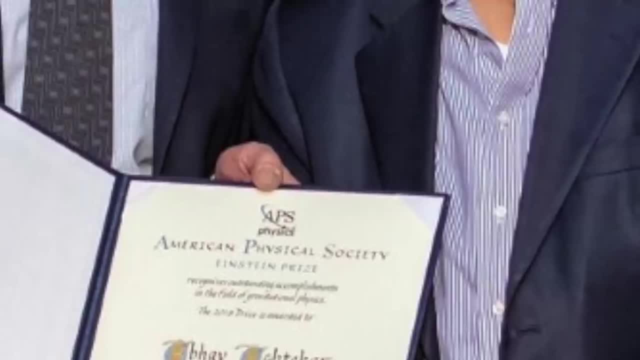 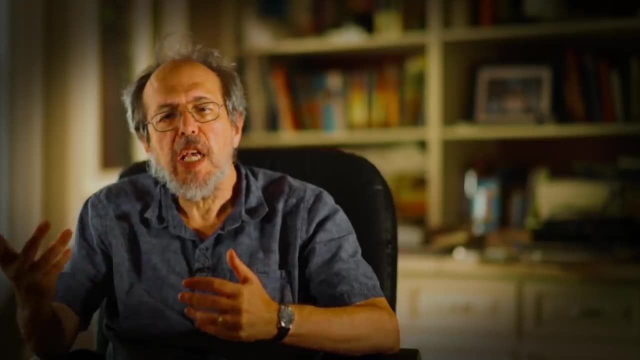 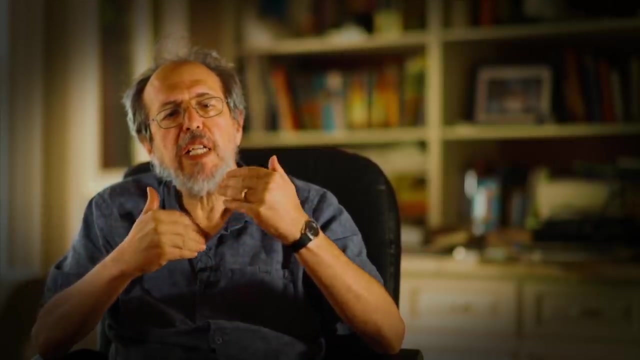 movements. Abhay is a mathematical relativist and a mathematical physicist, And he's, at the minimum, the best of his generation at that. There is nobody I know better to take an idea in this realm and make it a precise mathematical idea. I'm the opposite. I was 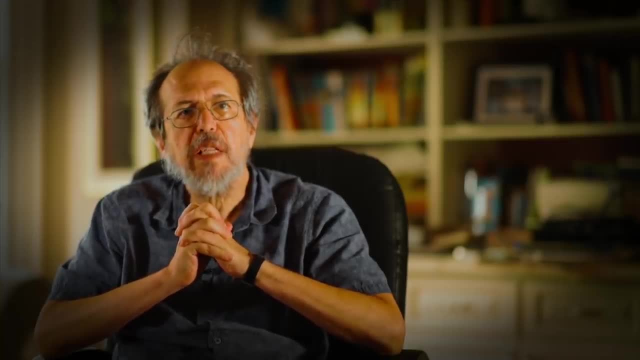 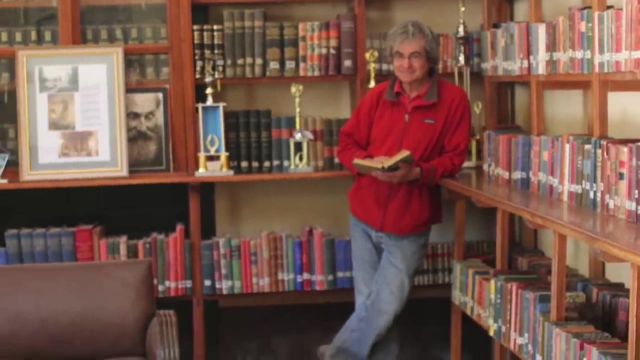 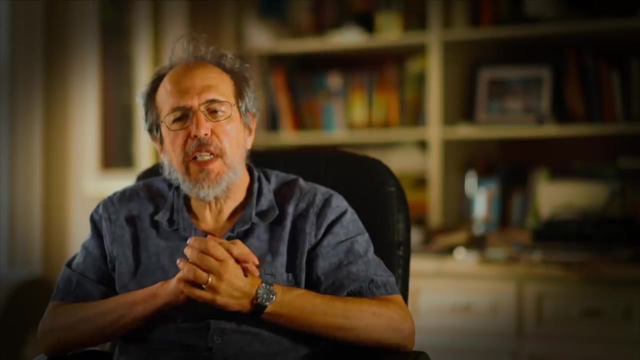 trained as an American elementary particle theorist by particle physicists who emphasize intuition. Carlo has some of both of our strengths. He's at least as good as me as a physicist. He's a fabulous physicist And he also has an easier time than I do speaking. 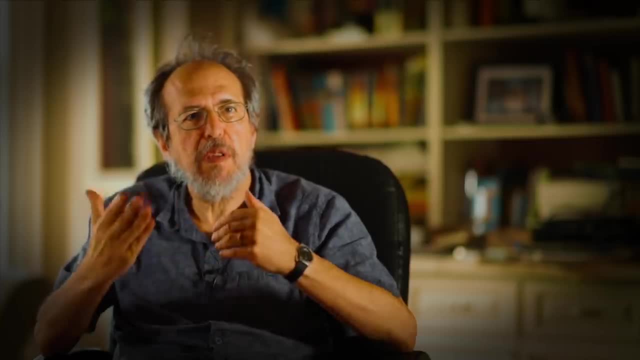 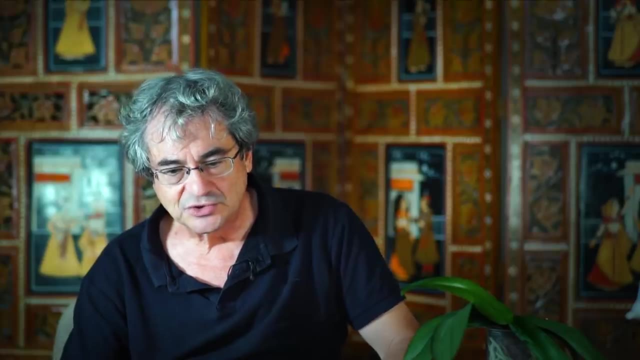 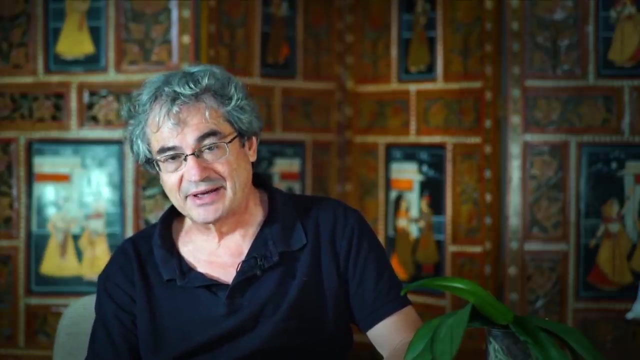 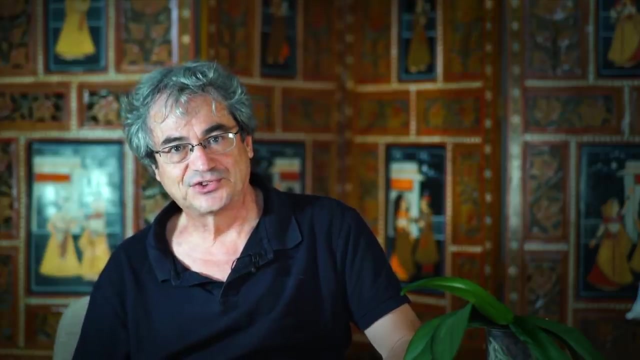 the rigorous language of mathematical physics and, working with Abhay Lee Smalling and Ted Jacobson, made a step which turned out to be crucial. They found some solutions of the will-or-the-wit equation rewritten by Abhay Ashtekar with the new variables, And these solutions were very mysterious because there was one solution. 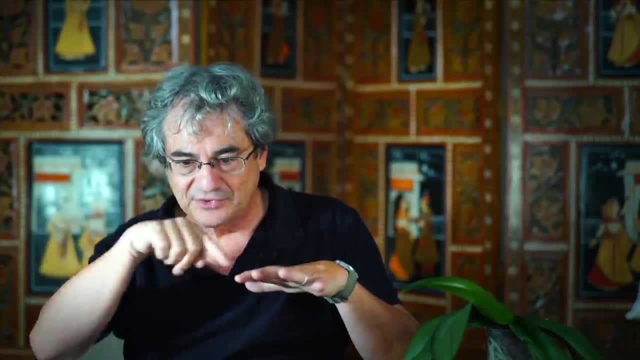 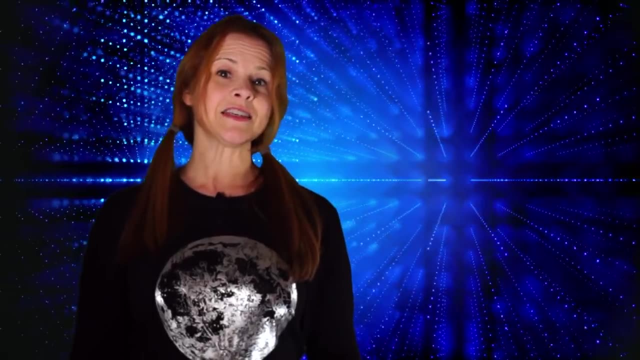 for every loop in space. So you start with space, you draw a loop and then there's a mathematical technique from this loop to have a solution of the will-or-the-wit equation. At that stage the ideas being proposed in Loop Quantum Gravity still used a back-and-forth. 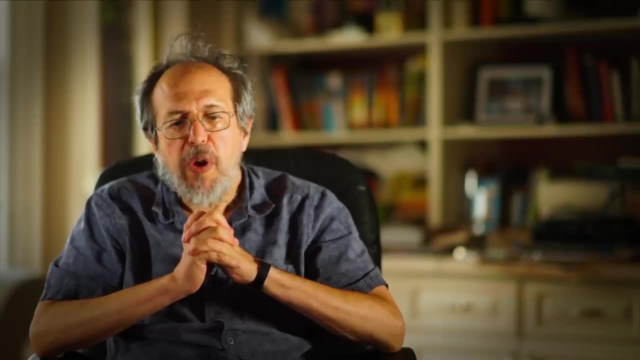 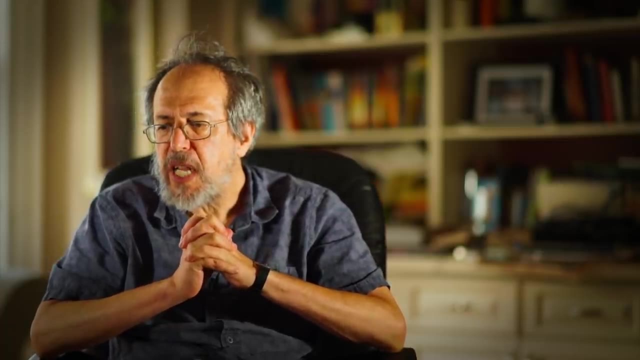 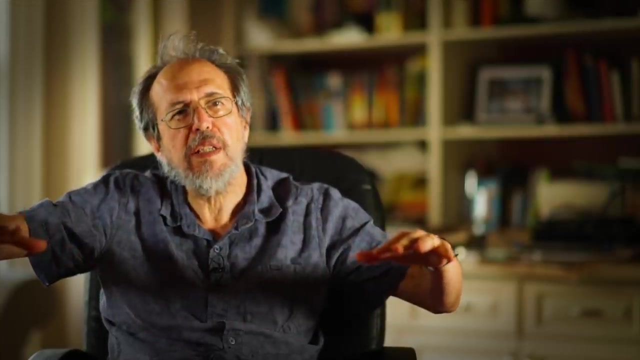 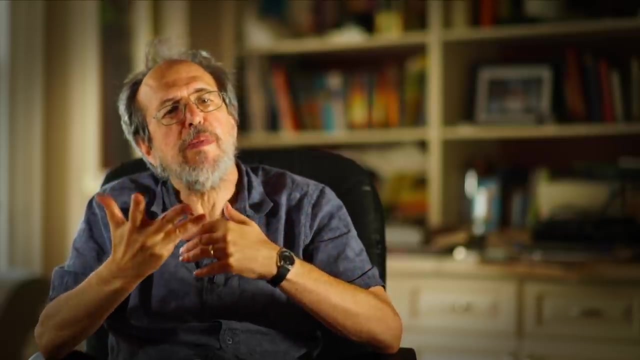 approach. One day I was talking with Ted and we wondered what would happen if we just took the lattice away and had these quantized flux lines of Abhay's variables just moving around in space without being stuck on the lattice. And so we wrote that down and we tried to apply the 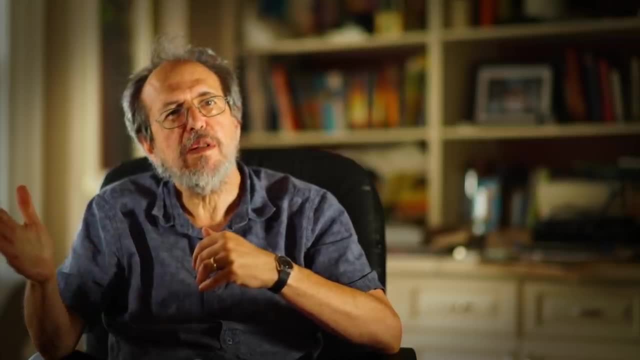 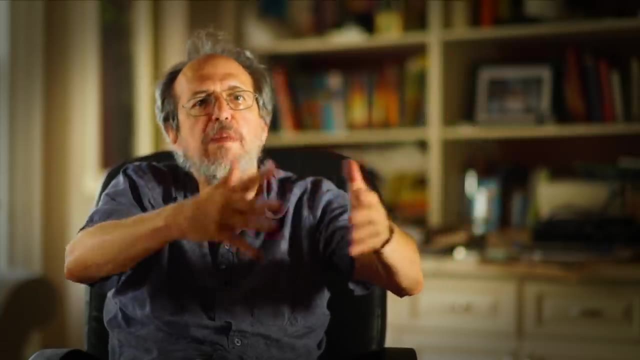 will-or-the-wit equation, because since there's no time outside the universe, the wheel of the wheel equation says you take a quantum state of the gravitational field, you act on it with a certain operation and you're supposed to get zero. And we plugged-in these. 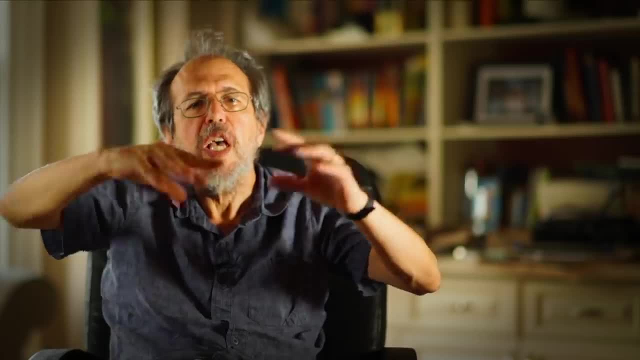 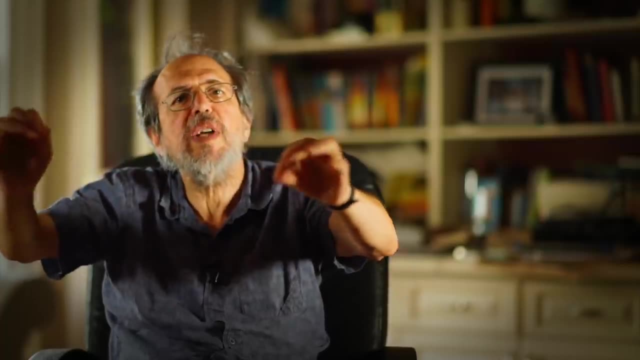 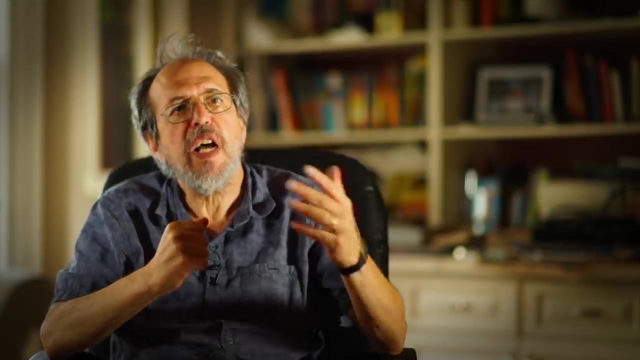 lines of a quantized electric flux and discovered that as long as the lines didn't intersect each other, as long as they were closed loops or knotted or braided, we got a solution to the wheel-of-the-wit equation just like that. and we got an exact solution, not an approximate. 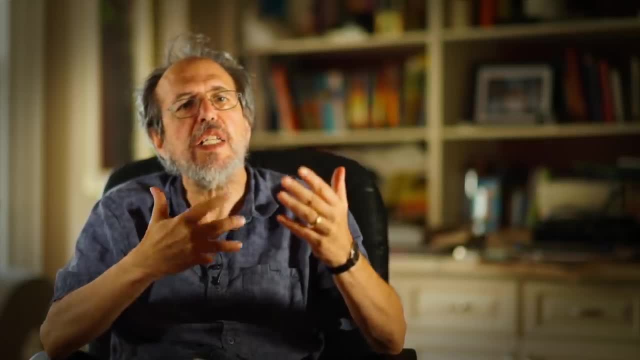 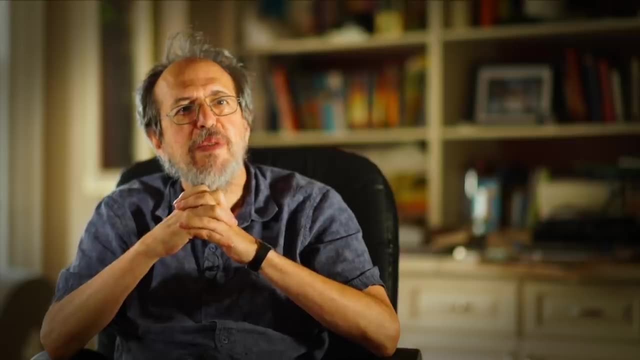 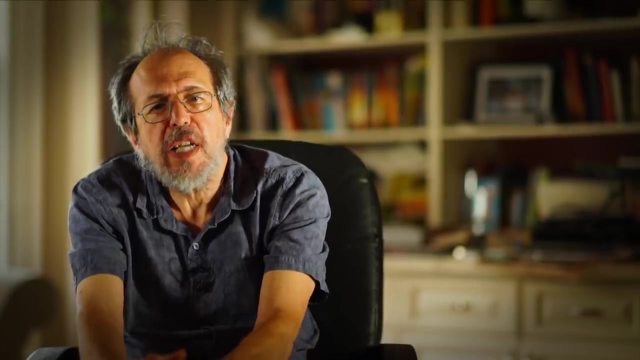 solution dreamed was possible, but we had. it was literally took 10 minutes. so all of a sudden we had quantum geometry in front of us. that was that was a wonderful moment. so we had solved the wheel of the wheel equation. but there were three other equations that you had to solve to make a quantum theory of gravity. they 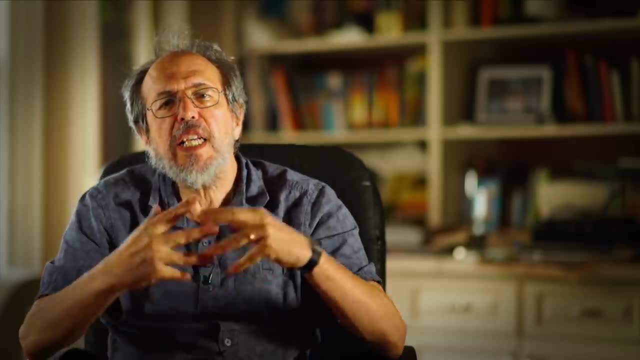 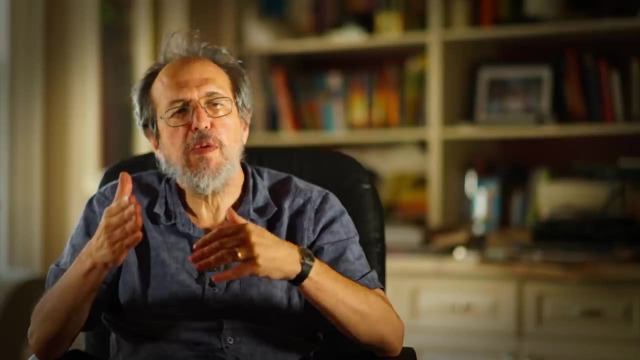 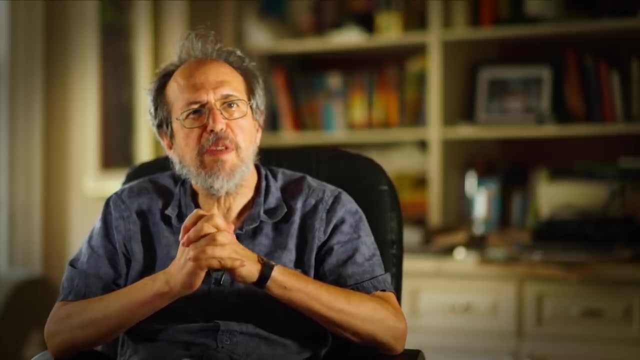 are called the diffeomorphism equations and they express the idea that there's no preferred observer. there's no preferred coordinate system in space. we couldn't solve the diffeomorphism equations with the same variables that we used to solve the wheel of the wheel equation. when Carlo showed up, I was 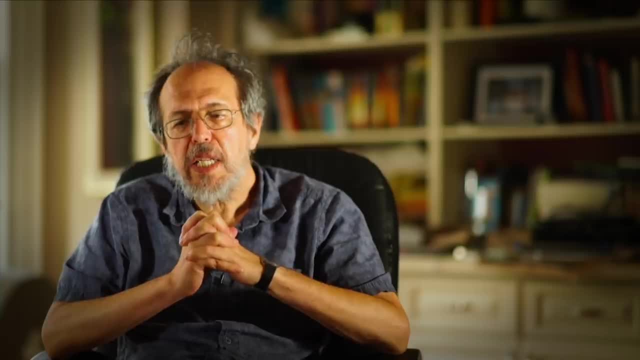 convinced that the problem was impossible and we were stuck. then I looked at Carlo and I said: for some reason, do you like to sail? and he said he did and I was just learning to sail. so he went back and said: I want to learn to sail. and he said I want to learn to sail. and he said he did and I was just learning to sail. so he went. 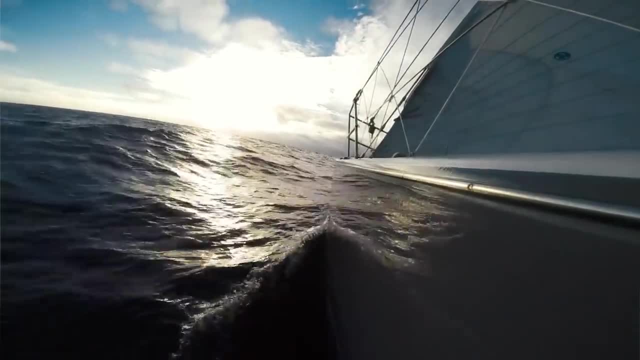 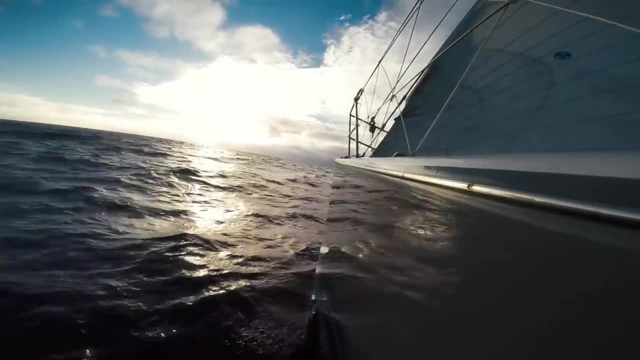 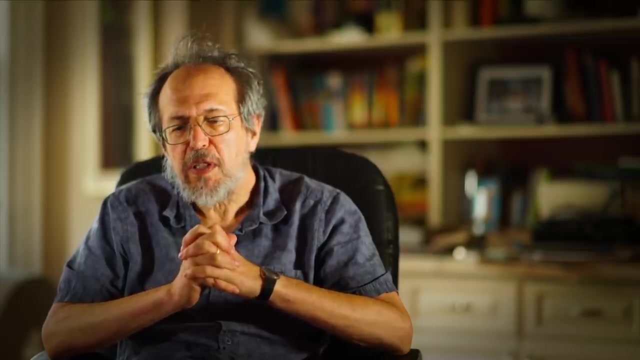 and sailed and talked about his girlfriend troubles and my girlfriend troubles and we started to become friends. we really bonded. then he disappeared for three days and on the next day he came, came into my office, took off these new jackets- because he was always freezing in America- and said: 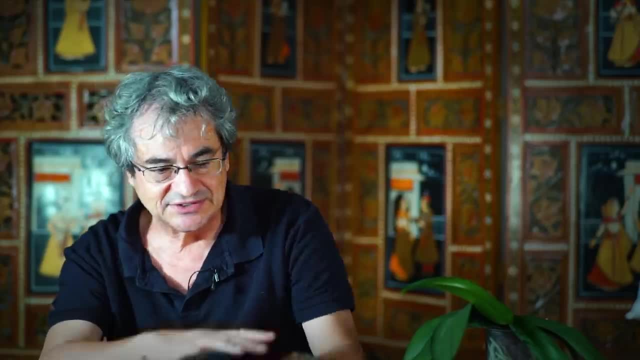 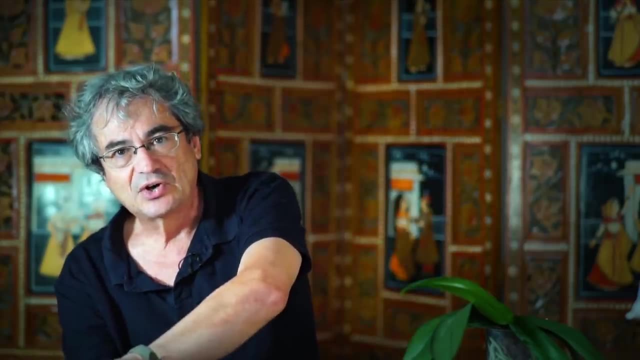 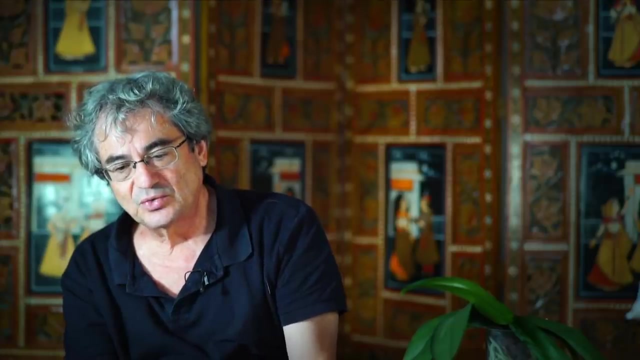 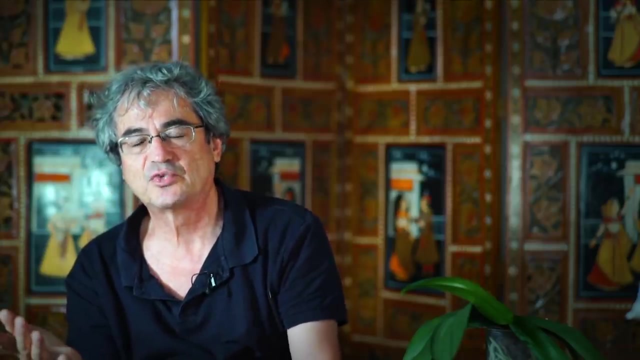 I've solved all the problems. instead of starting from a space and a connection, write the quantum theory directly in terms of linear combination of these solutions of loops and we immediately realized that by doing that we could solve the full set of formal equations of quantum gravity. we were not. 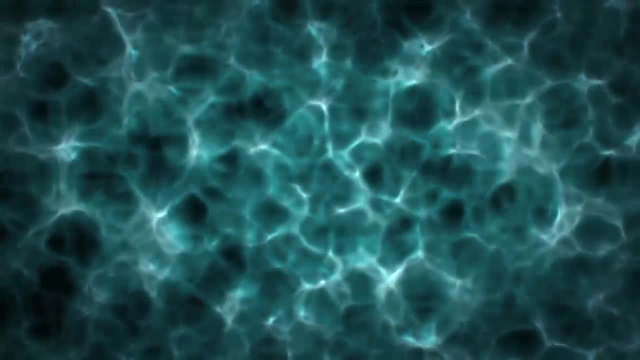 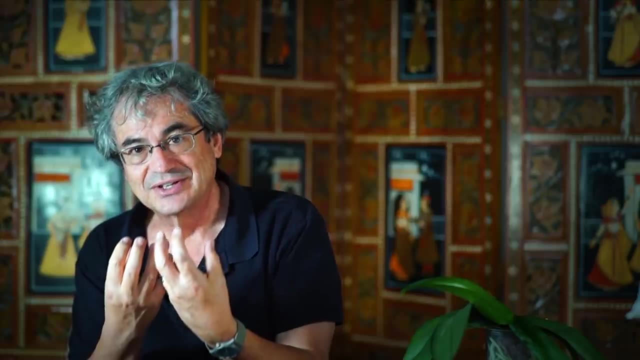 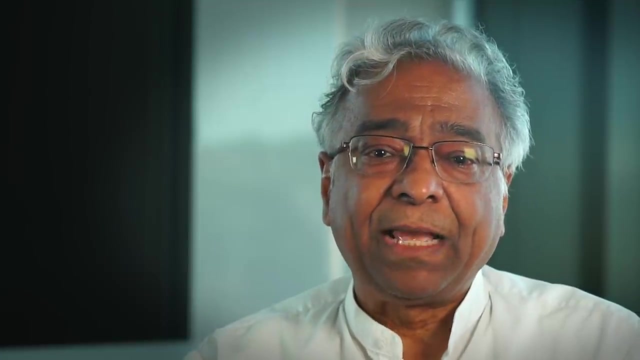 describing excitations that move in space, these loops, those were the excitations of space itself. we were describing space-time as a collection of threads. if you look at a two dimensional surface like this, like the shirt, for example, right now, then from a distance it looks like a nice. 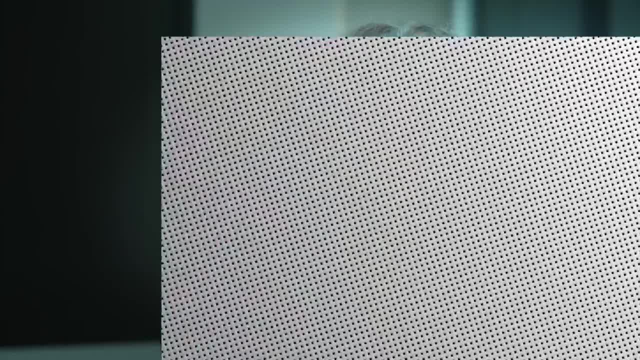 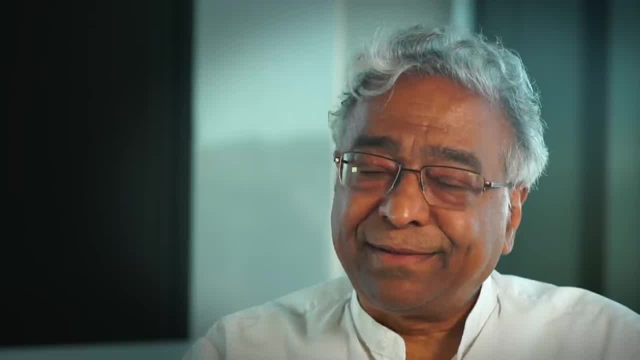 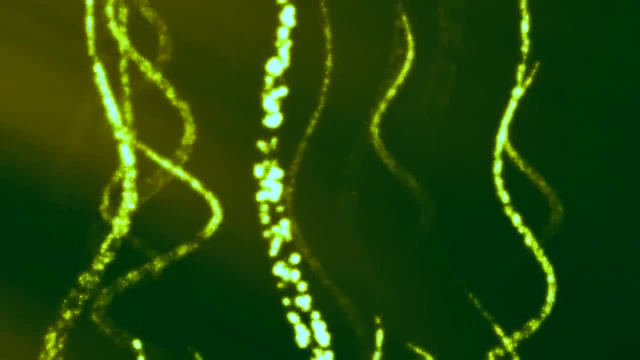 smooth continuum. but if you look under a magnifying glass you will quickly see that is really over by one dimensional tracks. so, similarly, the idea is that the raw geometry in this room is really woven by one dimensional quantum threads and one of these quantum threads, that these quantum threads are fundamental excitations of the gravitational field. 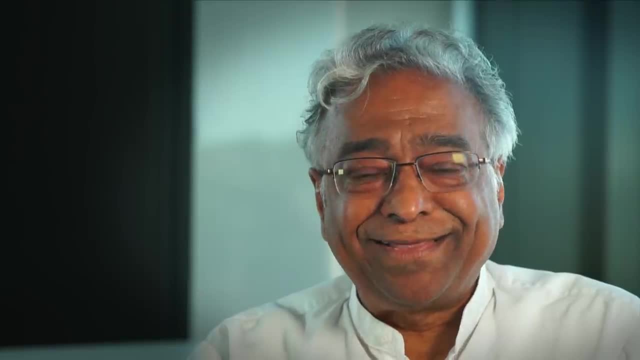 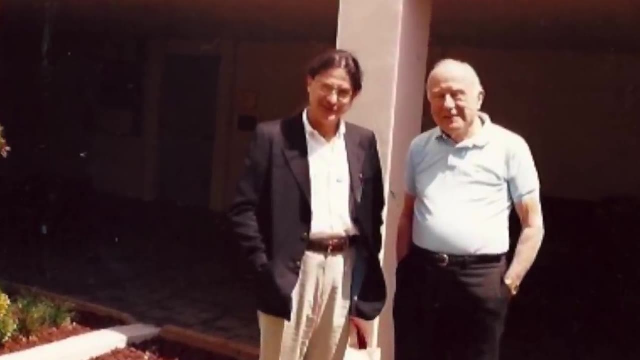 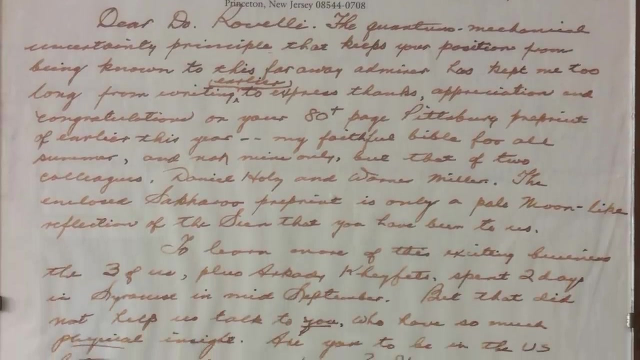 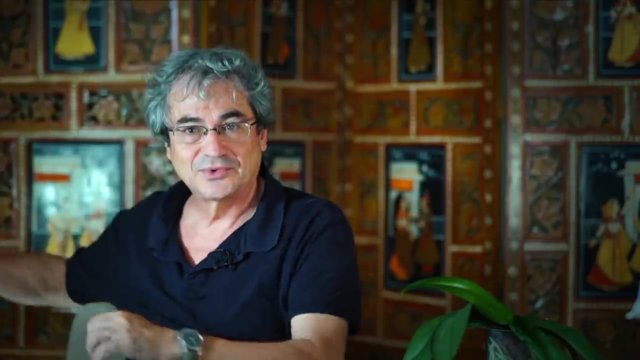 so they are not loops of object, but they are. they are the. they are the loops from which geometry emerges. John Wheeler got very excited with loop quantum gravity. he wrote to me in his very emphatic style he always used with a lot of wow. I still have his little letter on my office and on a wall because of. 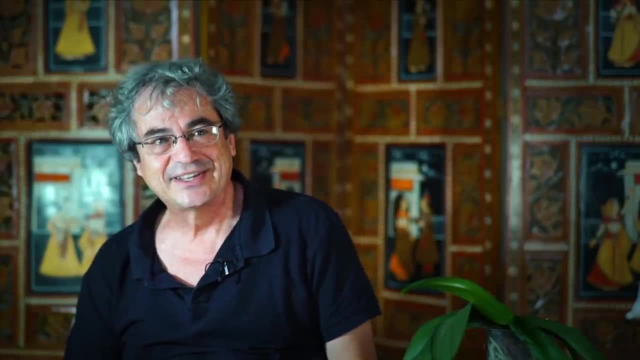 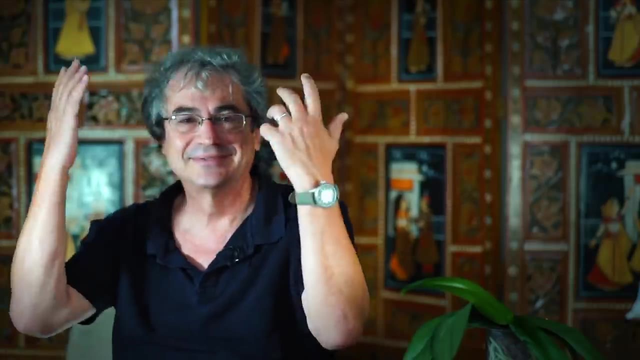 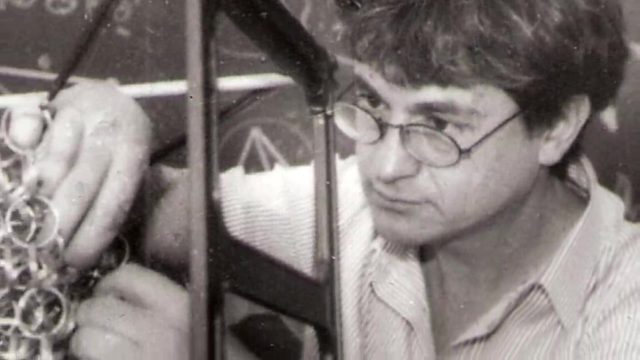 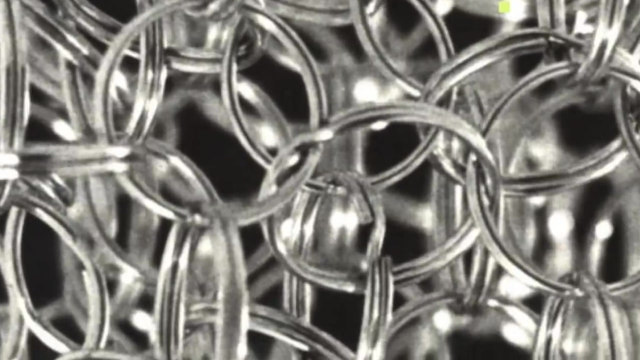 you know, for me he was the great hero, the great intellectual hero. so receiving a letter for him, excited about my work for the young kid, I was with more than I could ever dream. I came to Princeton with a piece of a little thing which I made. there was a lot of key rings attached to one another, which was 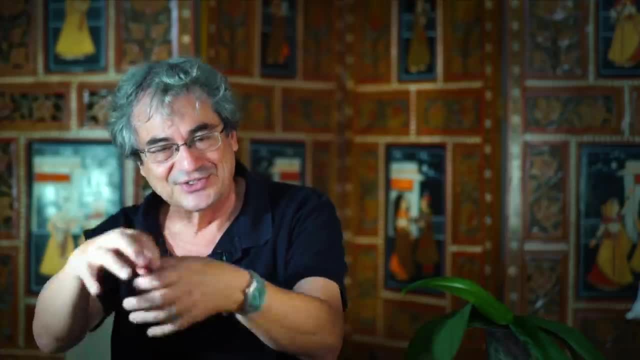 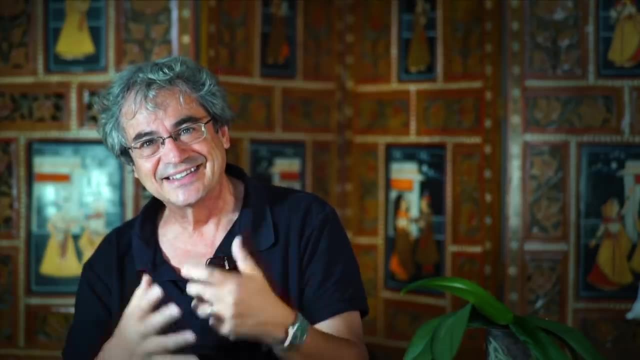 supposed to give the idea of the three-dimensional structure of space time. and when John saw it he jumped and said, yes, that's what I was always been thinking. and he came with his book. in a picture of his book, look, he says it is a. 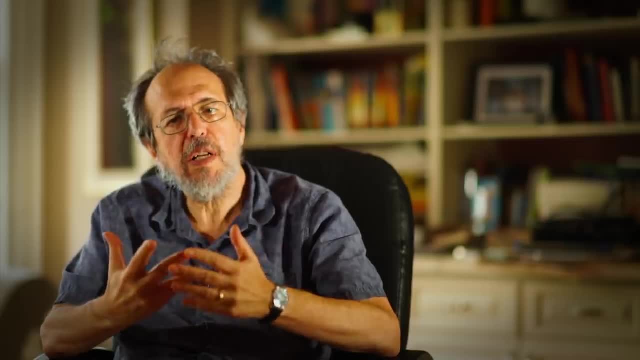 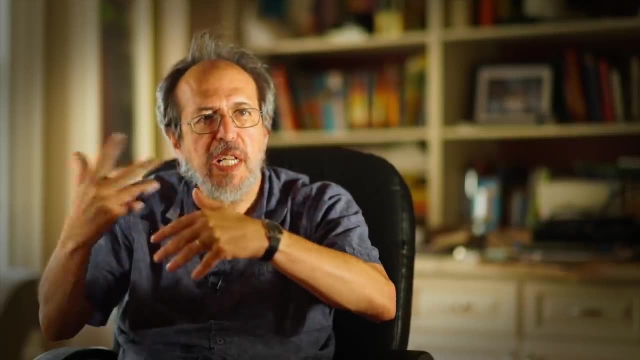 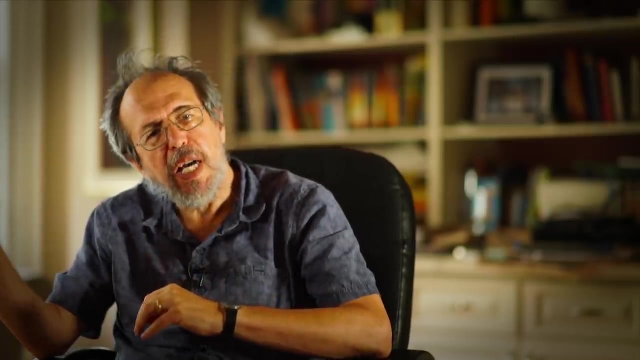 quantization of general relativity. so, unlike string theory, it's not a different theory than general relativity, which might have something to do with gravity of general to be, it is general relativity as given to us by Einstein, as modified by Abai and Ashtikhar, and then 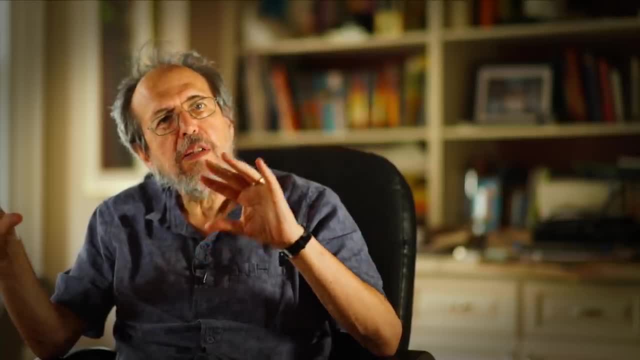 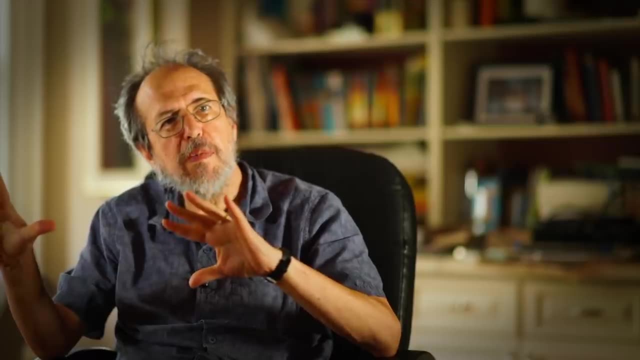 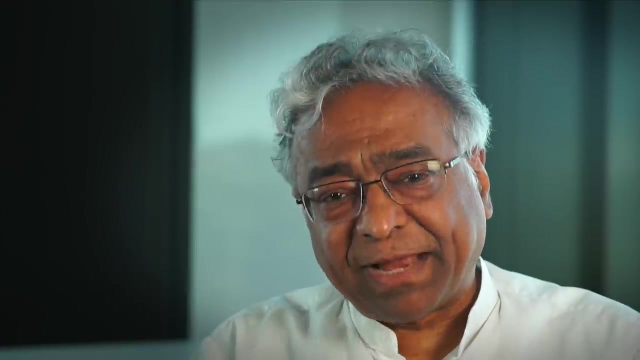 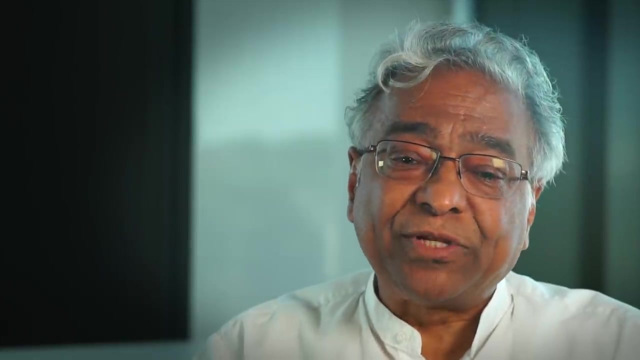 And then quantum mechanics, using ideas that were brought in to study gauge theories by Polykov and Wilson and other people. But it is just the quantization of general relativity. We realized that loops had some technically were inconvenient and therefore the loop representation is really not so convenient to use. 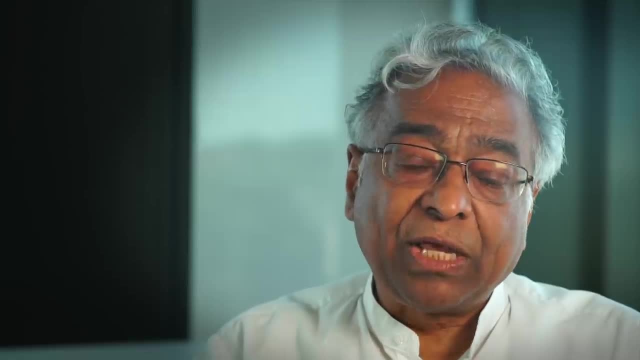 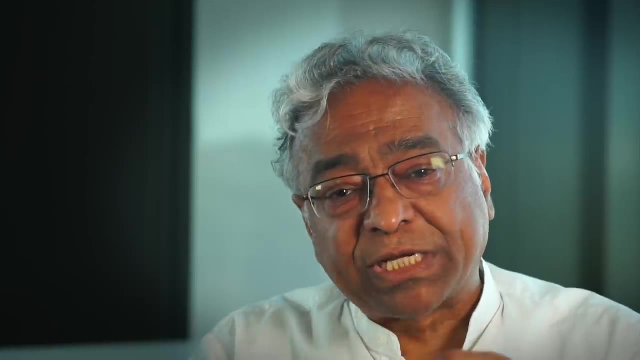 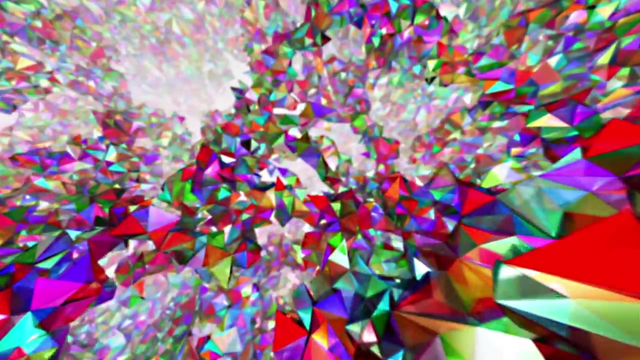 and to get the interesting properties from it, and so on. So we introduced instead of loops what is called as graphs. So loops are, so to say, closed curves, whereas graphs are objects in three dimensional space, for example, in which has nodes and their links, And they can have many, many configurations. 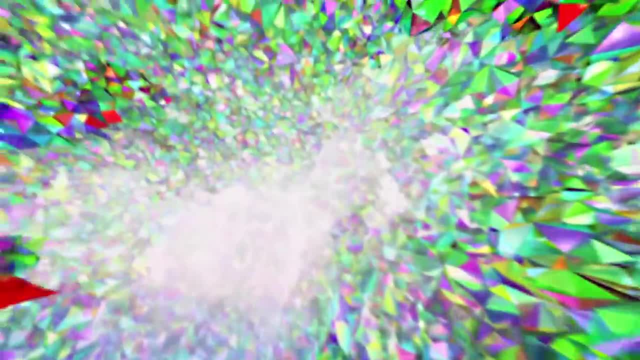 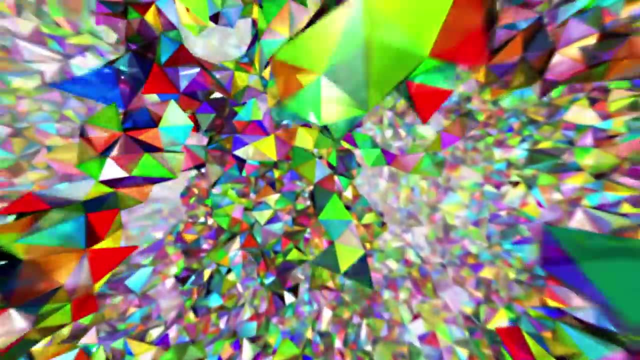 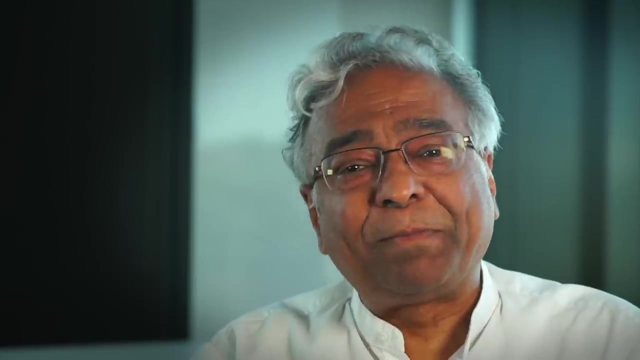 And it turned out that the same ideas that were underlying the loop representation can be carried over, with the same integration theory and so on, to graphs, And then several of the technical problems Disappear in this particular way, And so in a certain sense, it is really true that the loop representation is a misnomer for what is being done in loop quantum gravity. Or loop. quantum gravity is a misnomer, But it is very similar to what is string theory. I mean, string theory is a misnomer because originally there were just strings, But then people realized that there are also other external objects: membranes and so on. 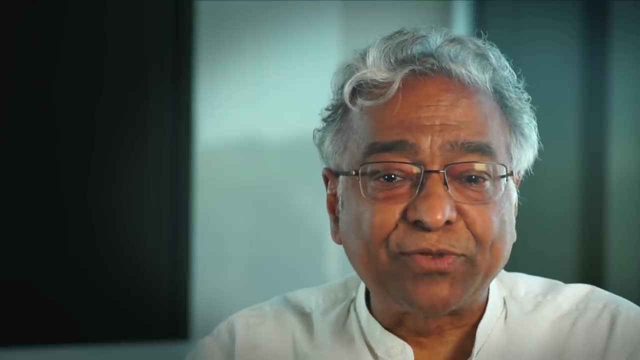 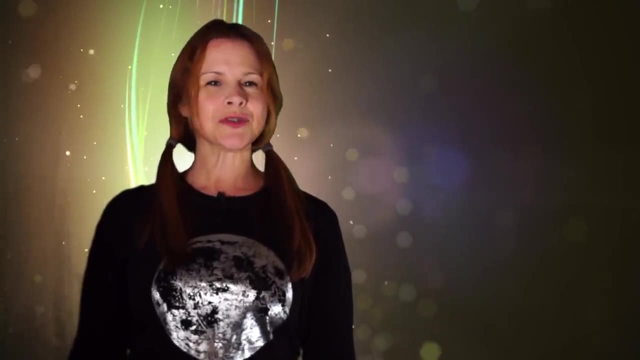 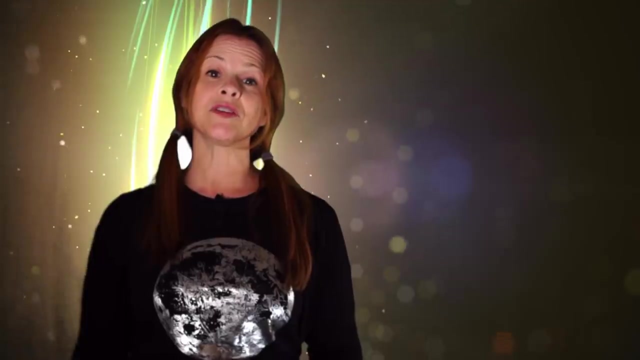 And strings are no more fundamental than other objects. They are all on the same footing, so to say. But since it was called string theory, it is still called string theory, As loop quantum gravity was being developed. a student of Smolin's, Berne Bruegelman, was given the task of applying loop quantum gravity to the theory of the strong nuclear force. 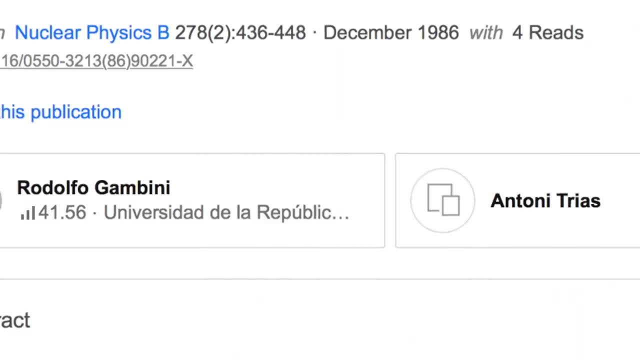 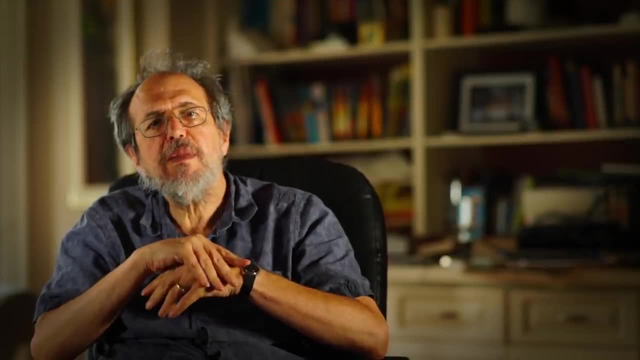 Quantum chromodynamics. But in doing so he discovered the work of Anthony Trias and Rudolfo Gambini. And then one day he came to my office with a look of horror on his face and he said: this has been done before. I was shocked. 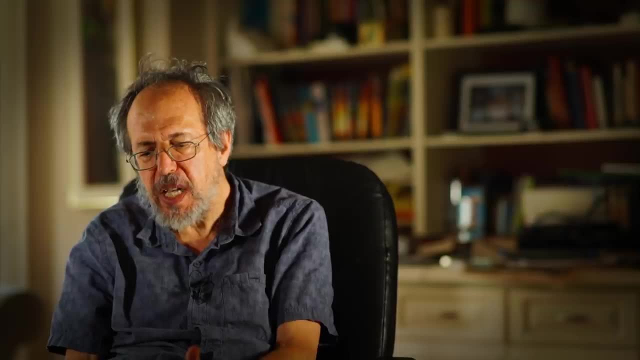 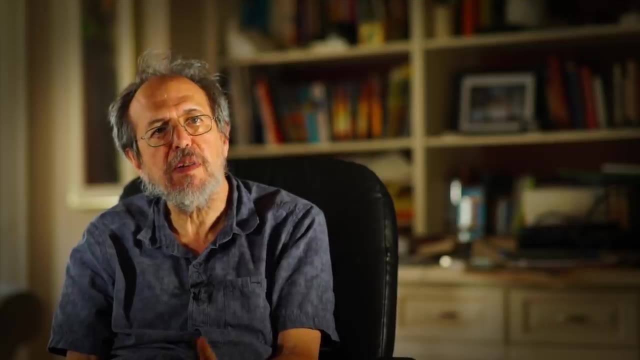 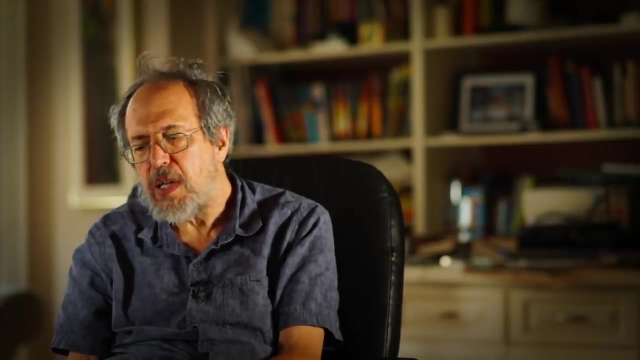 I was embarrassed, I was pissed off at myself and faith and everything. So it wasn't only our discovery, And it was just a few years before Carlo and I had invented this technique. I wrote them a letter. They had an address in Barcelona. 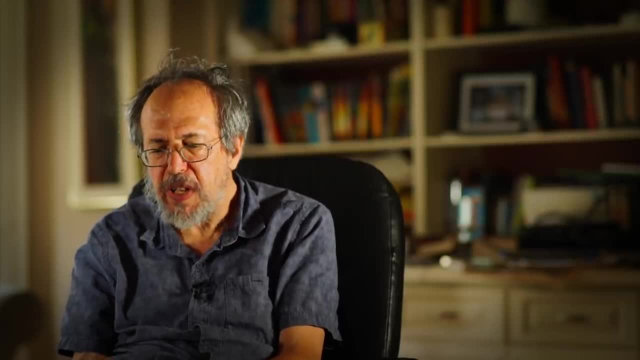 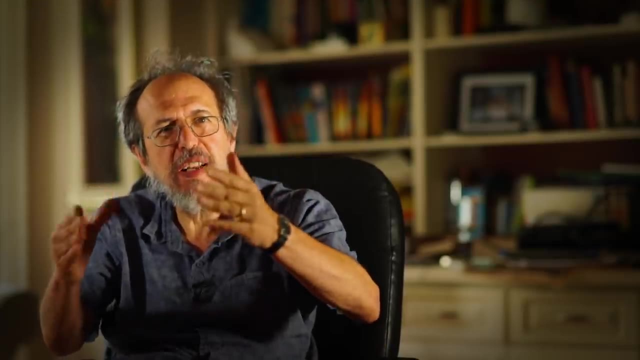 And said that I was very sorry that we had developed this technique in quantum gravity and the astrograph variables And we just had not known of their work. I actually wrote a physical letter And Rudolfo says: what are you doing tomorrow? So he said we'll be there. 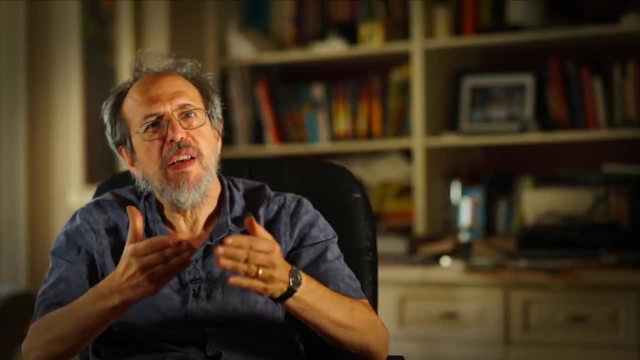 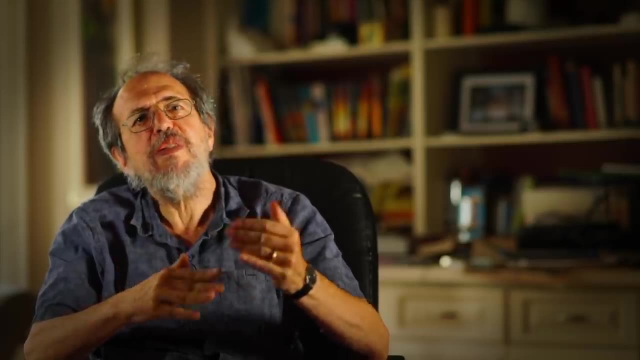 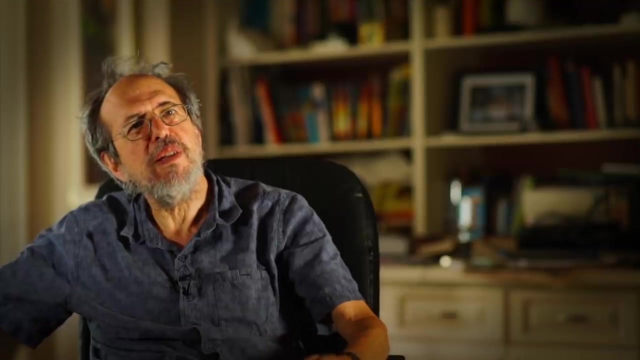 And he hung up And they went downstairs, got in his car- It was a little sports car with the two of them- And they drove from then, that was the afternoon, overnight, from Barcelona across France, across the Alps, to Trento in north of Italy. 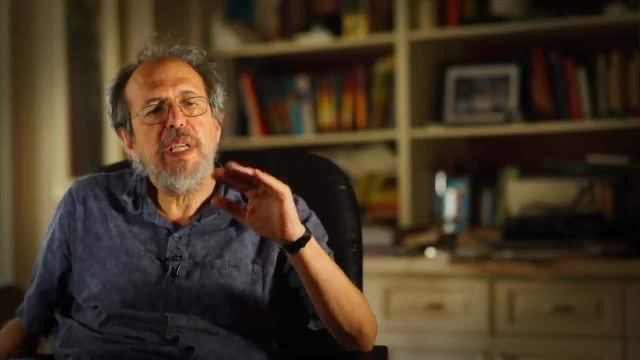 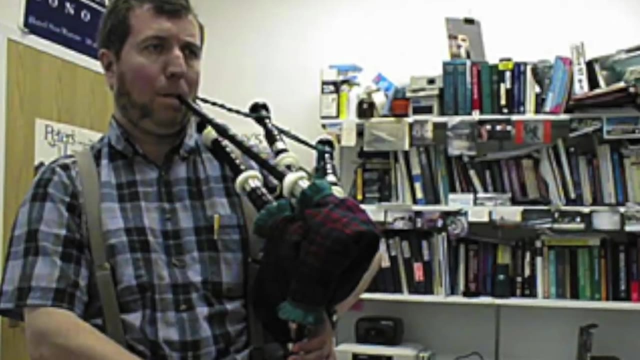 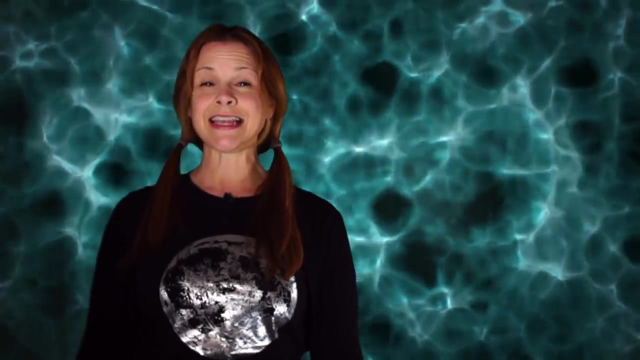 And they arrived the next morning. Gambini, very quickly after that, began to work with a young Argentinian physicist, Jorge Poulin, And the byline of Gambini and Poulin have been. they've done many things together. During the 1990s a key breakthrough in loop quantum gravity was made. 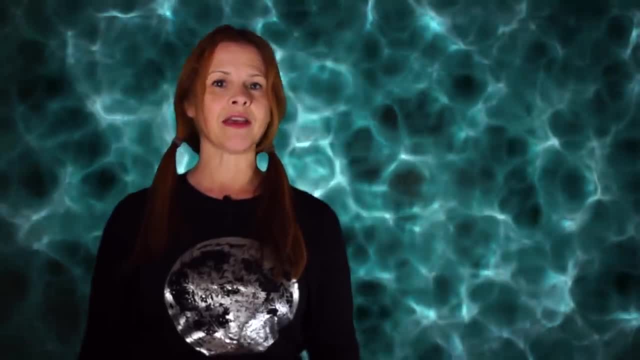 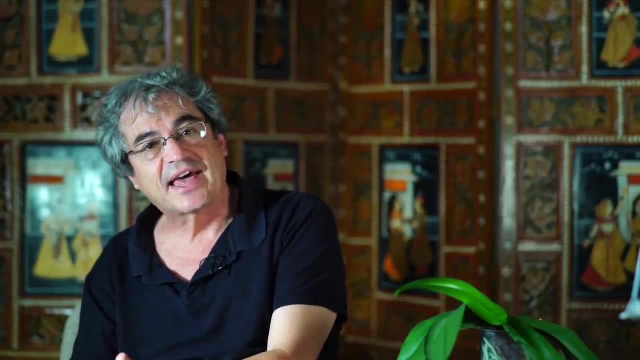 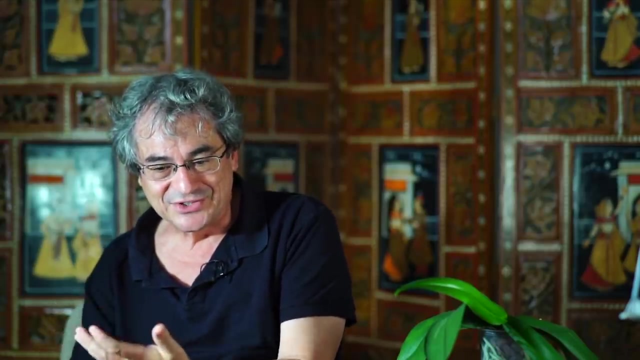 How to calculate the values of the area and the volume of the discrete chunks or atoms of space. We did that in the middle of the 90s. It was another super exciting period And it was the other moment of great sort of collaboration and enjoyment with Lieberman. 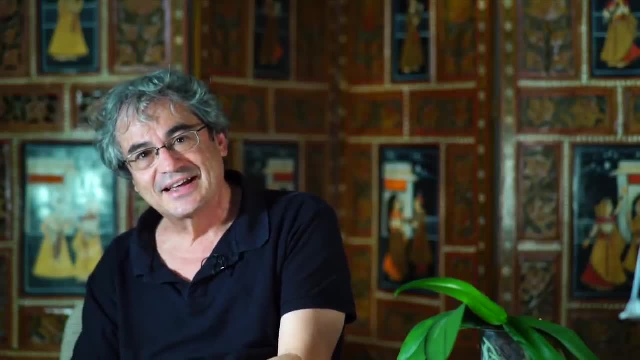 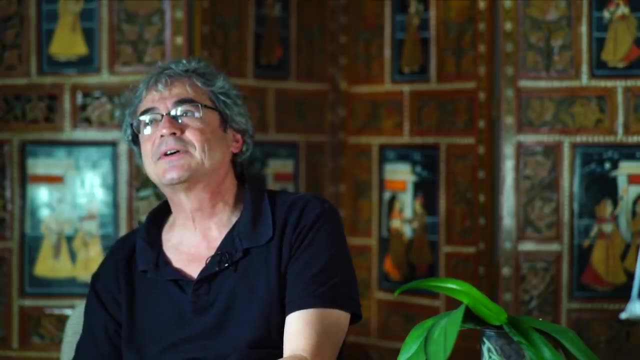 Lie was in Italy at the time. Lie and Abai were often coming to Italy. We would work together And when Lie came one summer it was 95. I think we just realized we could do that. In fact, this is an idea by Lie. 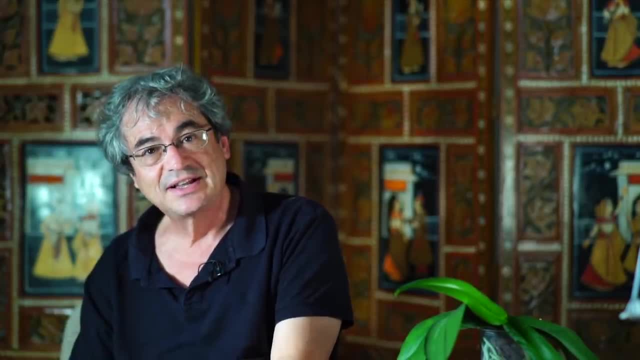 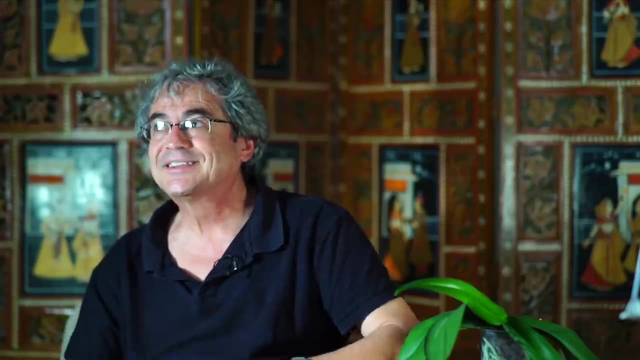 He came and said: we can do this calculation. And we plunged into it And of course we did it wrong at some first moment, And then we corrected it, And that's the moment in which we realized that the mathematics of the universe, the mathematical solution of this spectral problem. 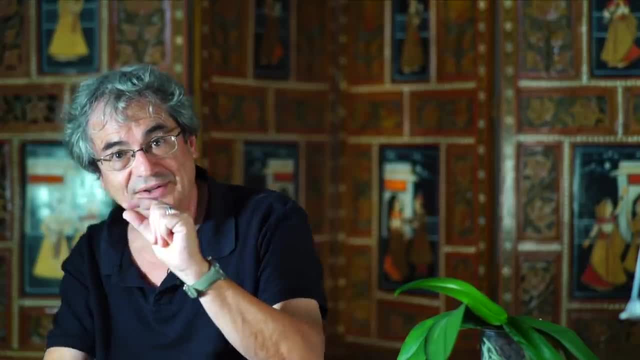 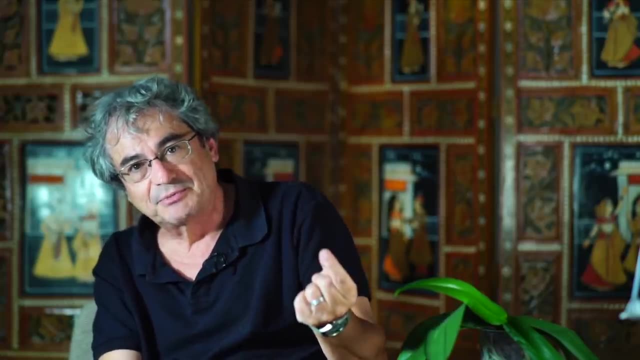 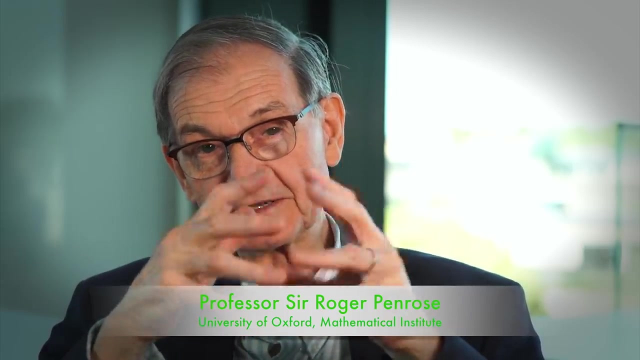 this diagonalization of the operator area and volume to compute the discreteness had as a solution. Roger Penrose, pin networks- I think it was in the early 50s when I'd been worrying about various things that maybe space in the small scale would be discrete in some sense. 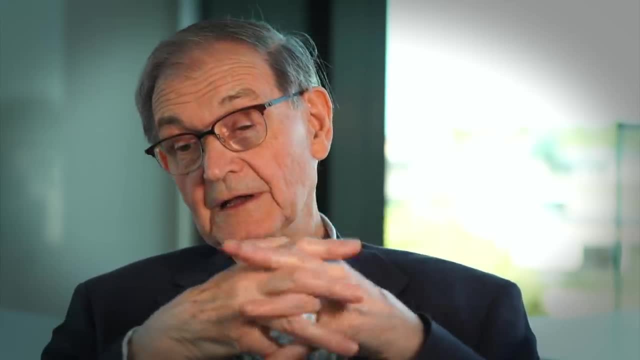 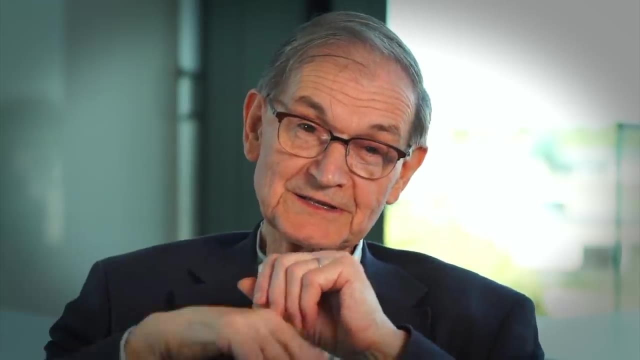 And also quantum mechanical. And also I remember I was a good friend of Dennis Sharma's who used to drive very fast and run his car And when he got thrown to the side he said: well, that's the action of the fixed stars. 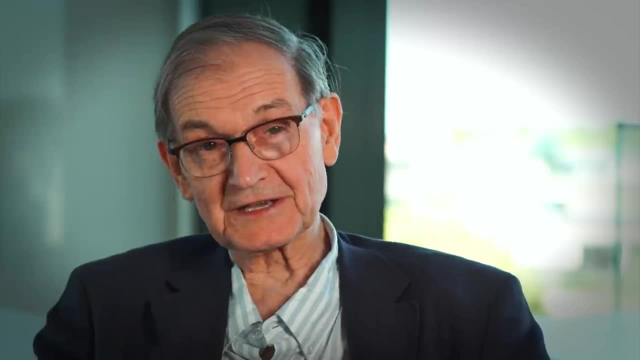 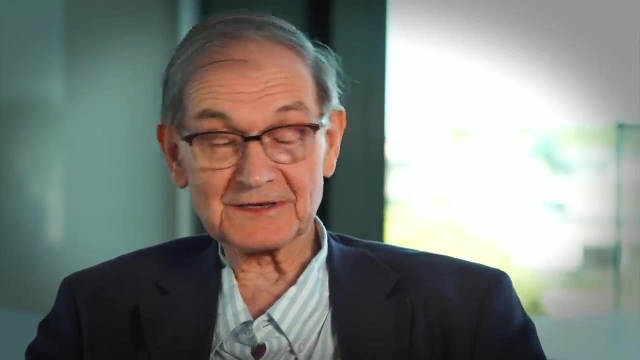 So the idea was that the inertial frame was determined by a distant thing. So we used to talk about what happens if you removed all the stars. Then would you lose your feeling of inertia or something, Or would the car determine your frame? And then suppose you took the car to pieces and took all the atoms away. 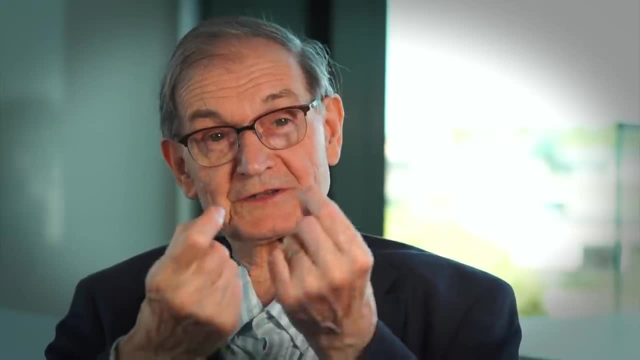 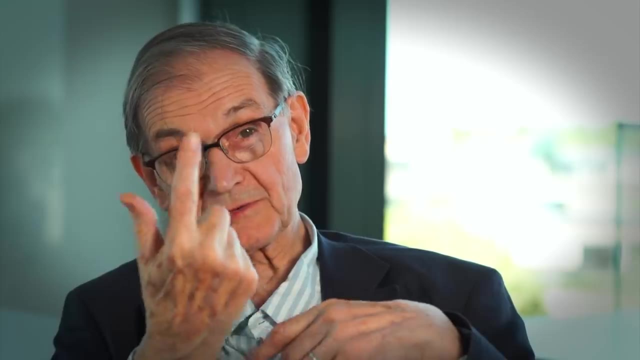 And I thought of the extreme case where there were just two particles left, both of which had spin half. Now you see, in the normal description you'd have a quantum mechanical description would give you, you'd have a direction. The wave function would determine a direction. 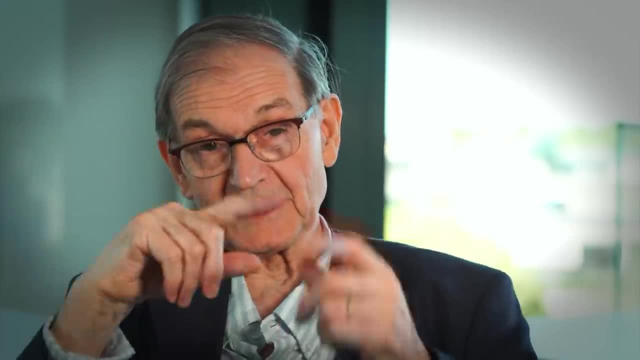 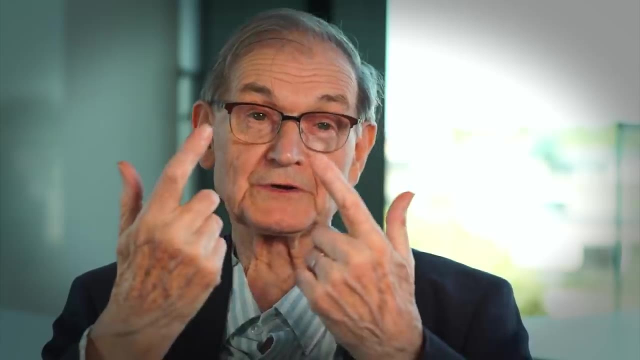 The spin would be about that direction. So you'd have different cases like that. But the idea was that you wouldn't have any concept of direction, You'd just have the only thing you would know would be the total spin. So if you bring these two spin half things together. 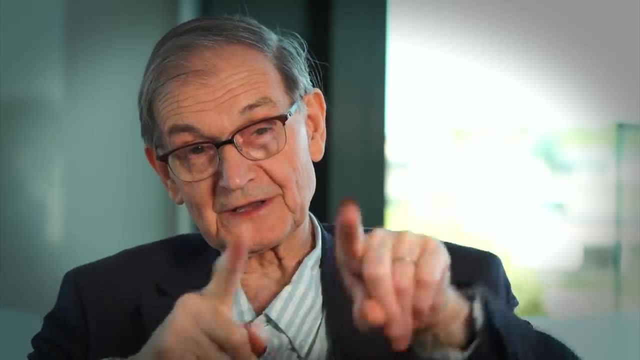 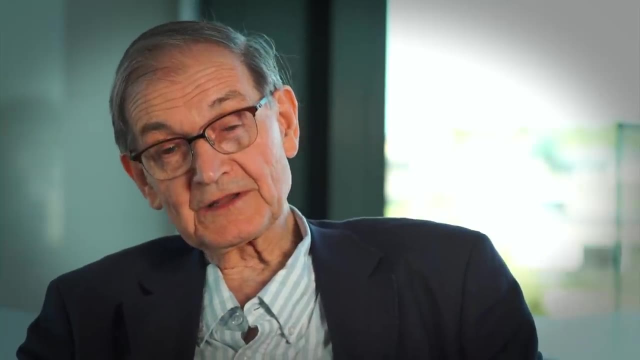 they could make a spin one thing or a spin zero thing, depending on whether they're one or the other, And there were probabilities involved And I thought: well, suppose you bring more particles together, and so on. And then there's the question of how do you know whether the probabilities come from? 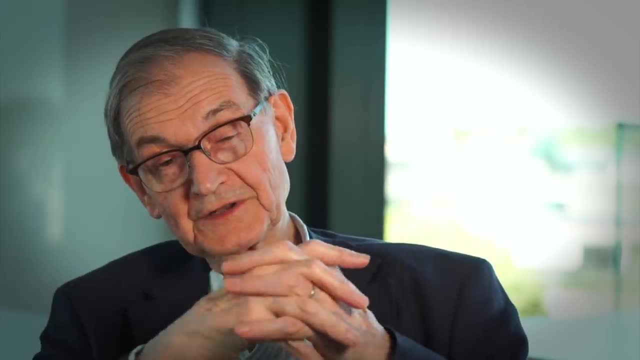 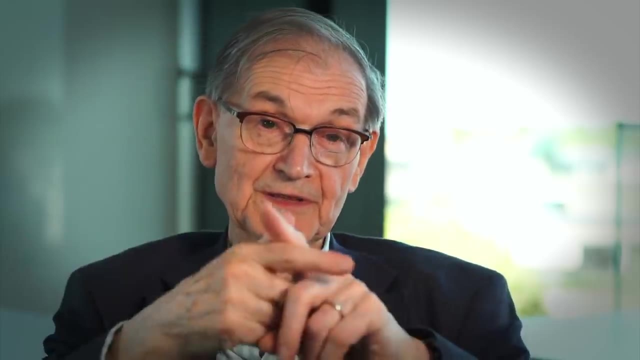 the directions of their spin, in a sense? or does it come from something? just because you don't know? I mean, the probabilities is all you're going to get When you bring these together and take them apart and so on. you only get. 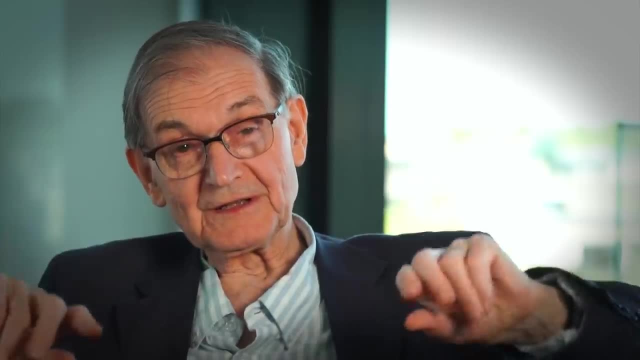 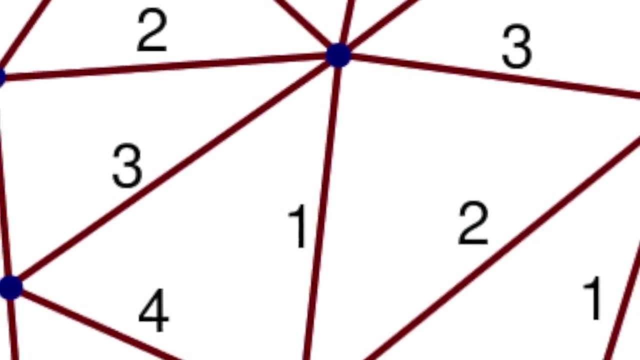 the final thing is you'd have a great network of these. Think of them in sort of time. You have these particles coming together and this one comes together with that And all you know is the total spin value. So this was a way of trying to make a discrete model. 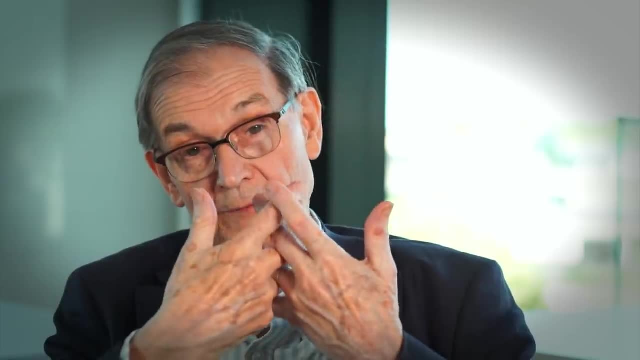 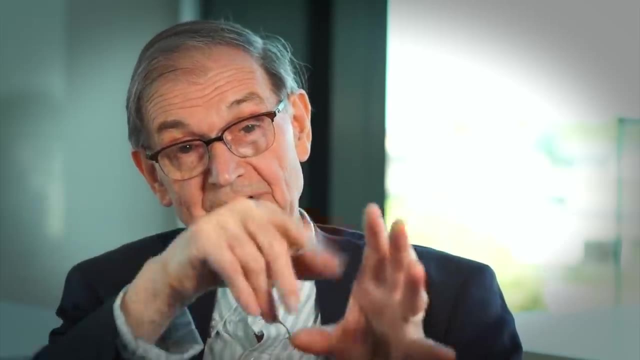 which is purely quantum mechanical, purely combinatorial. You didn't introduce any complex numbers or any differential equations or anything like that. It was just counting loops, counting loops and assigning values to the loops. But I think there were a lot of things in spin networks. 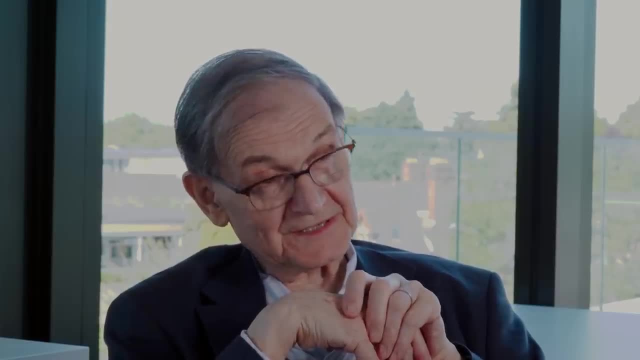 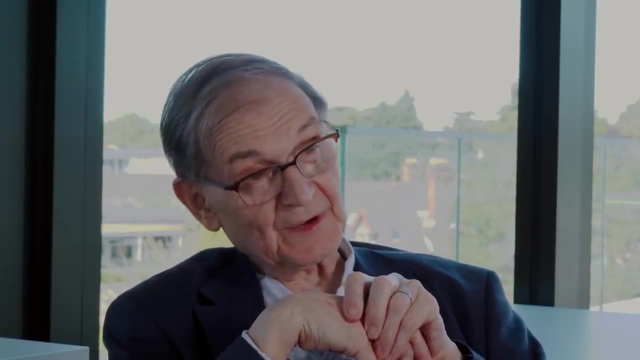 which could have been explored more, and I was glad to see that the loop quantum variable. people did pick up on this or they used the theory in a rather different way from the way I'd originally intended, but it's interesting to see these differences as well. 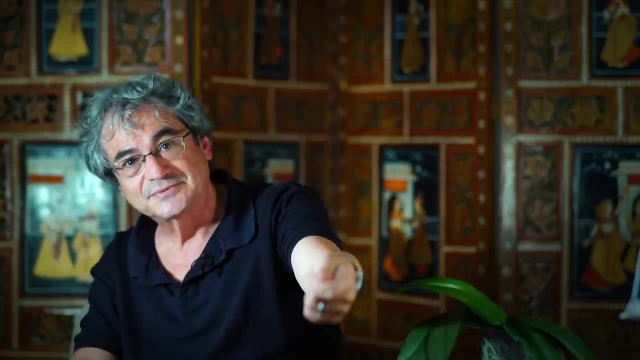 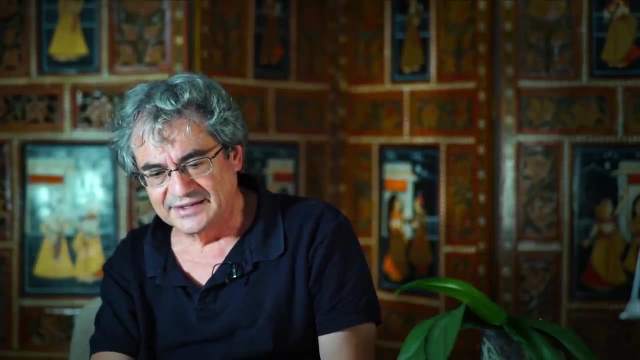 And Lee took a plane. He went to Oxford to talk to Roger because we were confusing whether we should put a plus or a minus there. I remember a phone call with Lee and I asked Lee. so what did Roger say? Is this a plus or a minus? 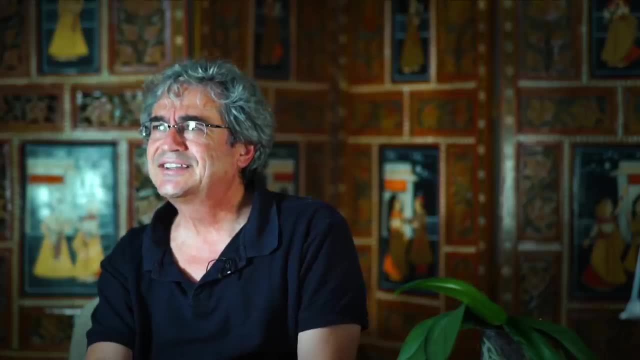 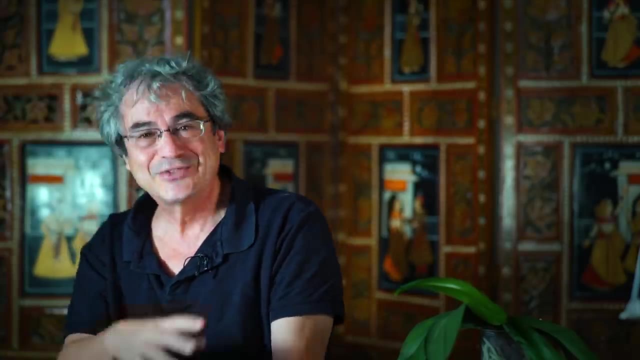 And Lee, with a sort of sad voice, said: well, Roger said it doesn't matter, both are okay, And clearly he was not understanding, nor was I. And then of course, we came out with the technical difficulties. we clarified that and this is a 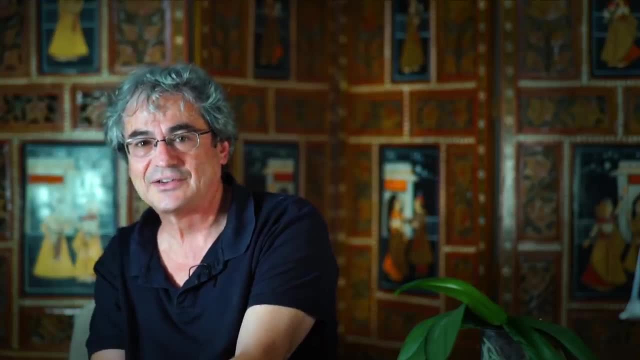 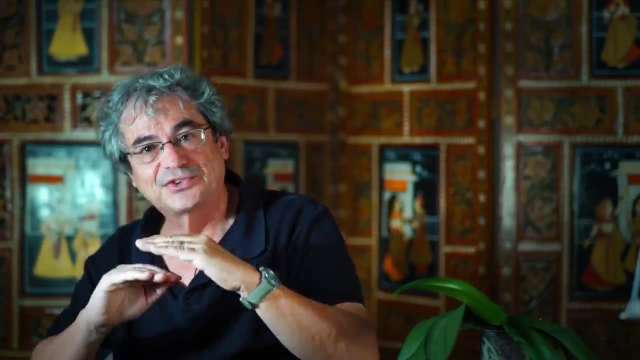 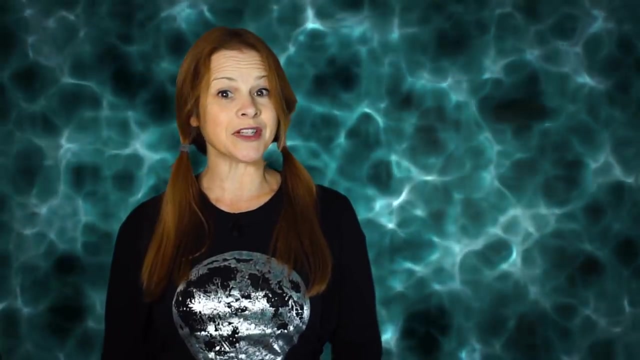 technically. I think this is a major success of loop quantum gravity because it's a precise prediction of the discrete values. Well, Roger Penrose was not directly involved in the development of loop quantum gravity. It's no surprise that his ideas were influential. 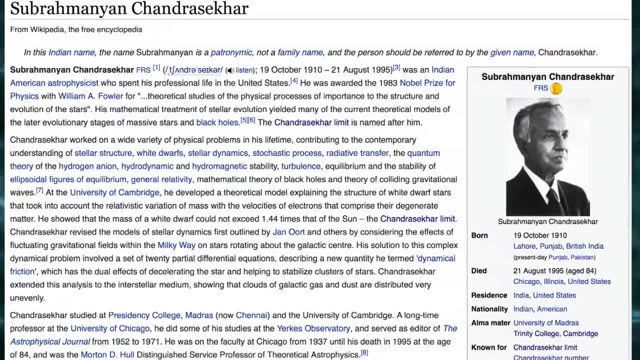 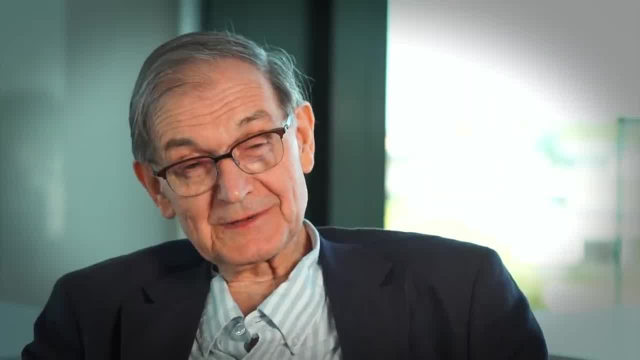 not least because Abhay Ashtekar, on the recommendation of the great physicist Subramanian Chandrasekhar, was one of Sir Roger's postdocs. I'm sure he came with extremely good recommendations, or else we wouldn't have taken him on. 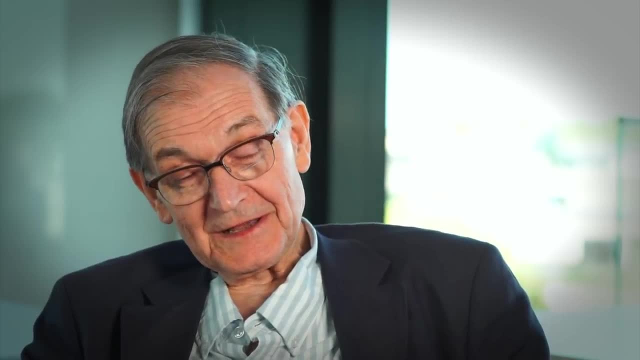 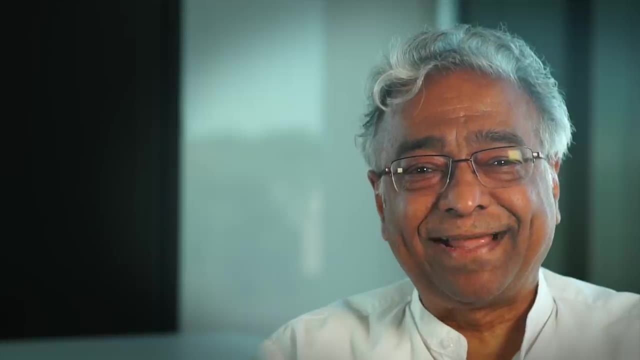 And he obviously fulfilled these recommendations and I was very impressed with what he'd done. Chandra felt that the place I should go to was Oxford and that was to work with Roger, So Chandra actually apparently wrote. Roger told me this much later. 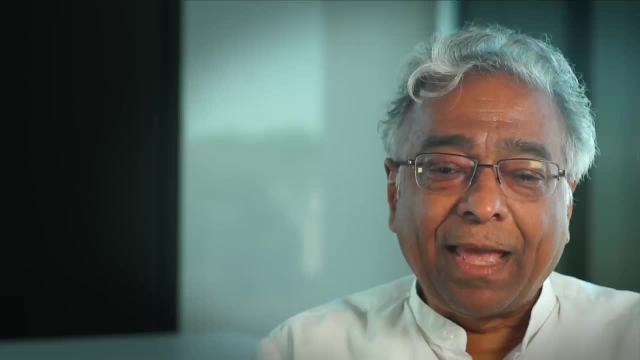 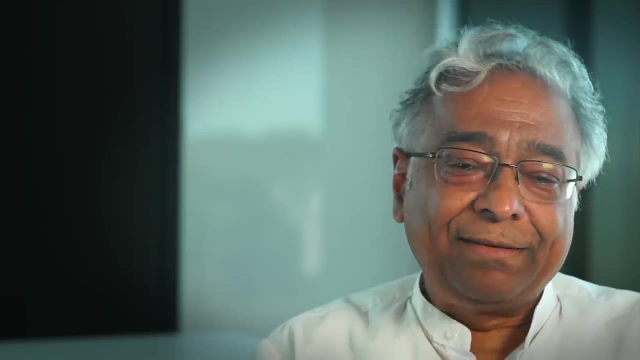 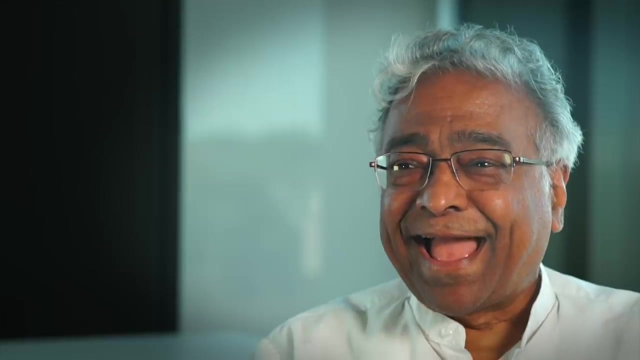 a letter completely unsolicited for me. I also then, after Chandra told me this, I actually applied to this position. And then, you know, eventually I got a telegram from Roger saying offering you a postdoctoral position. do you accept? 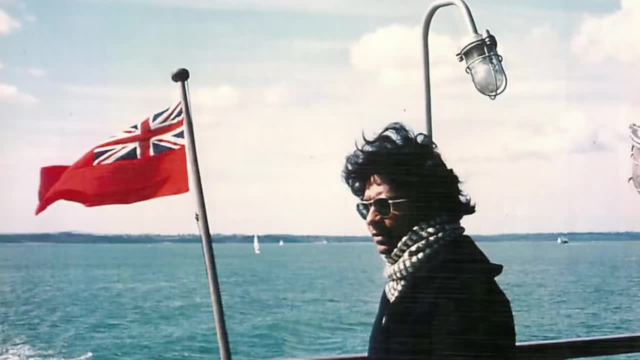 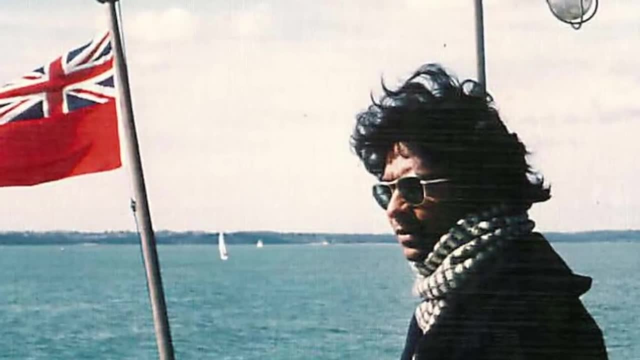 And I didn't know what it meant because I was a poor graduate student and in any case from India. there was no way to get any money from anywhere. So I called him and Roger, of course, didn't know what the salary was. 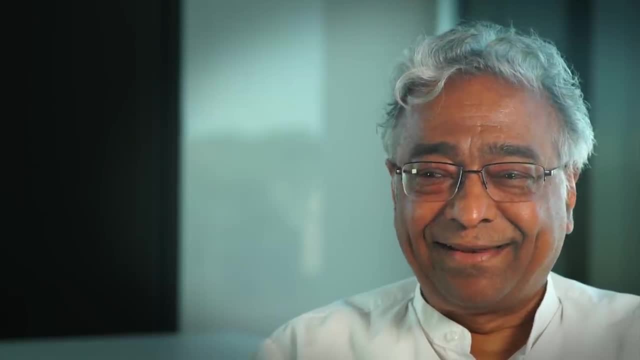 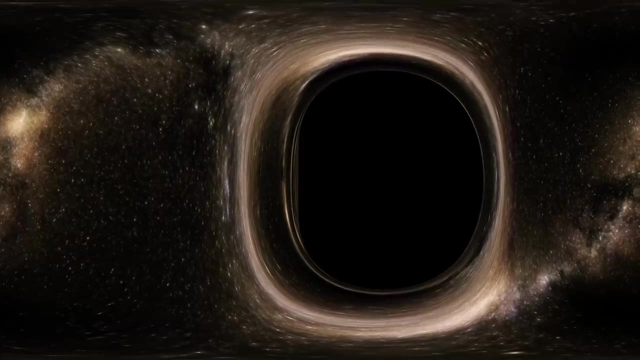 So I said, is it enough to live on? And Roger said yes, yes, I said okay, I accept. So that's how I came to Oxford In the 1970s. Stephen Hawking and Jacob Bekenstein. 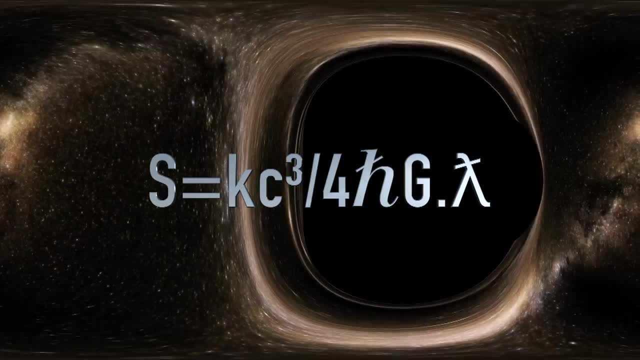 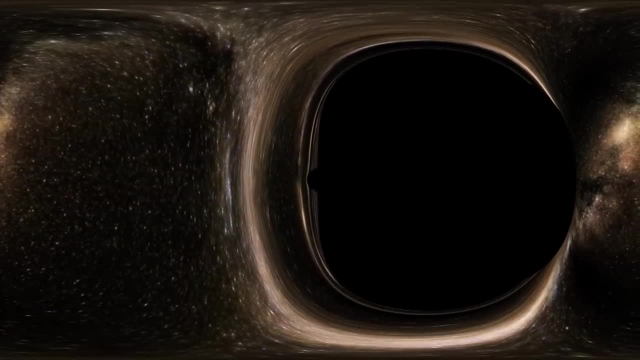 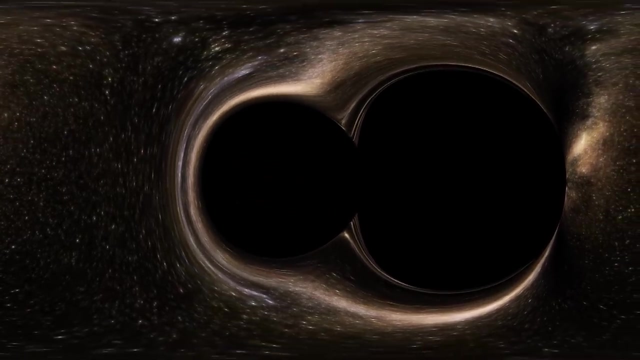 had shown how to calculate the entropy of black holes, But this was based on the assumption that space is continuous. Two decades later, loop quantum gravity researchers began to wonder if the formula could be recovered from the principles of the discrete quantum space time. 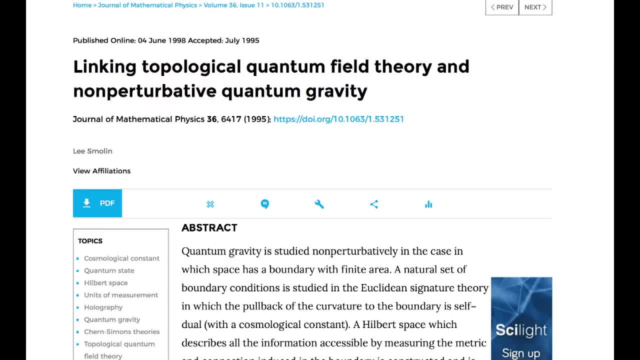 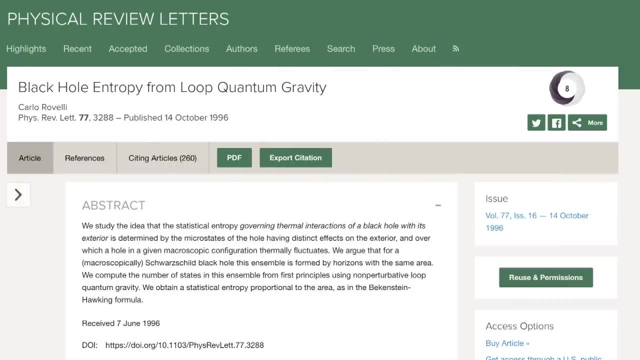 After some preliminary studies which revealed pieces of the puzzle, the full computation of black hole entropy was presented in a landmark paper by Ashtakar Baez, Corici and Krasnov. And it is very simple: A black hole has a surface. 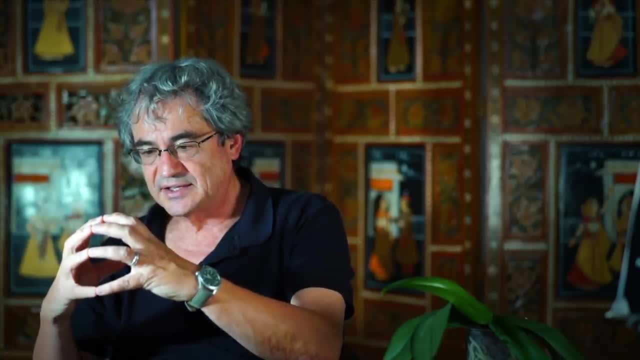 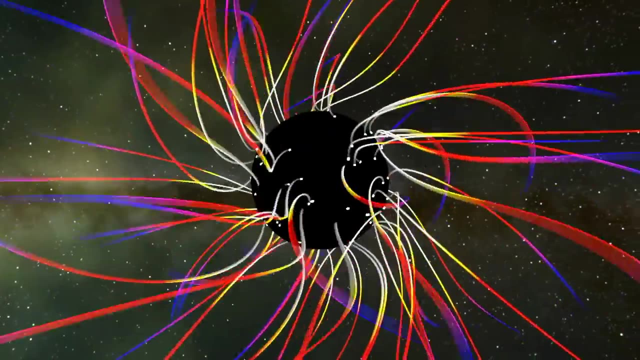 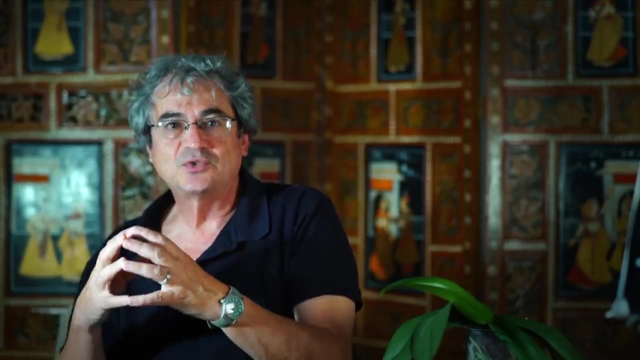 which is a sphere and the quantum state of the geometry are loopy, so are little lines that punch this sphere, And on any punch there is some degree of freedom. When I say degrees of freedom, I mean the independent ways in which something can move. 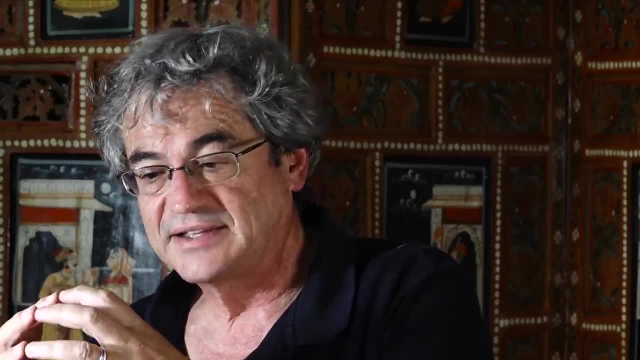 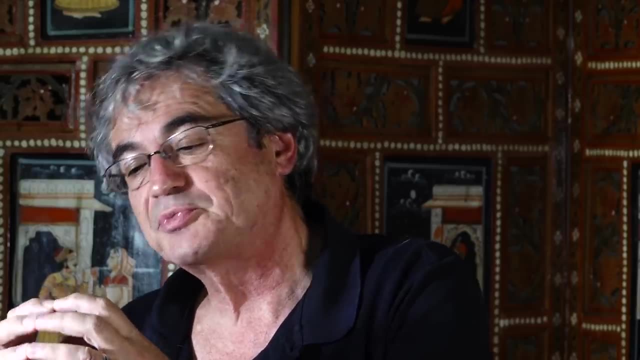 And you just count this degree of freedom, and the number of them should tell how many degrees of freedom there are on the surface of the black hole, Which correspond to the geometry of the horizon. So the horizon is a sphere, but it is not exactly a sphere. 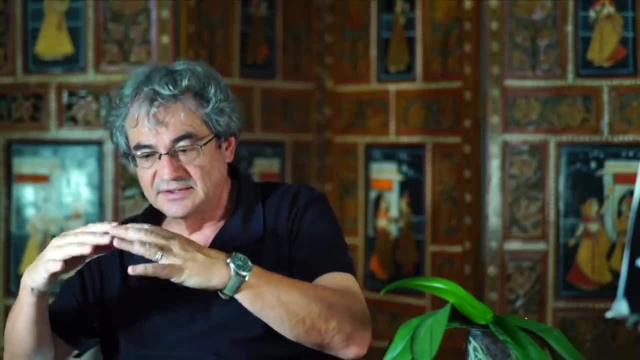 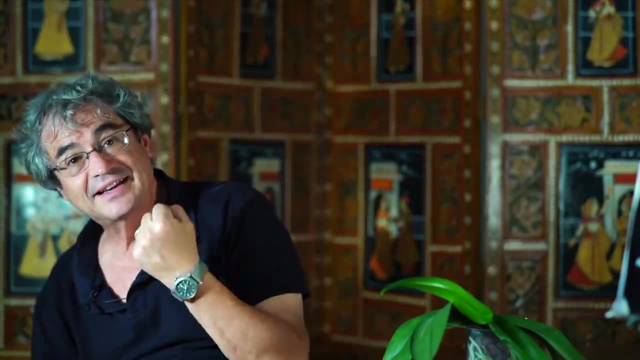 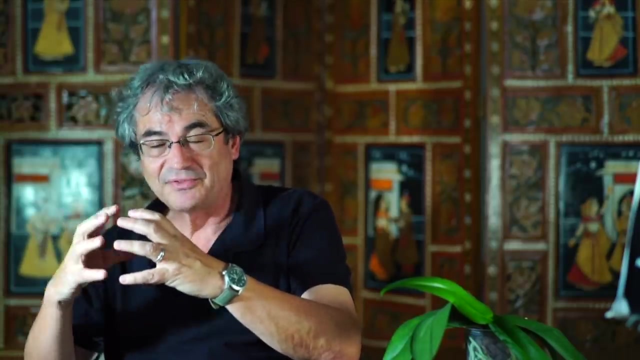 it is a sphere that can move, fluctuate, and these fluctuations are degrees of freedom that sits on the surface and you can count them, And in the classical theory they are infinite, of course, because geometry is smooth, so you can do arbitrary small fluctuations. 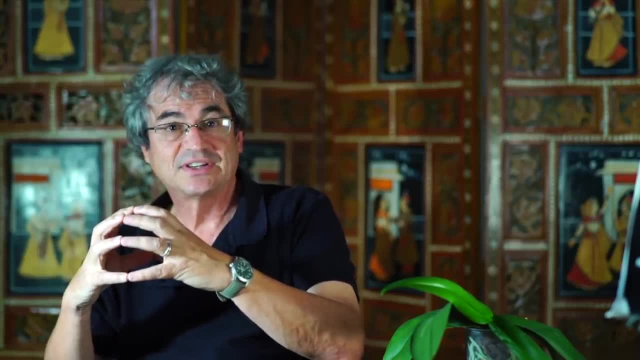 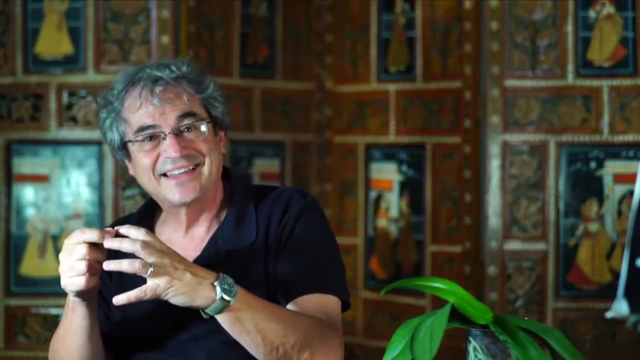 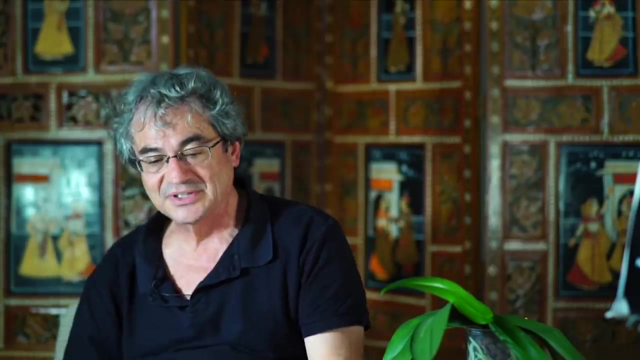 But in loop, quantum gravity, there is no continuum geometry, it is discrete geometry. so there is no, there is no excitation smaller than the scale, the minimal scale of the geometry, which is the Planck scale. So you can count the number of fluctuations on the geometry. 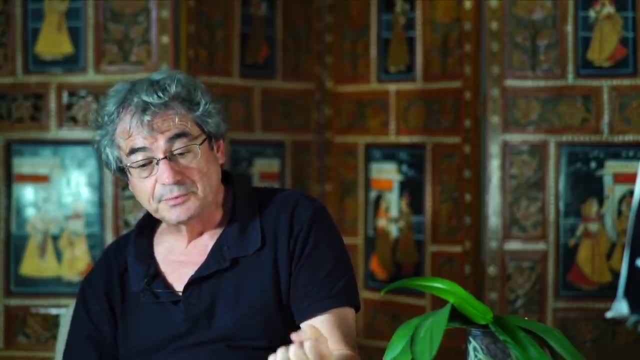 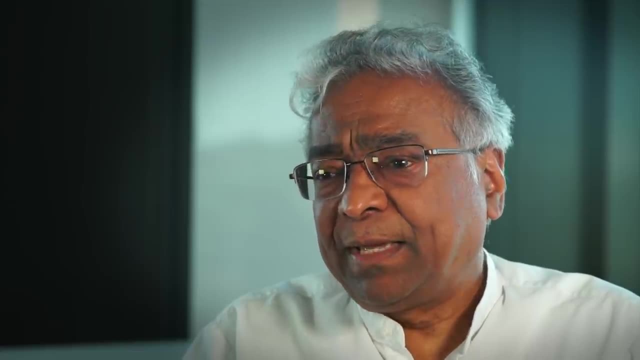 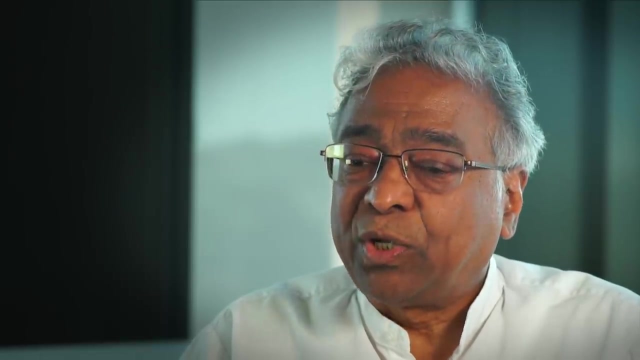 and the counting of degrees of freedom correspond to a calculation of the entropy. When we do loop quantum gravity, there is a certain ambiguity in quantization. This is not uncommon. There is a similar ambiguity in quantum chromodynamics, the theory of strong interaction. 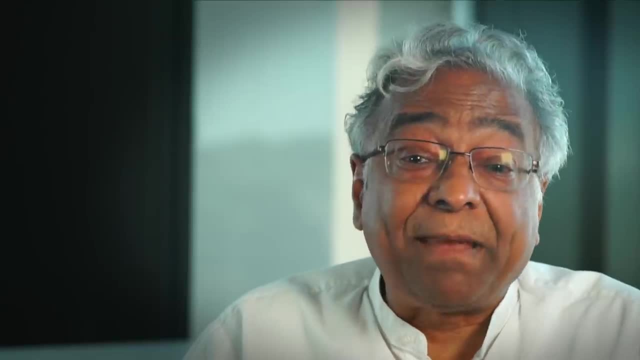 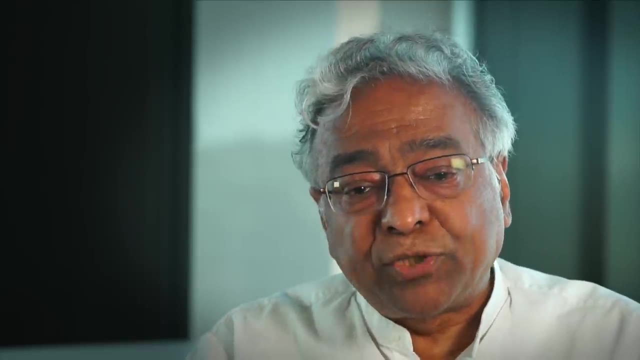 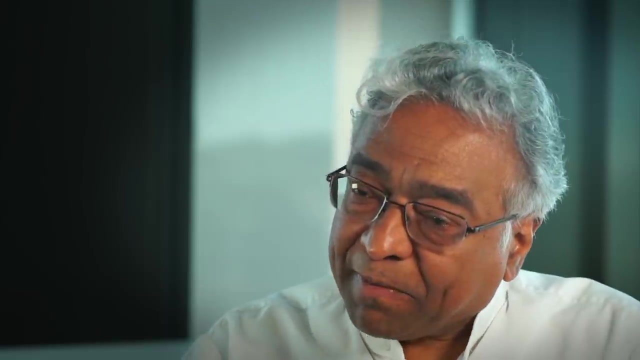 which is called the theta ambiguity. And so theta is a free parameter in quantum chromodynamics, It is no classical analog and its value is determined experimentally. So similarly there is ambiguity in the in the in loop quantum gravity when you go from classical theory to quantum theory. 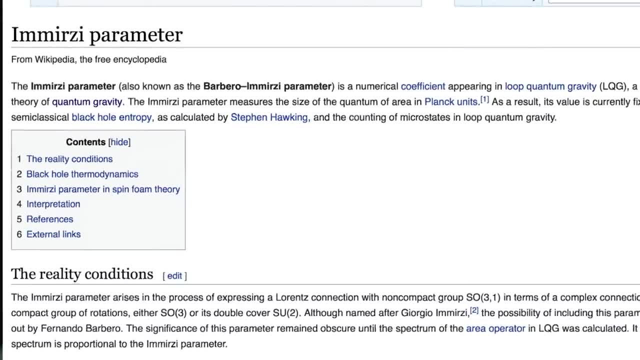 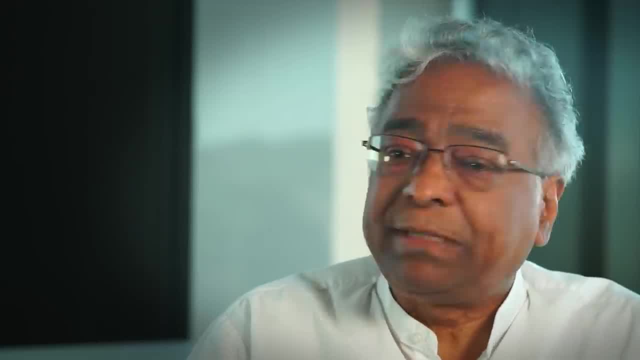 and it is called the Barbero-Immerzi parameter. If there was an experiment by which I could measure the smallest area gap, I would know its value and the theory would be determined, and I would be happy. But this is far beyond any technology. 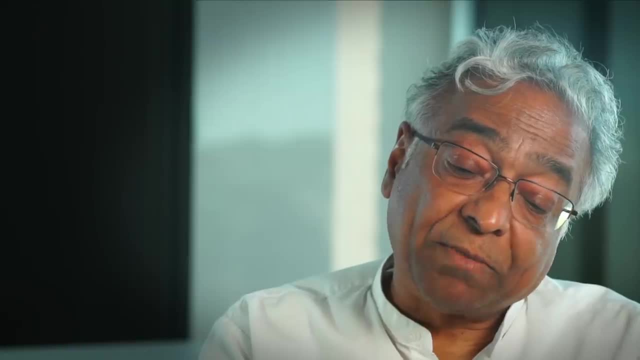 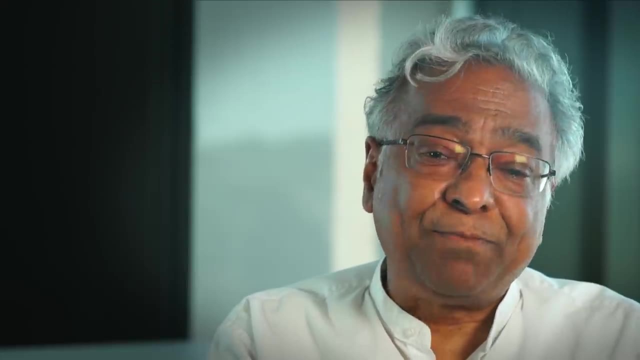 We don't even know how to think of such experiments today, Since the quantum of area depends on the Barbero-Immerzi parameter, the number of microstates depend on this parameter, And we just blindly put this parameter equal to the value that is needed. 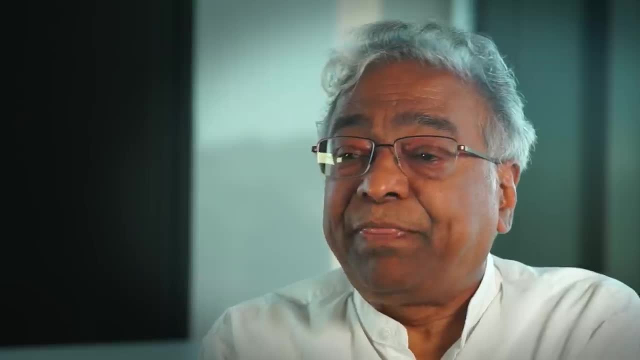 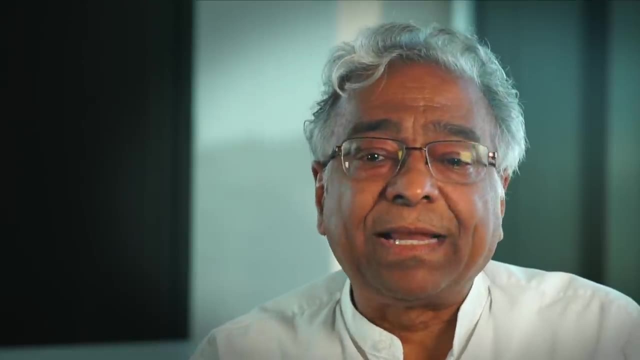 to get agreement with the Bekenstein-Hawking formula. This requirement fixes the Barbero-Immerzi parameter, But I did it just for one black hole, And now one can ask the question about any other black hole and one finds that the 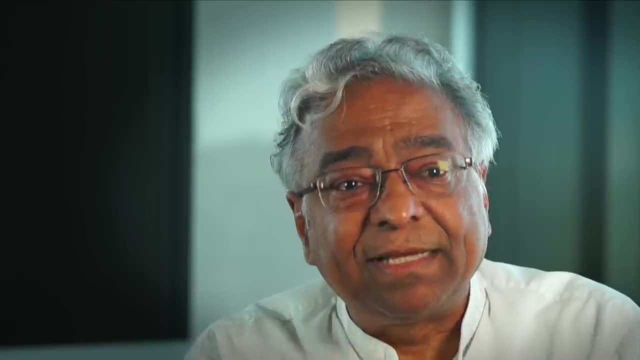 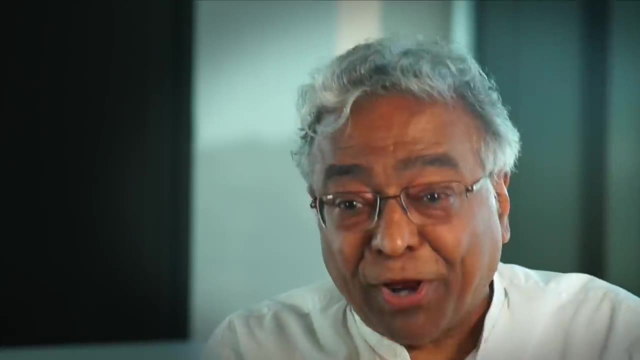 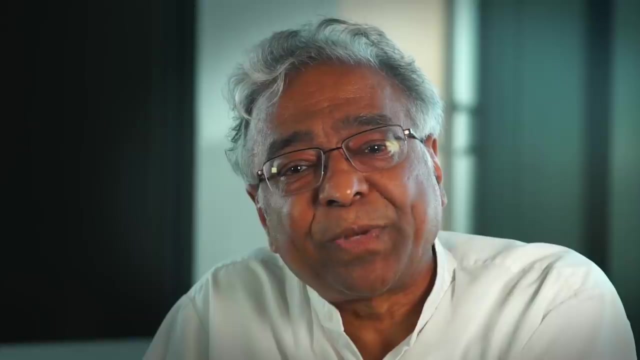 the leading order term is again the same. So in that sense there is a check on this Barbero-Immerzi parameter and this area gap. More recent work in cosmology is also giving checks on this, this area gap, and therefore indirectly on the Barbero-Immerzi parameter. 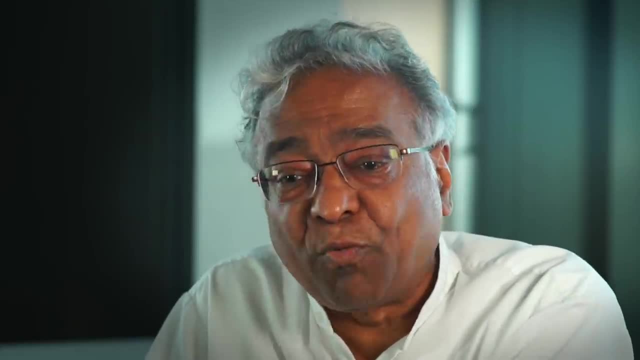 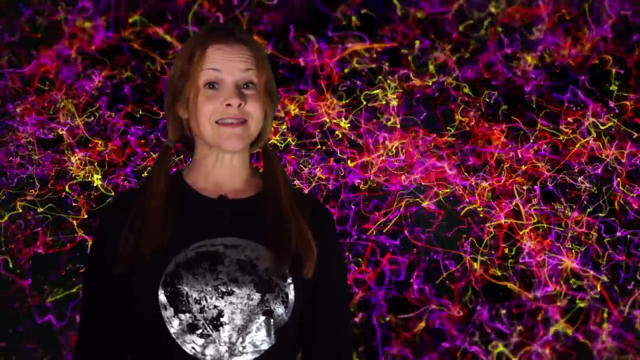 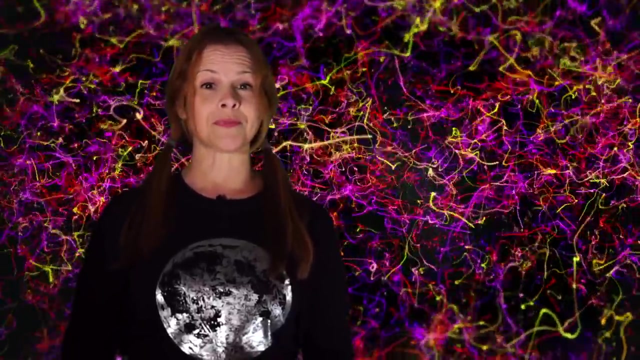 We can leave this as a free parameter and determine it using one of the two methods and then check if it is true in the other one. Loop quantum gravity is not the only theory to have success in the field of black hole entropy. String theorists also claim to be able to infer this formula. 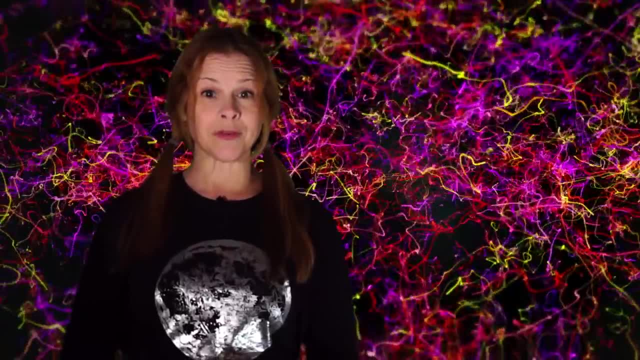 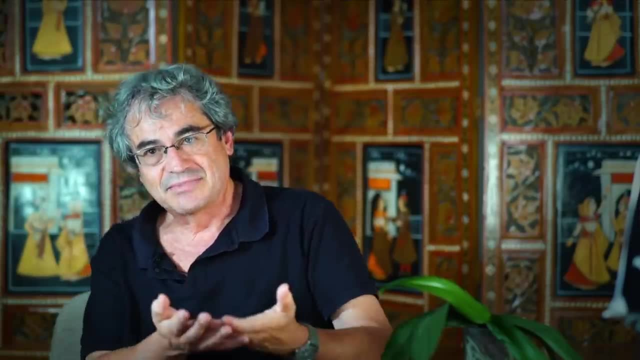 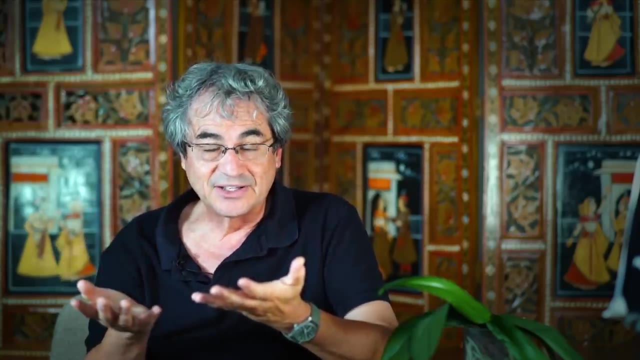 But one of the key differences highlighted by loop theorists is the background-independent nature of the theory. You do quantum gravity not by having a space and physics on this background, but rather by doing the quantum physics of space itself. That's background-independence, very simply. 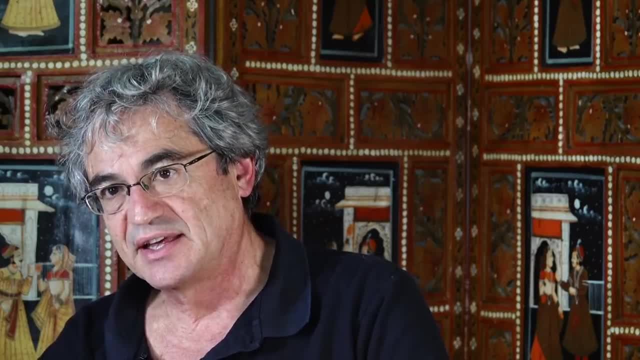 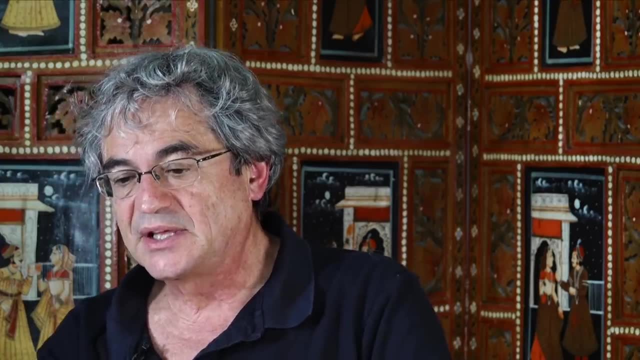 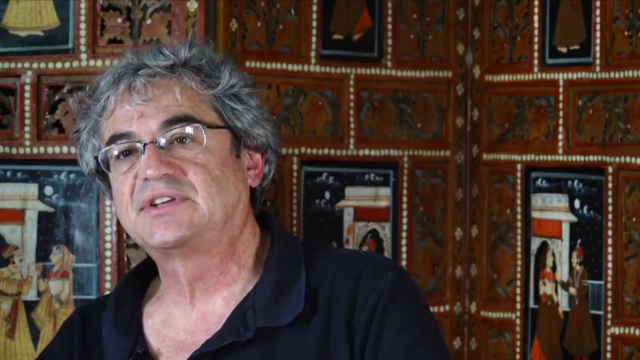 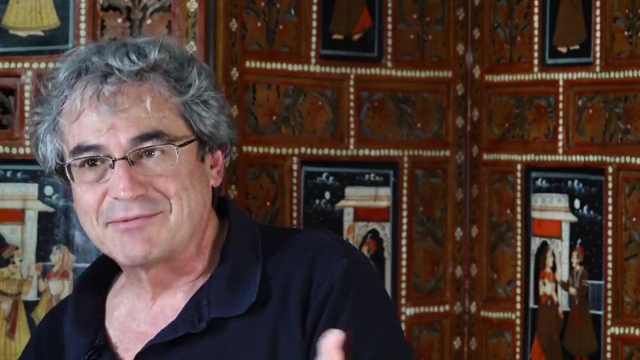 String theory developed as a background-dependent theory, so developed on a fixed space. In recent years there have been a lot of effort to bring string theory into a background-independent language. In fact, in some sense the ideology of string theory has come much closer. 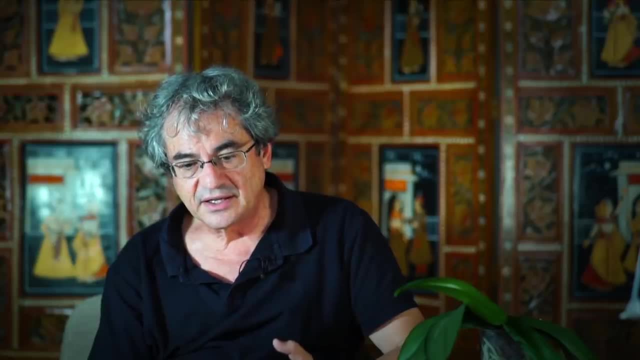 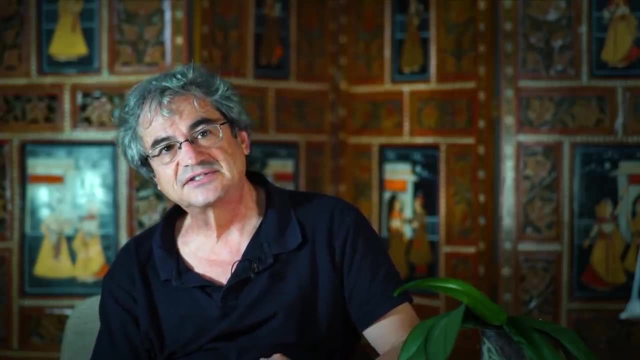 to loop quantum gravity in recent years. It's a very beautiful idea, string theory. It's a very courageous attempt. I think it has not delivered. A lot of beautiful things have come out of string theory, But the project of making a theory of nature. 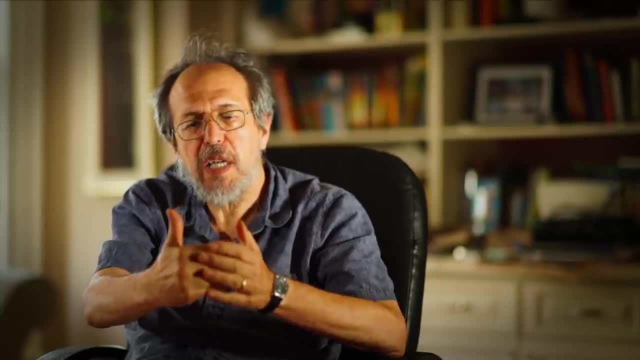 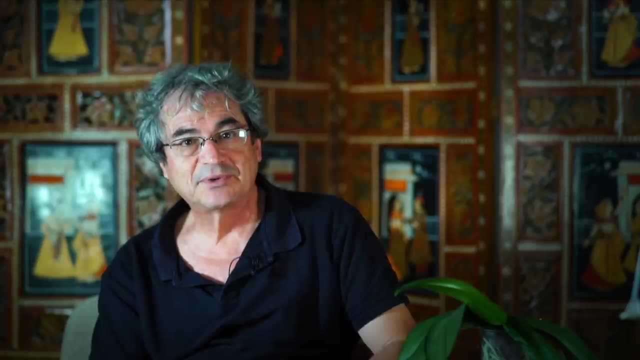 on string theory is, in my judgment, basically stuck. The dreams of the eighties have not come true. Nobody has been able to compute the parameters of a standard model, Nobody has been able to derive the groups of the standard model, and so forth. 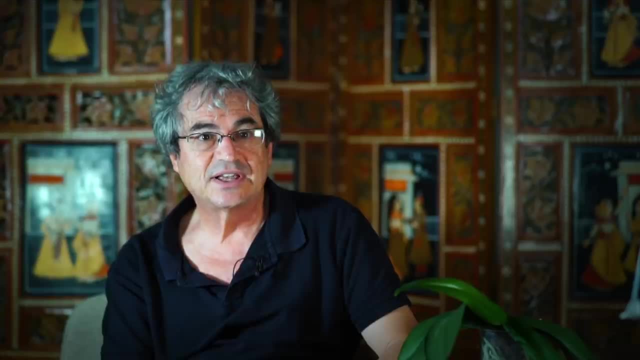 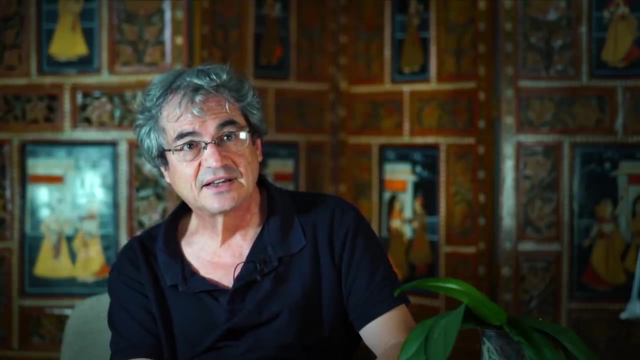 In fact, the few predictions, so to say, of string theory have been disappointing, because one sort of prediction in which most string theories were very convinced of was that if there is a cosmological constant, it has to be negative. Then the cosmological constant was measured. 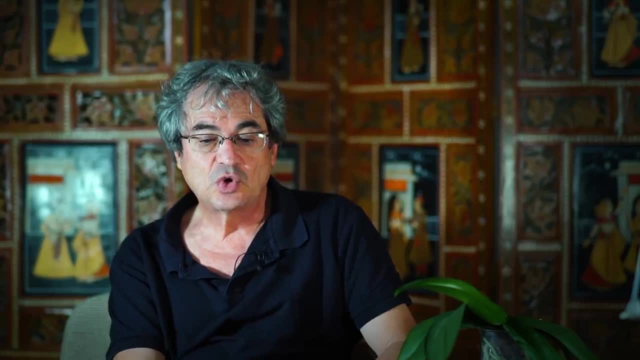 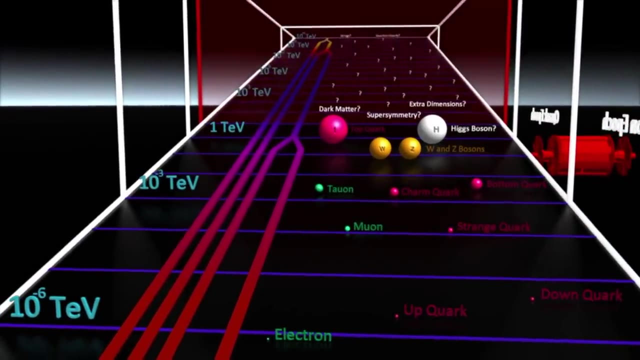 and turned out to be positive, And the other prediction was that we were supposed to find supersymmetry at low energy, at LEP or LHC, and it did not come out. This doesn't mean it's necessarily wrong, but I think as a research program. 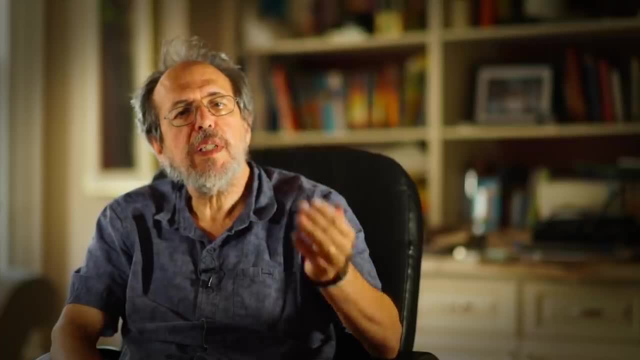 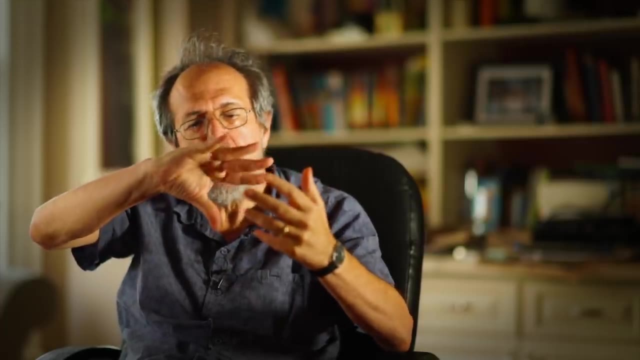 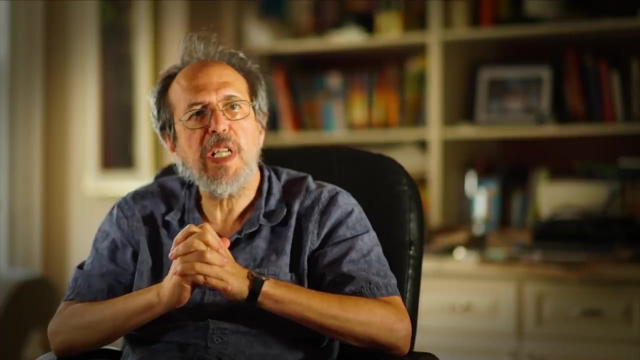 it's losing ground. String theory comes in an infinite number of versions because it has to have these extra dimensions, with there being an infinite number of ways to tie up the extra dimensions, And so there's a huge problem of empirical content, or predictivity. String theory really, at a fundamental level, appears to require supersymmetry And in loop quantum gravity supersymmetry or higher dimensions or a negative cosmological constant are not at all necessary. Loop quantum gravity is not claimed to be a theory of unification. It doesn't offer a specific way to unify gravity with the other forces and unify them with the different elementary particles. the way that string theory, at least initially, was thought to provide such an insight into unification Loop quantum gravity is far less ambitious. 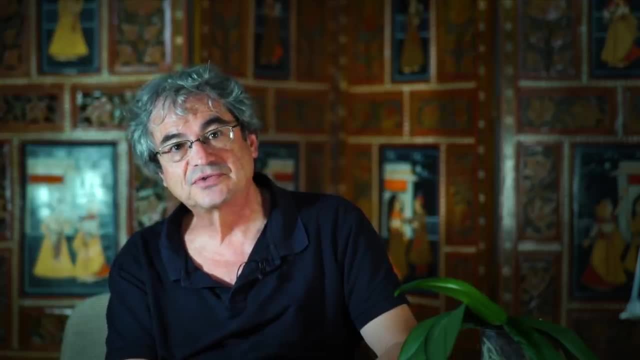 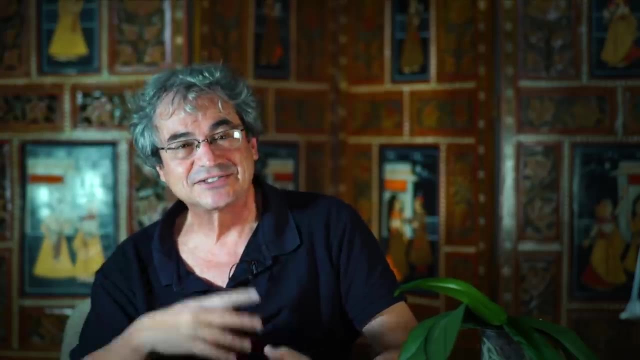 I personally think that we are not at the point of writing the theory of everything. We don't know probably a lot about the universe, and maybe there are other fields, other particles, other, whatever We don't know. So we better do one problem at a time. 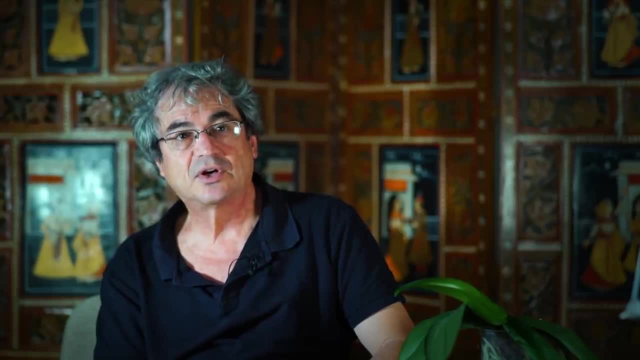 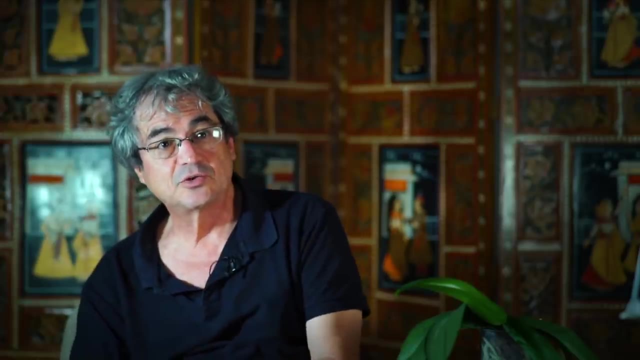 And the problem of the quantum aspect of gravity is a well-defined problem. We have a lot of information about it, so we can write a theory just about that And loop: quantum theory is a theory about that. So it's a quantum theory of gravity. 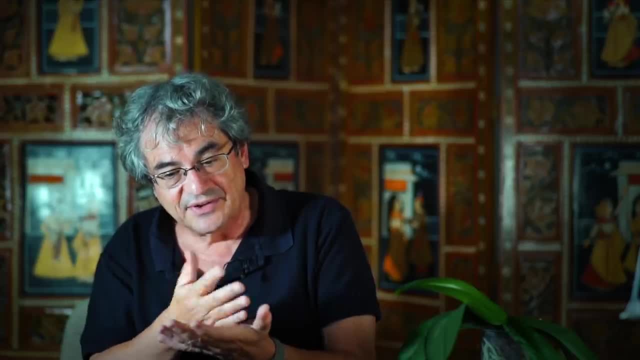 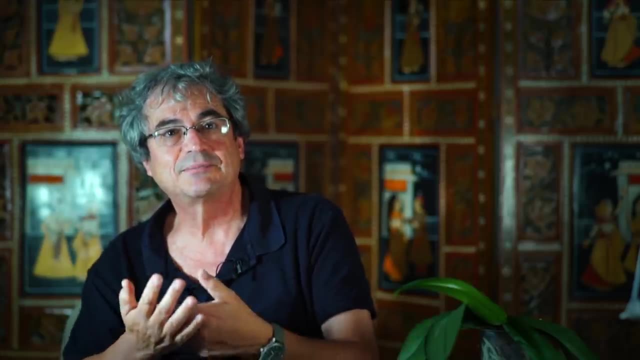 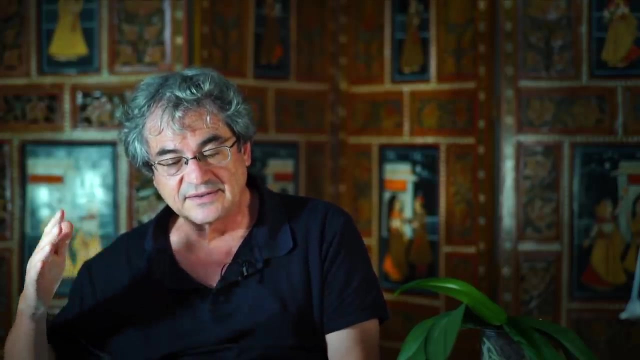 And I would say it has happened the opposite of string theory, because in the 80s, when we started, there were a lot of unclear issues and things that seemed very hard to go ahead with, And it has progressed in the 90s and at the turn of the millennium. 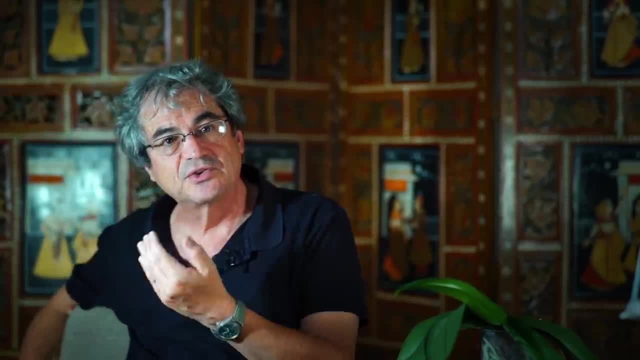 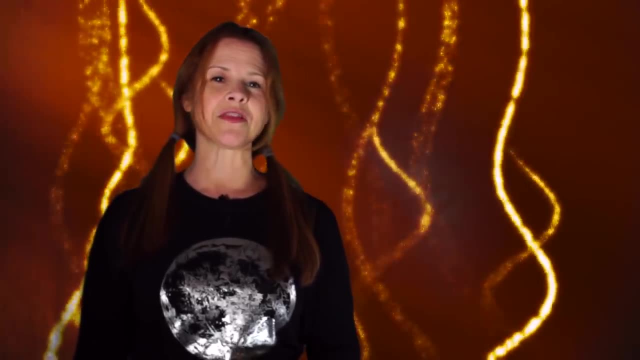 and in this first 20 years of the new millennium, more and more and more. And each big problem has been solved. A frequent criticism of loop quantum gravity is that the theory can't specify the dynamics of how a system evolves. One way of breaking 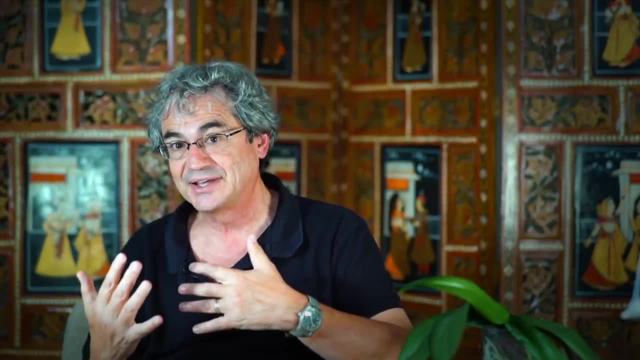 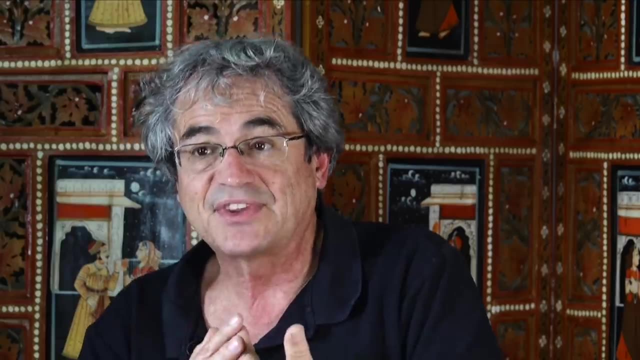 the definition of a theory, especially a quantum theory, is to separate the kinematics and the dynamics. The kinematics is everything you can measure. The dynamics is how things move. One still finds this, this comment, loop, quantum gravity, one doesn't know. 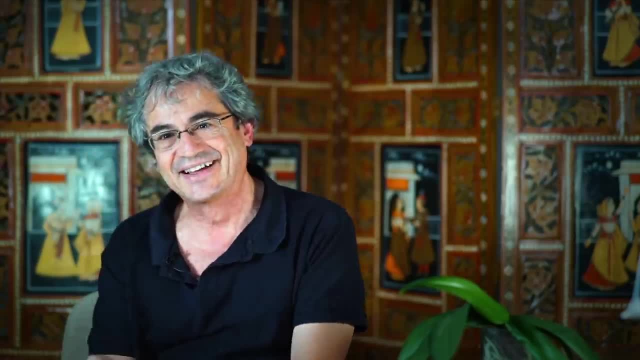 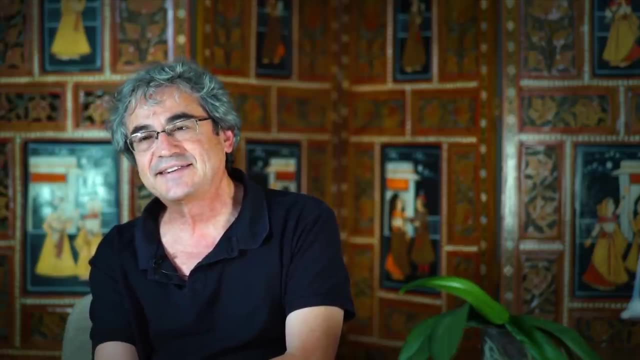 how to write the dynamics, But this was 25 years ago. There is some criticism about loop quantum gravity, which keeps bouncing since I was a kid. No well, since I was in my 30s, And people just haven't read the last 25 years of literature. 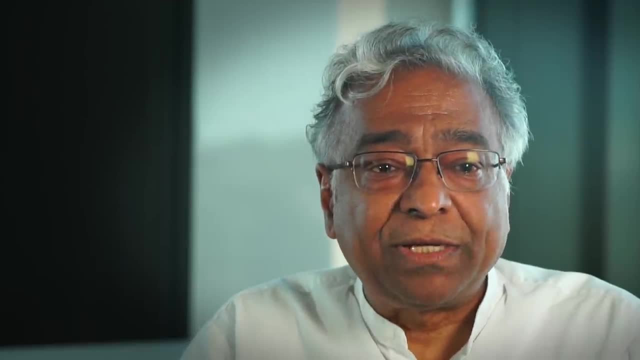 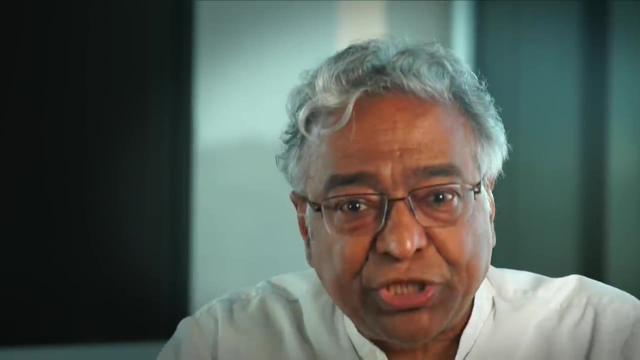 For full general relativity. I don't have a general solution of Einstein's equation, But let me go to a physical problem like a spherical black hole, Then I can write and I know what the solution is, Or a certain cosmology. 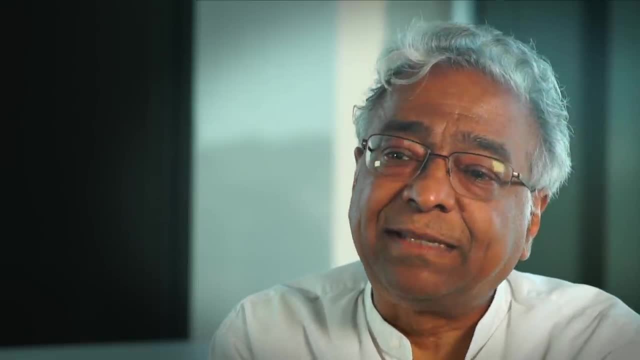 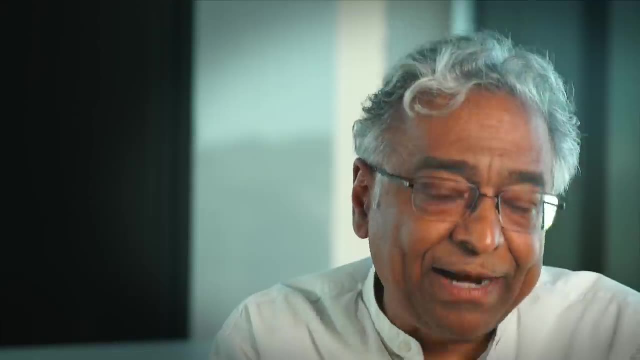 then I know what the solution is, And so loop quantum gravity has done the same thing And concrete proposals for dynamics have been made, have been verified, have been checked in many, many ways in these models And I think today the loop quantum gravity. 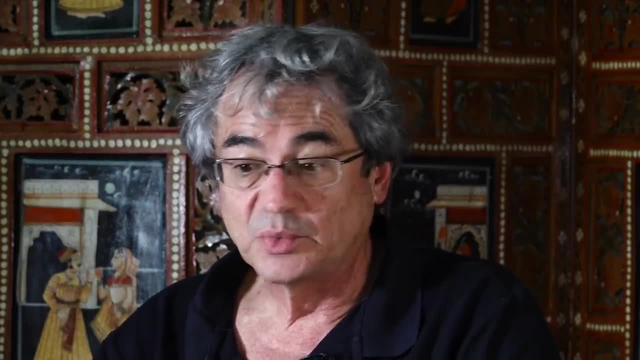 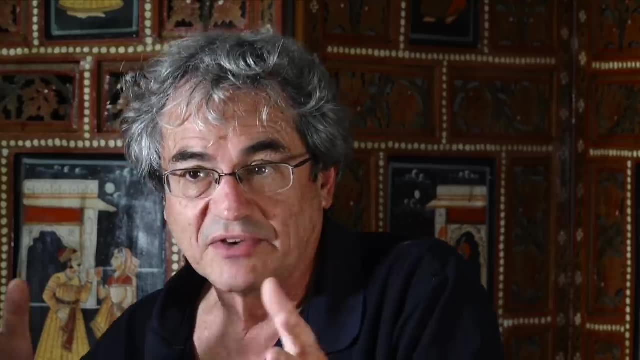 is in a good shape. There is a theory. We know the basic equations. We know that in the classical limit it gives general relativity. We have a lot of indications of that. Is it the right theory, or is it not the right theory? 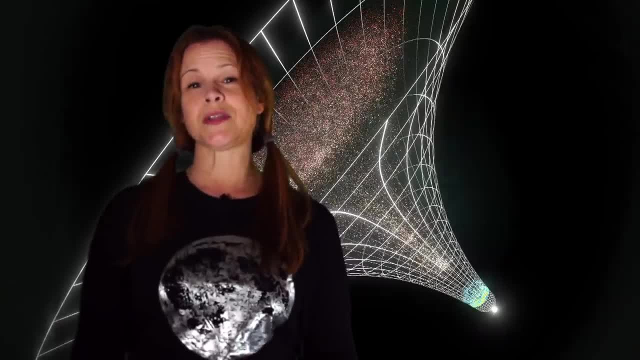 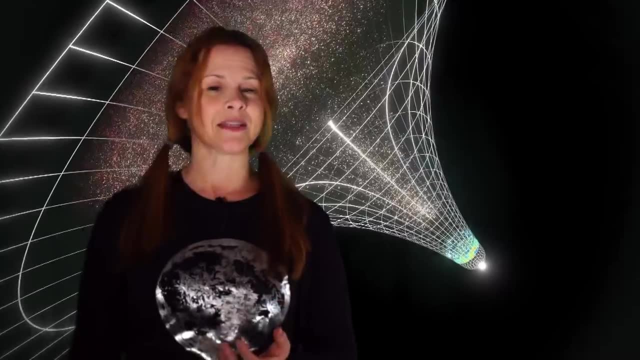 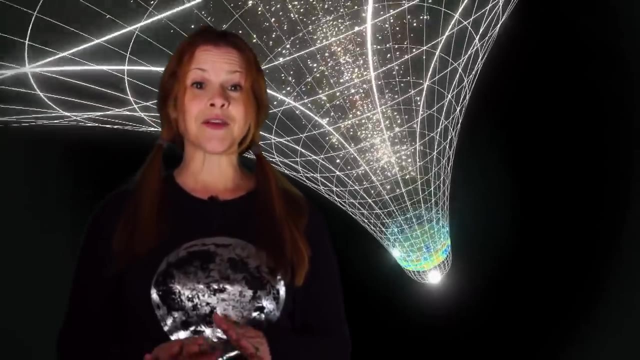 And for that we need to apply it. In order to determine if loop quantum gravity is right. it has to make novel predictions about nature which are confirmed by experiments, And perhaps the most stunning application of loop quantum gravity has been to the very origin. 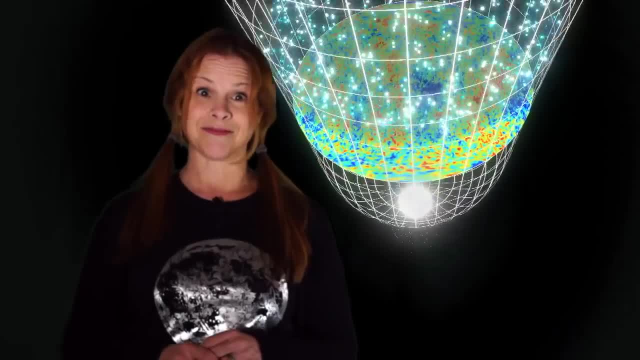 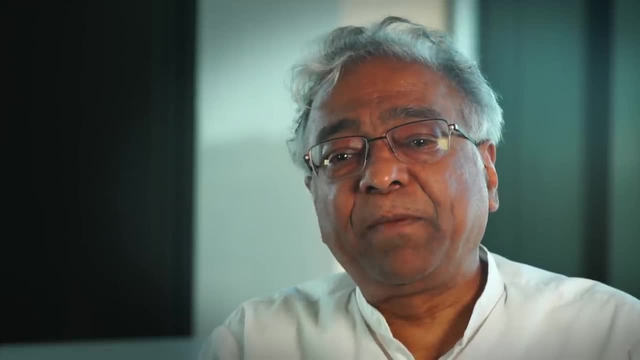 of our expanding cosmos. the Big Bang, When it was first put forward and, you know, also studied by people like Lemaître in detail, the Big Bang was really the beginning of the universe. I mean then. Now I think 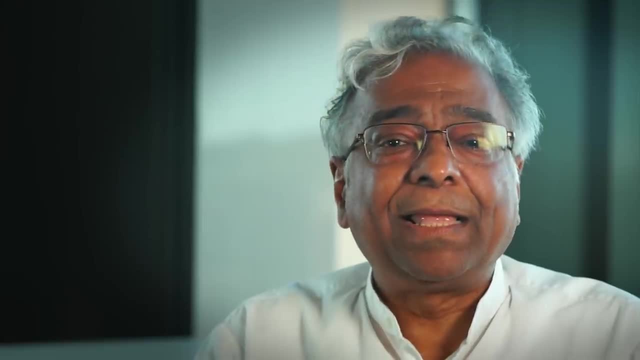 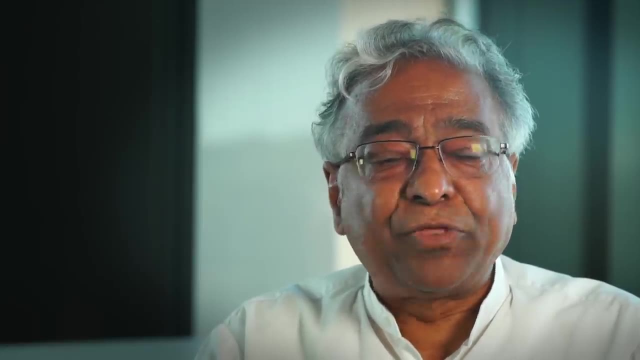 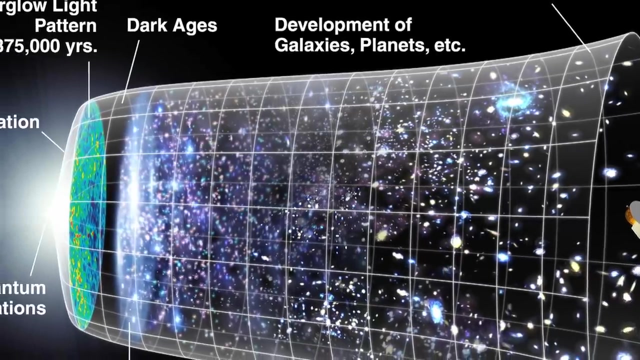 the working cosmologists of early universe think about the Big Bang as really the time at which the universe became hot. So it is a time at the end of inflation, Say, for example, in the inflationary scenario, During inflationary era. people don't often emphasize this. 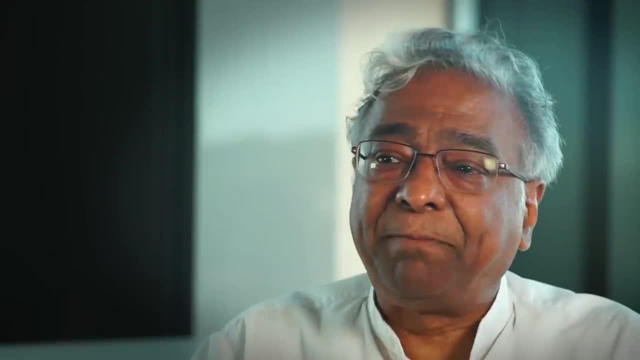 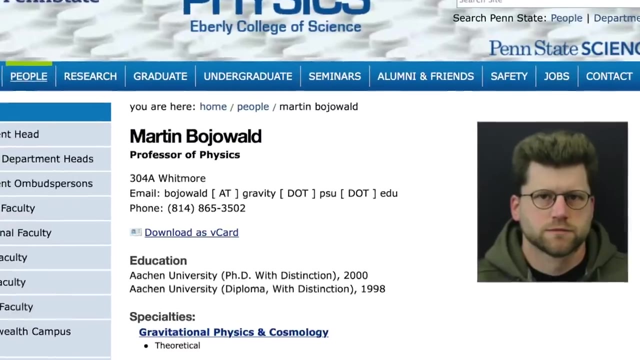 what is using quantum field theory at zero temperature? Big Bang is really a prediction of generativity in a regime where it is not applicable. Martin Boyle was a postdoc who had come from Germany and from Aachen and he had done his PhD thesis. 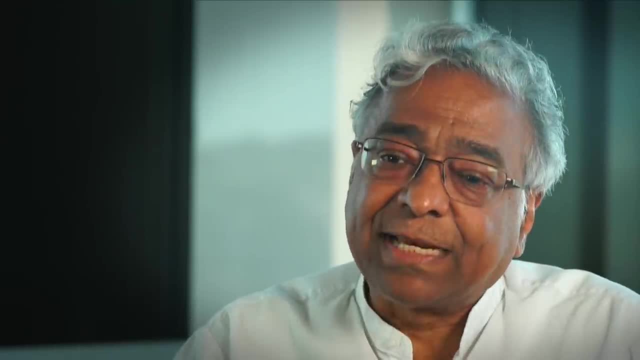 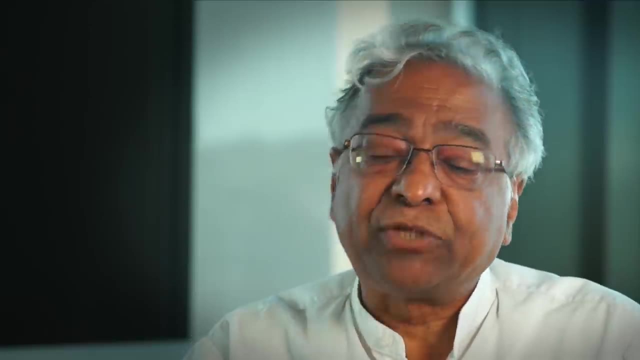 precisely on cosmological models on the classical side, Little bit of quantum side, mostly classical side, And so he really knew the mathematical background very, very much. So he took up this problem and he did some simplification, Simplifying assumptions and found that in fact 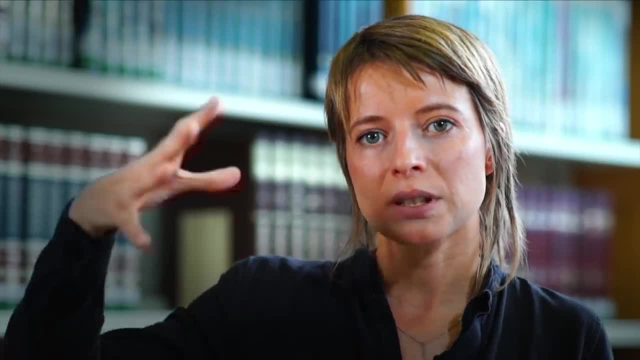 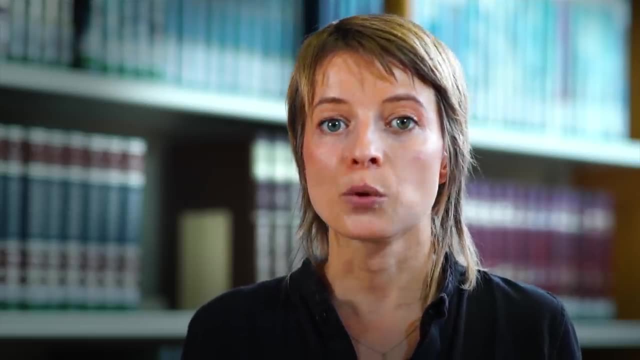 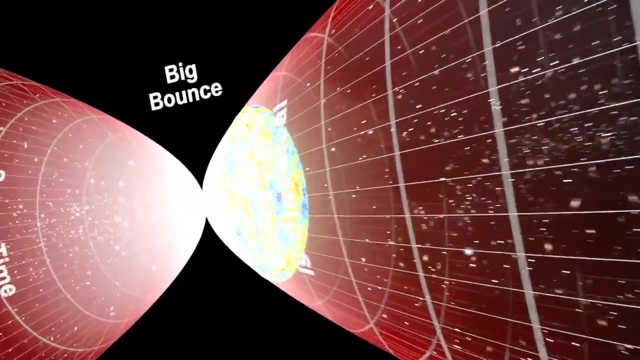 the Big Bang, singularity was resolved. So the current expanding phase of our universe is in fact just the continuation of a previous phase in which there is a contraction and then an expansion. As we evolve back in time, one reaches a point of maximum density. 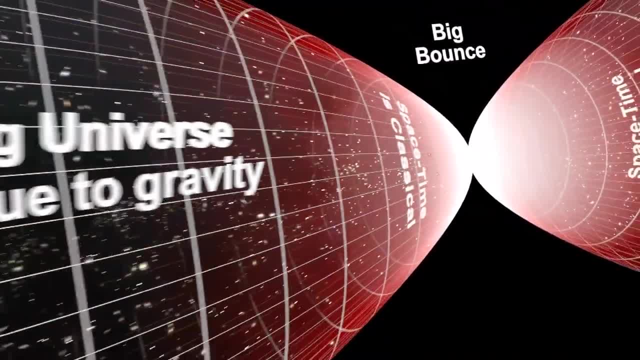 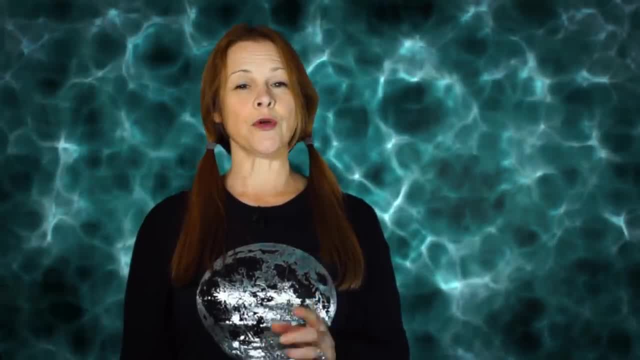 So this is what we call a bounce: The universe collapses and bounces back. One of the problems of Boyle's work was that the bounce could occur when the density was far too low to be realistic By 2006,. Astrakhar, Pavlovsky and Singh. 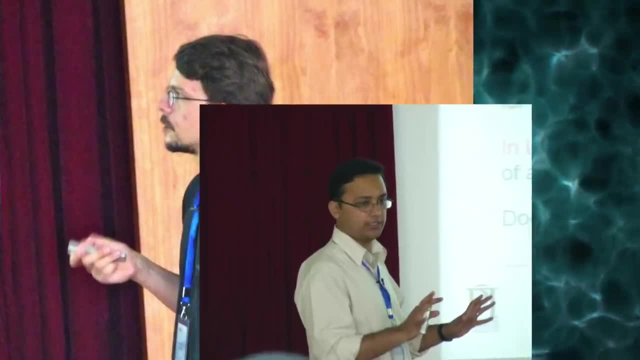 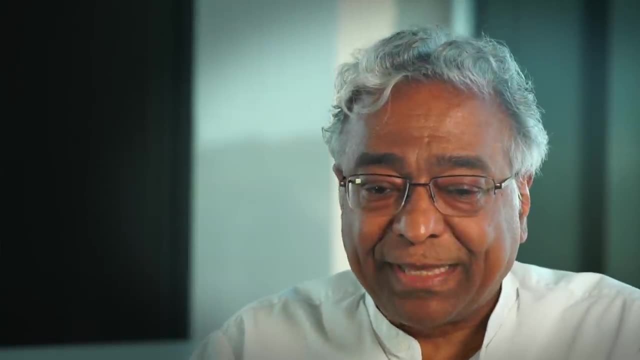 made a key breakthrough, showing the bounce only occurs when the universe is close to the Planck density. I thought it was too good to be true, so to say. I mean that it is something that is, And I wanted to be very, very careful. 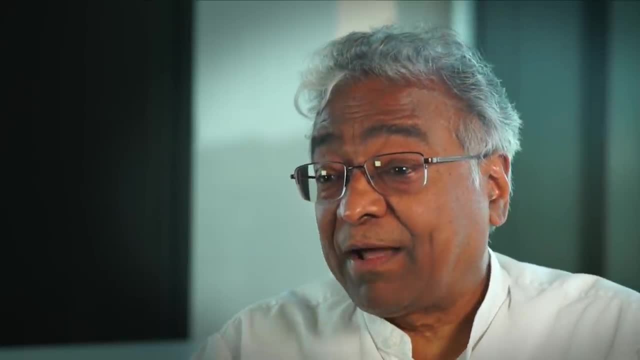 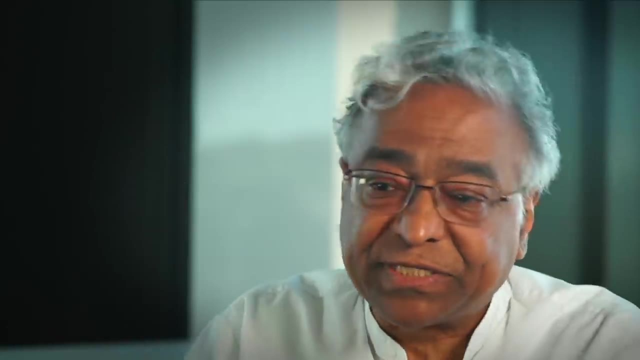 So the question was whether this was an artifact of our specific choices, For example the choice of state we made. So we varied states, still keeping them peaked, but we changed states, We changed various things in the computational models. I kept asking a thousand questions. 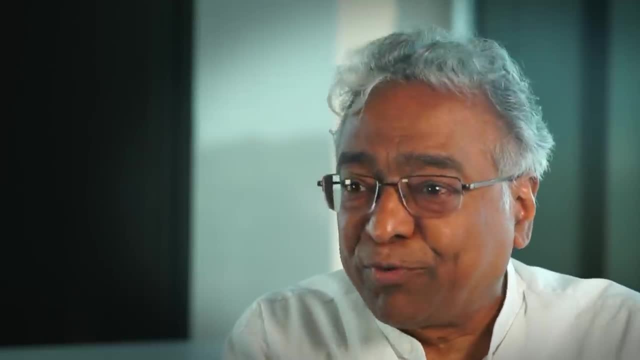 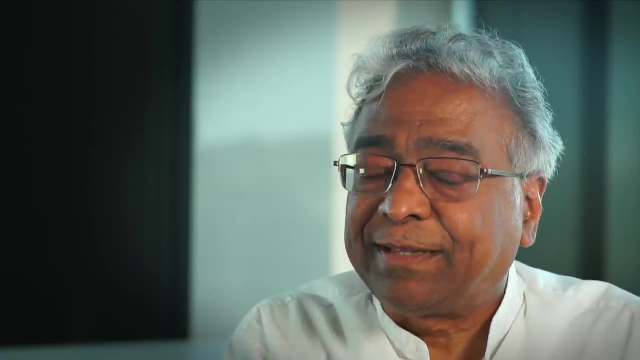 to the postdocs who were doing the simulations to make sure that something, nothing was slipping us. But the prediction remained robust in all these things And after about eight months of these checks and re-checks, we decided that we should write it up. 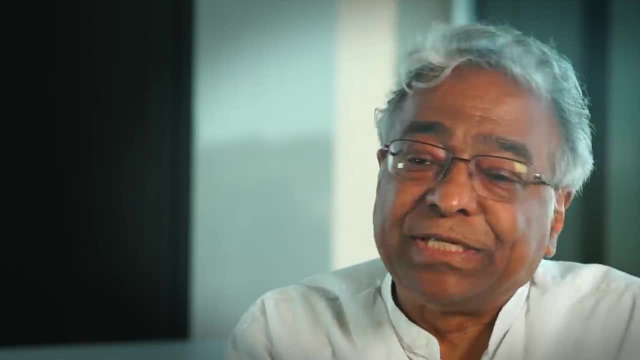 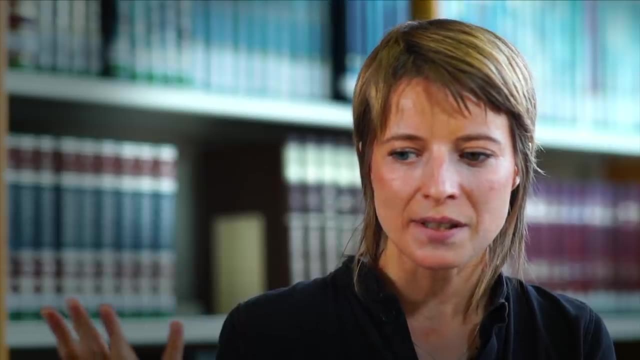 and publish it, And that's what we did. If there is a bounce, if there is a contracting phase, how can we check if there is a bounce or if there is a contraction phase? How can we check if there is a bounce or if there is? 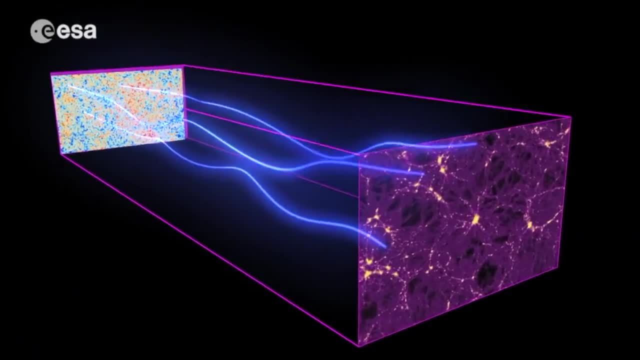 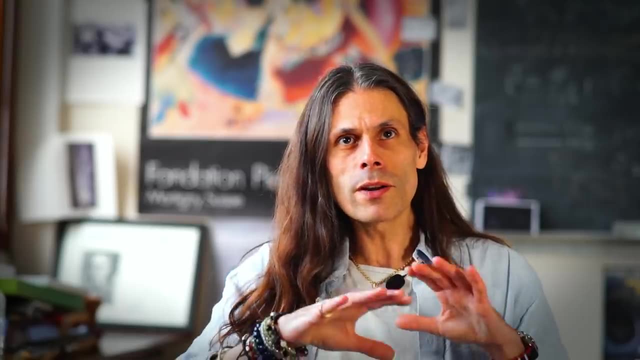 a contraction phase. How can we check this? We expect this to leave a signature in the CMB, in the Cosmic Microwave Background At the big bounce. you are in a very strange state. The universe still has some curvature and therefore your initial conditions. 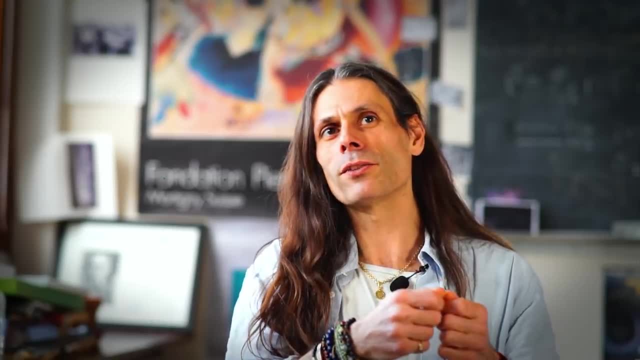 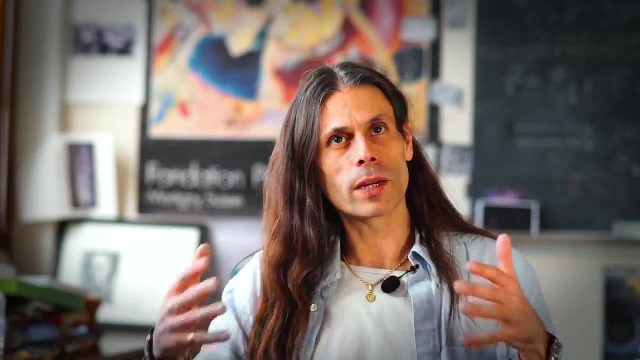 for perturbations are not the same as in the usual model And this might change the spectrum, that is, the shape of the perturbations, and this could be seen in the future experiments devoted to CMB. But observation is the most important part of our research. 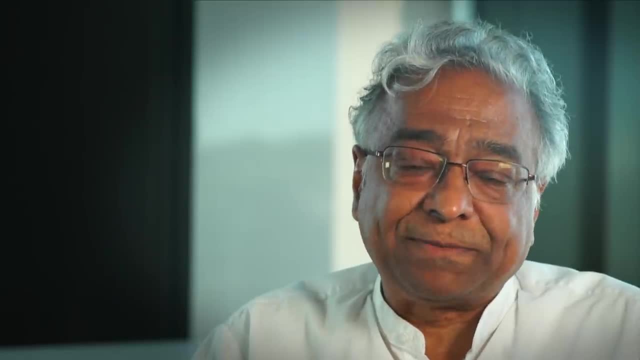 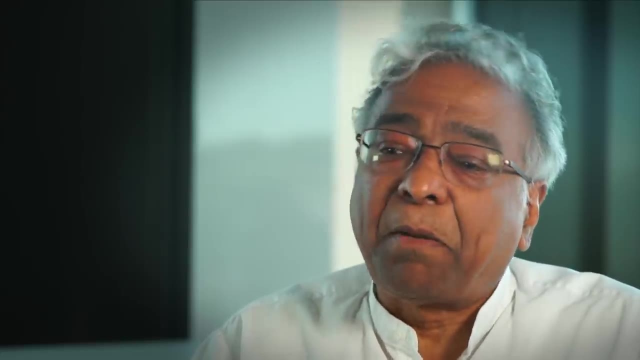 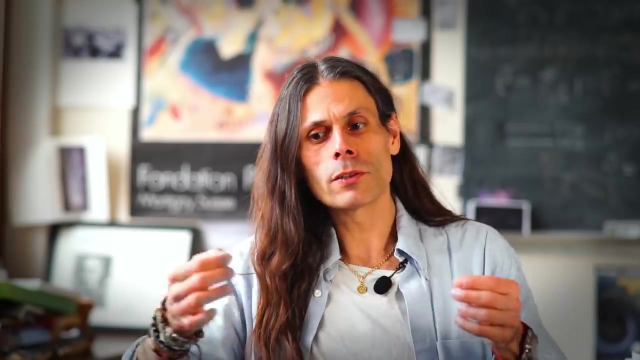 It is the most important part of our research because the perturbations have certain anomalies. The standard inflation predicts what is called a power spectrum, how much energy there is per unit frequency. The power spectrum tells you how much power you have in the fluctuations. 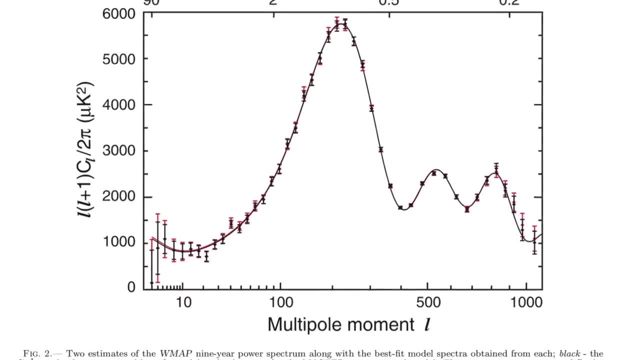 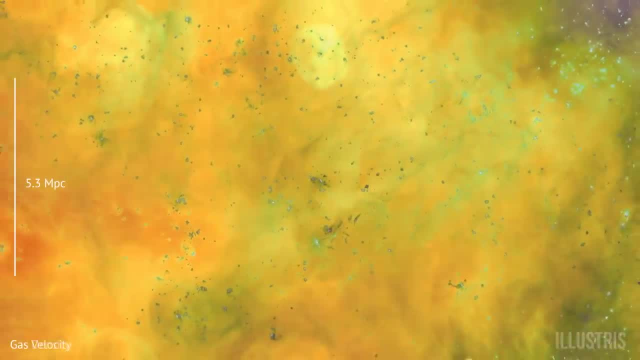 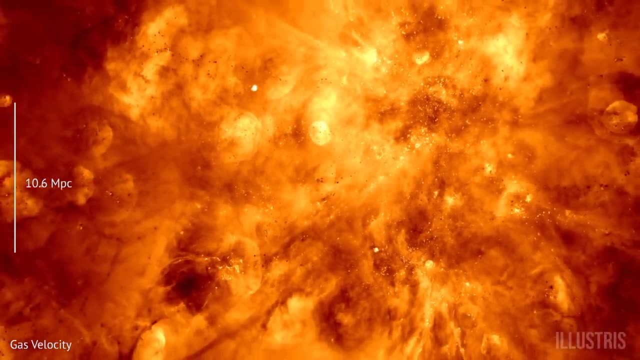 as a function of the L-multipole, which is the inverse of the considered length scale. So, intuitively speaking, big L, large L means small scales and small values of L means small L. so if you have a power suppression or excess at small L value, 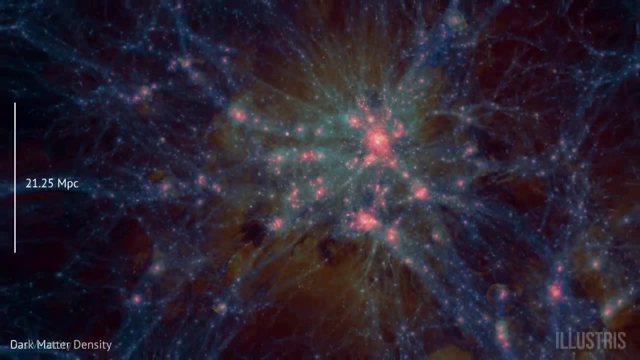 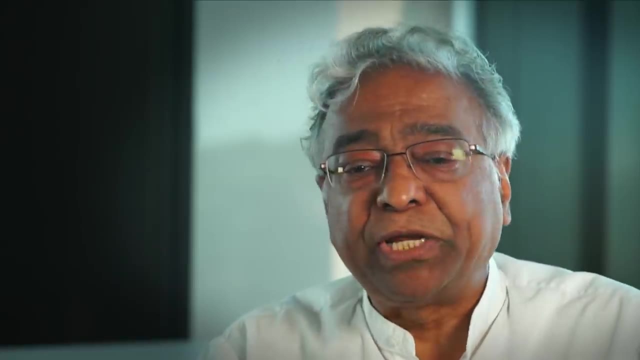 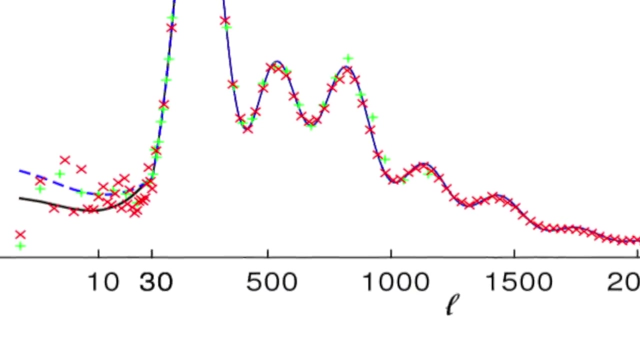 it means that you have a power suppression or excess for very huge distances in the universe. This power spectrum agrees with the standard inflationary predictions for suitable potentials, such as the one that was put forward by Starobinsky, for example, very well at small angular scales. 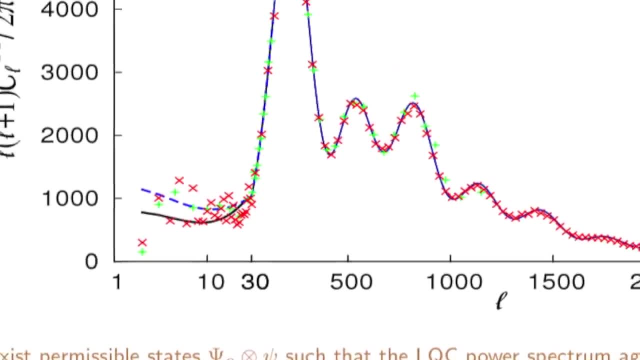 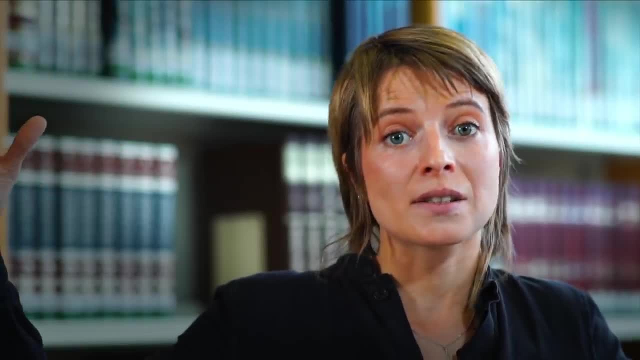 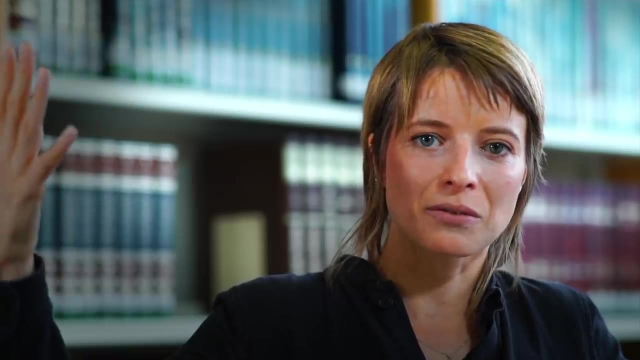 but at the largest angular scales it does not, Because these effects correspond to the largest scale in the sky. these are also the ones on which we have the most uncertainty, So there is a competing effect between the uncertainty coming from the observations and the effect that we are predicting. 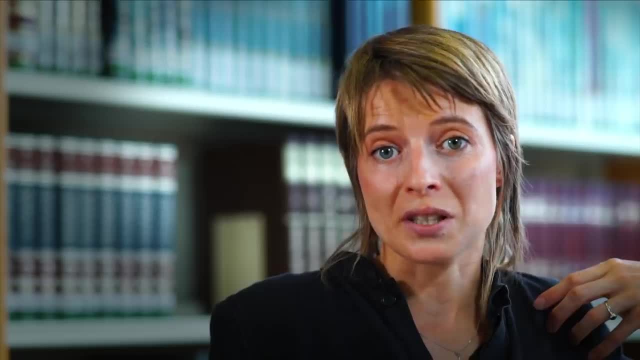 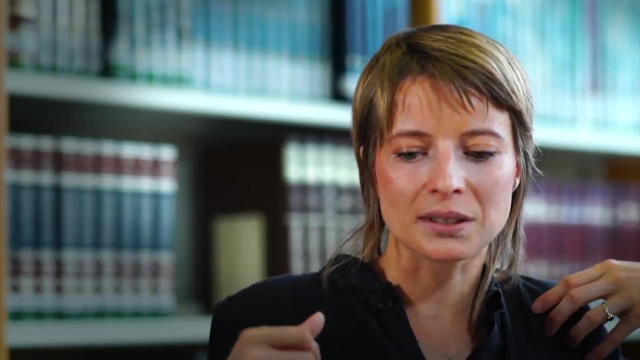 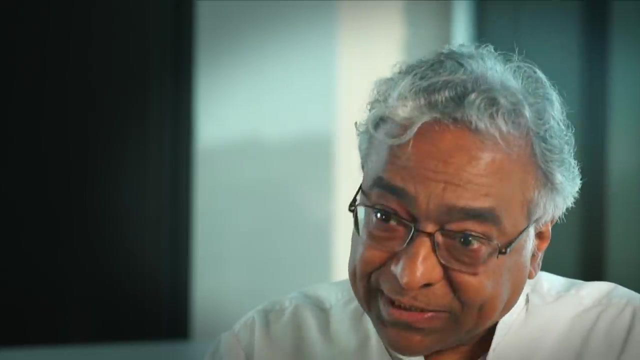 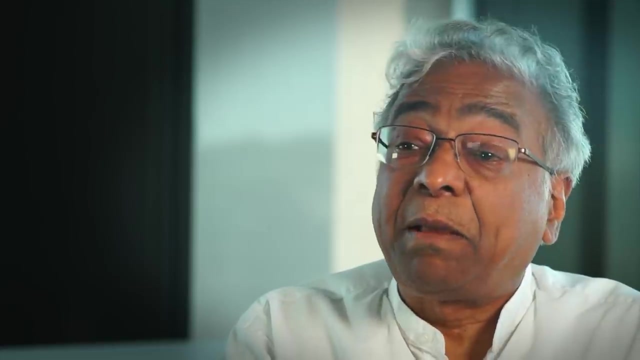 So this makes the research particularly hard. But predictions are there. maybe with future observations we will be able to look at the details, And the happy situation is that loop quantum cosmology has some predictions at low L's. these are compatible with the power suppression, for example. 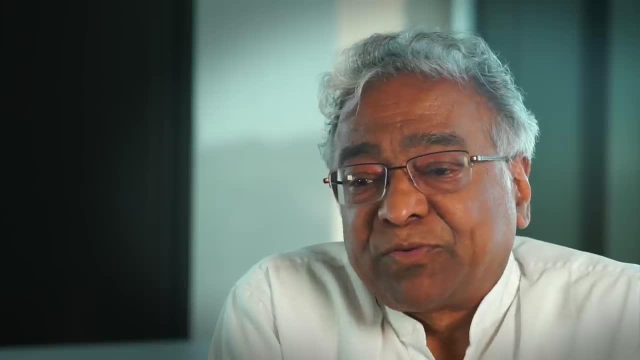 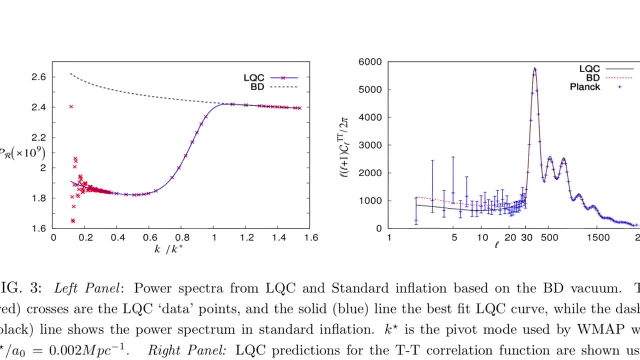 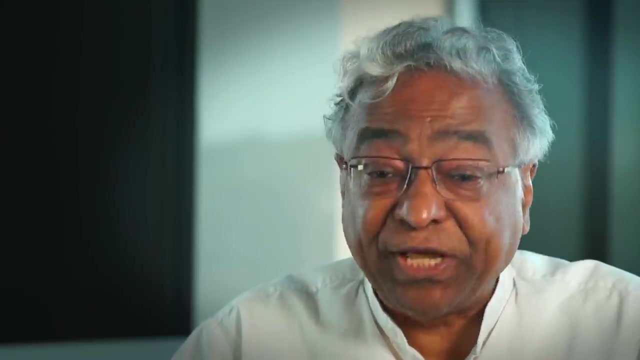 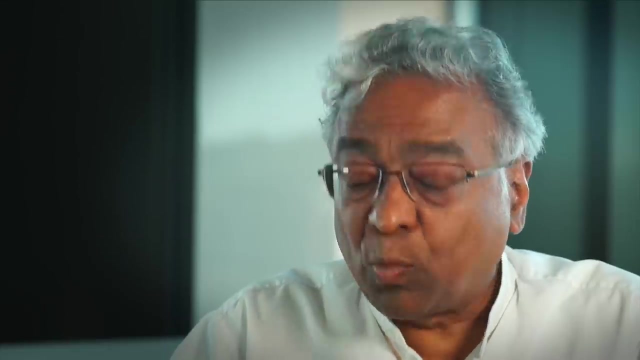 of observations, but we also have predictions for other observables, which is called the electric electric polarization correlation function, electric polarization and temperature correlation functions. If, in fact, observations have predictions, then we will re-examine what is happening. What went into this prediction is two things. 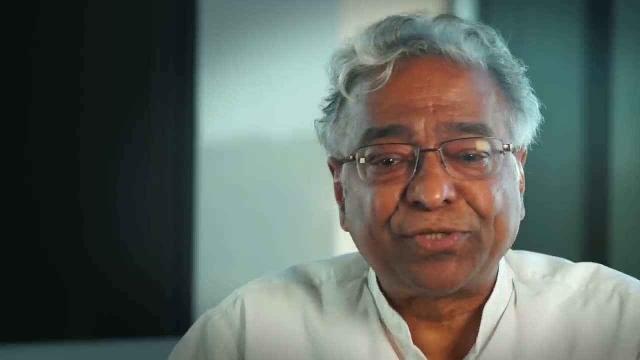 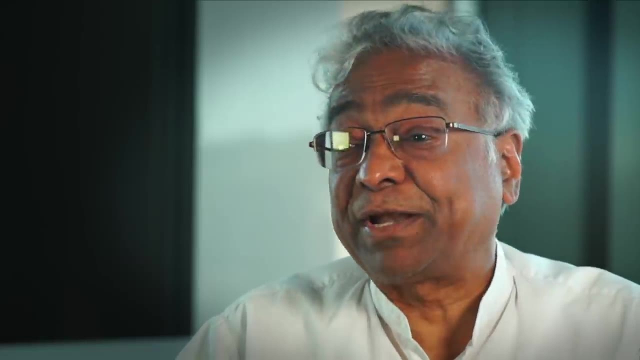 one is, of course, the basics of loop quantum cosmology, and second is initial conditions, And to me, of course, the most fragile things are initial conditions, and so one would have to go back and see: you know, are there some better initial conditions? To me, these are: 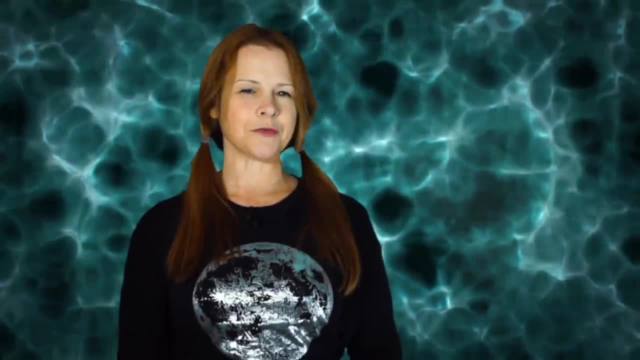 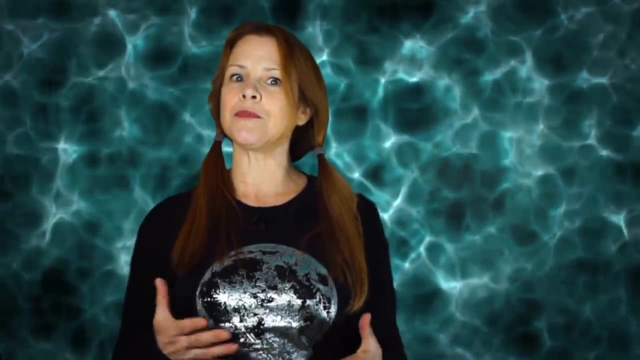 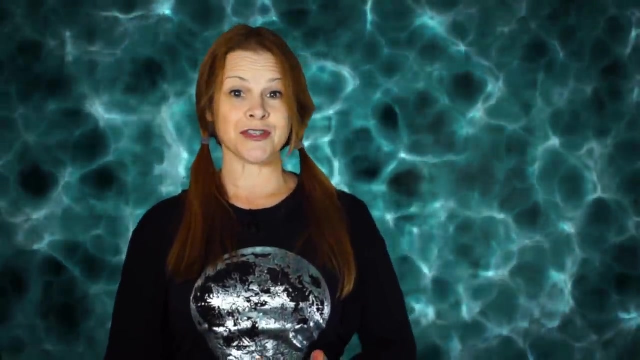 very well motivated in some fundamental aspects, but of course they are rather far removed from experiments. It's exciting that loop quantum cosmology has provided a concrete bridge between fundamental theory and observations. Contributions from several young researchers, especially Aguiu, Nelson and Gout, have been 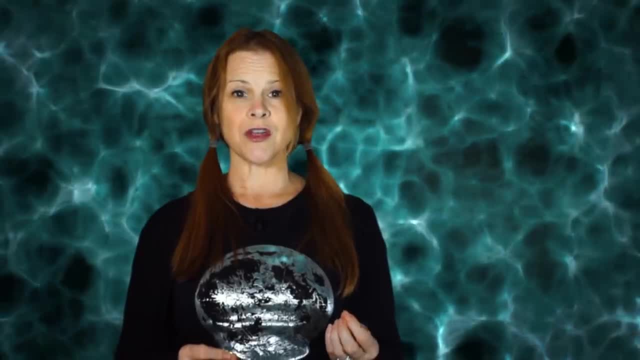 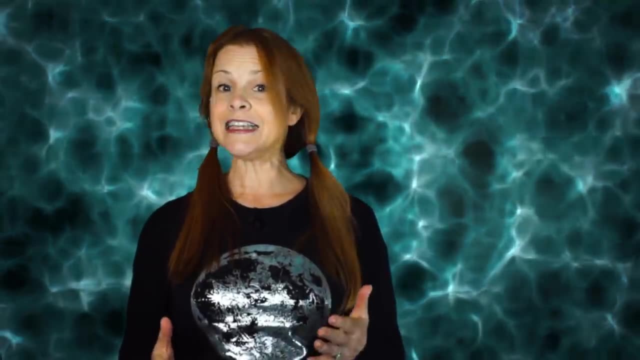 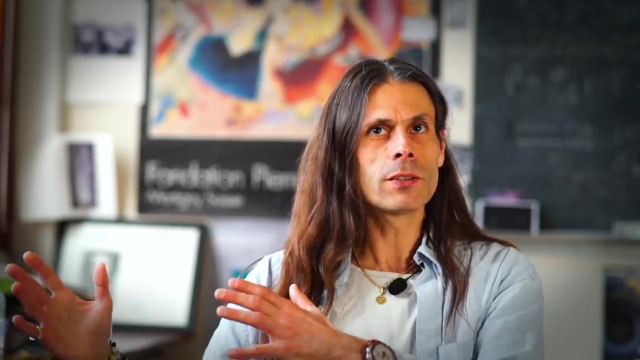 vital in this process. In addition, younger researchers are also pursuing other directions and although these are not yet fully formed and therefore speculative, they lead to a very complex theory. In general relativity, we can test the assumptions because we compare the theory with the observations in a regime. 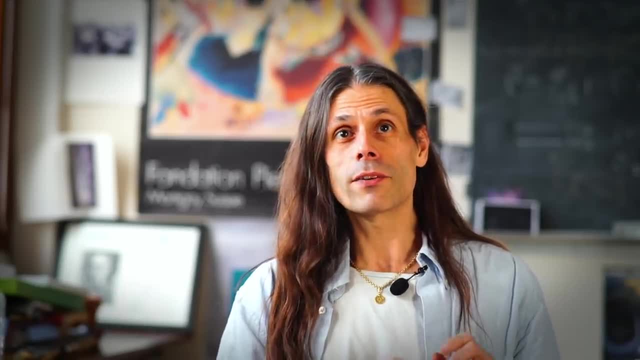 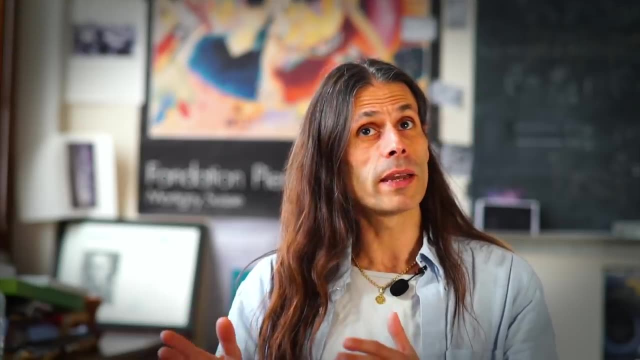 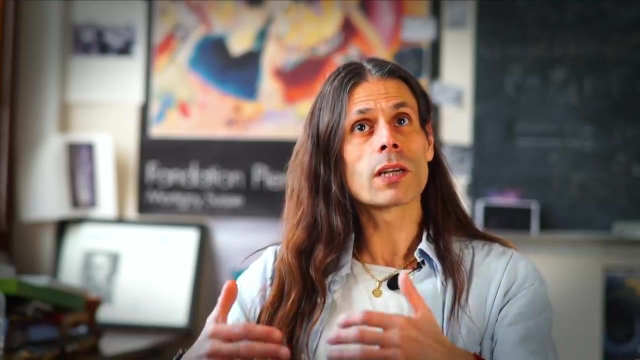 where we know how to test it In quantum gravity. we cannot just compare with the real world in the regime where the theory is useful. Therefore, you have to guess what are the correct assumptions, and at this point nobody knows which assumptions are legitimate and which are not. 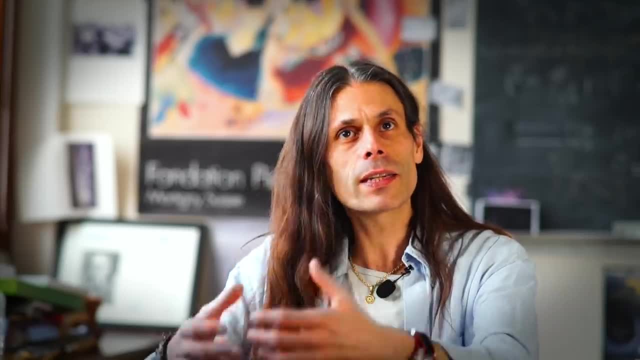 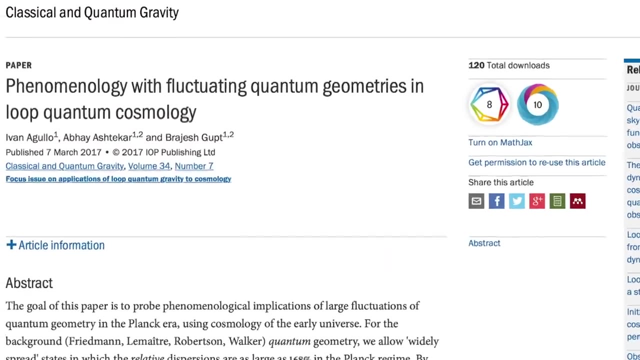 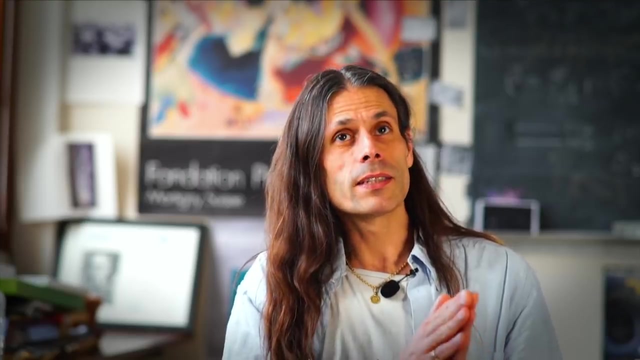 So we have the same mother theory, but we don't have the same effective theory to describe the universe. One path has been followed by H T Carr and his colleagues. I follow another path and in this specific framework then we find a disappearance of time. 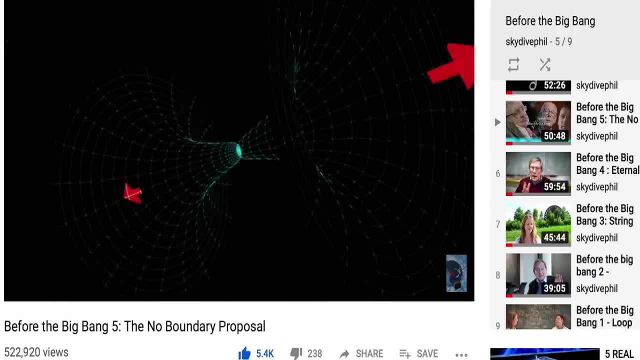 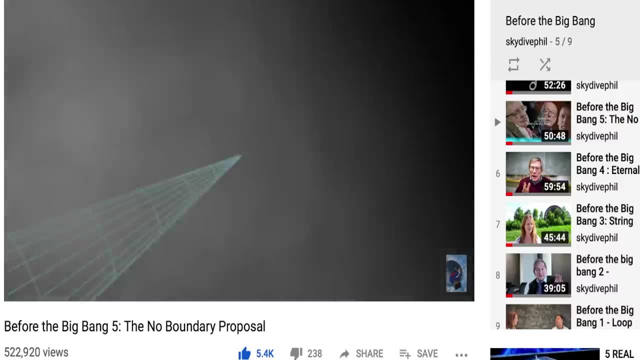 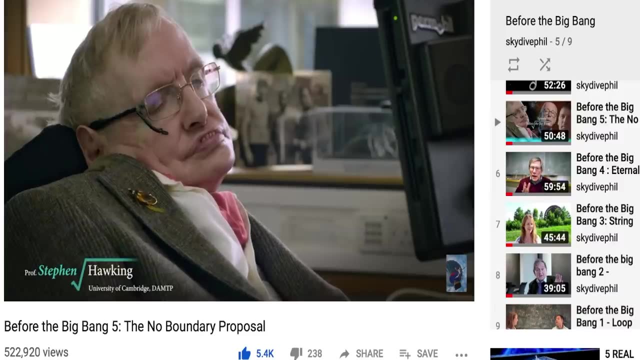 We cannot know if this is real, but it is extremely exciting because it has been postulated in the past, for example, that there is a beginning of the universe, which is often associated with a beginning of the universe. But, as we saw in the film, there is a real. 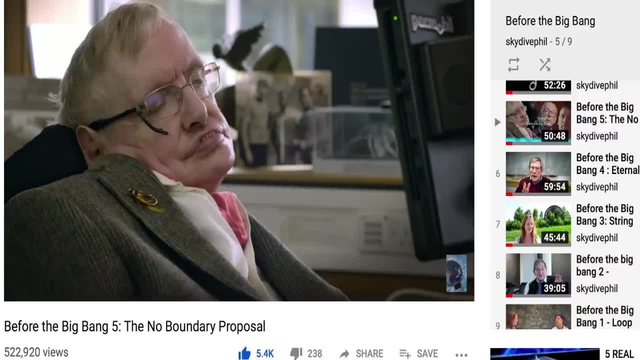 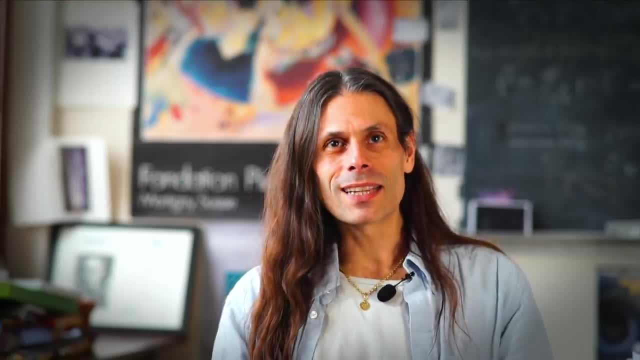 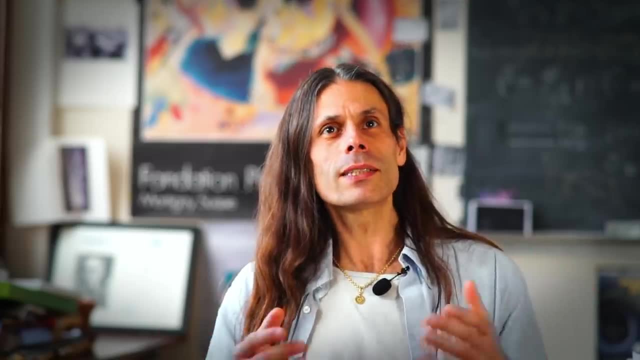 and imaginary time component. The beginning takes place in imaginary time, whereas in real time, like in loop quantum cosmology, there is a bounce. So I know that Abai is not a big fan of this idea of disappearance of time and appearance of four-dimensional space. 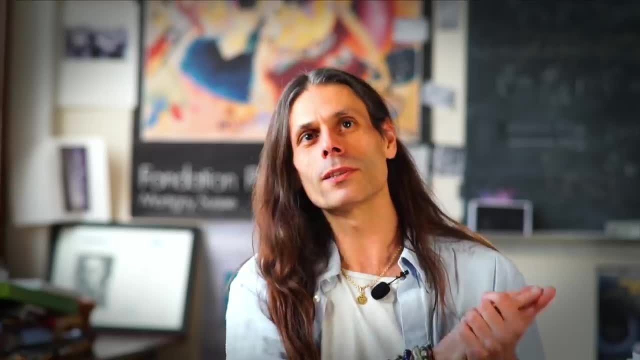 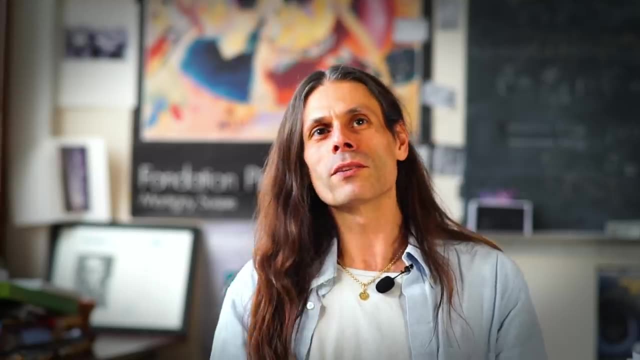 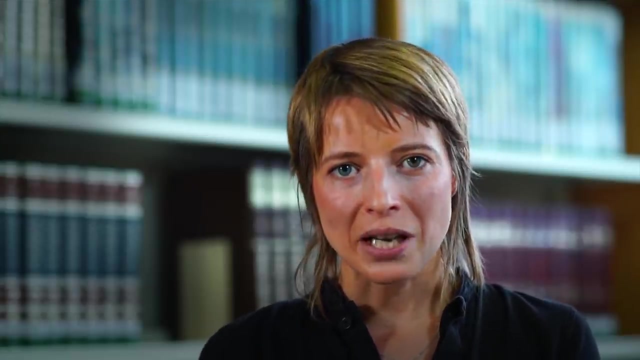 but I am sure this is not demonstrated and this is not a very hard consequence of loop quantum gravity, but it is something that would be so fascinating with huge experimental consequences. so in my opinion it should be considered and calculation should be continued. So it doesn't. matter how you do it, no singularities can form in the early universe, so there will be no singularities, and so you can't predict the duration of inflation. and you can't predict the duration of inflation because you have a clear prediction thanks to the bounce on the duration. 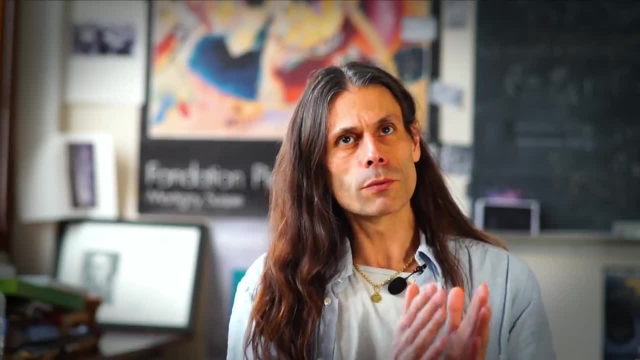 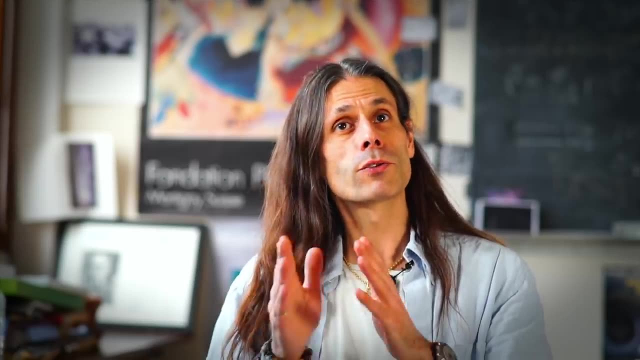 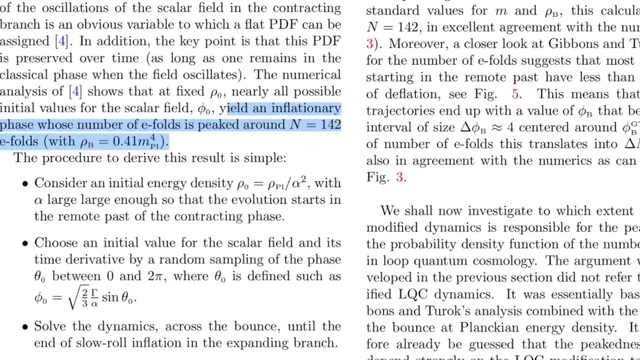 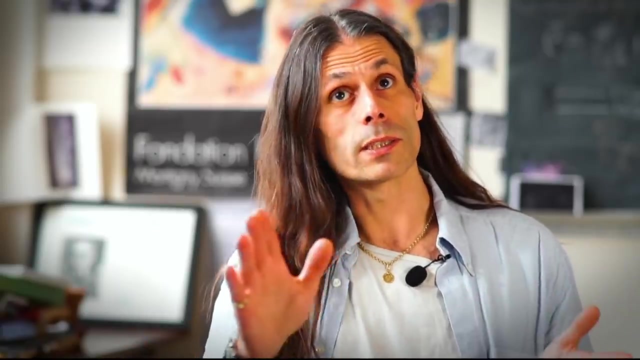 of inflation and this could be experimentally probed. To me this is highly reliable and very interesting because you don't have that in the standard model. From the observational viewpoint, we know that the minimum number of defaults should be around 60, and we end. 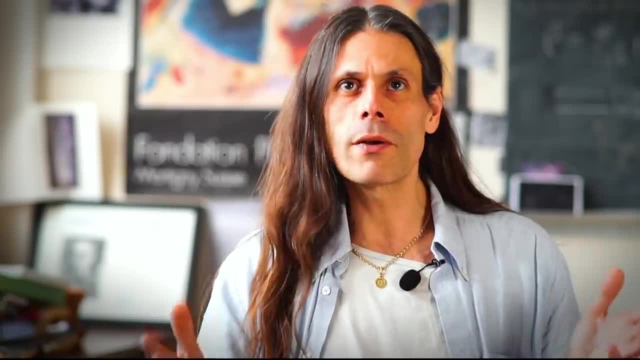 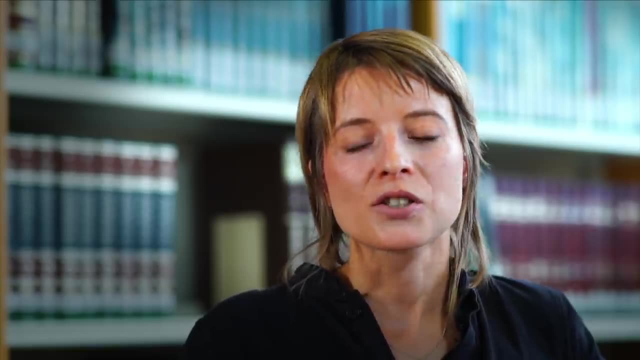 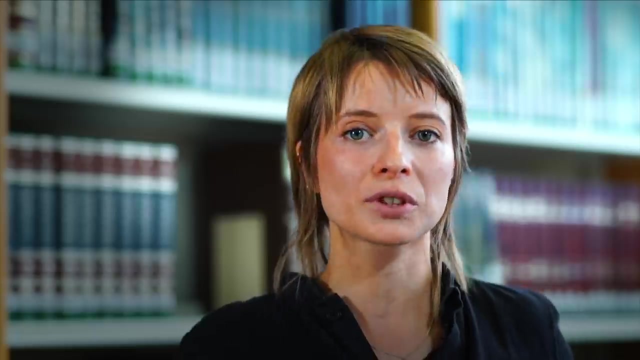 up with a value which is of the order of 100.. 100 is above 60, so this is good. otherwise the model would be excluded. but it is not much above, so this is very good news for testability. There are a lot of experiments. 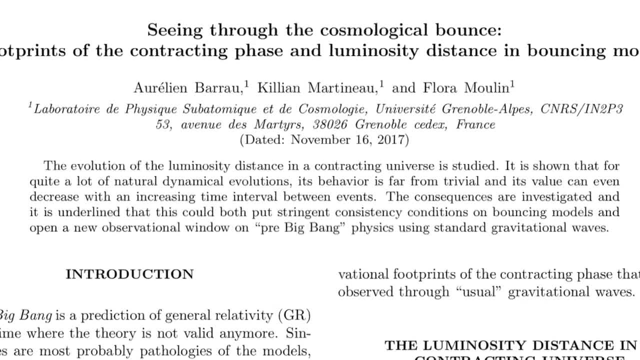 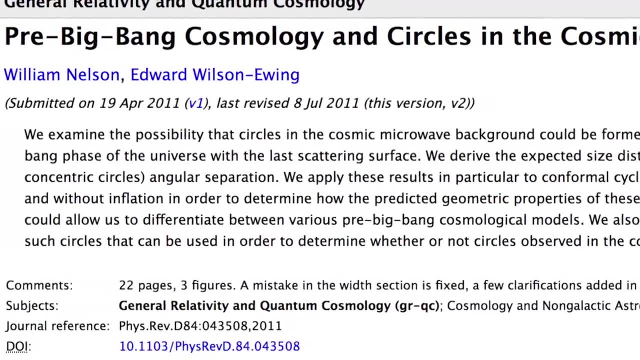 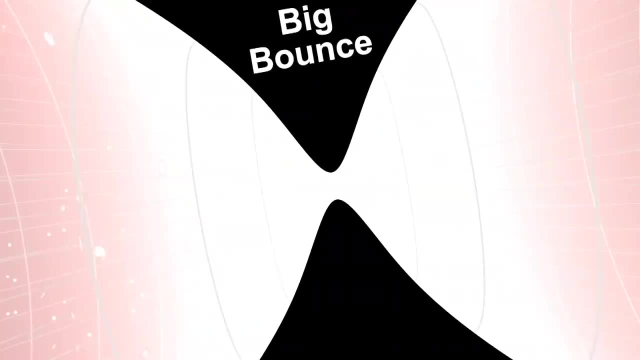 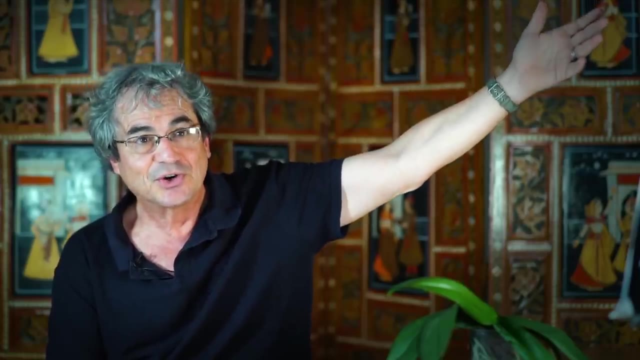 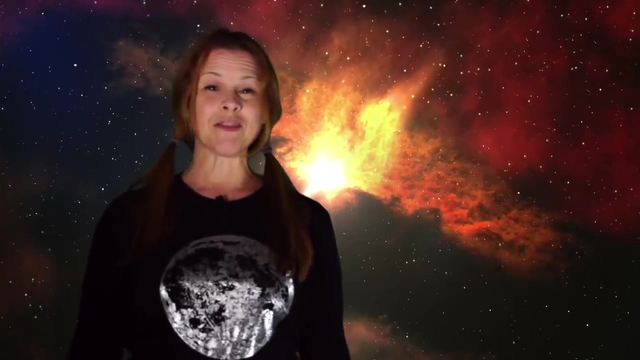 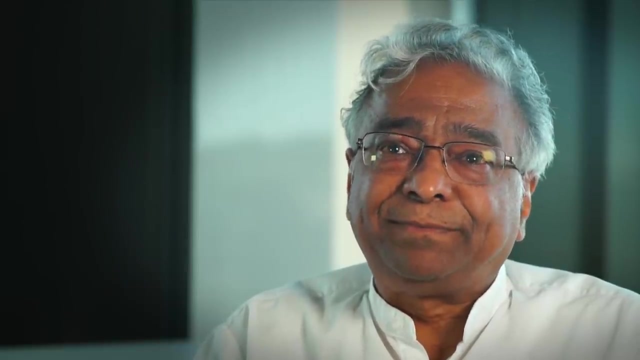 that have been done to predict the duration of inflation, and this is a very interesting experiment because we know that if the universe does not begin at the end of the universe, we would never get to now if the past stretched back for eternity. These arguments to me. 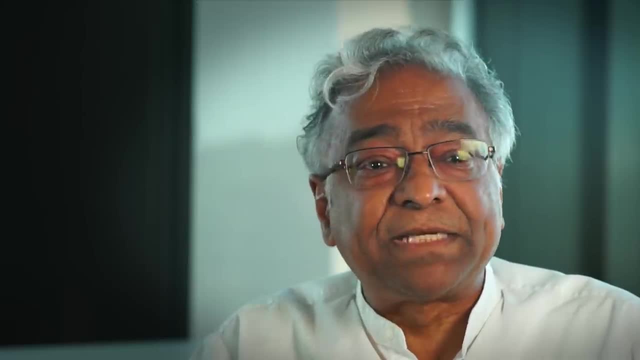 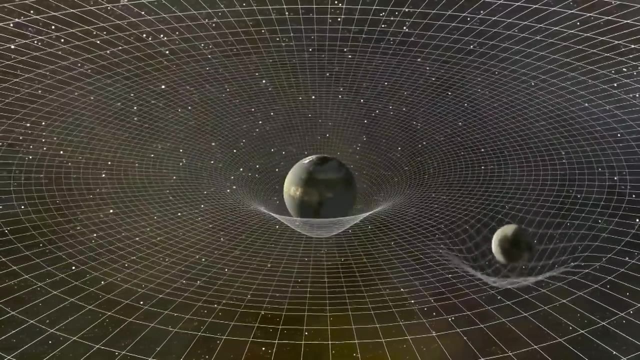 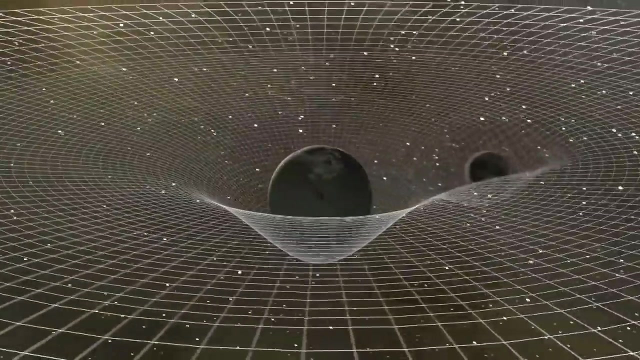 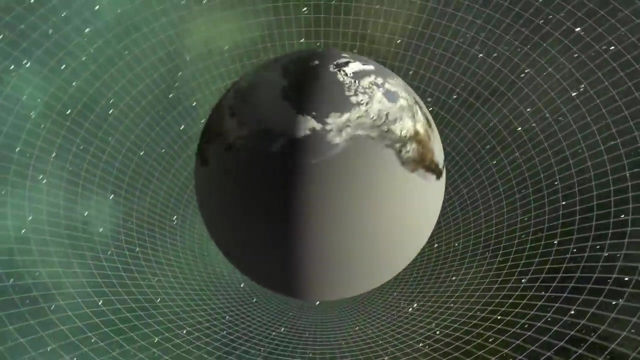 seem a little bit like the arguments that were used by neo-contists in the early days of general relativity to say that one needs space-time, So how could it curve space-time? And very serious philosophers argued this, and we know that this is a 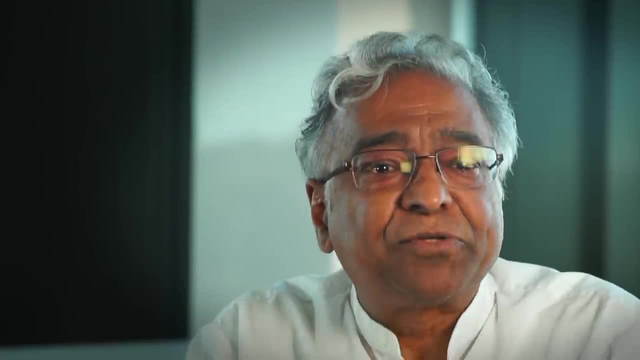 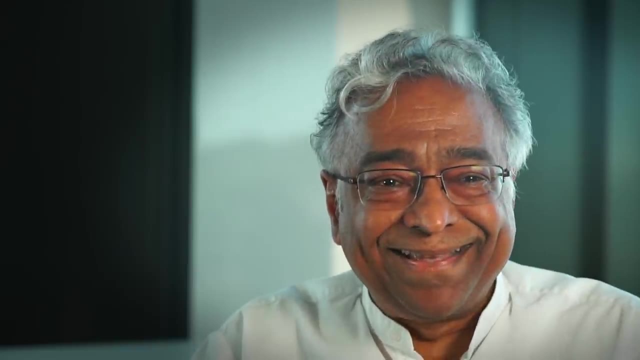 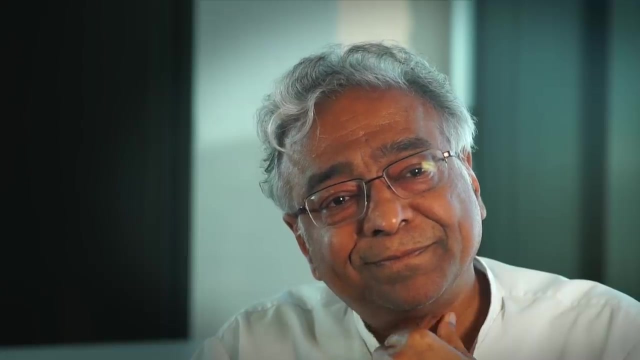 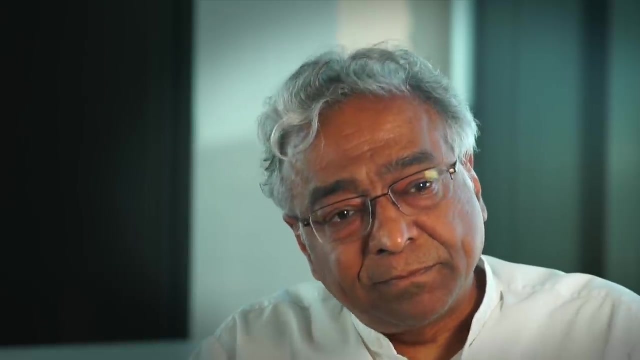 completely vacuous argument. It's not that there is space-time first and then that curves, but everything comes together. So what I've heard expressed is: well, suppose you were to start a race, and I'm going to start my starting gun. I'm. 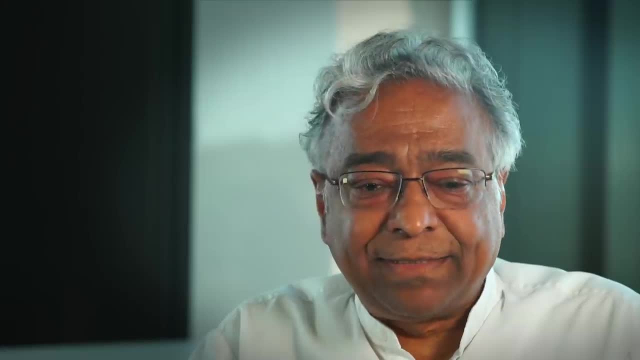 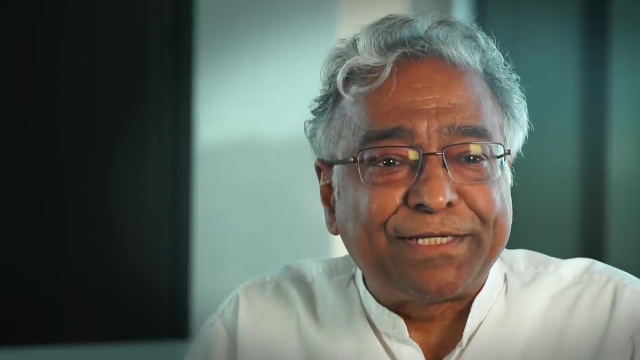 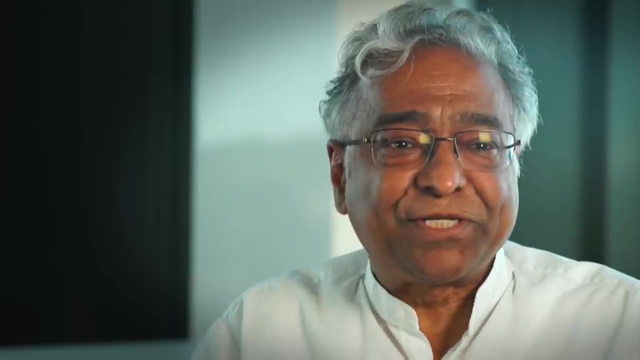 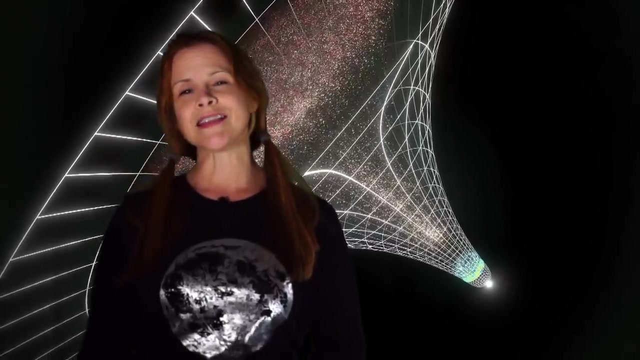 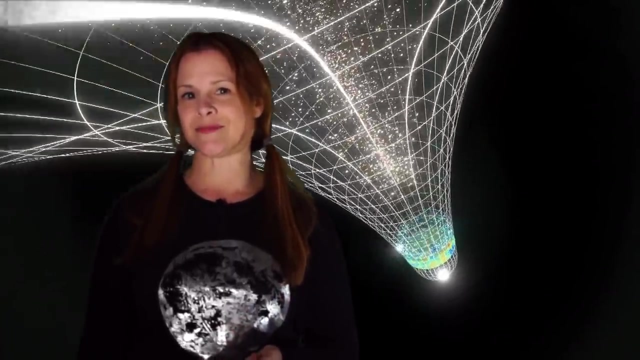 going to wait for an infinite amount of time before I shoot the gun. You just cannot have a finite beginning. So these people will just say that well, I just dismiss it, because I mean the statement is: there is no gun. Another reason for. 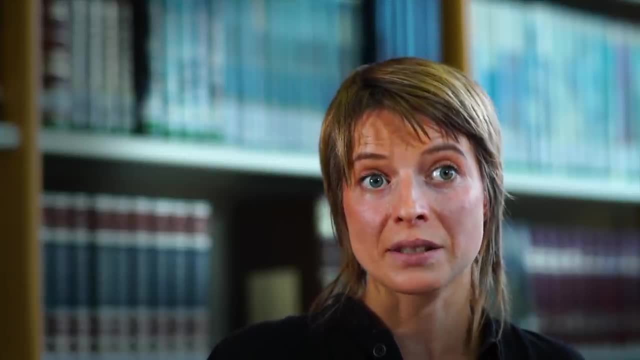 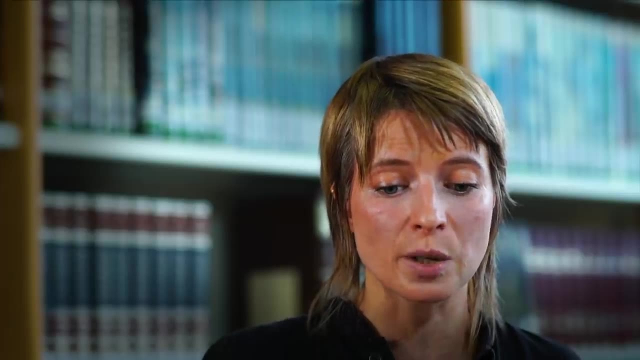 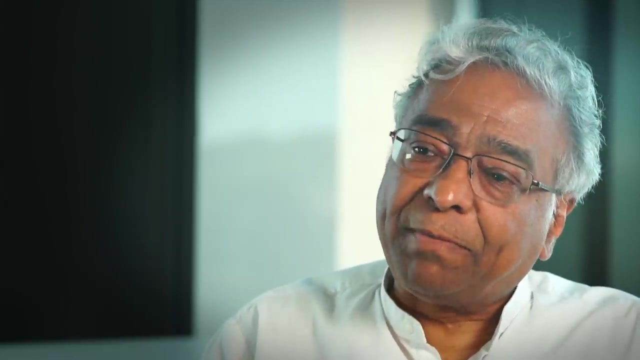 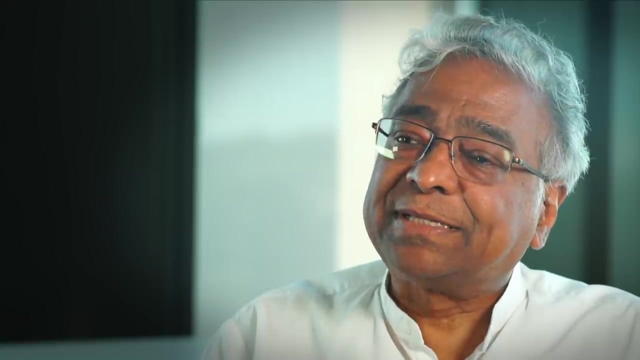 thinking the universe began with the big bang are singularity is one of the hypotheses that you are using to formulate this theorem. There was an initial singularity theorem that was proved quite some time ago by Penrose, Hawking and Garrosh, and. 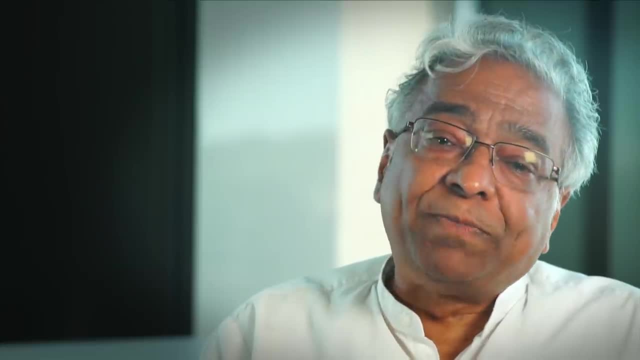 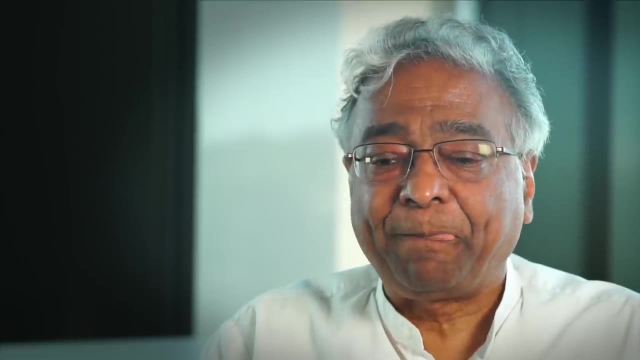 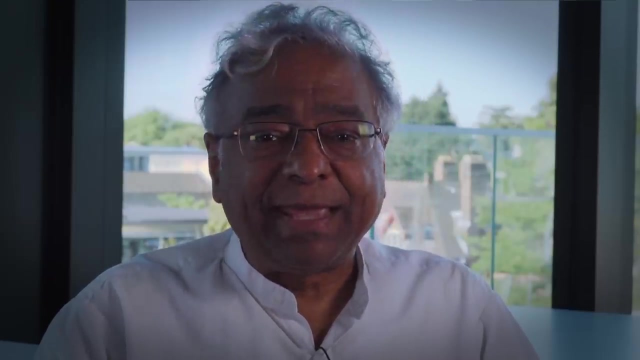 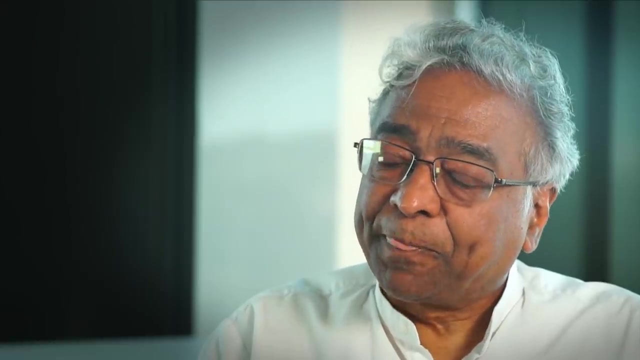 others which made some assumptions about the kind of big bang singularity. But a theorem proved by Borde, Guth and Vilenkin showed that this is not the case. Even if you don't make any restrictions on matter of the type that we 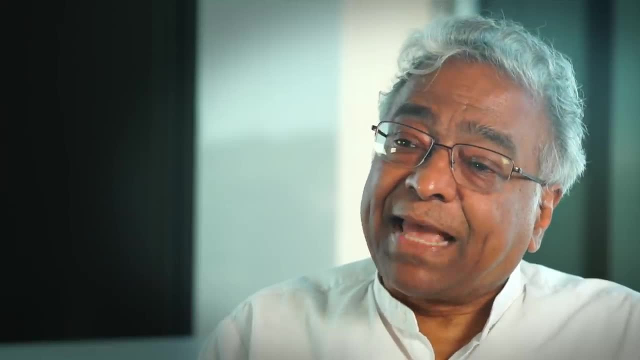 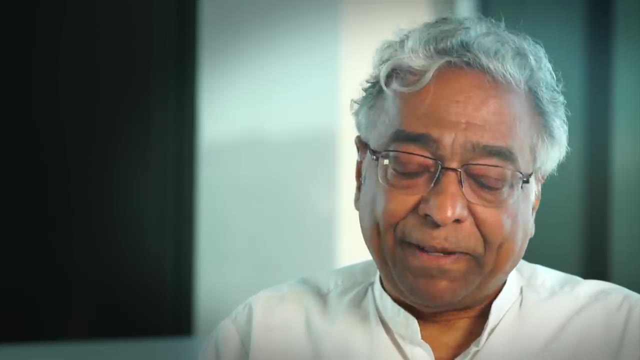 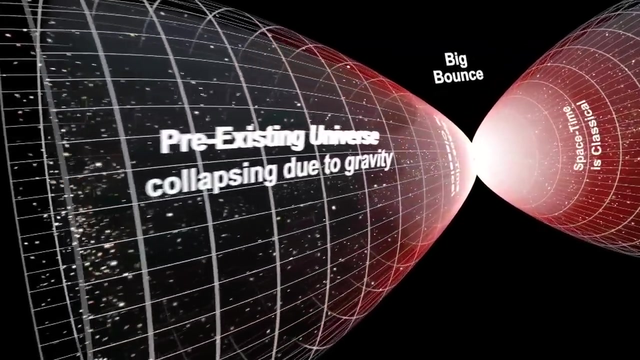 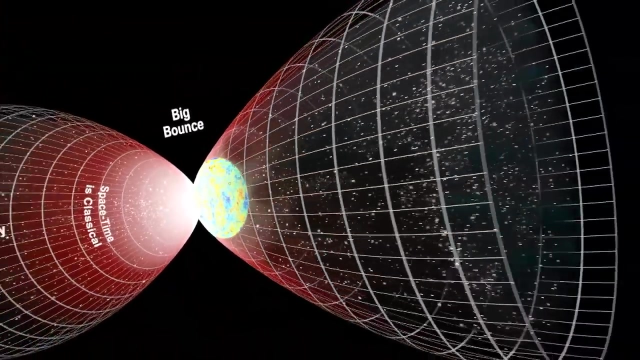 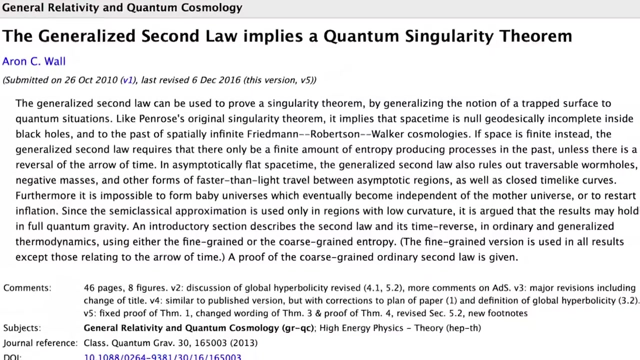 made before, but if you assume that there is inevitable big bang type singularity, Now this conclusion is evaded in new cosmology. Initially the universe is contracting and it expands only after the mouse And therefore the assumptions that they made is violated. 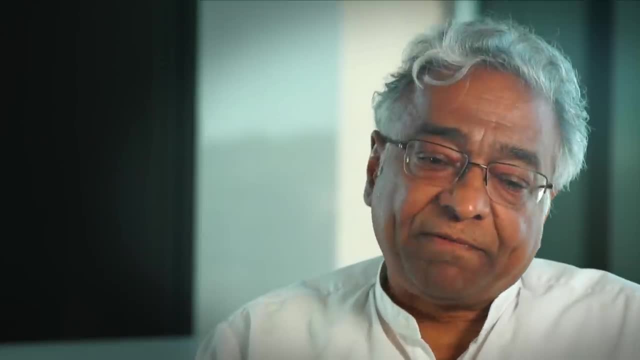 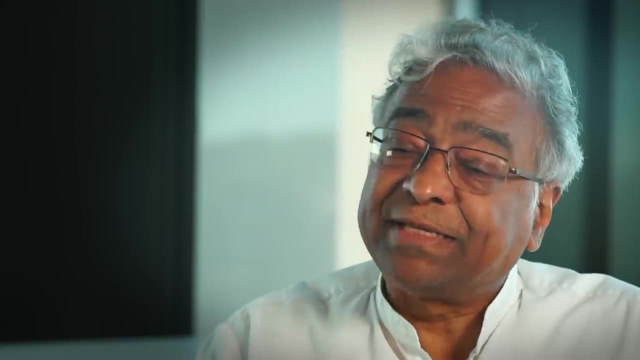 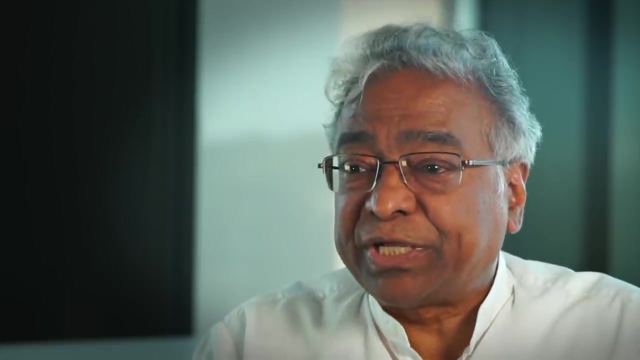 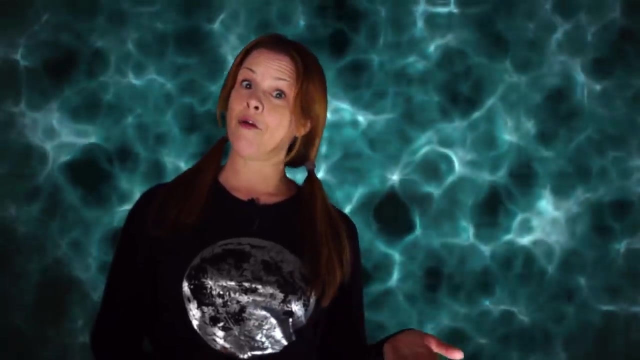 A new singularity theorem of the second law of thermodynamics is really fundamental and should be a fundamental ingredient in this series which determines whether there will be singularity or not, And I don't agree with that. I think that it really is something that would. 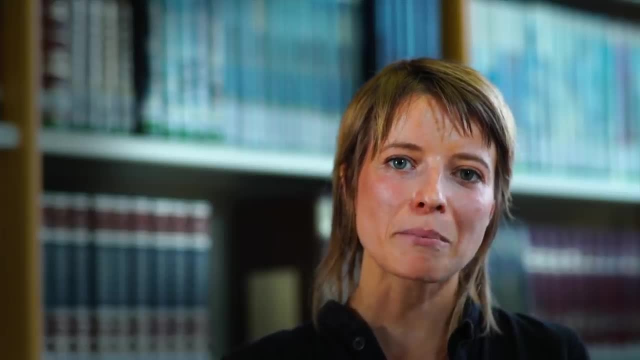 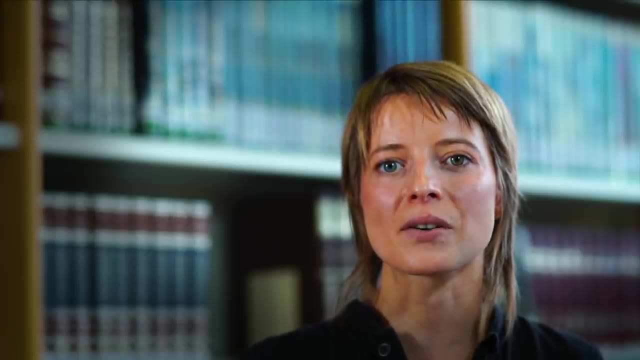 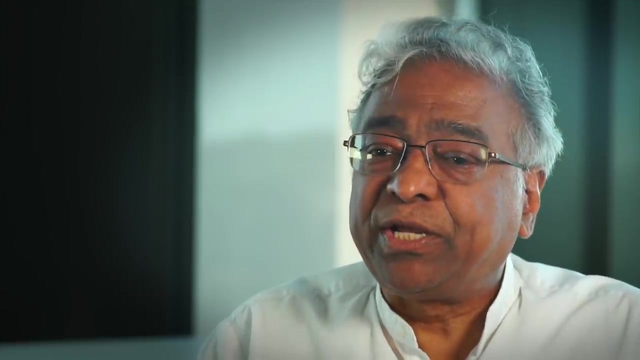 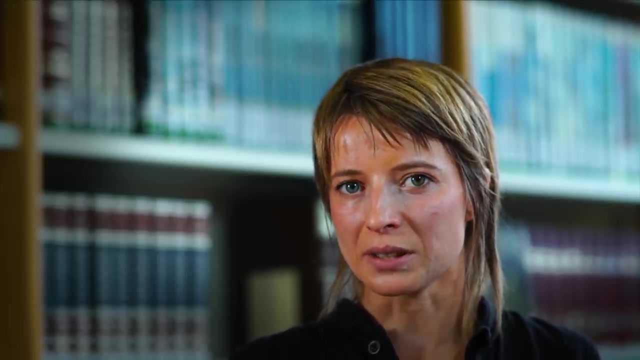 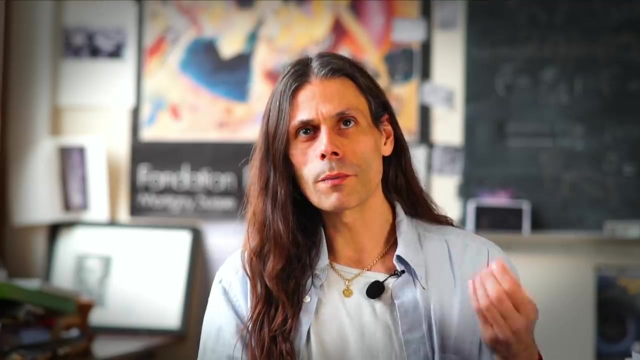 emerge in approximate sense of clarity if we realize the fact that entropy is not an absolute concept. In fact, it's a relative concept. Entropy is really counting the number of microscopic configurations which lead to the same macroscopic configuration. When we look at a system, 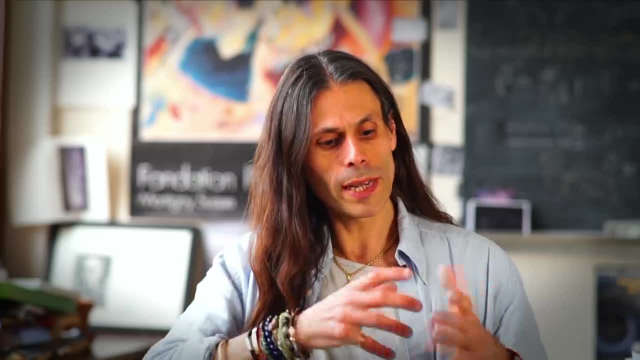 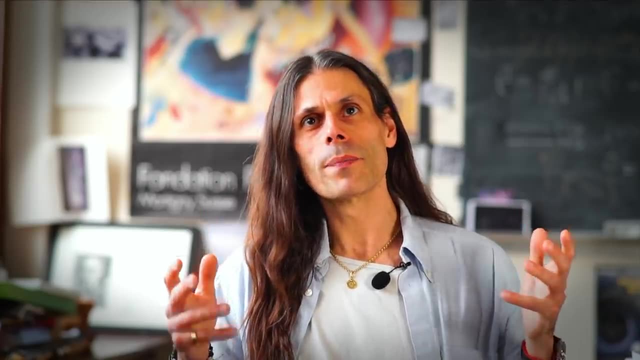 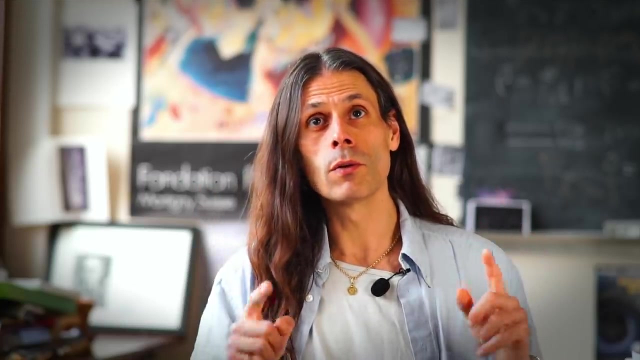 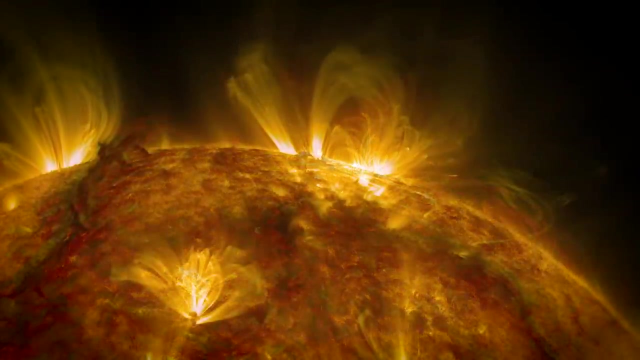 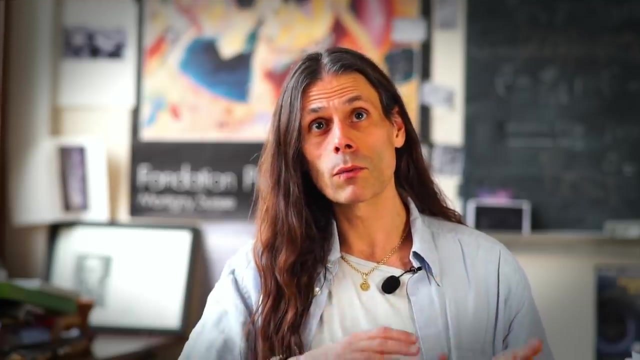 which is not purely objective, but which is somehow related with the way systems interact one with the other. So, clearly stated, it would mean that the entropy of the universe was not low at a big bounce. It means that it appears to be completely subjective, because the way 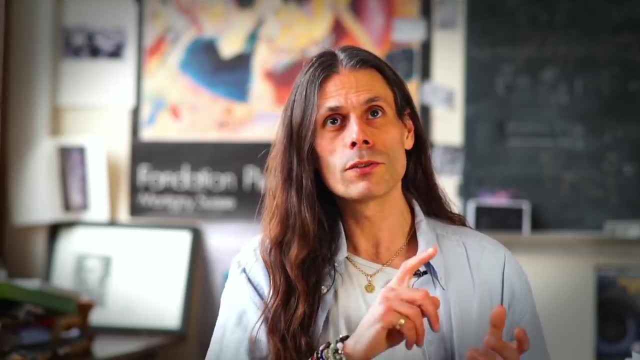 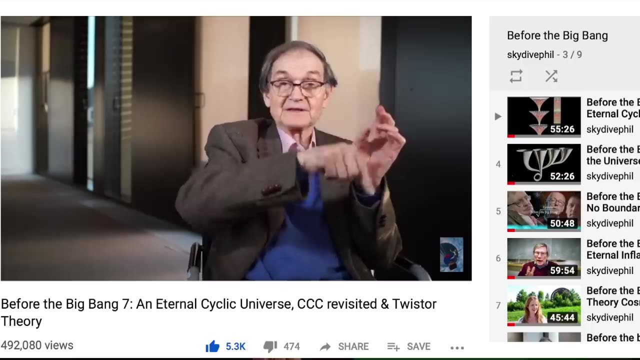 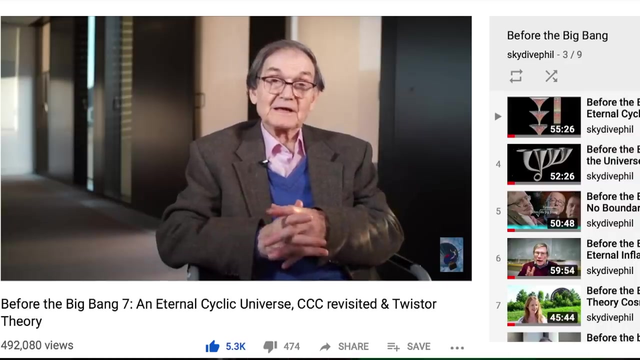 you couple to another system depends on the kind of system you are. In one of our previous films, Sir Roger Penrose proposed that dark matter may be related to the remnants of black holes in the pre-Big Bang universe. Penrose dubbed these remnants Erebons. 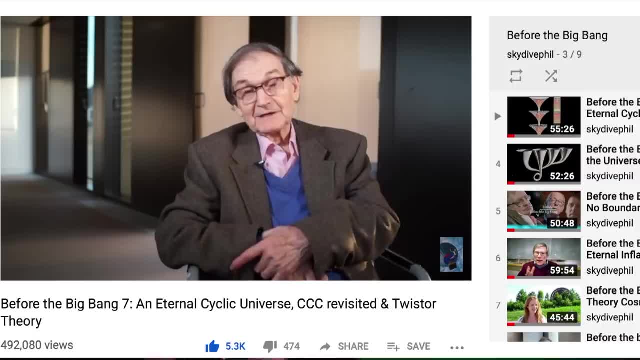 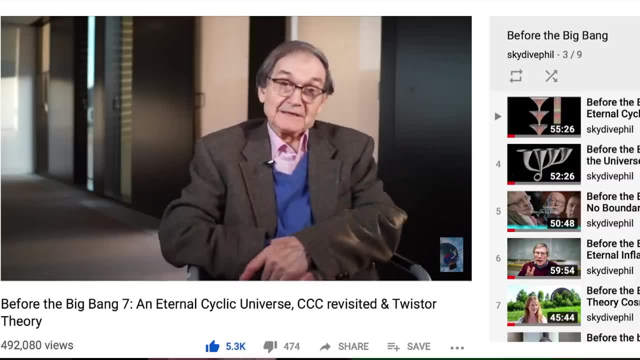 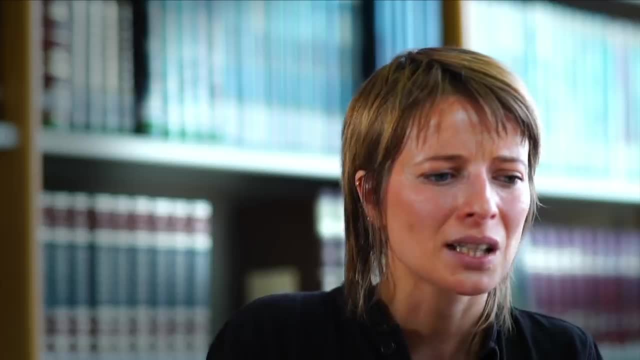 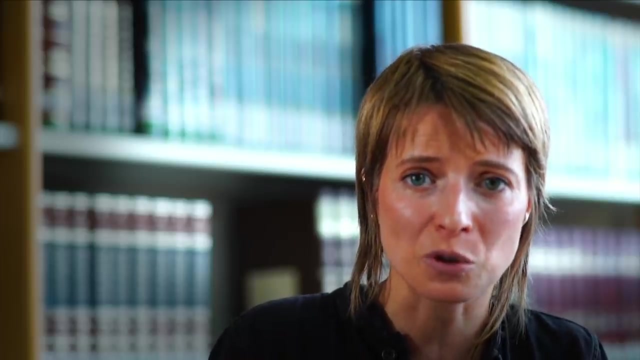 after the primordial universe. Such black holes may have a large volume, even though they have a small area. This can be used to explain the low entropy condition at the bounce. If I look from the outside, the universe seems to be so small and there. 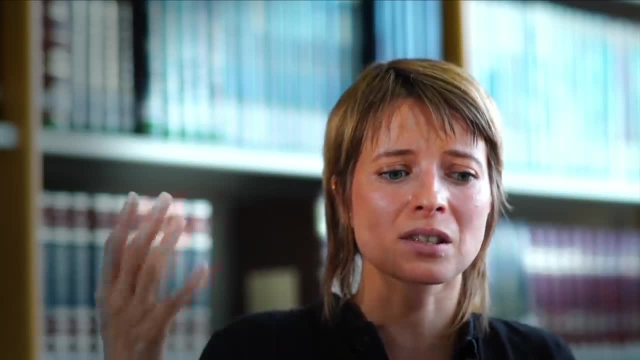 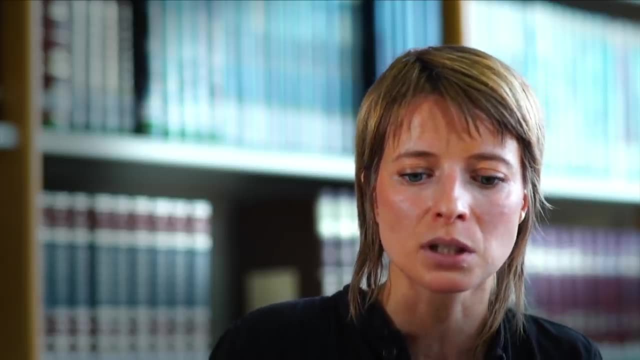 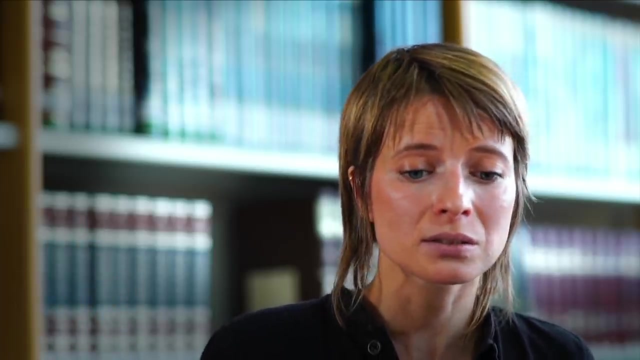 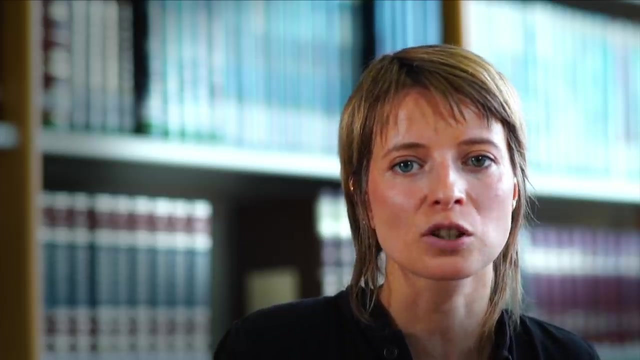 are not many black holes in the universe, But if now I can describe the universe as a wall, including also the interior of these Erebons, of these black holes, then there is a lot of space, there is a lot of way in which. 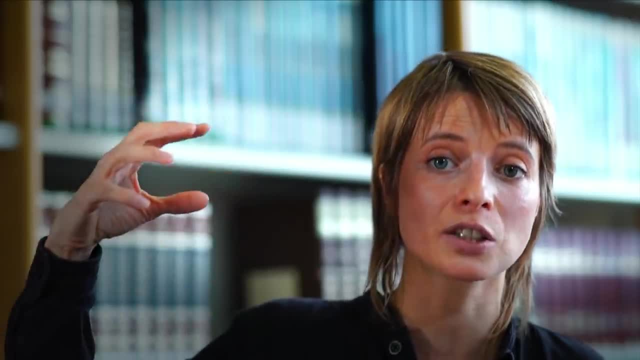 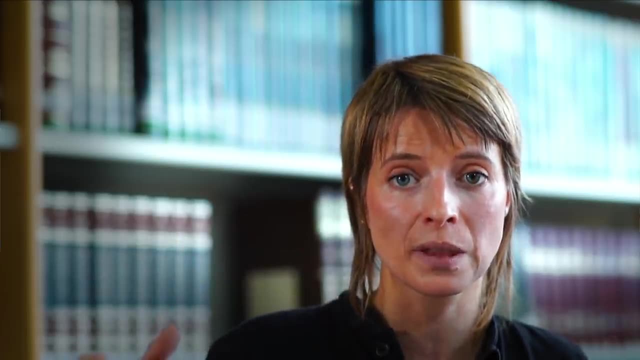 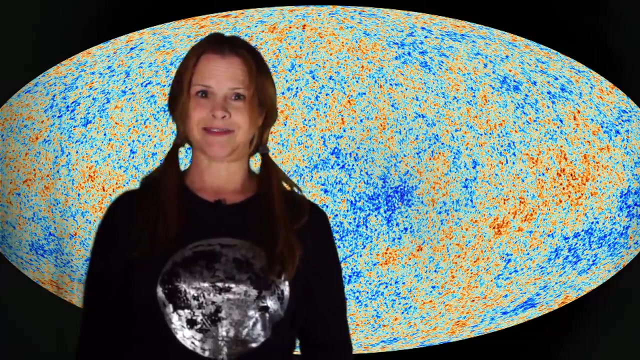 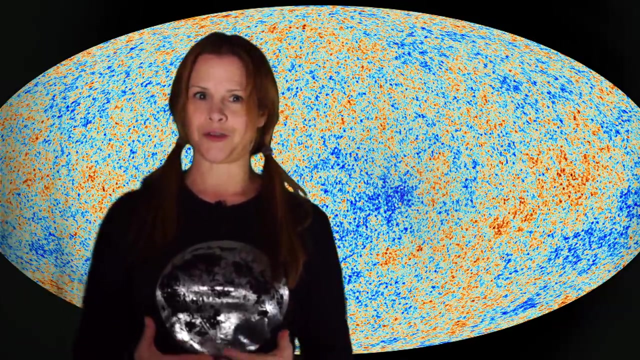 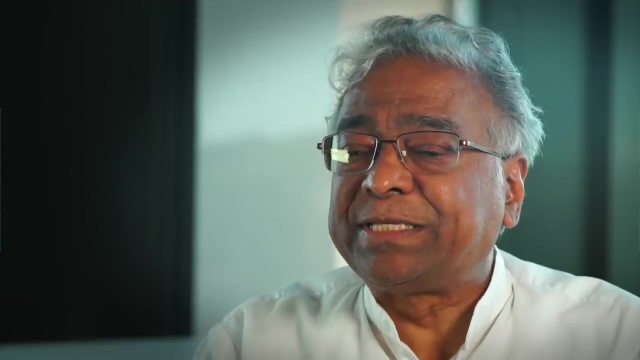 I can rearrange these black holes and I can only probe the physics associated with the exterior of the black holes. When we look at the oldest light in the universe, the cosmic microwave background, we find that it is not low entropy, it's high. 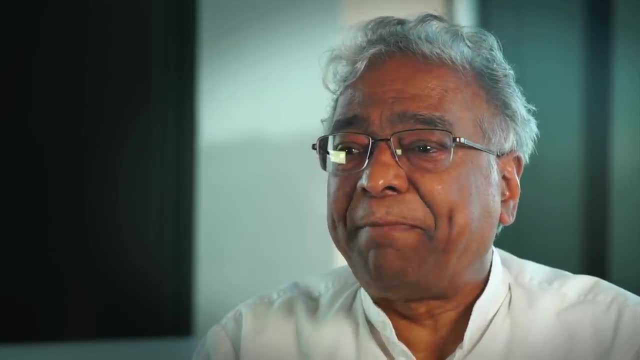 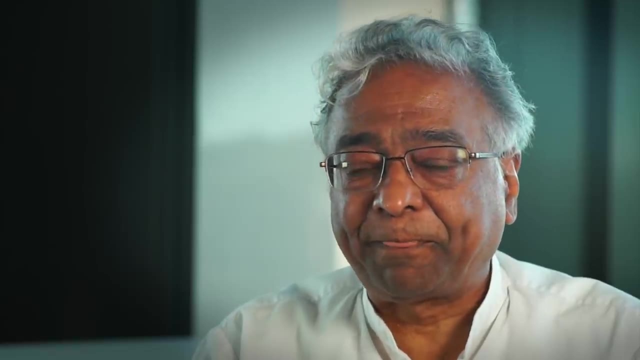 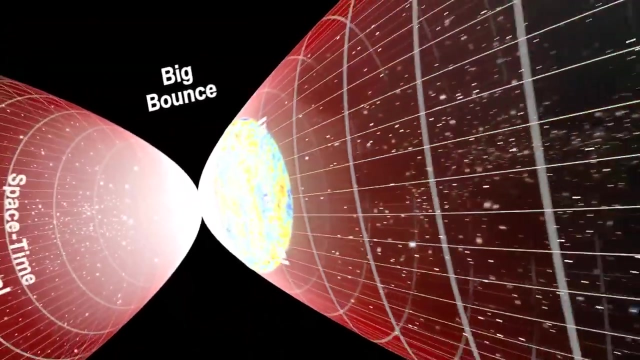 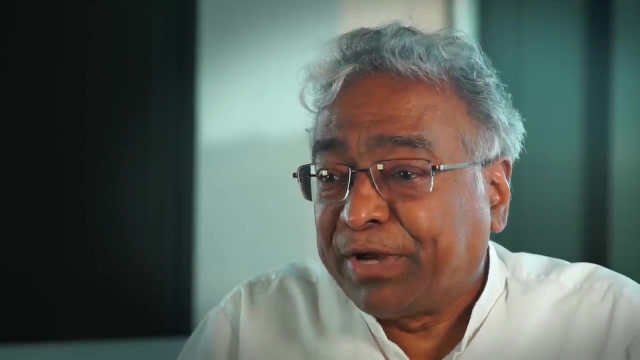 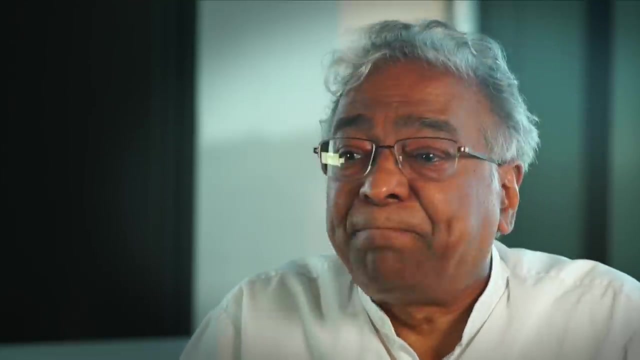 entropy. it's not just the entropy of matter, but also entropy associated with horizons, so to say the gravitational entropy In the contracting branch, because the dynamics is different from Einstein's theory. a lot of this entropy dominates completely the entropy of matter. 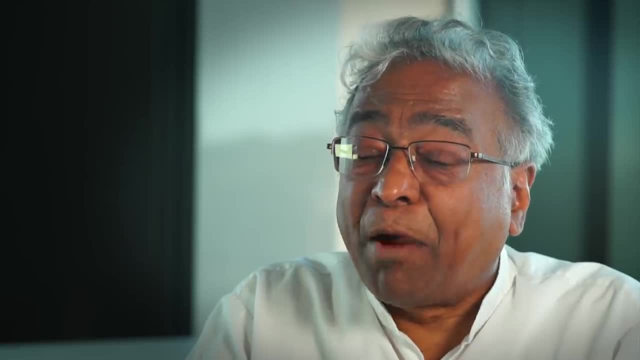 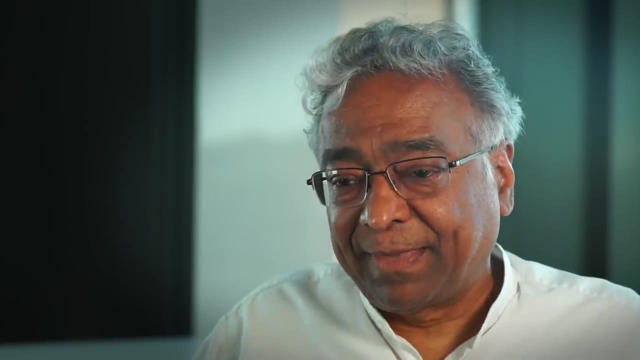 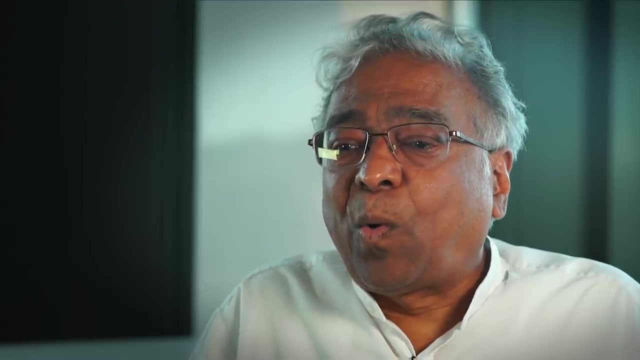 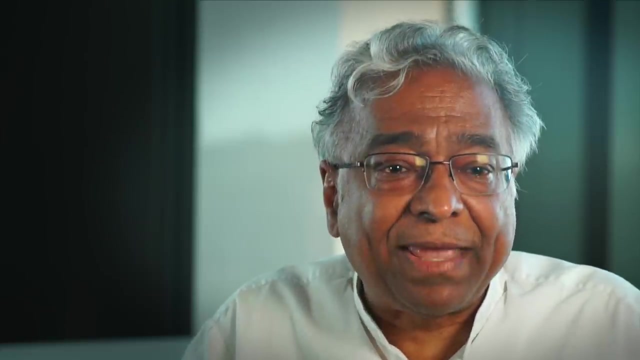 Therefore, the entropy is really growing very rapidly, but then at the bounce. the geometry is such- which is a non-trivial statement- is such that, in fact, the area of this horizon is the entropy clock, in a certain sense. 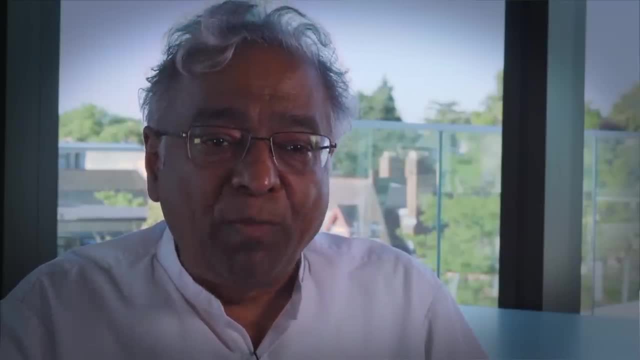 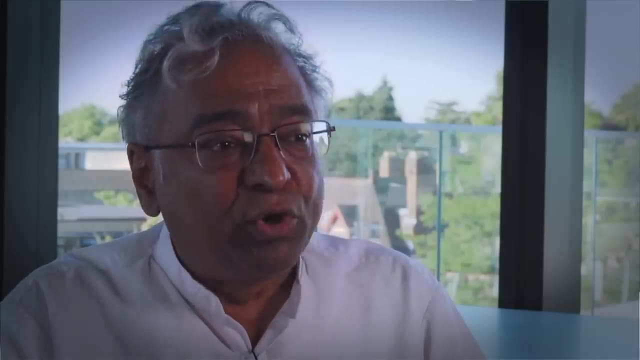 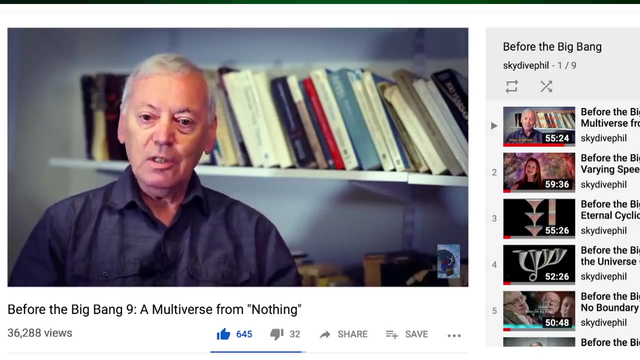 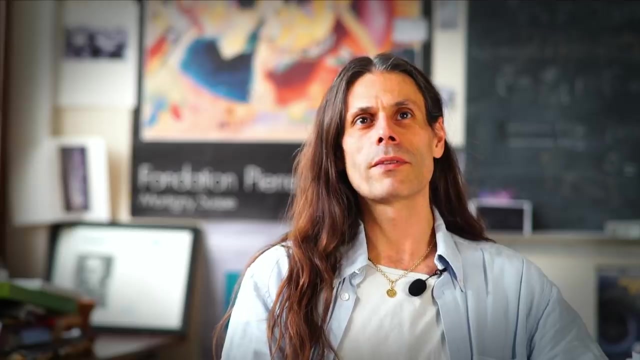 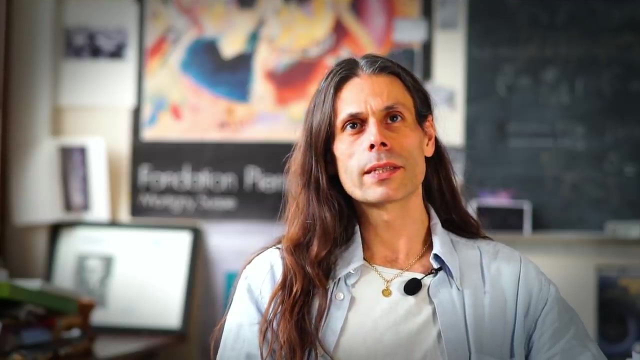 at the bounce and then the entropy again increases With the scheme that we have- precise scheme we have- the entropy is always increasing for the bounce. So it's very speculative and very difficult to decide whether the situation is stable or not, And even 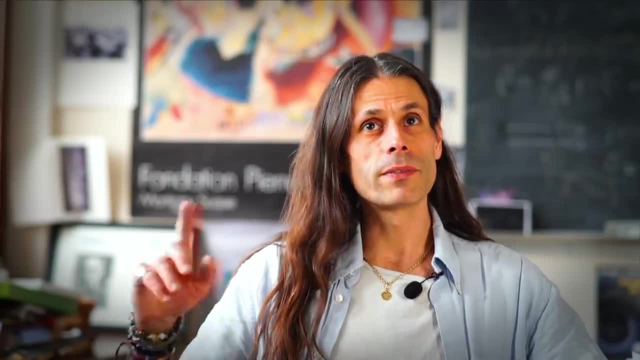 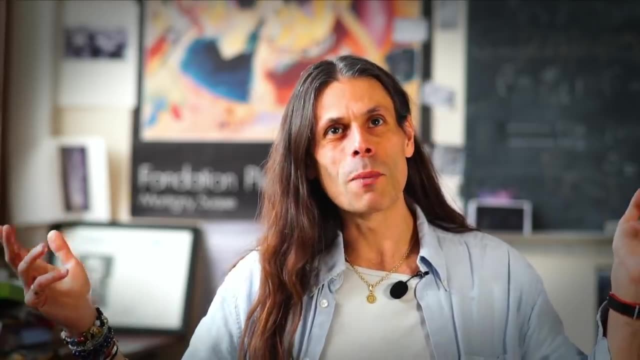 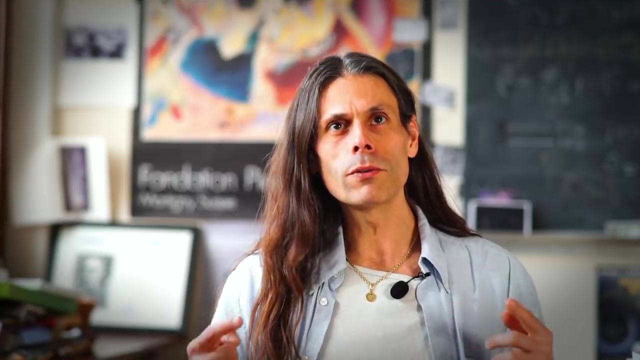 in the case where the situation is unstable. usually what it means is that the simplifications we use in standard cosmology cannot be used anymore. But you know that the model we use to describe these things doesn't work anymore. For example, you cannot use the Friedmann equation, because the universe is so inhomogeneous that the Friedmann equation is not usable anymore. So what? The universe doesn't care that we have to invent another equation. I think the correct way to think is not to go from one to 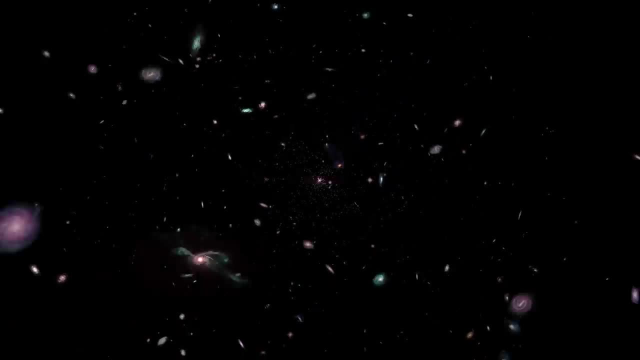 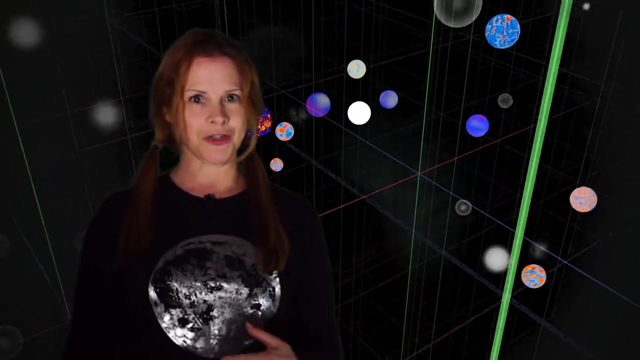 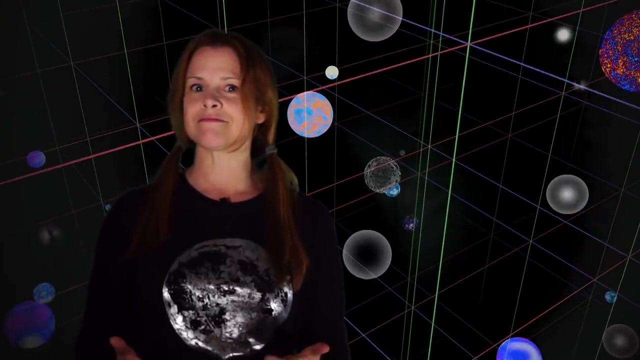 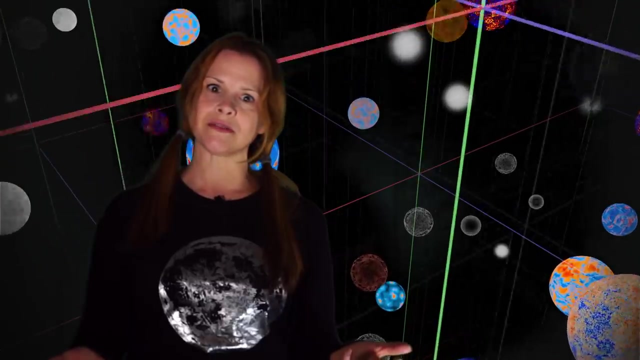 another. and then we go backward in time and we see what happened. And in our theory, when we go backward in time, we do not end up with a singularity, we end up with a bound. String theory seems to predict the natural selection. 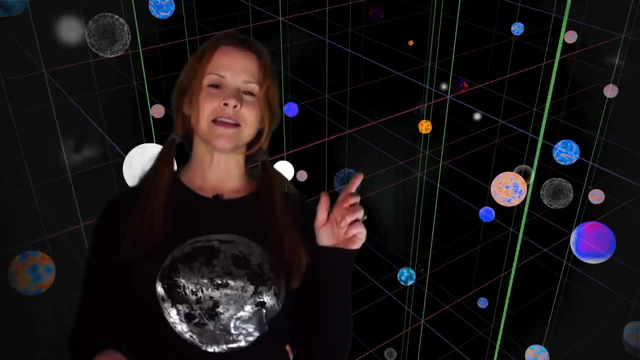 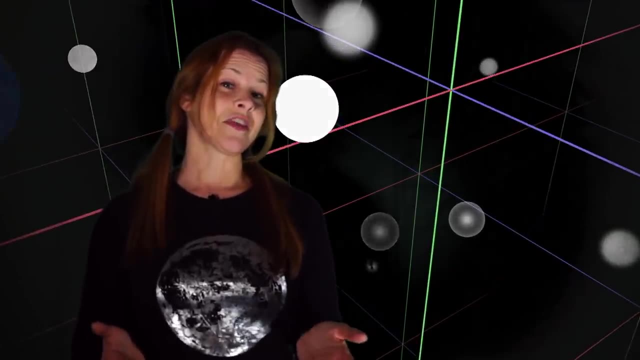 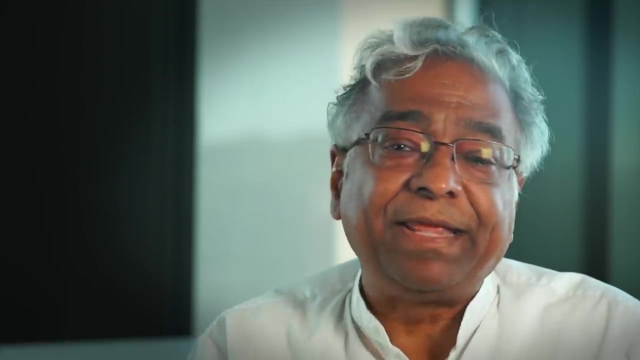 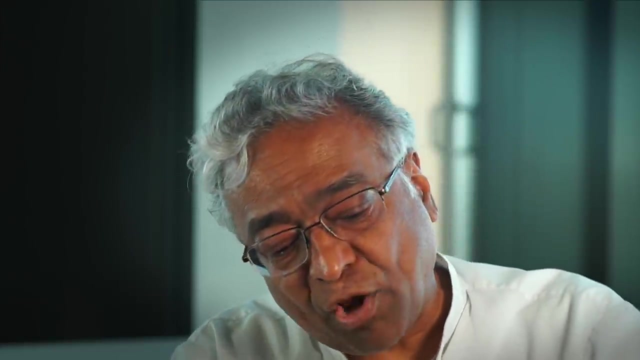 of the universe. We'll detail that in a future film. But other alternatives are that fine-tuning itself is an illusion and that the constants are set by necessity. There could be necessity in the sense of. I agree that all the detailed solutions are different. 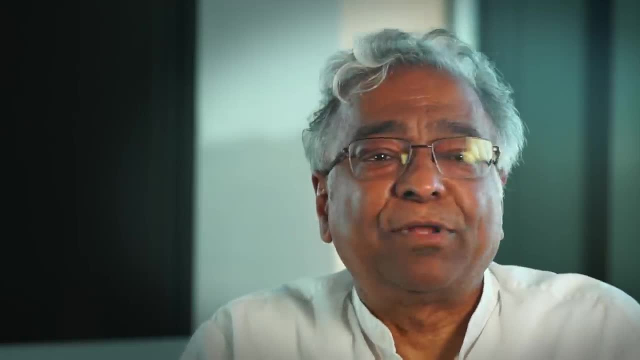 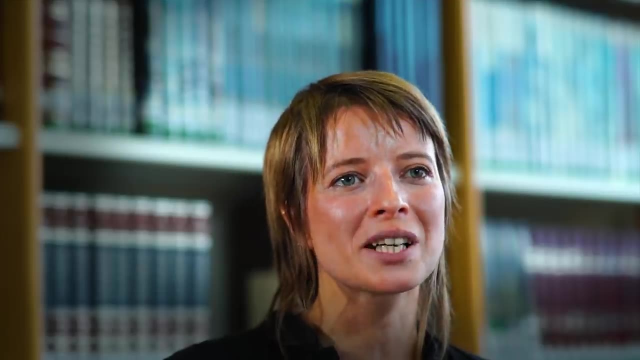 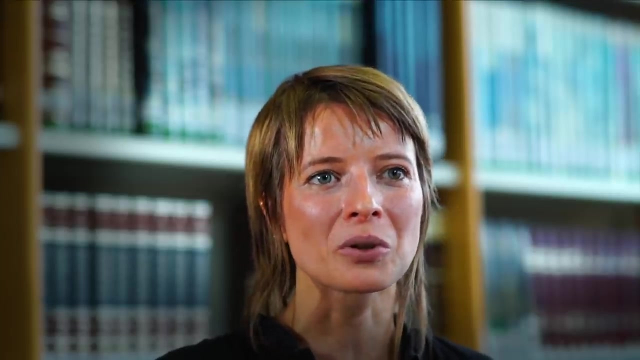 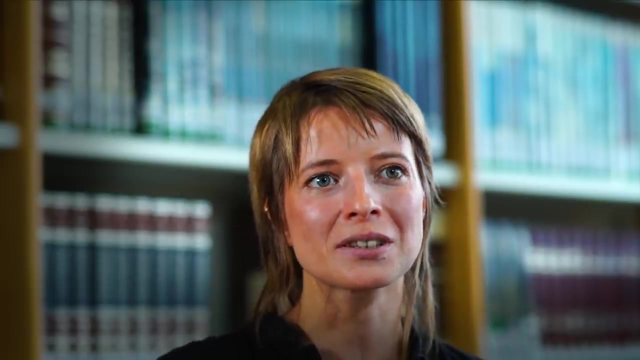 and yet life forms. That, to me, is not at all impossible. We have to be very careful in the way in which we treat probabilities. So when you say something is probable or something is improbable, it's with respect to the universe. I imagine that we 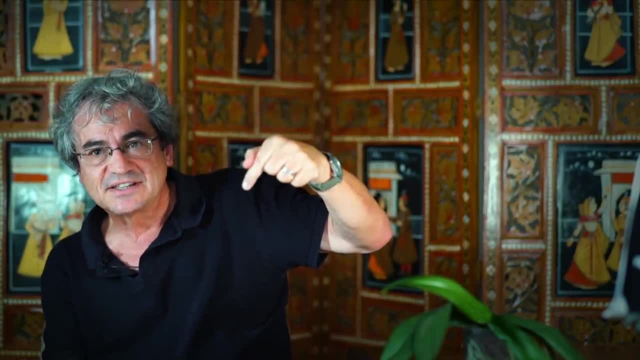 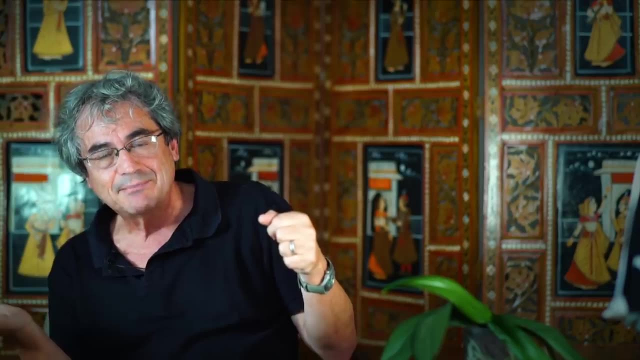 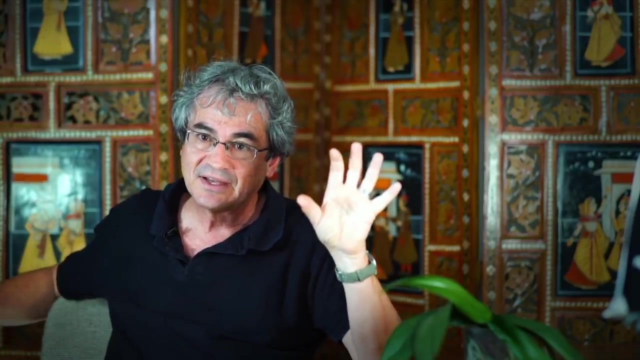 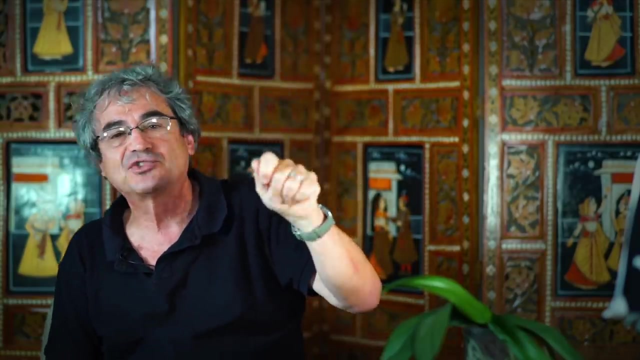 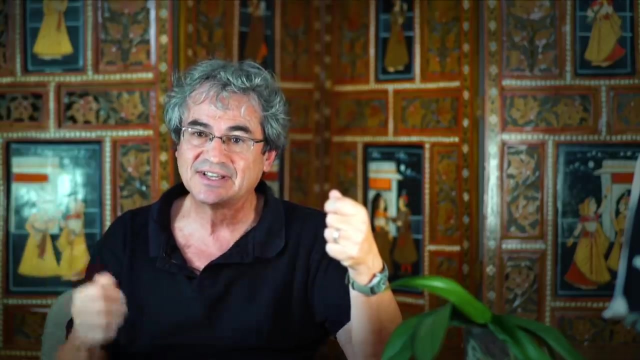 have only this universe And people say yes, but if the constants were a little bit different, there would be nothing. And that's incredible intellectual arrogance and stupidity, because nobody would be able to calculate a coupling of the Higgs. a little bit, Of course there would. 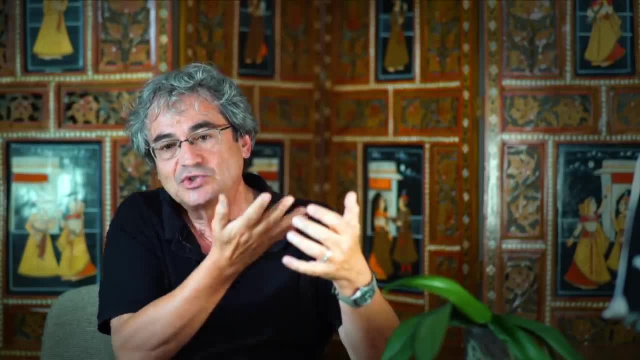 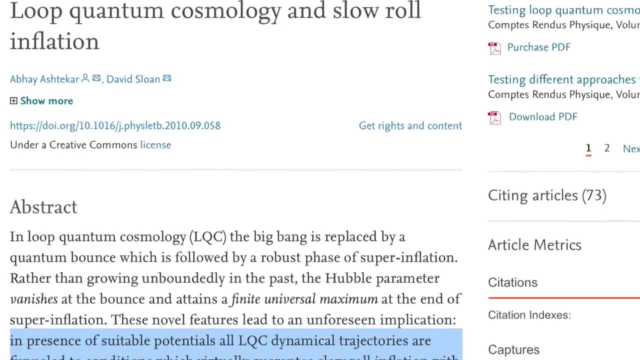 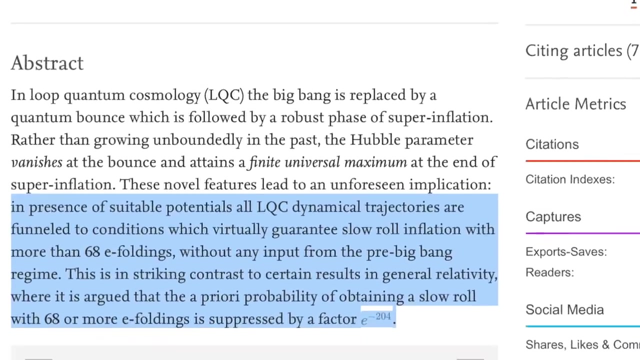 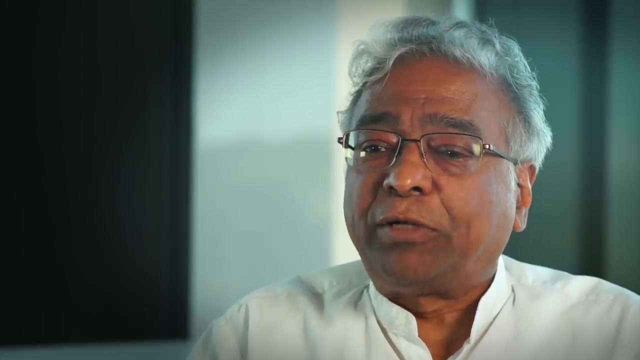 not be carbon, there would not be stars, but there would be something else, And nobody is able to say correctly and plausibly and credibly that the universe would not be in the universe. So the question is actually ill posed, because the answer depends on the time that you choose to ask the question. If the initial conditions are specified at the bounce, we have an unambiguous answer that almost all initial data specified at the bounce will actually evolve into giving us enough number of E-foldings in the future. 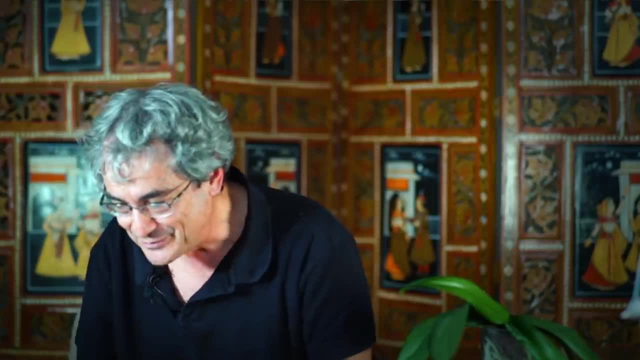 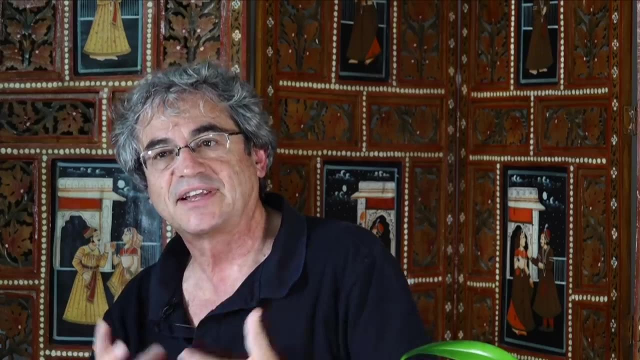 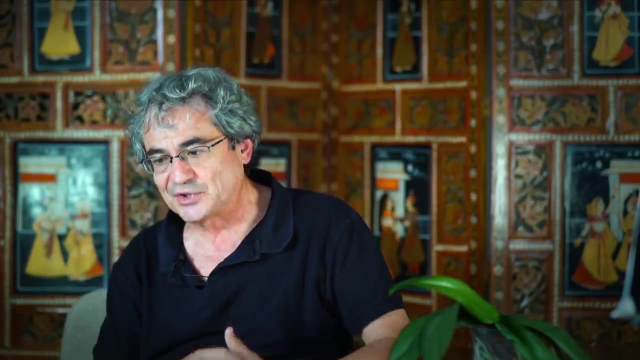 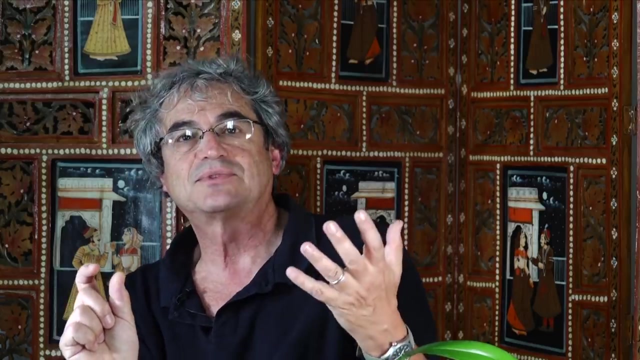 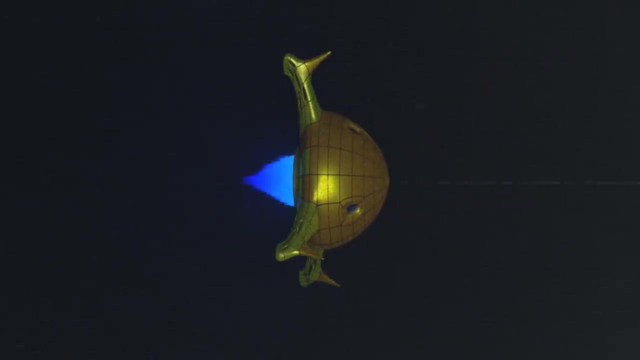 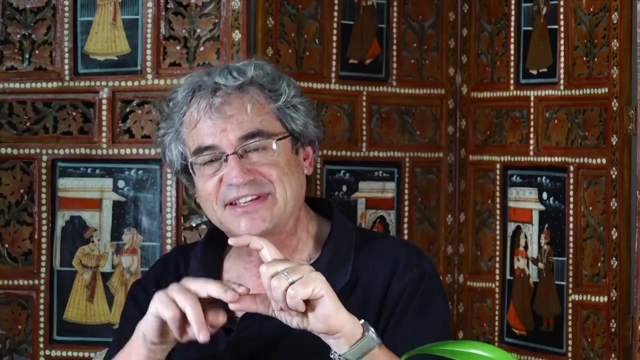 A key difficulty for any quantum gravity theory is how it deals with a fundamental feature of the universe. If you look at the mass of the Earth and the mass of the atmosphere of the Earth, you can see that the mass of the Earth, which is the mass, 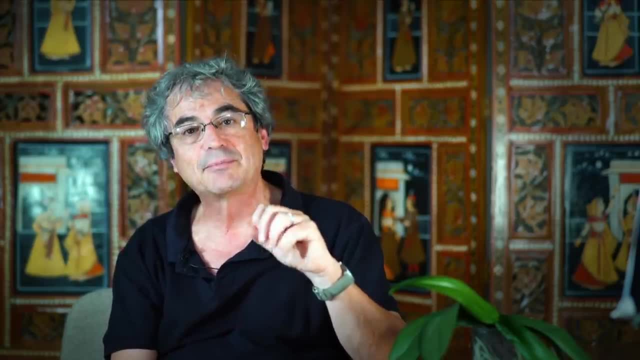 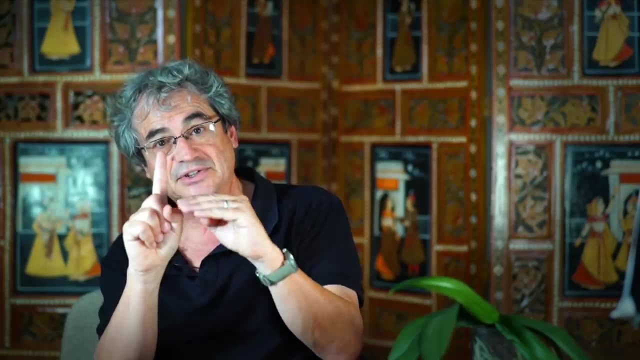 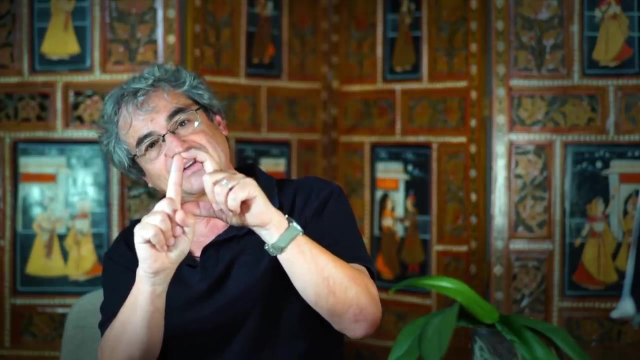 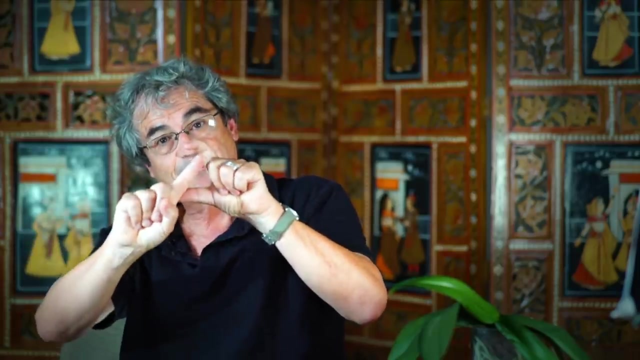 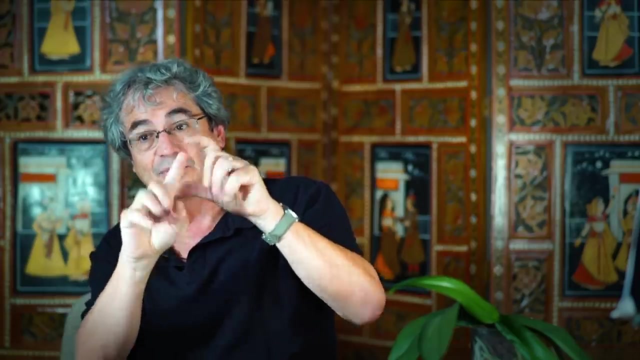 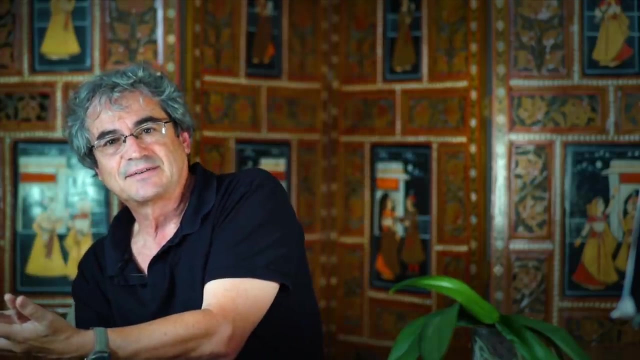 that is the mass of this planet. When you look at the mass of this planet you can see that the mass of the. So it seems incompatible the discreteness of a component of angular momentum with a rotation invariance. But everybody knows that in quantum mechanics there is a rotation invariance and also discreteness. 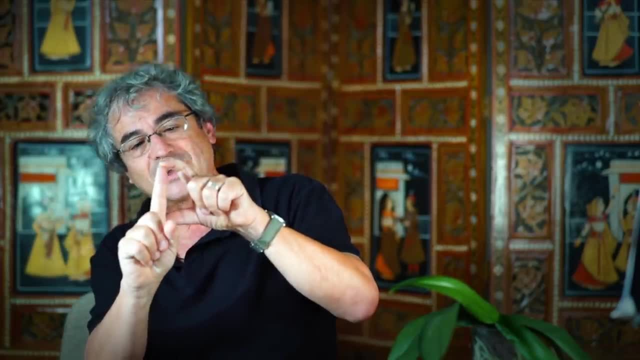 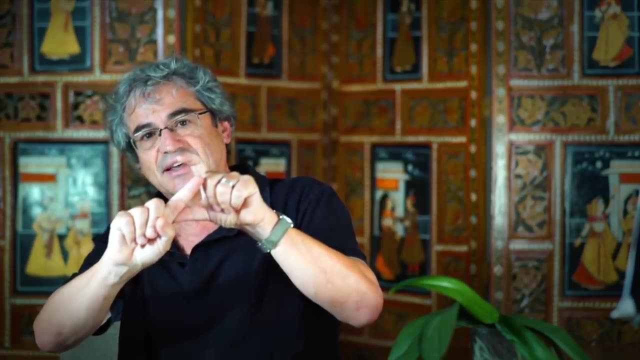 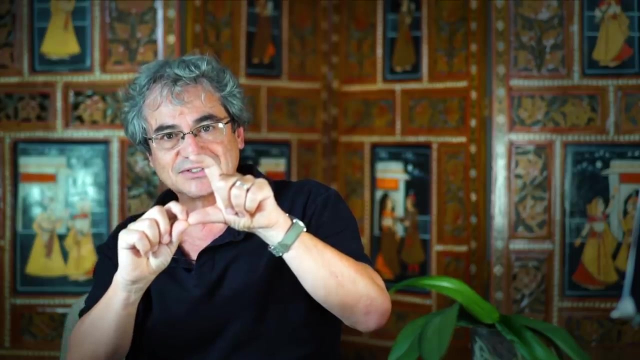 How does it work? Well, it works that when I turn my head, what happens is not that this shrinks, It's that you have a probability of seeing this full length and a probability of seeing it smaller, And the probabilities move, But you only see either this long or this long, only the discrete values. 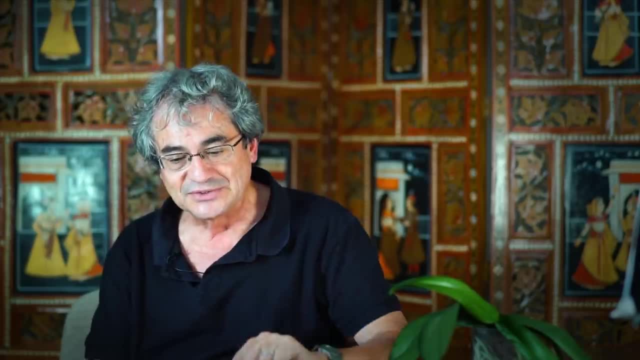 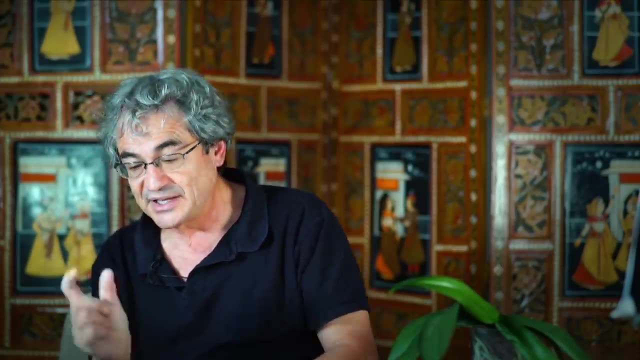 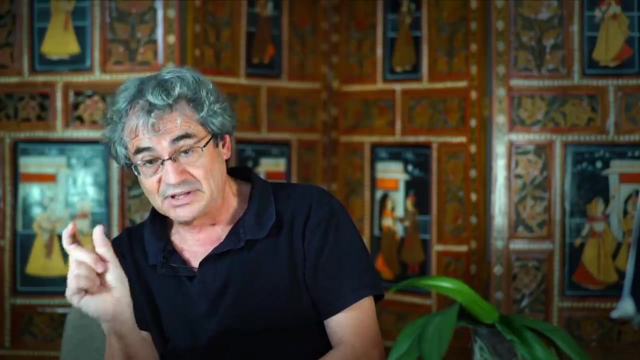 That's the answer. So the answer is probability And loop. quantum gravity is compatible with Lorentz invariance in spite of the minimal length. for the same reason, Namely, if you have something minimal length and you move fast, you have a probability of seeing it minimal length or a probability of seeing it zero length. 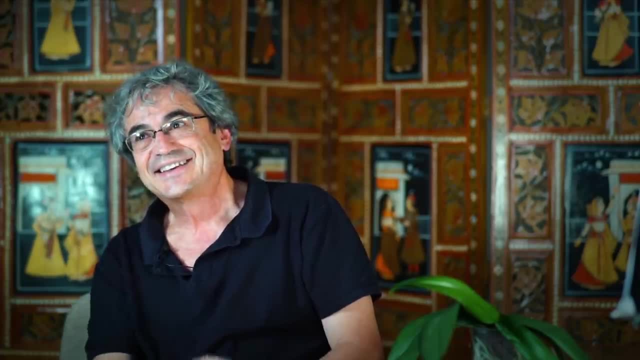 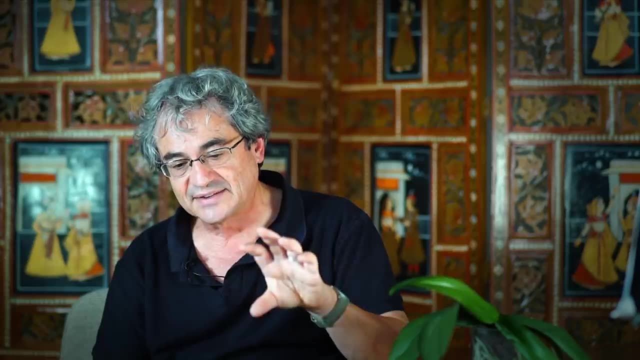 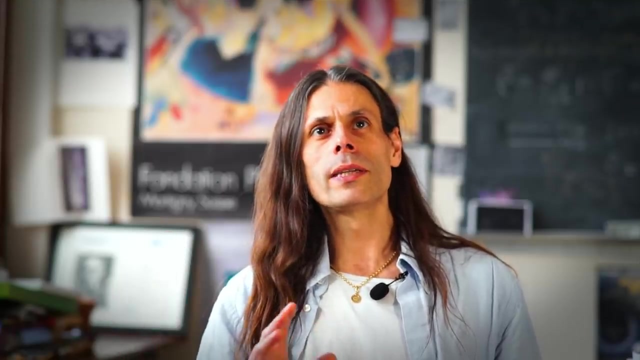 You never see it- half a plant length. So it's a beautiful example of how quantum mechanics allows discreteness and continuous symmetry groups to stay together. So here we are completely in the regime where you have to deal with effective theory. So you really try to guess. 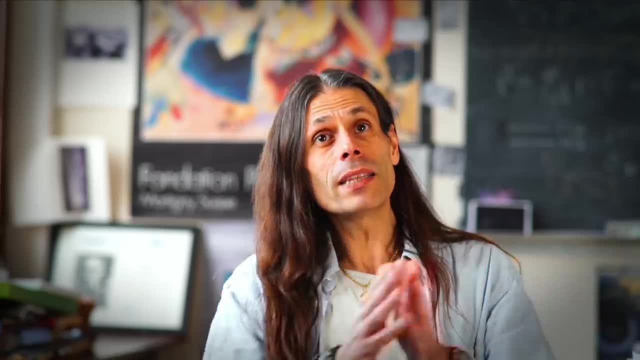 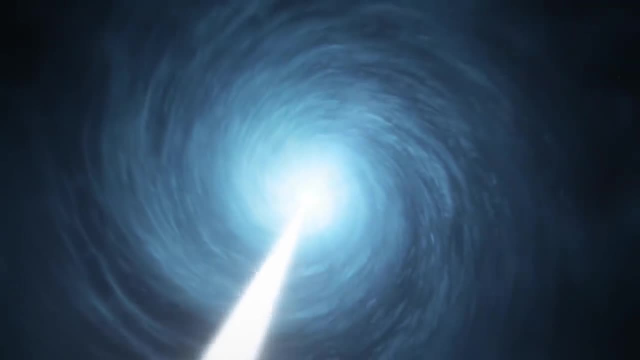 How Well the high energy quantum gravity effects will manifest themselves on a very low energy phenomena, because you know gamma rays. it's maybe 10 or 15 orders of magnitudes below the Planck scale. So it is very low energy with respect to the Planck scale. 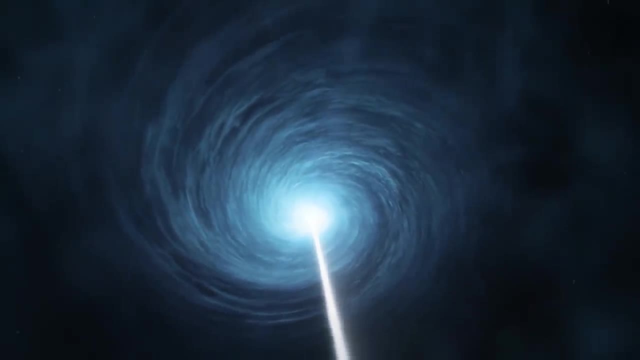 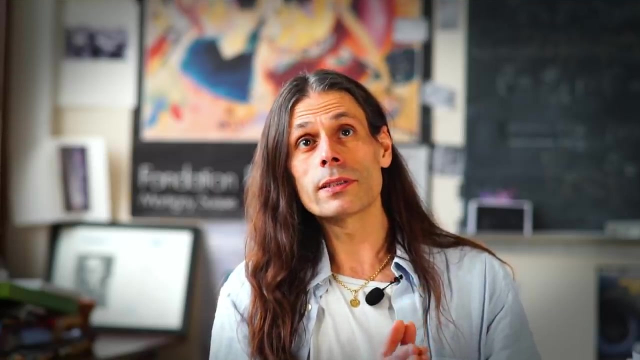 And once again there are different cases. So if you see nothing, as it is the case up to now, you cannot conclude, because it's perfectly possible that Lorentz invariance is indeed preserved by loop quantum gravity. But in the case you see something, you see that the speed of light Depends on the energy, even in vacuum, then this would be probably a smoking gun for quantum gravity, maybe not for a specific theory of quantum gravity, but for the idea that space is not continuous and that you have some atoms of space, like you have atoms in a crystal. If loop quantum gravity predicts the existence of spacetime atoms, where do the new atoms come from when the universe expands? Well, that's the same question as asking classical general relativity. the universe expands And the volume increases, So you can just ask the question: what creates this volume? 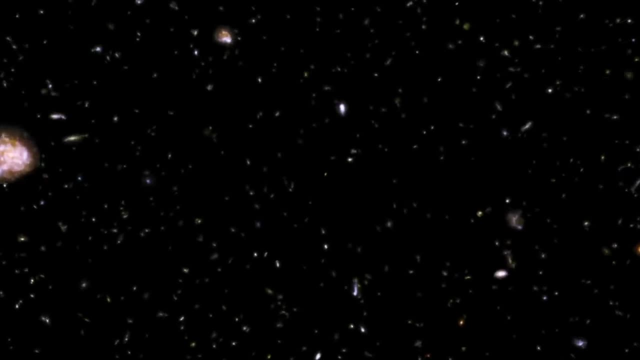 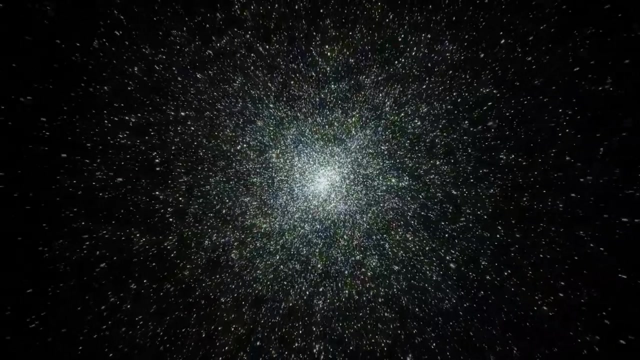 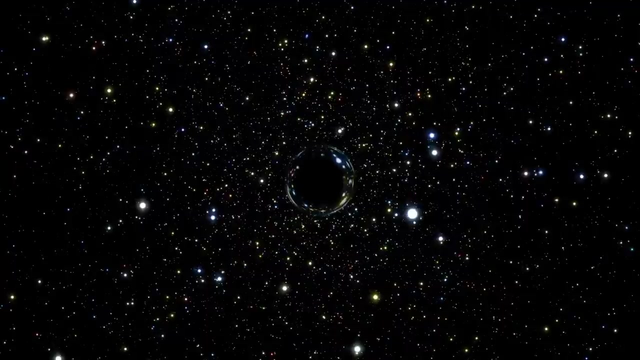 Well, it's dynamics which creates this volume. So there is no conservation law for volume and there is no conservation law for the number of atoms of geometry. Another route to exploring experimental testing of the theory comes from nature's most mysterious objects: black holes. 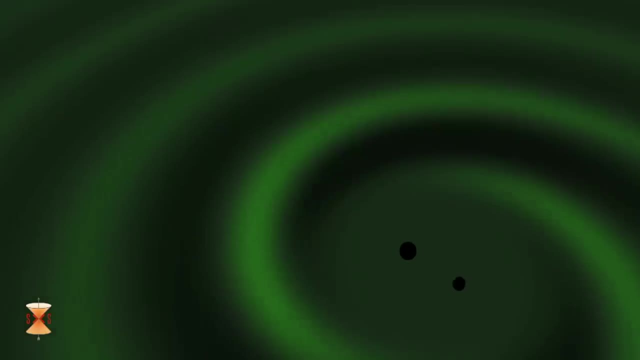 A few years back, we have detected for the first time gravitational waves directly thanks to LIGO. These are the black holes that exist in the US and the Virgo antenna in Europe, and what we are basically seeing is the coalescence, the merging of two black holes and then the relaxation of the big black hole coming from that. 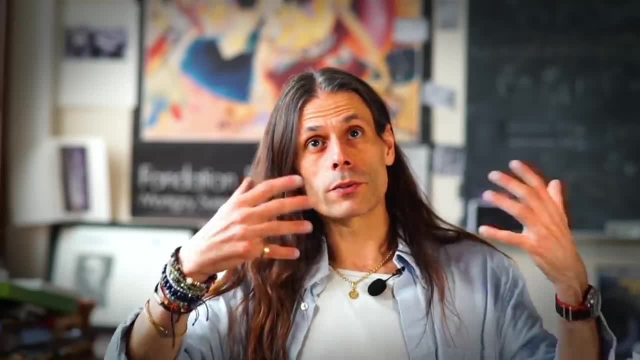 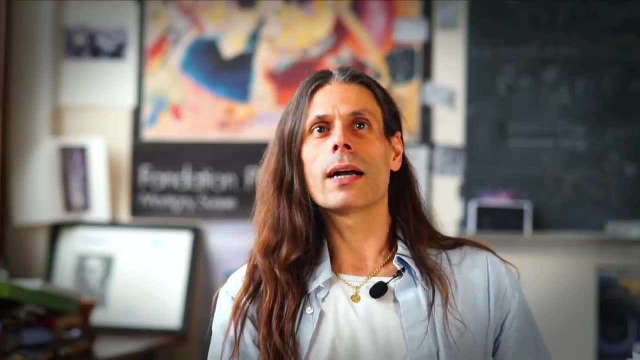 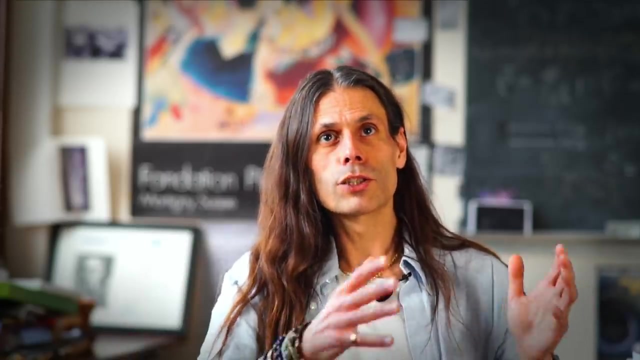 And the way this big black hole is losing its energy through gravitational waves might depend on quantum gravity corrections. So it is still speculative at this stage, but it is possible that some quantum corrections outside the horizon of the black hole change This relaxation mode of the black hole and this could be probed by gravitational waves. 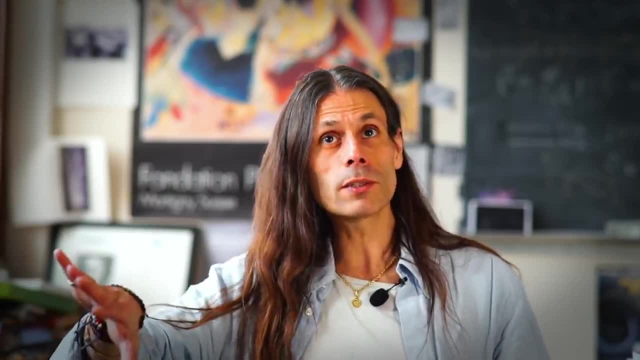 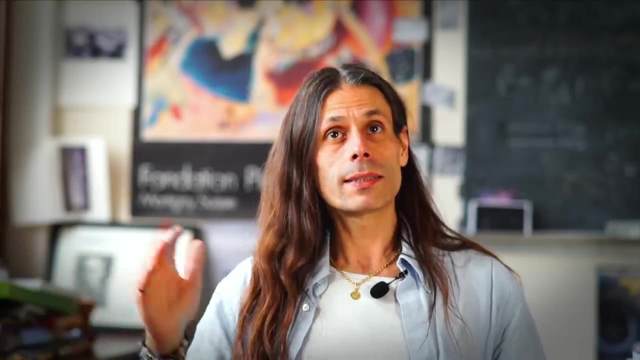 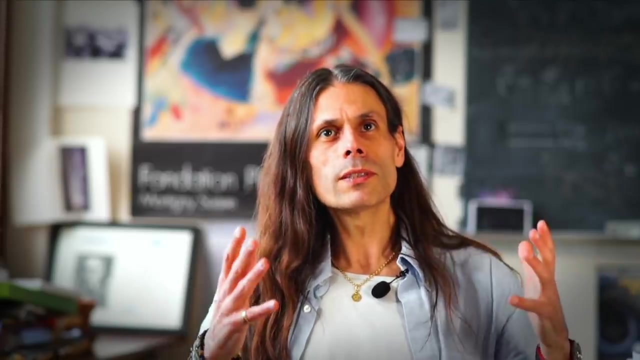 There are similar ideas in string theory with, of course, different consequences, hopefully- But it's very exciting that we now think about possible ways of testing quantum gravities thanks to gravitational waves, because the way the black hole moves tells you something about the proper modes of spacetime. in itself, 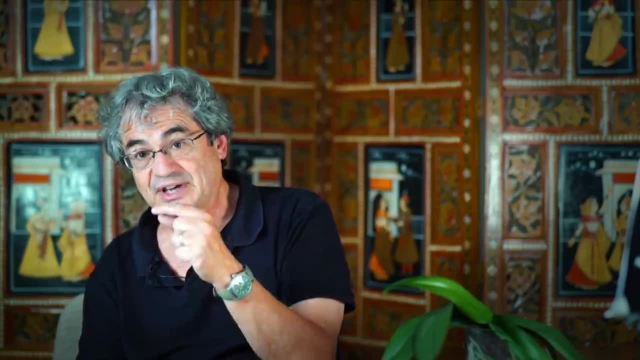 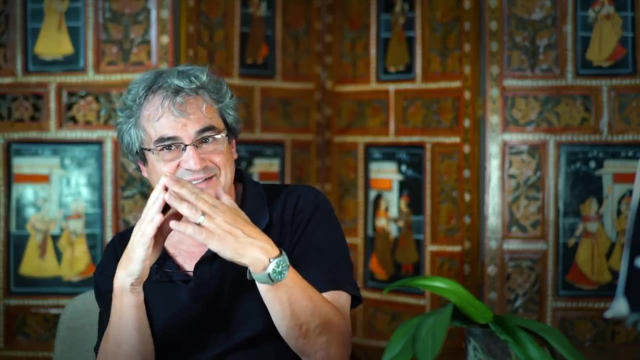 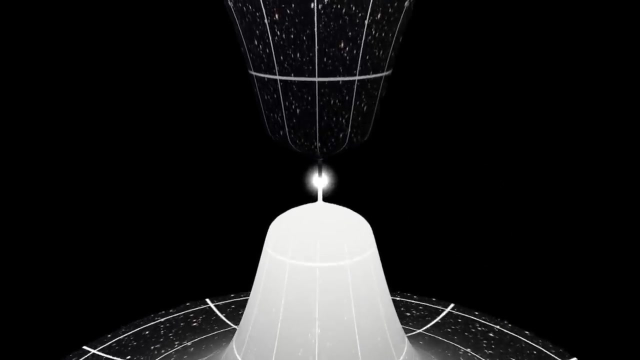 We got convinced in recent years, and we are trying to convince the community, that when you go to the center it doesn't end there: the universe. you continue, You continue. you go through a quantum region, but very rapidly you go out of this quantum region. 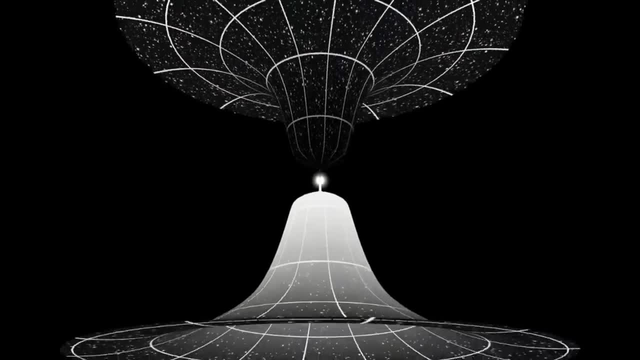 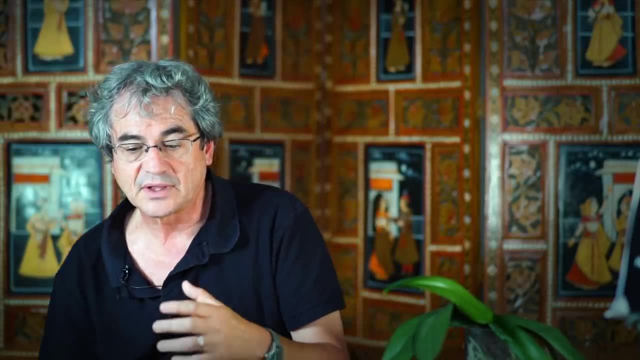 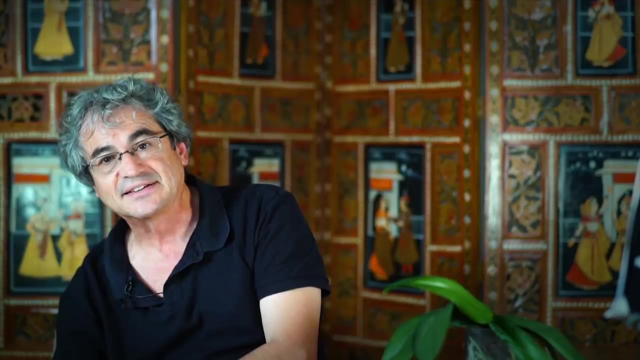 and what you have on the other side of the quantum region is very simple. it's just the time reversal of what went in. And the physics is simple: if you take a ball, you let it fall, it goes down, and what happens when it hits the ground? 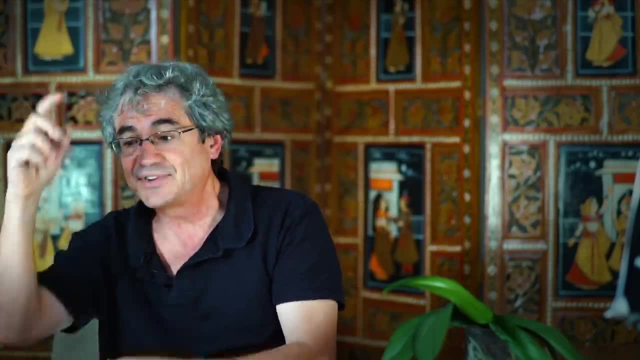 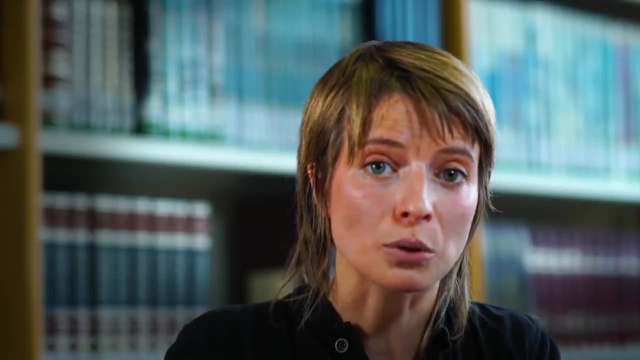 Well, the first approximation, it just comes up. And how does it come up? It's exactly the time reversal of when it went down. The way in which these effects are manifested, as we know from quantum cosmology, is in the form of an effective repulsive force. 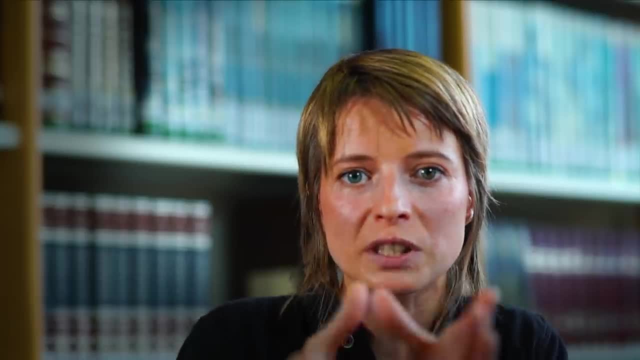 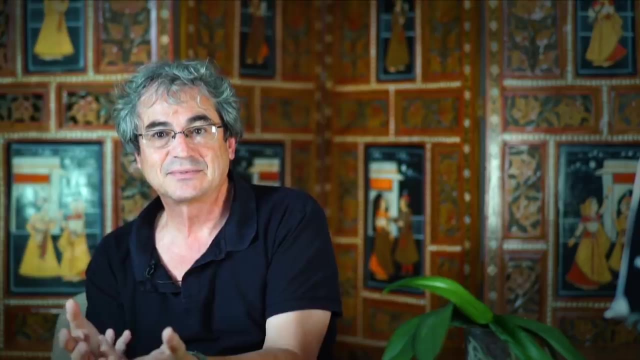 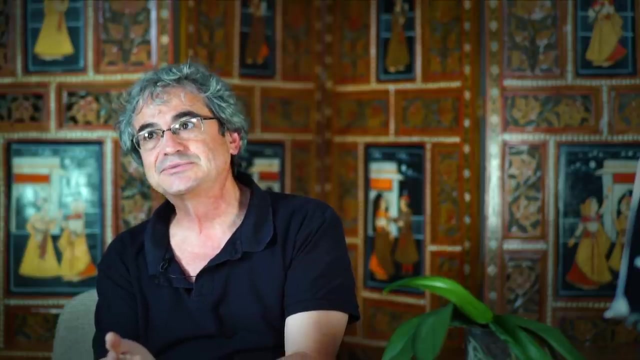 So this collapsing phase should evolve into an expanding phase. And why it bounces? Well, because you cannot compress things too much. there's a limit in compression. You know. there is a Heisenberg uncertainty principle. for the same reason, an electron cannot be squeezed in an atom. 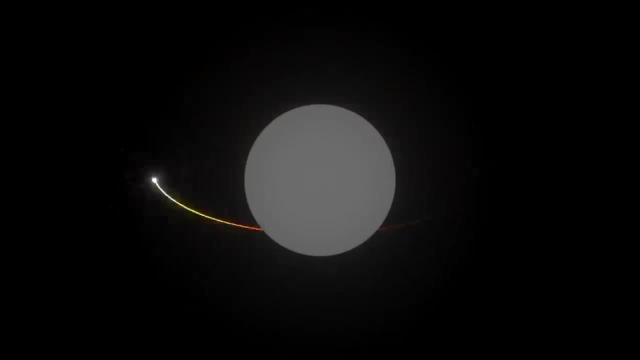 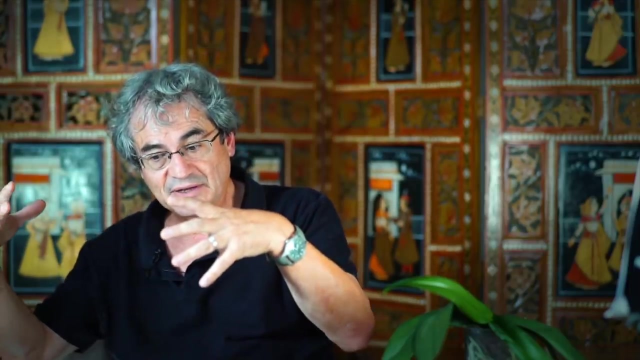 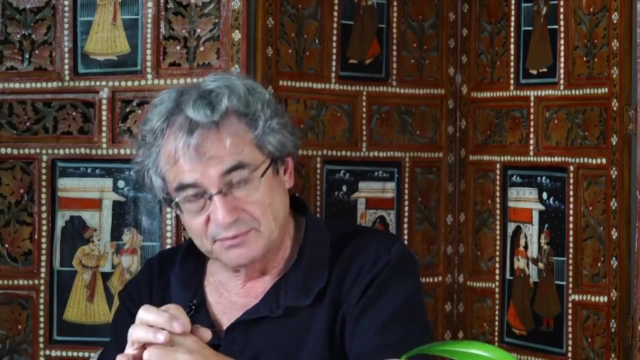 You know, classical theory predicts that an electron is going to fall on the nucleus of an atom, but it doesn't Why it doesn't Because of quantum theory. Quantum theory forbids something to squeeze something too much. What happens is that the matter bounces, but seen from the outside, 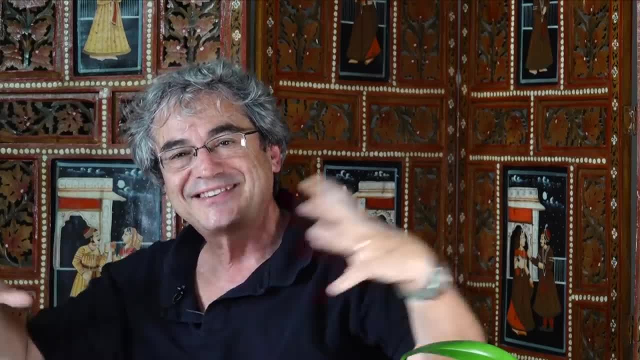 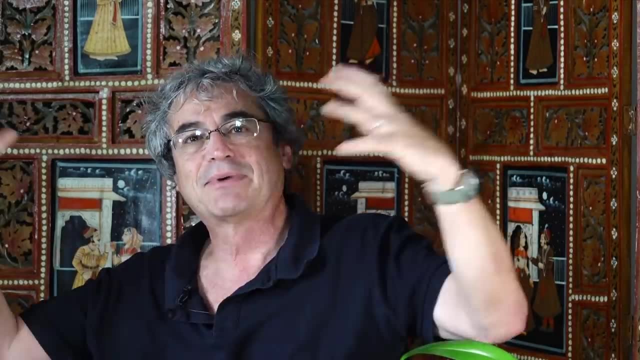 this bounce takes a very, very, very long time. So the physics, if you fall in, is vroom, vroom. You go to the minimum and you bounce up, But seen from the outside, you see these things in some sense. 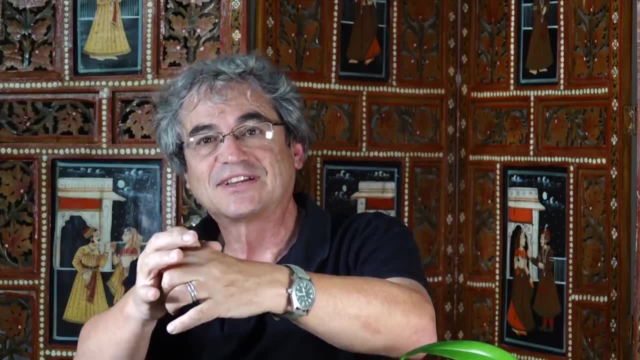 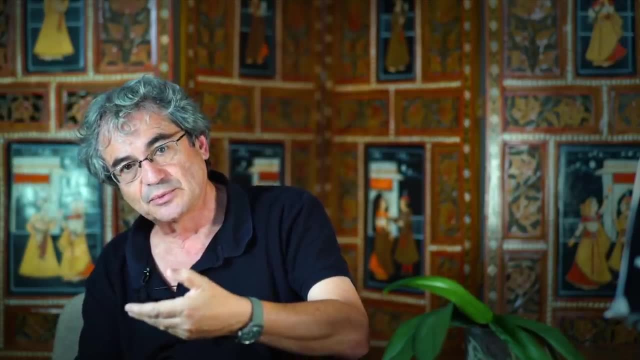 slowing, slowing, slowing, slowing, slowing down takes billions of years, and then slowly, slowly, slowly coming up. I'm convinced that what a black hole does is go through a quantum phase, becoming the time reversal of a black hole. 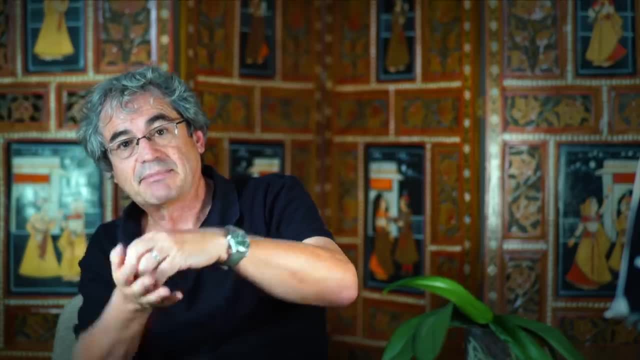 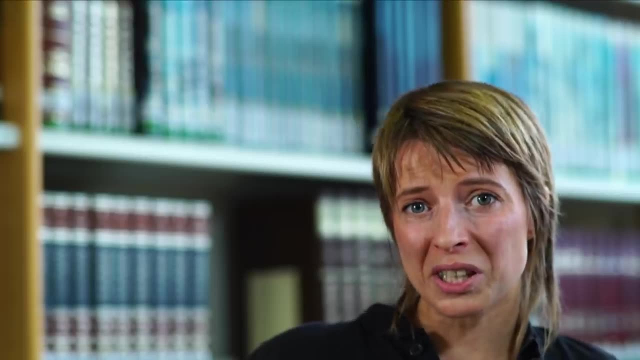 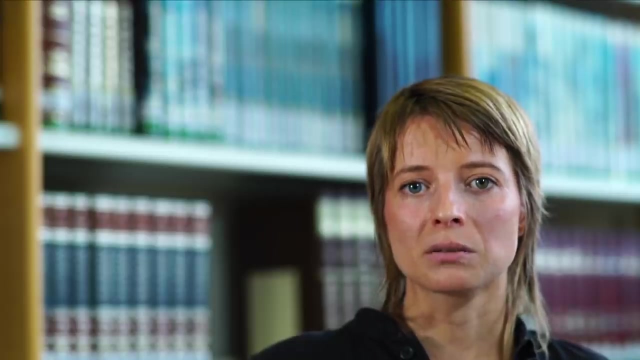 which is called the white hole, and bounce out. So what do we need to do to test this idea that a black hole evolves into a white hole? What we need are black holes that are old and small enough to be exploding today, So this means that we need what are called primordial black holes. 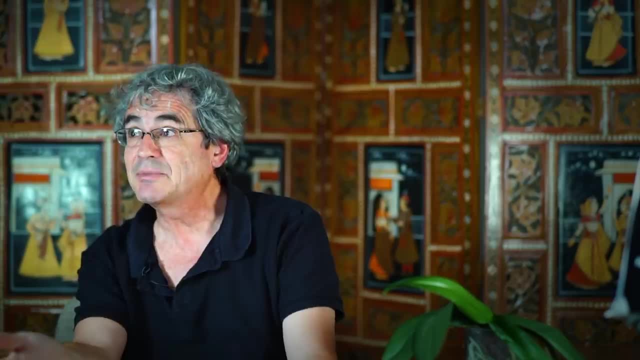 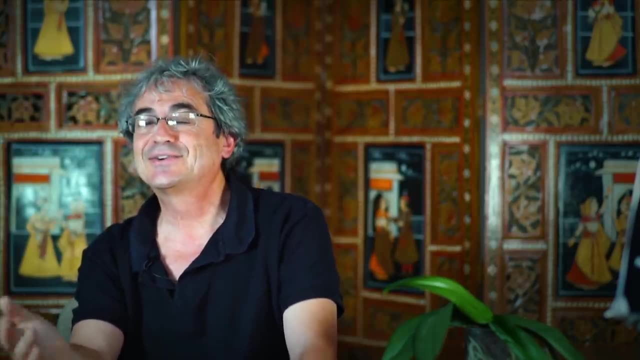 black holes that formed in the very early universe. I remember Francesca calling me and saying: well, you know that this fast radio burst. I had no idea what it was, this fast radio burst. So she said, look into that. 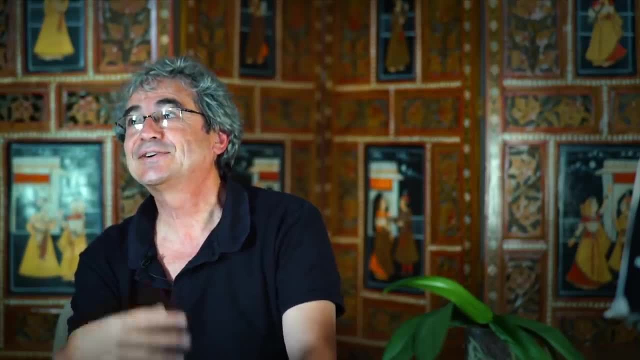 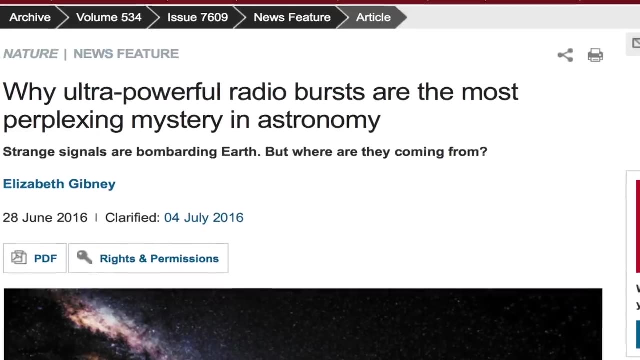 And so I googled fast- radio bursts, And it turns out that there was an article. Nature said: the biggest mystery in astronomy. So what's the biggest mystery in astronomy? Apparently they're seeing these very violent signals with a radio telescope. 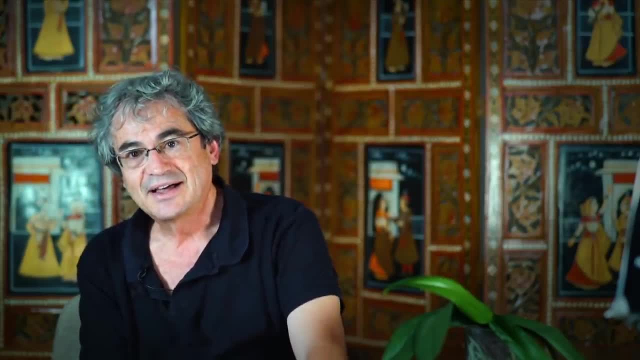 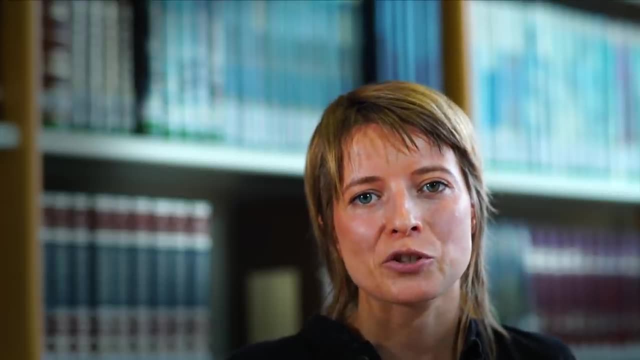 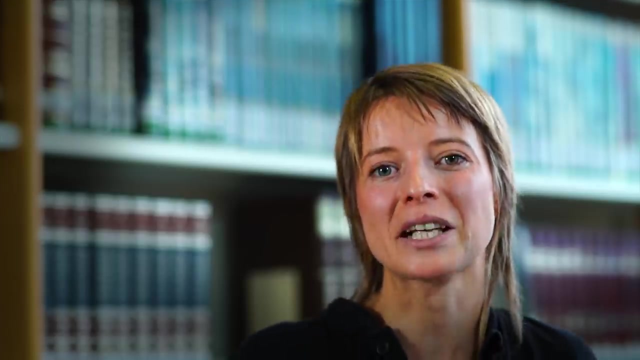 We're seeing Australia and Arecibo, And they were so strong that they didn't believe them at the beginning. We have too many explanations today. We have more explanations than the number of actual detections. We had this idea that perhaps fast radio bursts are exploding white holes. For gamma ray bursts. we know now that, depending on their duration, they probably have different physical origins. So it could very well be that fast radio bursts do not all have the same origin. There are so many radio sources in our universe, so many sources of radiation. 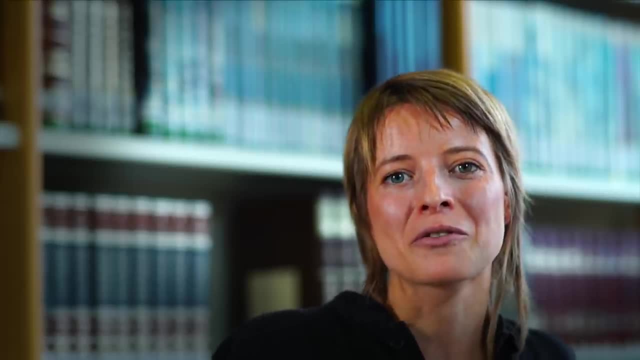 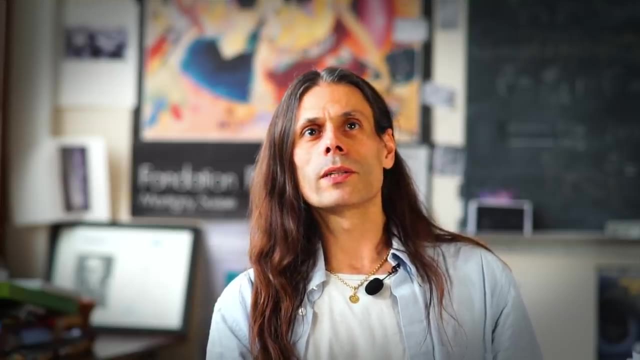 So how can we distinguish radiation coming from exploding black holes from all the other sources? With Carlo Rovelli and Francesca Vidotto, we tried to make a full phenomenology of the phenomena that could take place due to those bouncing black holes. 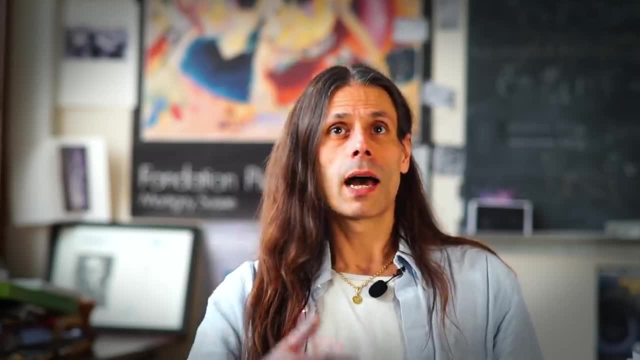 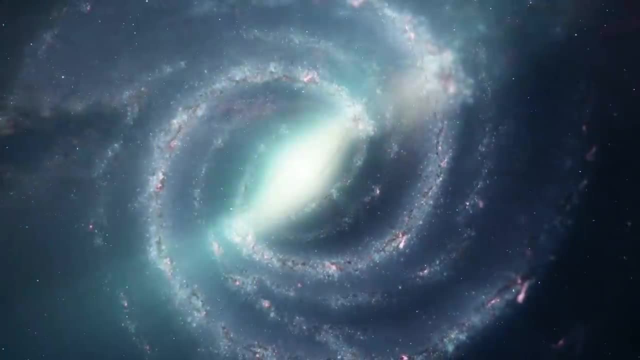 So it's correct that fast radio bursts could be explained. I have also shown that the Fermi excess, that is, the too many gamma rays we see from the galactic center, could also be explained by this model. This is not very convincing, because when you are a theorist and you have a model, 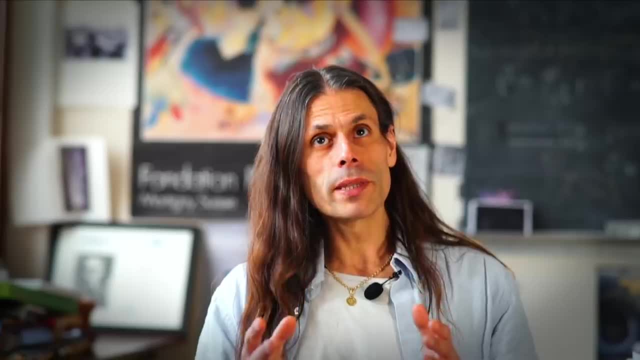 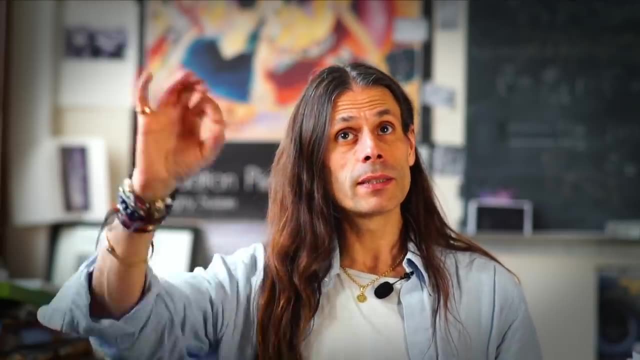 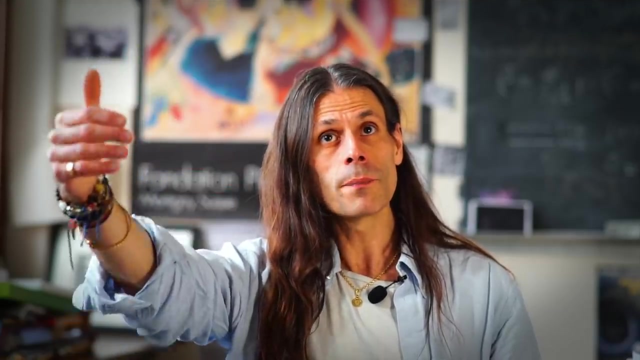 you can basically explain nearly everything. We know how to discriminate between this model and all the other models that are currently available, And the reason for that is that the redshift dependence- that is the way the signal coming from bouncing black hole depends on the distance at which the source is- will not be the same for our models. 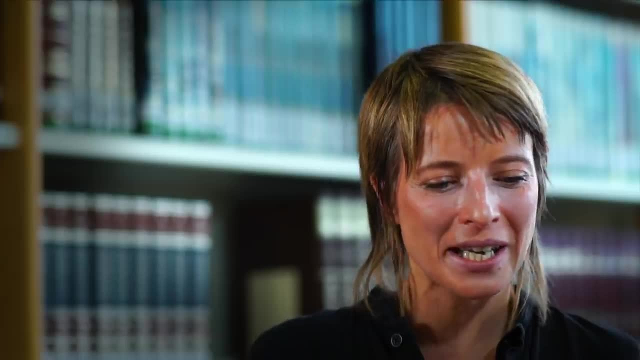 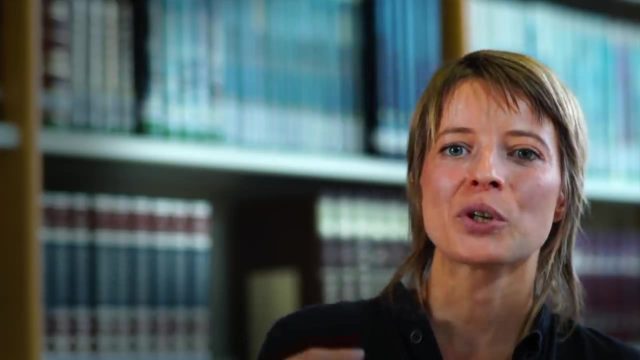 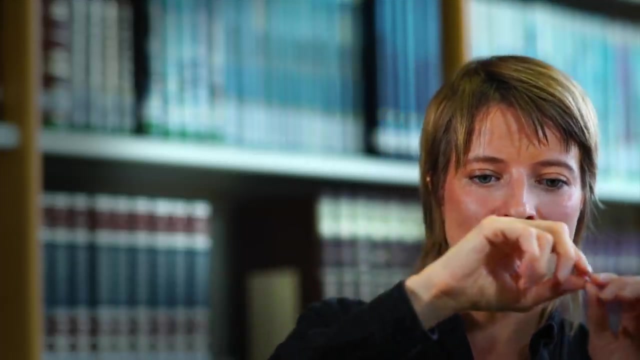 and for all the other astrophysical or particle physics models. If I have a burst coming and it's exploding black holes, I can put them on a graph in which I have their observed wavelengths and their distance, And this would form, instead of forming a line as all the other astrophysical objects. 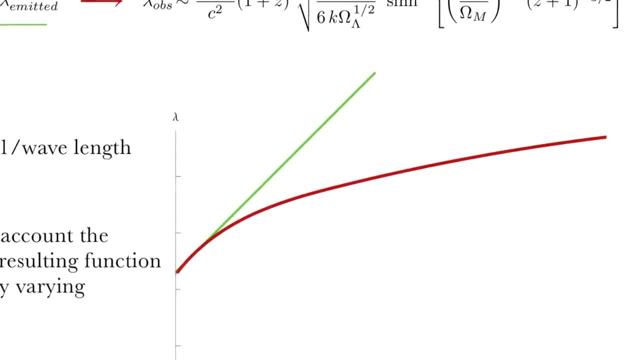 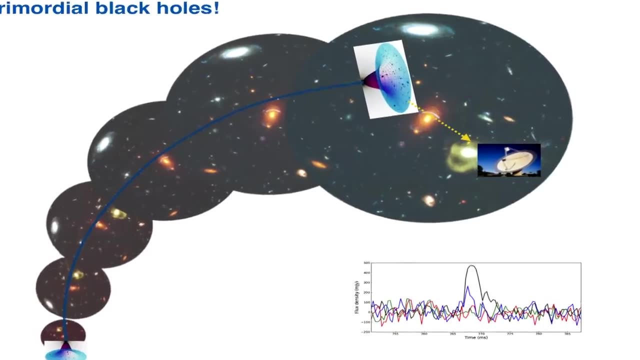 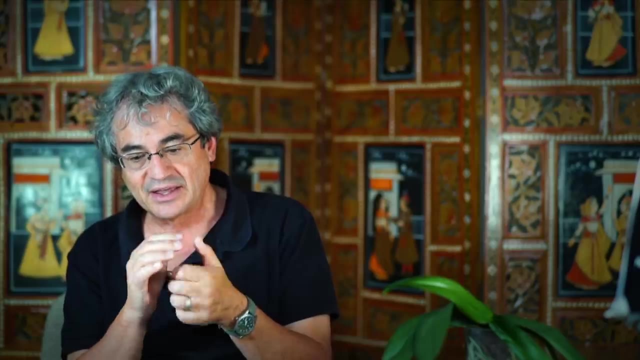 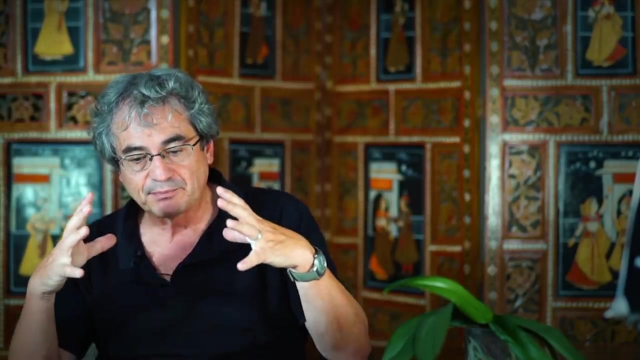 that would form a curve that is flattening for higher values. It would be fantastic because it would be a genuine quantum gravity phenomenon directly observed in the sky. There's a lot of ifs in this story. The main if is whether a black hole explodes when it's large or when it's small. 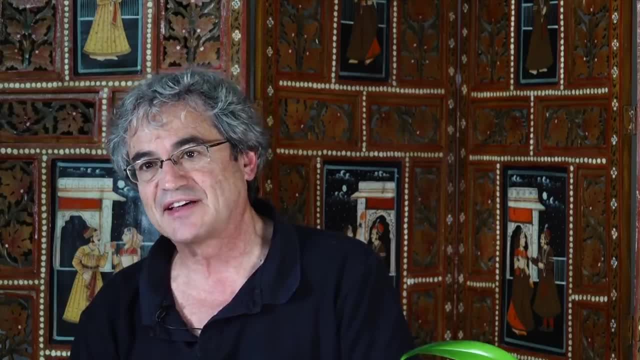 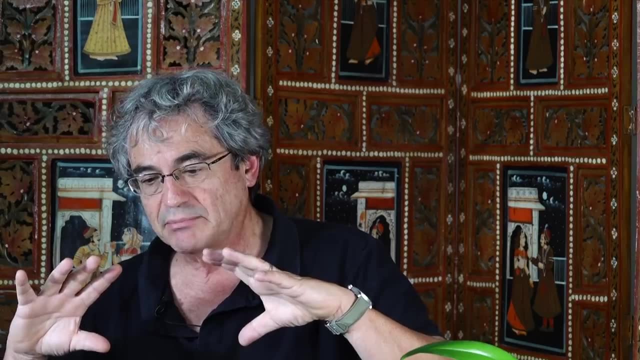 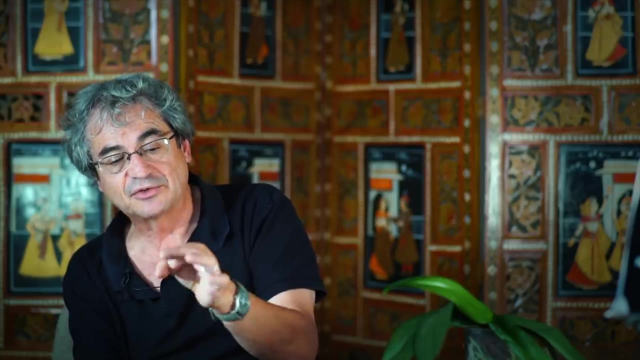 And we don't know, It's recent stuff, so ideas change, But I'm pretty convinced that the bounce from a black hole to a white hole, which was our main idea, that's solid If it happens at the very end of the evaporation. 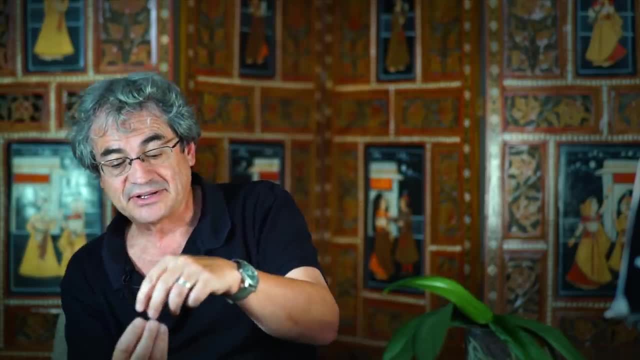 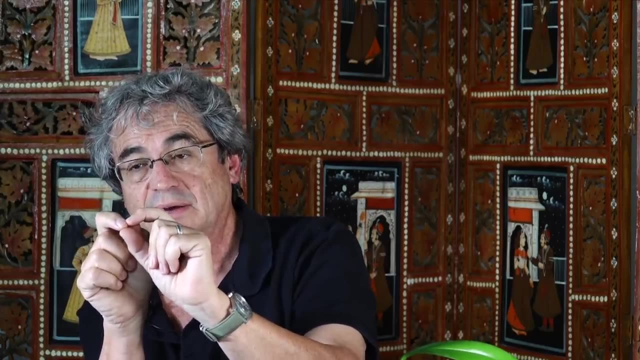 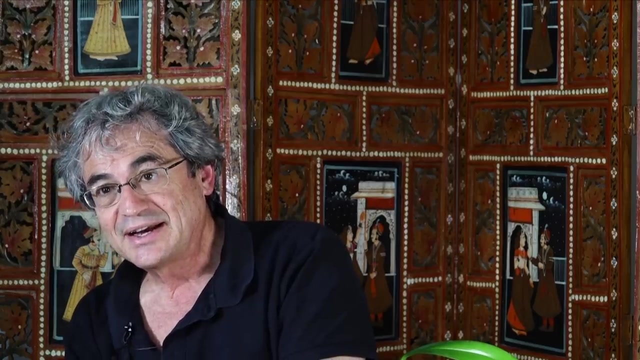 what comes out is a white hole, but a white hole which is very skinny, And this can stay there for a very, very long time before it dissipates all what is inside and come out, And these are the white holes that, if they existed in a previous eon. 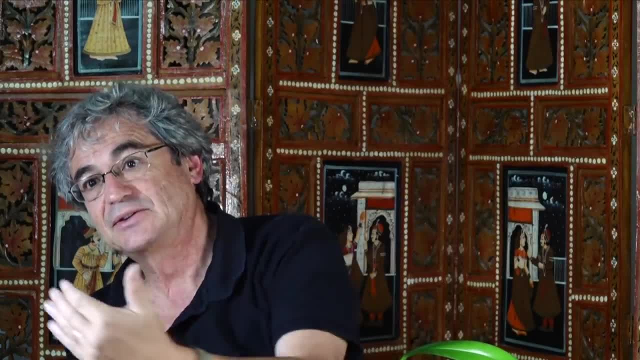 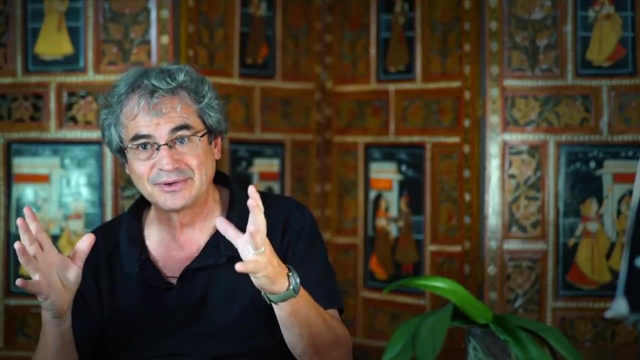 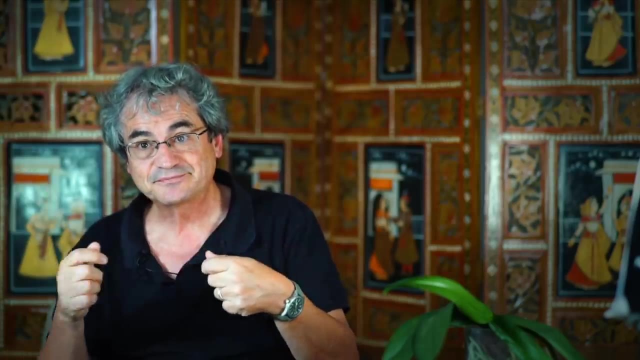 before the bounce, before the Big Bang, they had gone through the bounce. A couple of students of mine did calculations which seemed to indicate that no, no, no, no, no, it's very improbable that they explode when they are. We compute the probability, the probability of explosion, as a function of time. 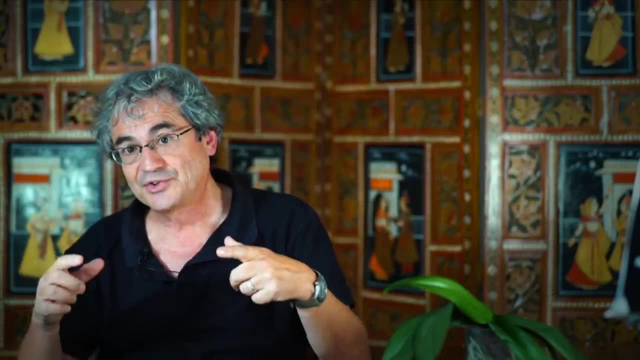 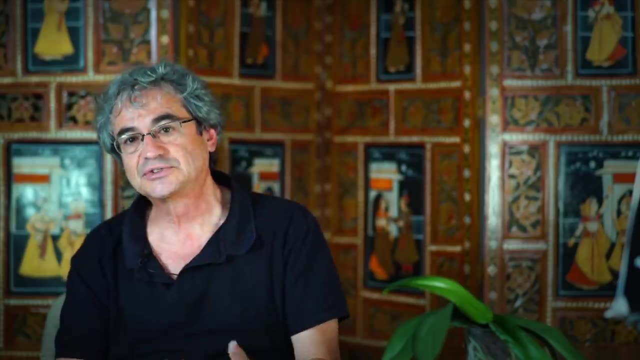 And their first calculation is that probability is too low, too small, So it becomes high only when the black hole shrinks down to small. Now it's a first-order calculation. We have to go next order. We don't know how reliable it is, but it goes the other way. 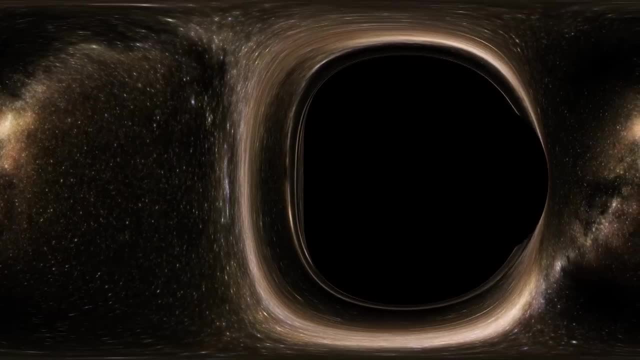 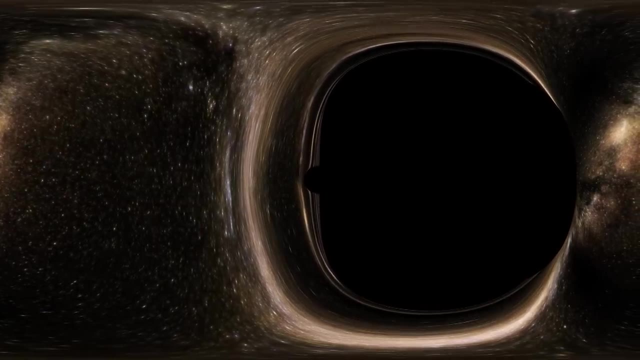 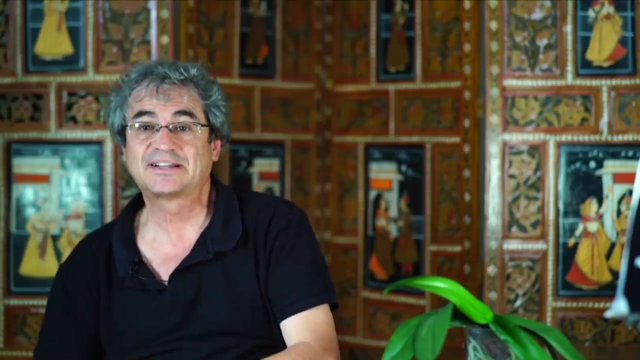 So we're in the middle of this, whether it happens when the black hole is large, and then it might be connected to the faster rebirth, or when it happens when it's very small, And then the hope to detecting it is through these remnants and connecting to dark matter. 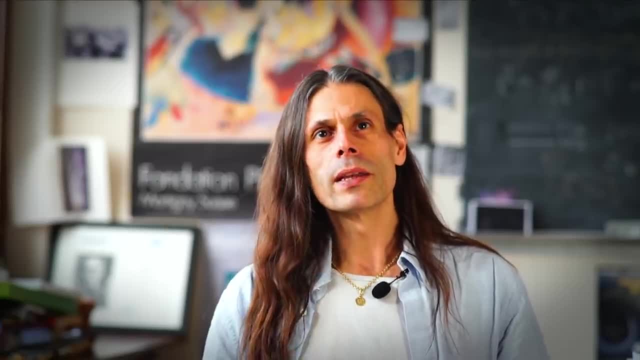 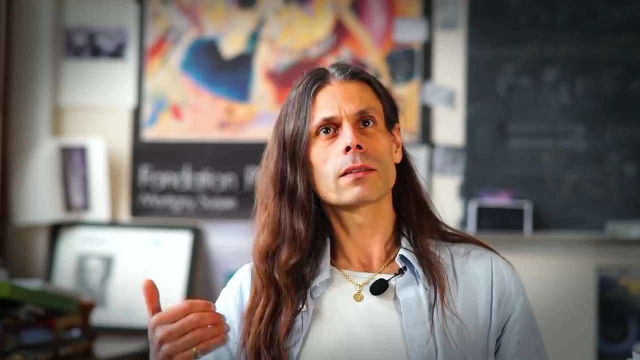 The reason of the discrepancy of the debate, of the controversy, is about the stability of the bounce, And it's true that the bounce can be made more stable if it is not symmetric, But it will not change the energy of the emitted quanta. So, as far as observations are concerned, you don't really care about knowing if the bounce is symmetric or not. The key point right now is: how much time does the bounce take? It might be less than the edge of the universe for some light black holes. 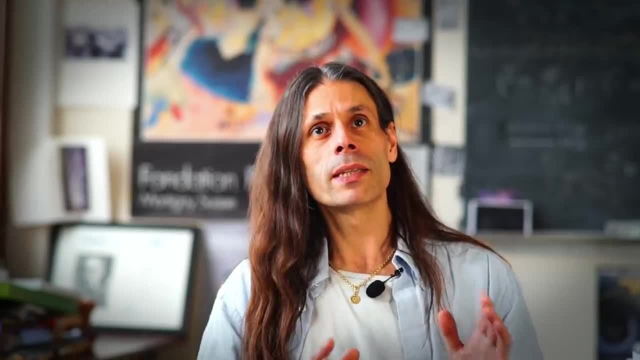 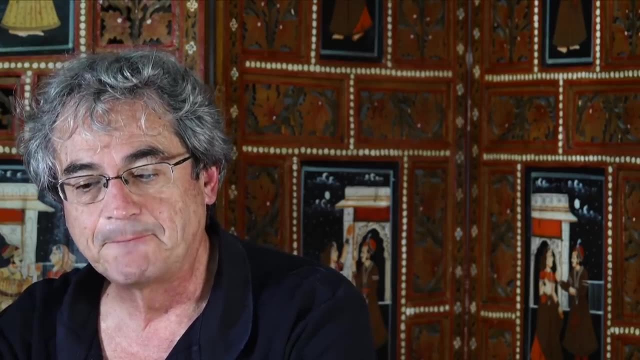 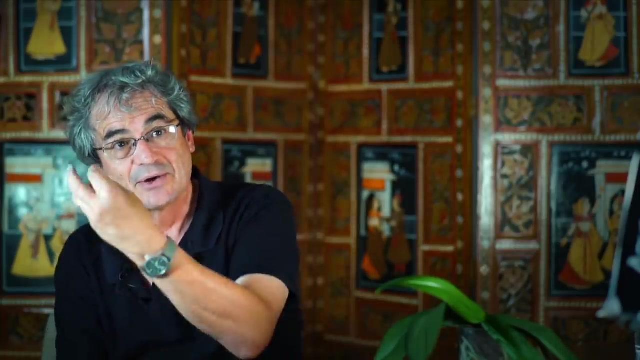 or it should be much more for the very same black holes, depending on the assumptions. Recently we have worked out a rather speculative idea, which is the possibility that something goes through the bounce. this cloud of small black hole remnants might go through the bounce and constitute a part. or maybe a large part of dark matter. I'm just mentioning this idea. it's speculative, it's new, it's not tested, But if it works it would be pretty good evidence of a bounce. Any kind of matter content will be destroyed by the bounce. This is obvious. In my view, the only two things that could survive the bounce are gravitational waves, because they are very weakly coupled to matter, and black holes. So black holes and gravitational waves might survive the bounce and they might be footprints of what happened before. There are interesting mathematical developments that show that it is possible. They are exact solutions of the equations of motion, for example with the bounce and black holes, So it is possible that they survive. Do they really survive in motion In real life? it's extremely difficult to say. 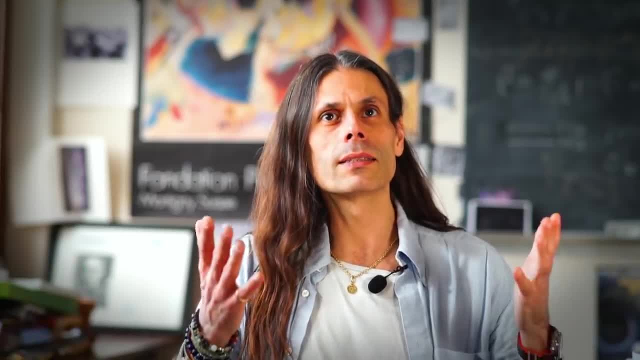 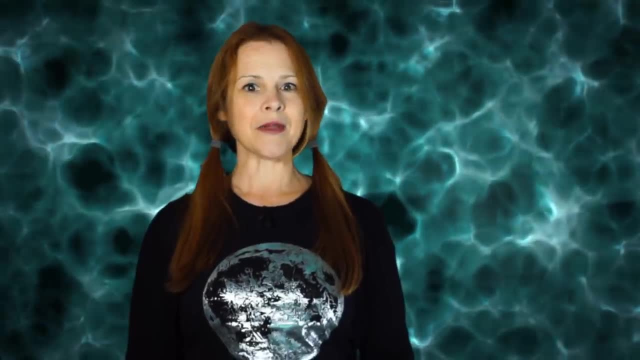 because we don't even know what was the matter. content of the universe at this time. Loop quantum gravity is one of the most exciting prospects for a quantum theory of gravity, and it may well be on the verge of experimental testing. These impressive advances have occurred. 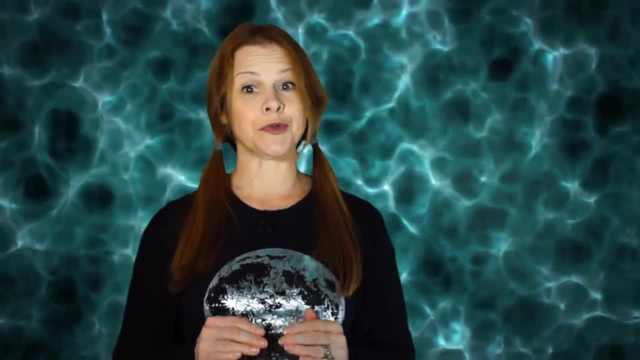 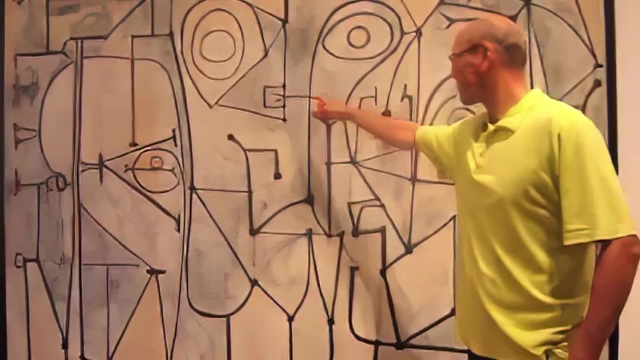 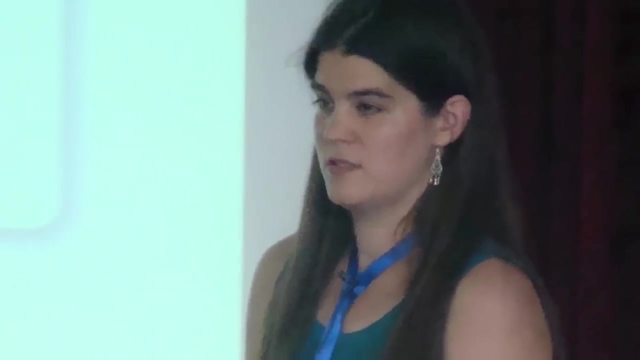 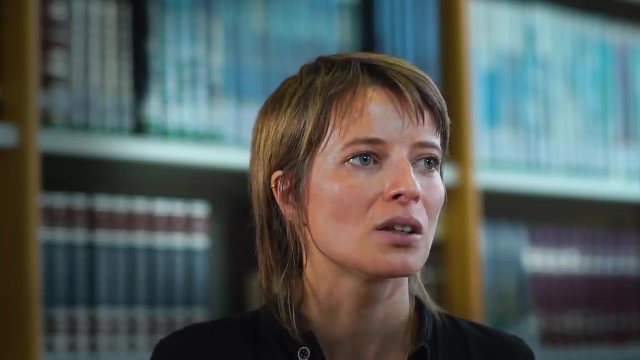 thanks to sustained creative contributions of several hundred researchers, including Barbaro Tiemann, Veraderogen, Lewandowski, Barrett, Friedel, Dittrich, Giesel and many others. So what comes next? We have a foundation of loop quantum gravity that is very solid. 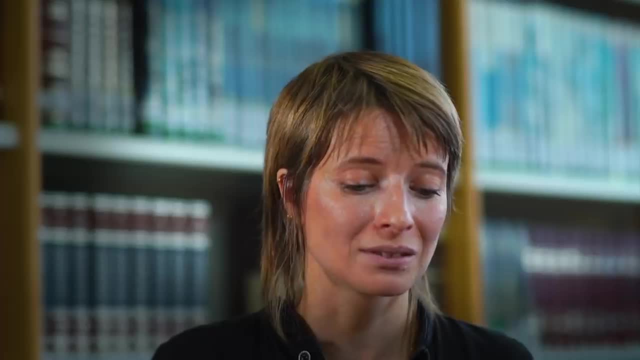 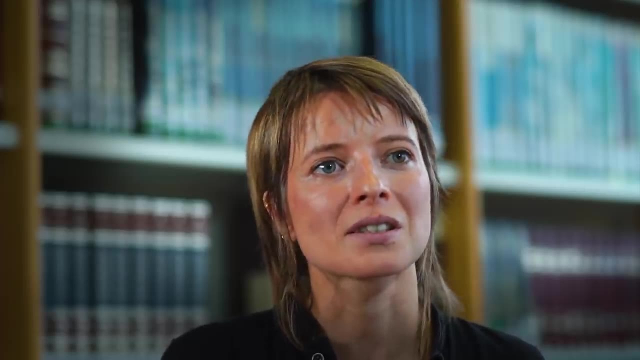 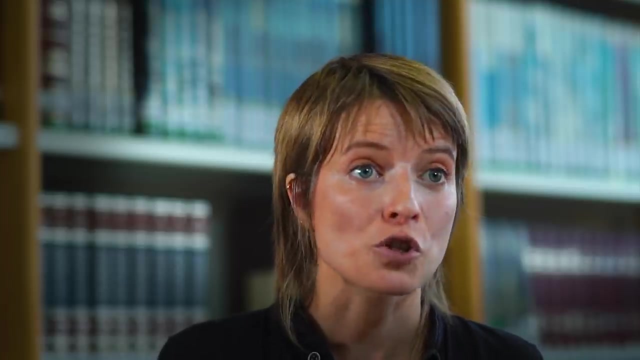 We have control about the fact that, whatever the shape of the theory will be in ten years, some things will not change. The discreteness of the area, the volume and so on will not change. The fact that the curvature is bounded will not change. 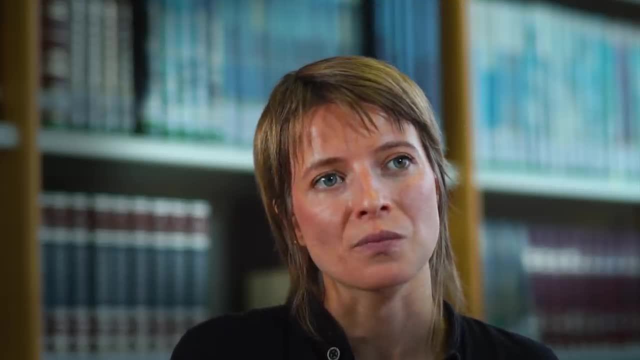 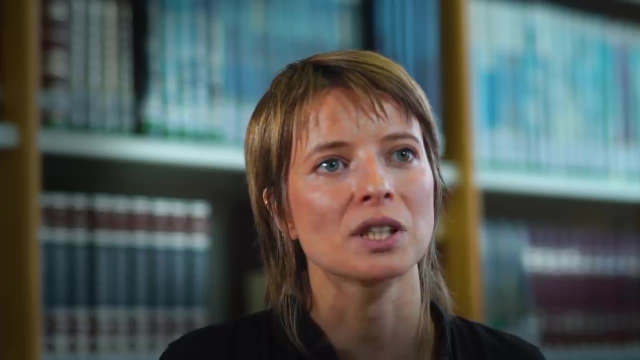 So we need to use this information to make predictions, to study the phenomenology. At the same time, of course, there are open questions also in the mathematical aspects of the theory, And I think that so far it has been underappreciated. 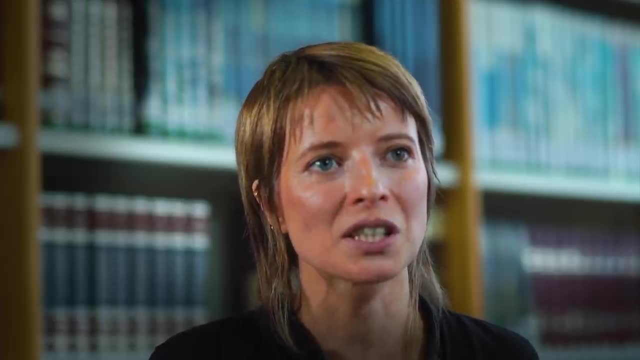 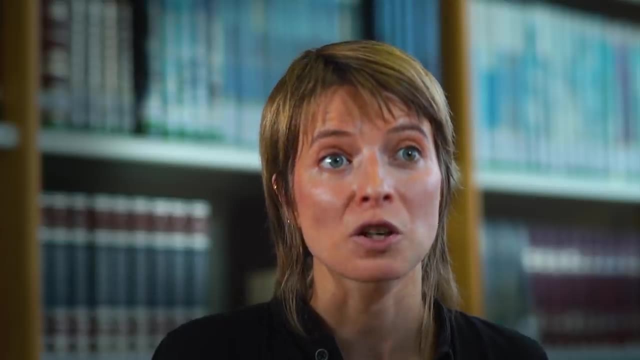 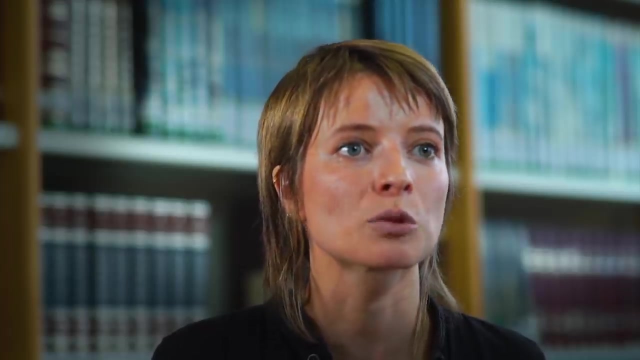 the fact that there is a beautiful mathematics related to group theory, with Chern-Simon theory, with quantum groups and so on. that is really very interesting to develop. So I hope that both mathematicians and astrophysicists will get more and more. 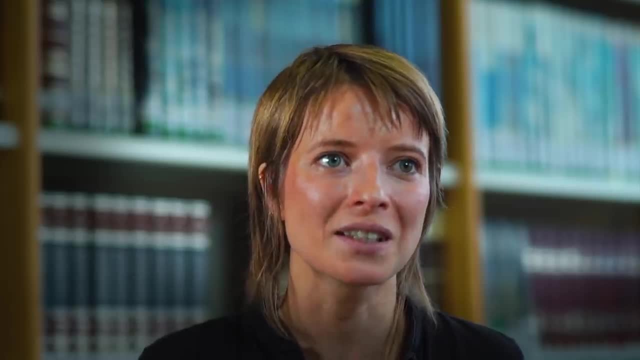 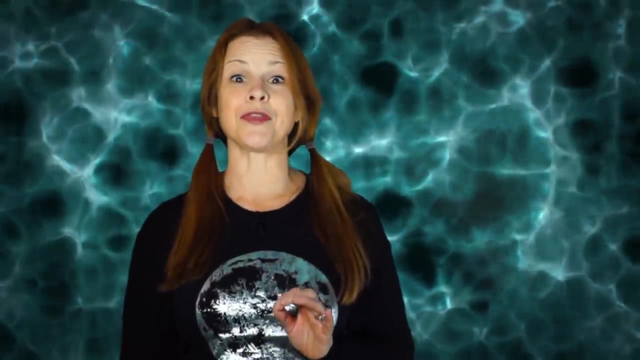 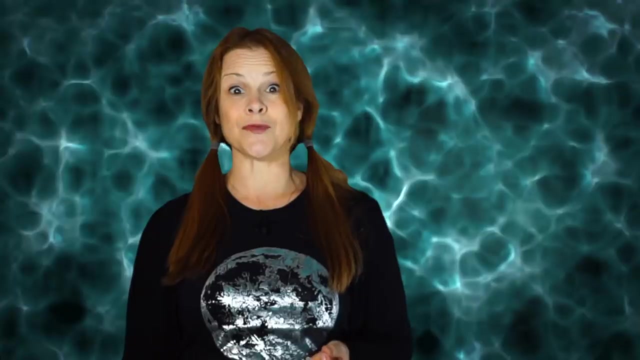 interested in what we are doing and will try to help us to develop the theory in both directions. Loop quantum gravity has been around for more than three decades And while it has made impressive advances, there is still, of course, the possibility that it is wrong. 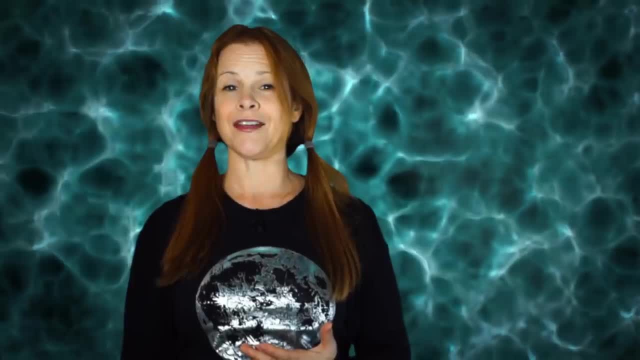 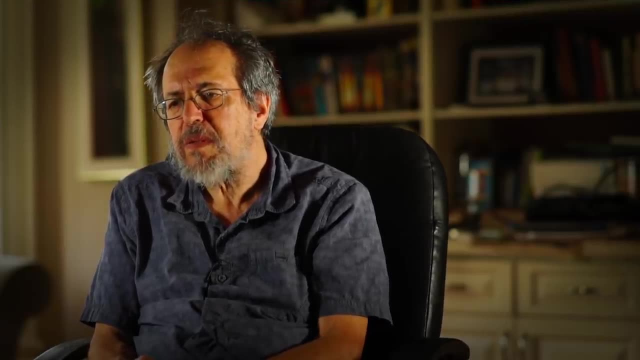 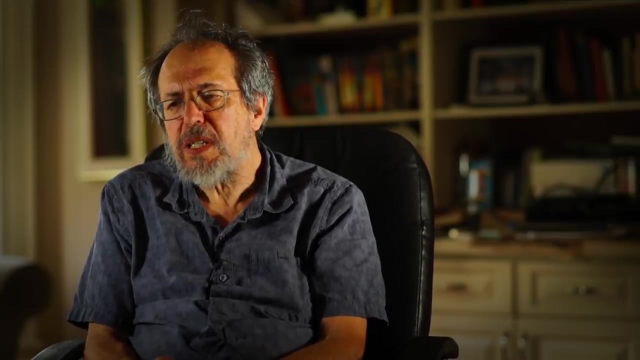 So how does it feel to risk so much time and effort without knowing if it will really pay off? There are very few times that a theoretical physicist has the opportunity to be part of starting an area, starting a research program And in loop, quantum gravity. if we don't yet know that it's the right theory of quantum gravity. 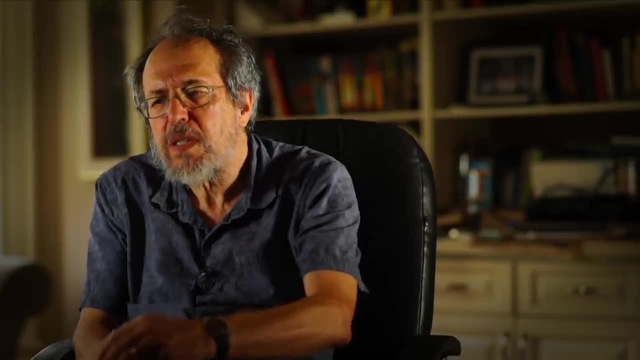 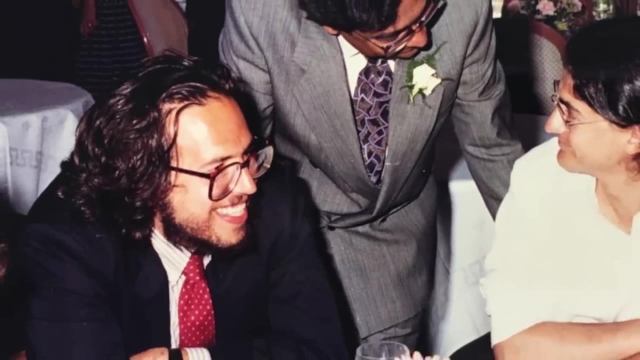 we know something absolutely marvelous in my opinion, which is that it's the way that the world might be. It's been an enormous privilege to have the experience of being part of the adventure of quantum gravity, And I'm grateful to everybody involved. 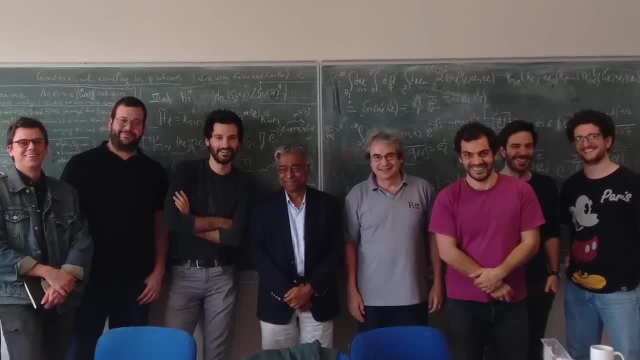 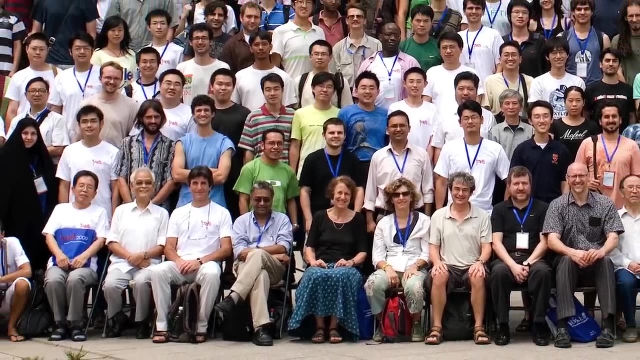 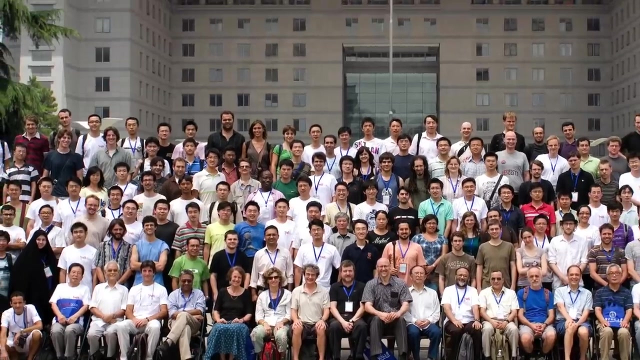 Abai, Carlo, Ted Louis and all the others. And then I'm also so just amazed by all the young people who come in and so brilliantly develop the subject. So it's a real. it's the privilege of my life to have had the chance to be involved with this, whether it's right or not. 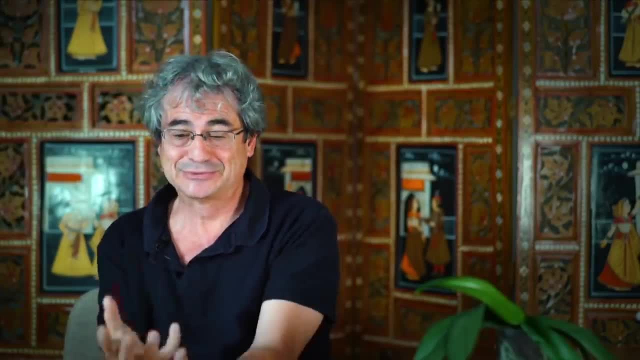 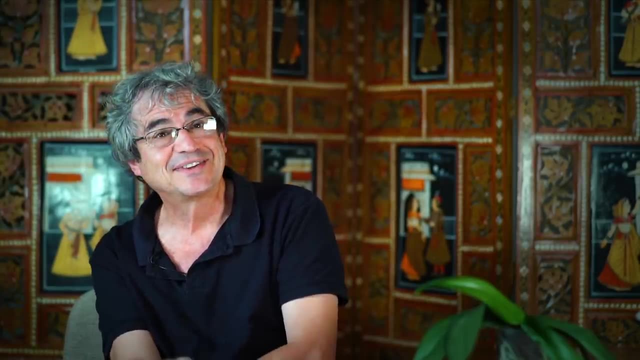 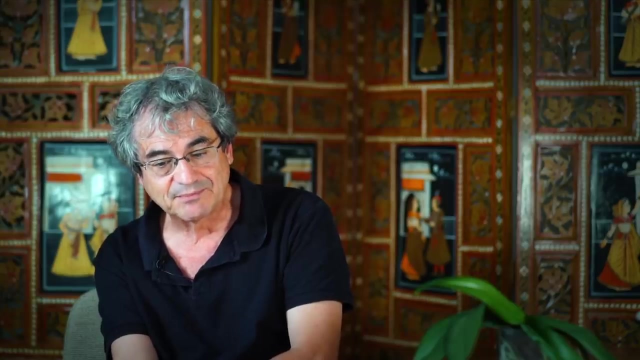 Sometimes I ask myself: well, why didn't I work on some more concrete problem which I could see the yes and no in? But you know, life it was, it is, And if all the work I've done in my life will turn out to be, 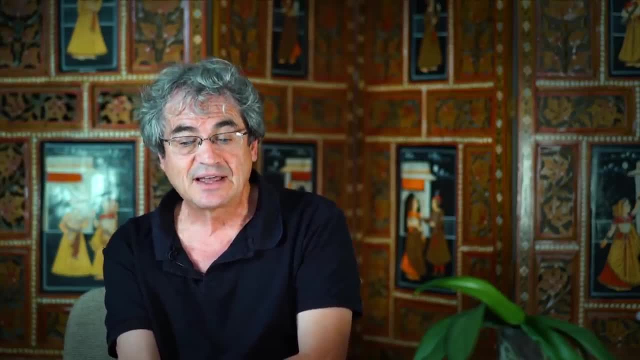 significant for understanding nature, I'm super happy. If only a small part or nothing at all of it, Well, I'll still be happy. less happy, but still be happy. It's been a fantastic life: working with friends, discovering, trying to discover stuff. 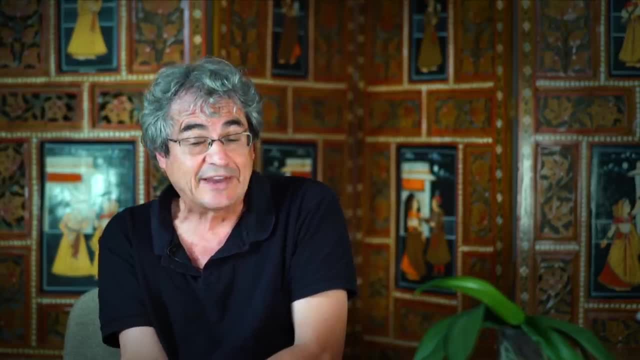 Investigating nature is great fun And we have to try. There is no alternative than than trying.